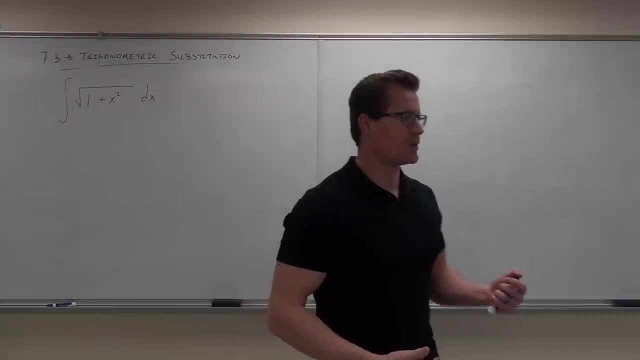 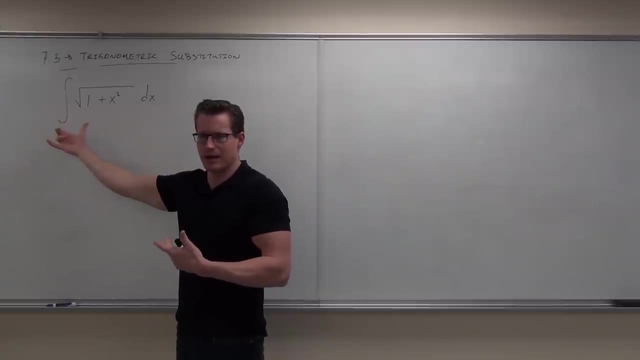 Okay, is integration by parts going to work? No, Not really Is, because if we have a piece of an integral, this thing would be the other piece. That'd be bad. We'd basically do integration by parts when we have a product in there somewhere. 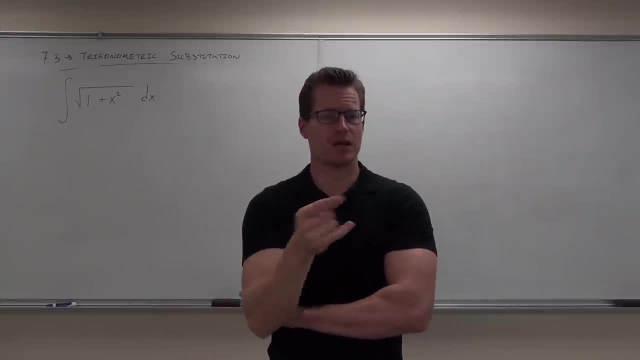 Alright. well, if we don't have that, is it a trig integral? Does it have sines or cosines? That's a part of it. Okay, so we can't, then we can have something else. Here's the something else. 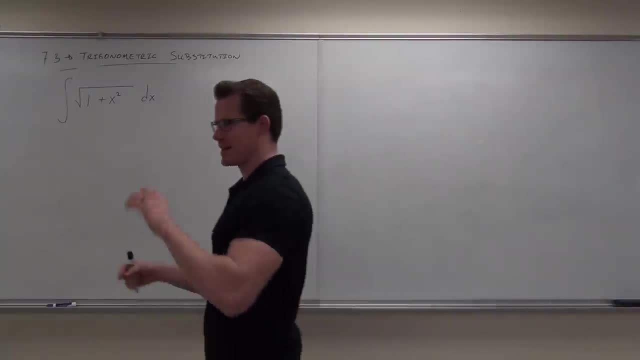 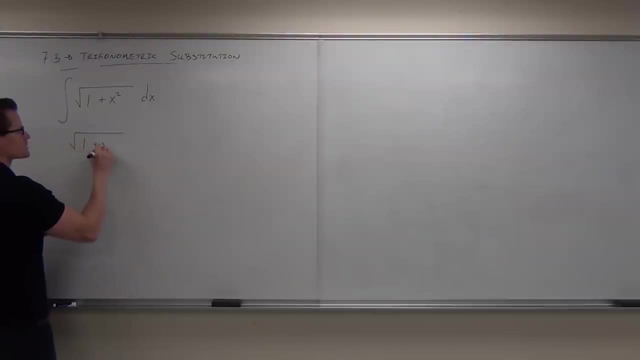 The idea is: let's kind of change this, let's think about this in kind of an out of the box kind of way. Let me just consider the square root of one plus x squared. Now, somewhere along the way, someone said: well, wait a second, you know what? 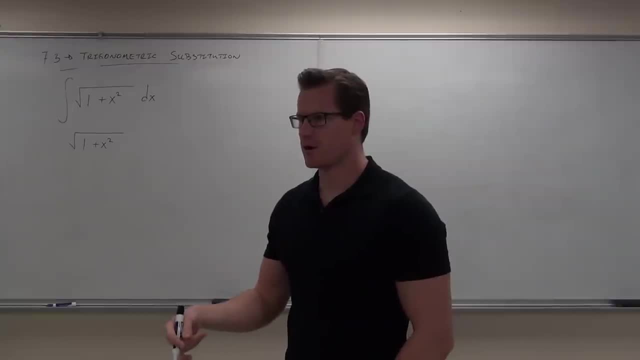 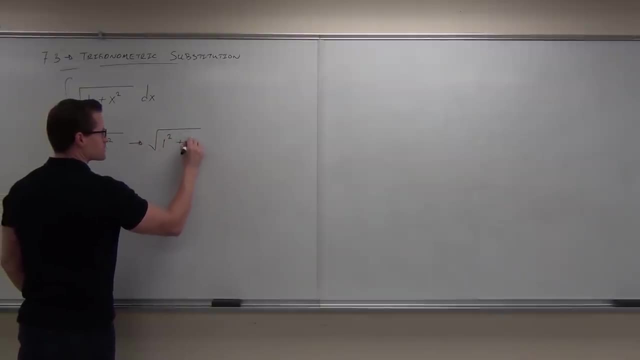 this looks a whole lot like Pythagorean theorem- a whole lot like it, In fact. this looks like I could do One squared plus x squared: same thing. yeah, Well then they said, wait a second if that looks. 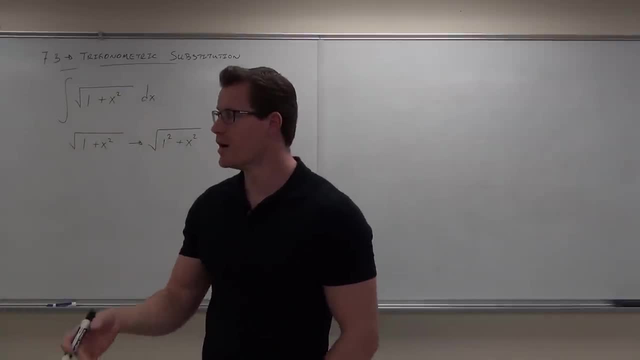 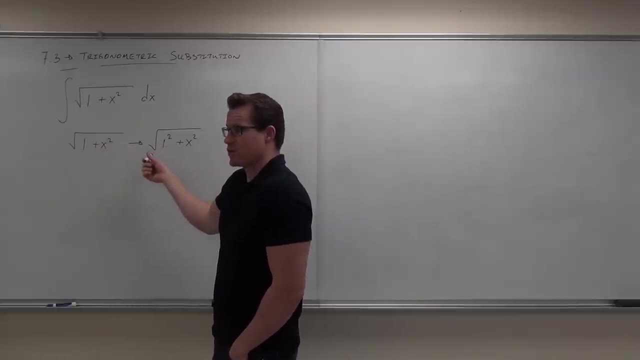 like Pythagorean Theorem, the stuff that we would get by Pythagorean Theorem, then maybe we can make a triangle out of this thing. So they said, well, can't do it like this? Well, this looks really similar, so let's make a triangle. 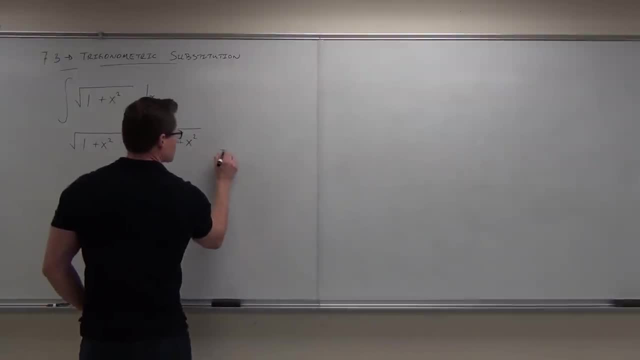 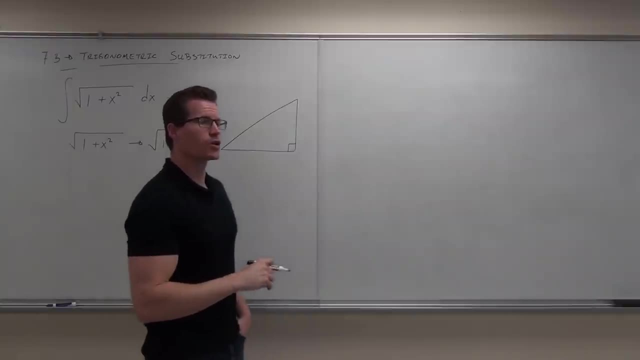 and see if we can actually use that. Here's a crazy idea. So we create this triangle, And what we're going to do is we're going to fit this piece of junk that we can't deal with as one of the sides of our triangle. 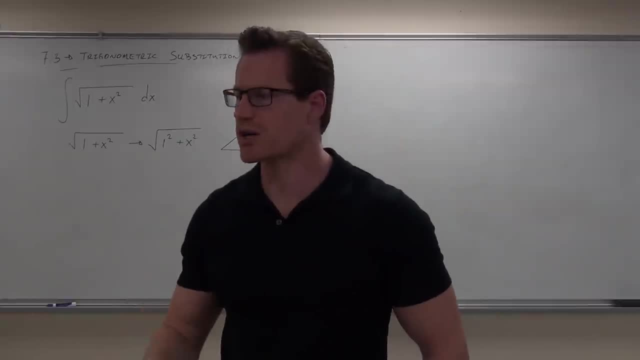 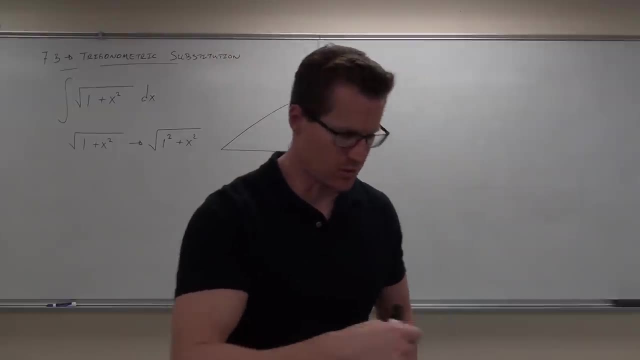 The whole deal that you're going to develop here in this whole section. I don't really want you memorizing a lot of the formulas I'm going to give you. There's only three of them. I don't want you to have to sit through and memorize. 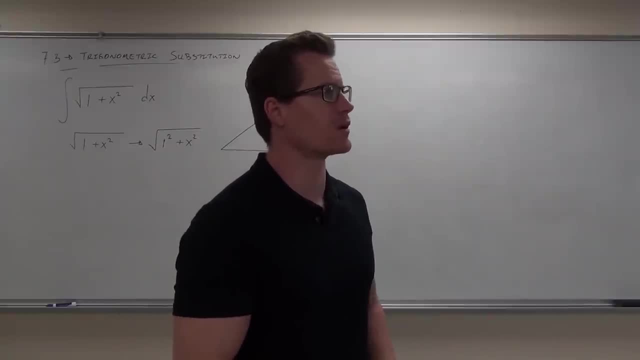 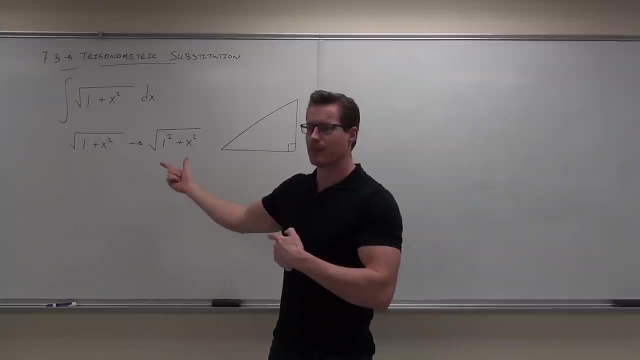 with flashcards. I want you to understand the concept. what is actually happening here? What's actually happening is that we're going to take this and we're going to make it a side of a triangle. Now there's a very specific way. 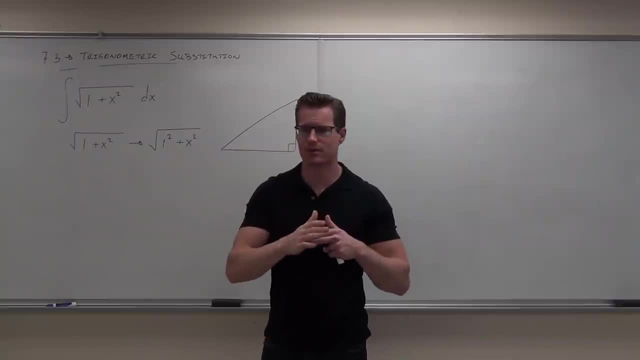 that you can do this. You have to tell whether it's a leg or whether it's the. what's the longest side of a right triangle? Hypotenuse. Whether it's the leg or the hypotenuse, It's not hard to tell. 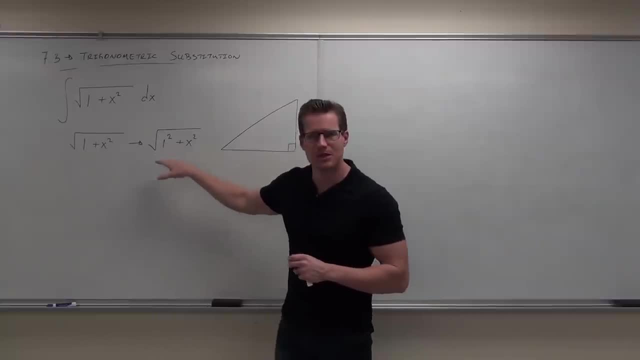 What would this be? a leg or a hypotenuse? That has to be the hypotenuse. The only way that happens is if I have a leg squared plus a leg squared, then I take a square root. That gives me the hypotenuse. 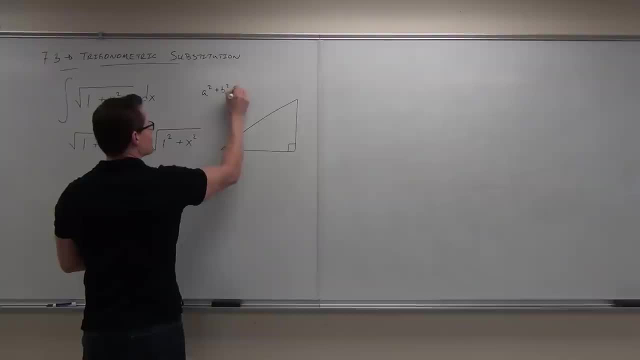 Remember this: A squared plus B squared equals C squared. Check it out. If it's This, Hey look it. If it's this, then this thing stands for a hypotenuse. Are you with me on that one? If it's this, what's that? 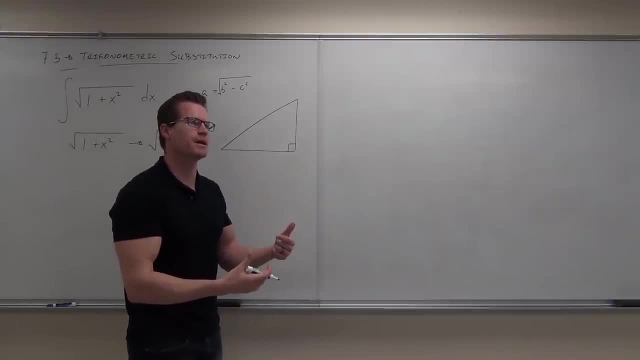 It's a leg. It's got to be a leg. Do I know which one? Well, we'll talk about that in a minute. You can choose. We'll pick correctly. There's only one correct choice, but we get to choose. 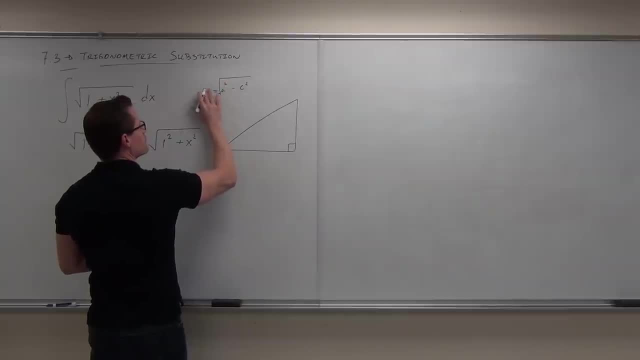 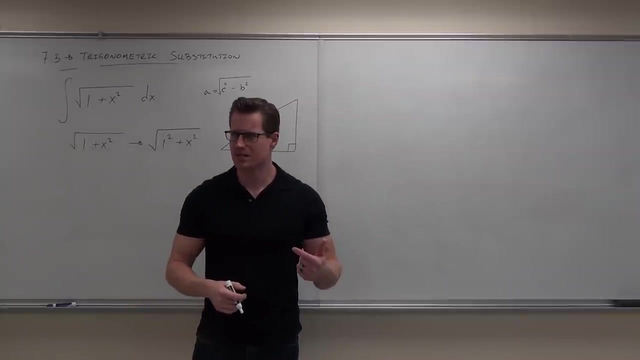 Or if it's the other way around, That's also. oh sorry, you know what that was? stupid, same thing. I meant this. Or if it's that, That's also a leg. Did you guys get the idea here? 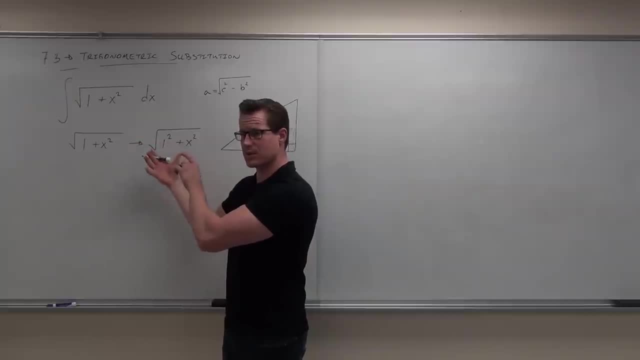 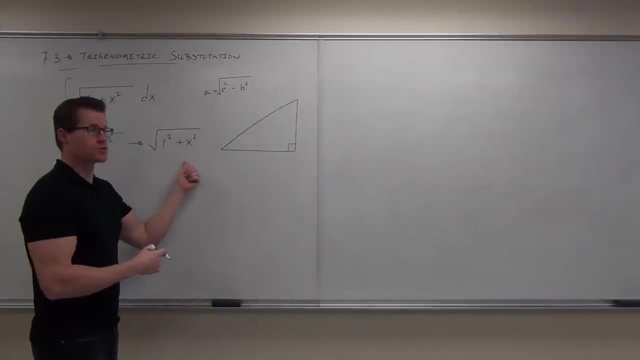 So somehow we can fit this square root of something plus something or something minus something as part of a triangle. In our case, this is wait a minute. the only way that I can make this fit a triangle is if this is the hypotenuse. 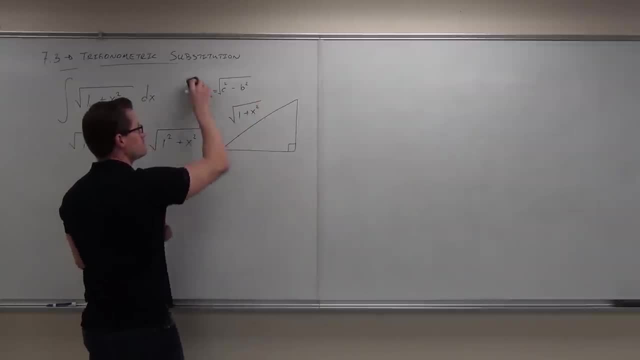 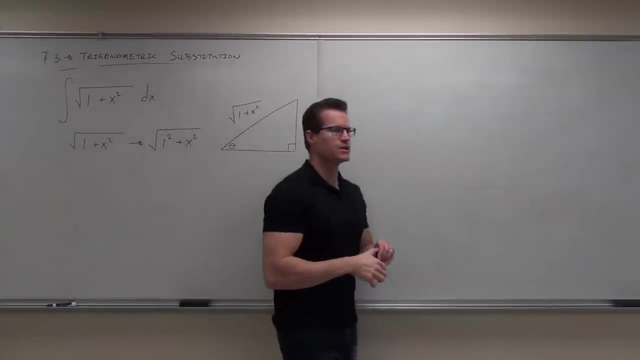 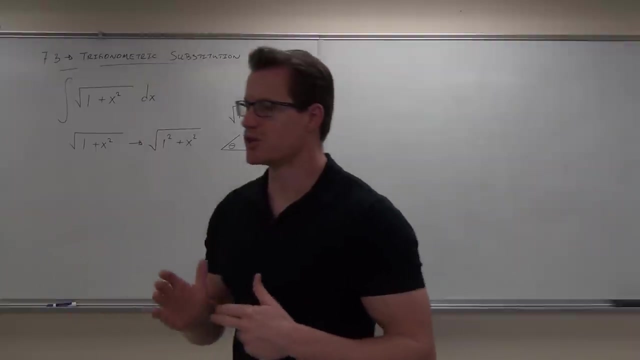 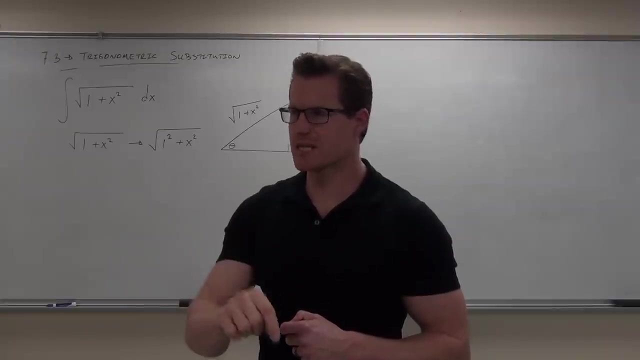 This is the hypotenuse, and this is my angle, and this is my angle, and this is my angle. Now here's the deal for the rest of your triangle. your idea is going to be to try to make the sides in some relationship that allows you to create tangent, sine or secant. 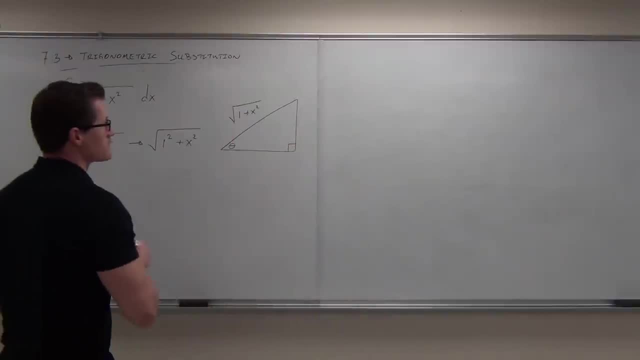 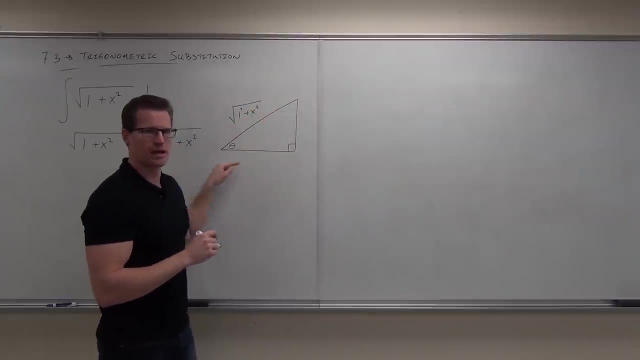 where you have a variable over a constant. So I'm going to do this, I'm going to do this. I'm going to say: wait a second, if this is square root of 1 squared plus x squared, can you tell me the lengths of these sides? 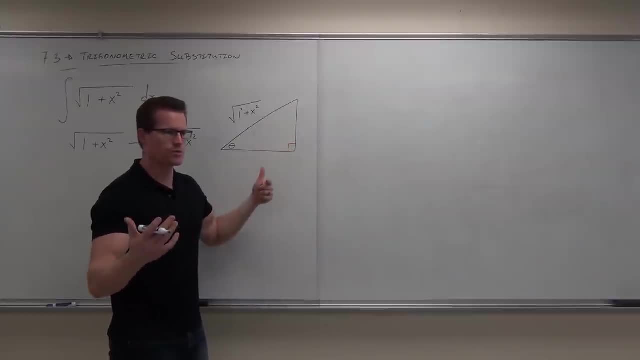 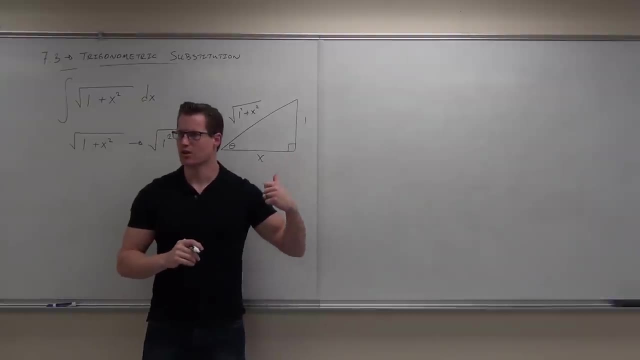 It's a piece of cake. One of them's x, one of them's 1.. That's it. Now, if I do this, 1 and x, that's a cotangent. Cotangent's really hard to deal with. 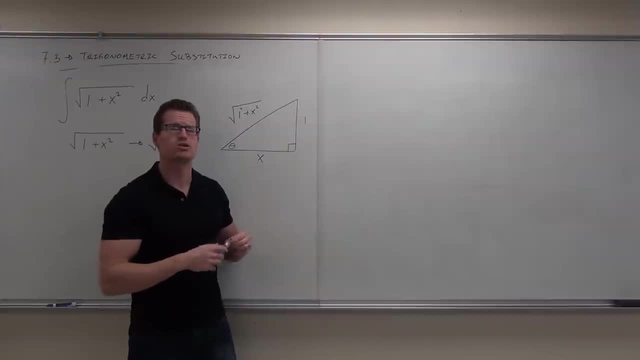 Okay, you know what? I kind of skipped a point. We're going to use a relationship here that allows us to not work with this one but work with the trigonometric relationship of the other two sides. So I don't like the square root. 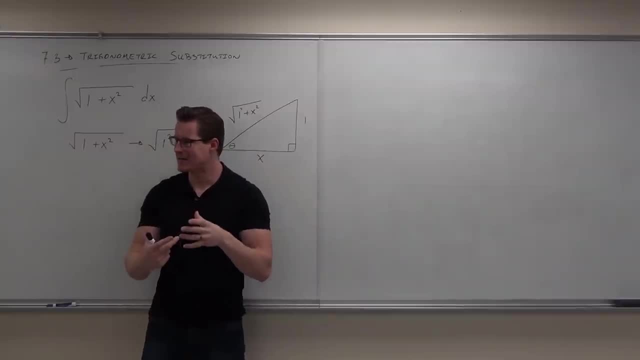 That's fine. It's really hard to work with, So I want a trigonometric identity that lets us work with the other two that don't have square roots- the easy parts of this. Does that make sense? So we'll make it easier. 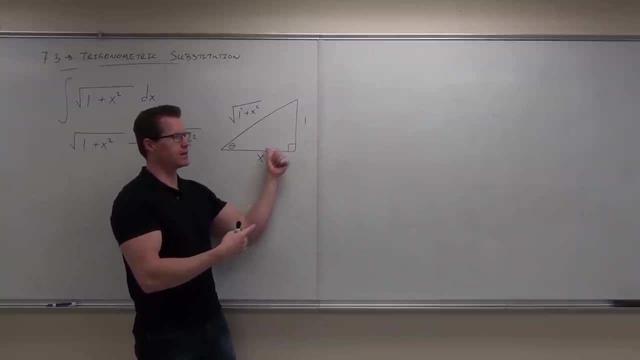 If I do this 1 over x, well then I'm not really going to get something nice, I'm going to get cotangent. Those don't have some nice. those have an identity. but we try to stick with easier identities. 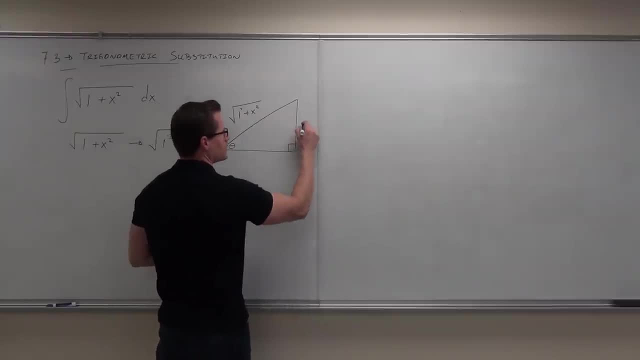 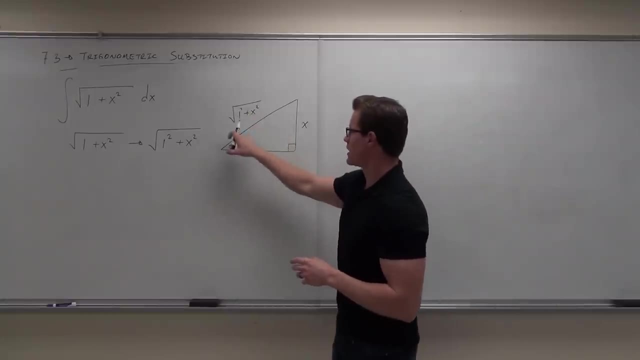 So I'm not going to do 1 over x, I'm going to do x over 1,, x over 1.. Now here's the plan. The plan was: If this is part of our triangle and now we have our other two sides- x and 1,- 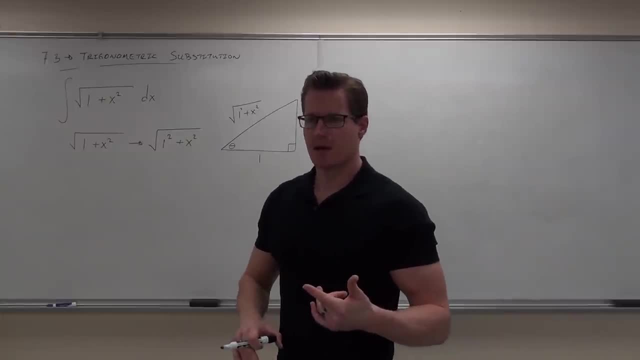 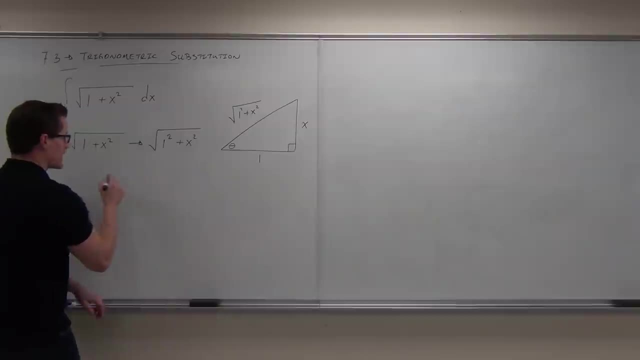 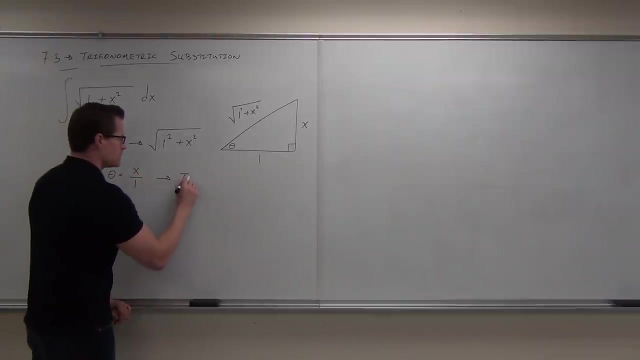 let's pick a trigonometric identity, trigonometric function actually, that allows us to relate the two other sides in a really nice fashion. For instance, if I look at tangent, tangent is for this specific triangle, I'm going to just tangent x over 1, or tangent. 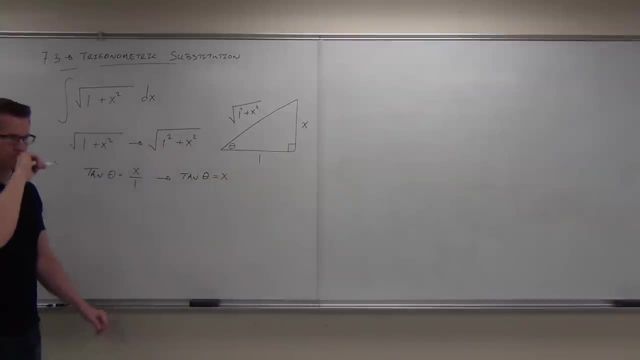 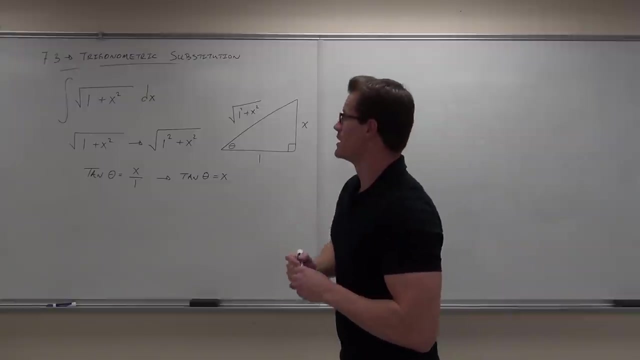 Tangent is, Tangent is. So we have tangent theta. tangent theta is simply simply x. That's great. I really need you to get this idea before we go any further. I want you to really see what's happening. What's happening is: we don't know how to do this. 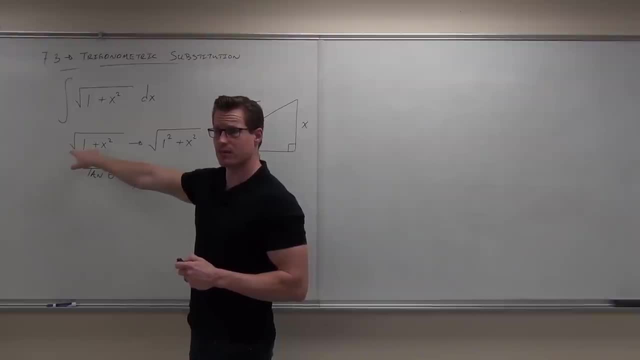 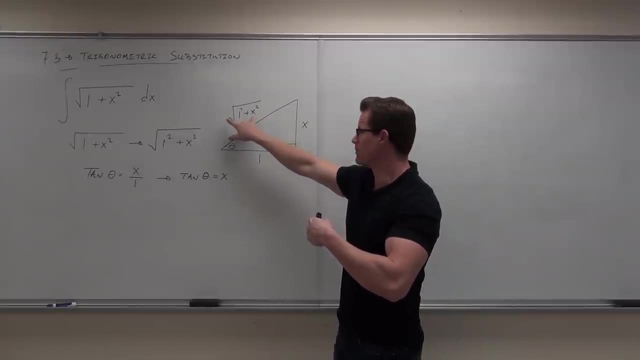 We take this part away, We go. you know what That looks? a whole lot like part of a triangle with Pythagorean theorem. Let's make it be part of a triangle like Pythagorean theorem, Then we can find the other two sides of that right triangle. 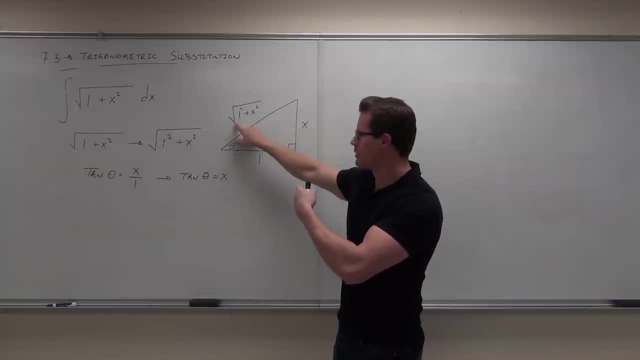 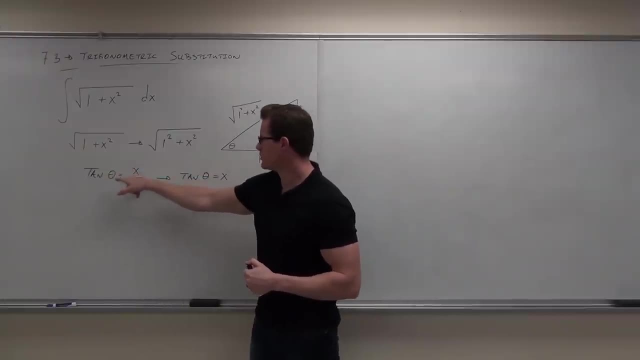 Well, it's really easy. I'm going to give it to you. One of them is 1.. One of them is x. We put them in this relationship. That way, when we do tangent of our angle, we get simply opposite over adjacent. 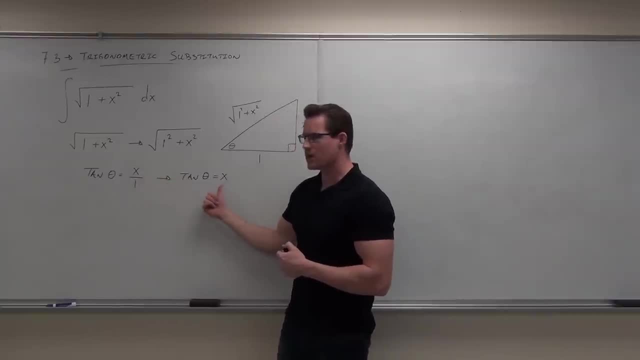 We get x over 1, or tangent theta equals x. So it makes you feel okay with that idea. It will become more clear, I promise you. there are a lot of examples. I'll also give you some of the formulas, but I'm going to teach this to you in a way that it makes sense. 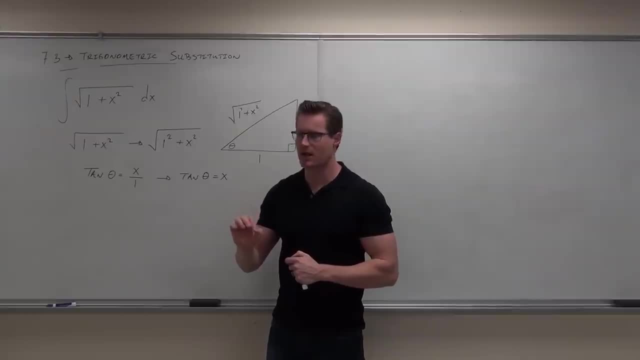 not that you just follow the pattern, Okie dokie. it does have to make sense to you Now. it'll become easier if it does. This is what is awesome about this. You agree that tan theta equals x. correct, Tan theta equals x. 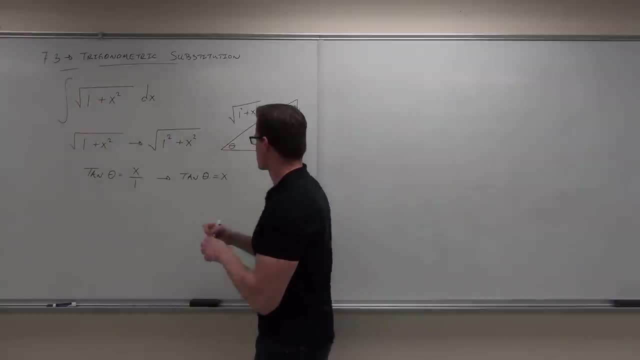 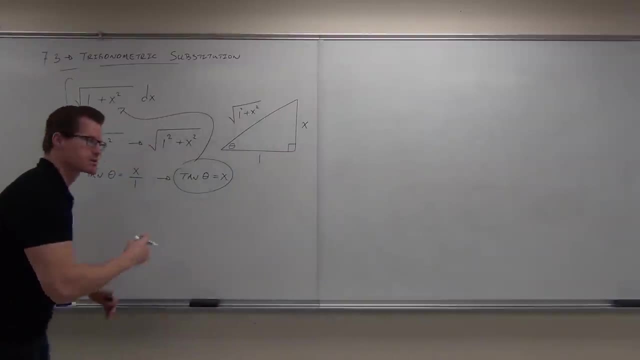 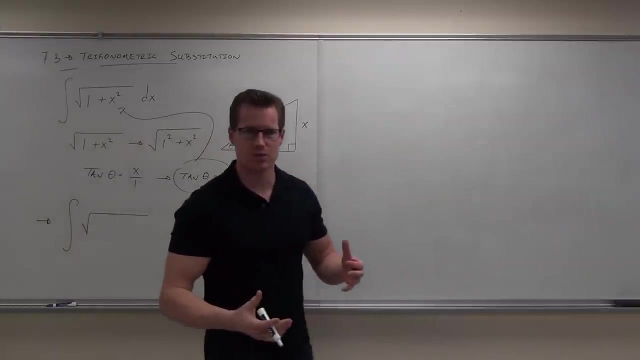 Tan theta equals x. That allows us to do a trigonometric substitution. So we'll have an integral. We'll still have a square root. Notice we're not substituting for the square root. We can't do that because there's nothing to get the derivative away. 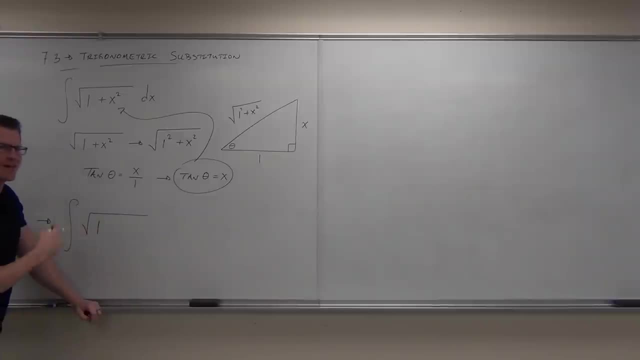 Square root. We're still going to have a 1.. Are we still going to have an x? No, No. Instead, what is our x? Tan squared theta. So we're going to have tan theta. Wait a minute, Just tan theta. 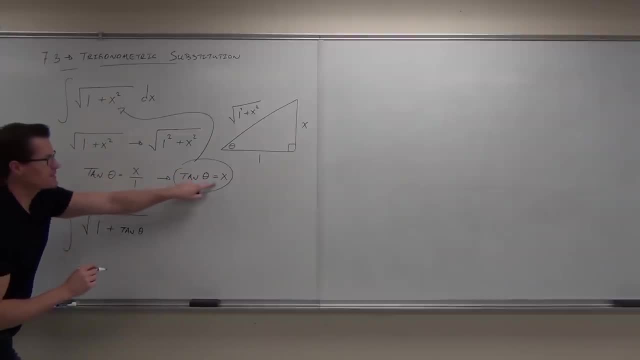 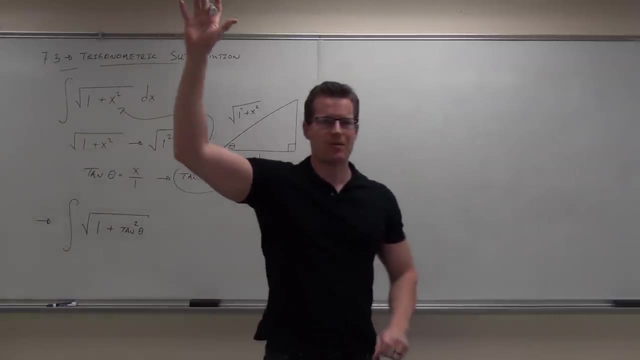 Tan squared. This was x squared. Hey, look at that. Tan theta is x. This becomes tan squared theta. I want to show our hands if you feel okay with this. so far, Remember those times your calculus 1 teacher- maybe it was me- told you: don't forget your dx. 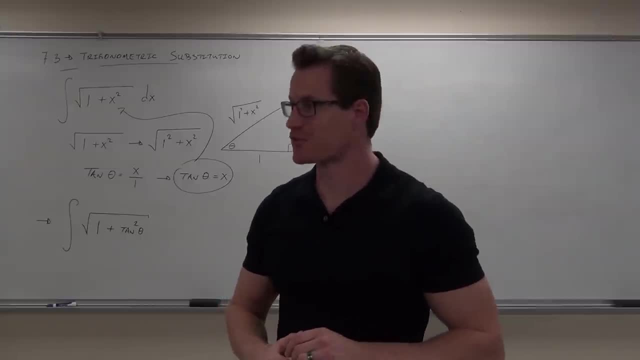 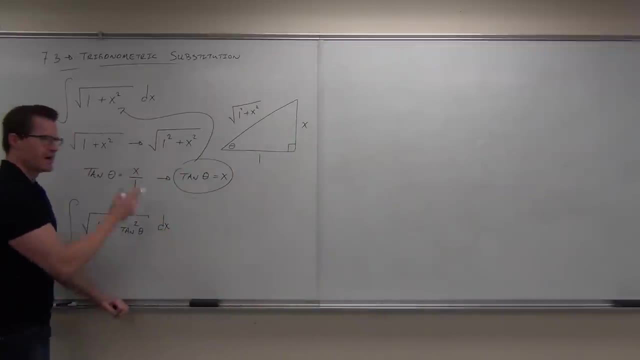 Don't forget your d theta, Don't forget those. Remember that And how some of you still forget the dx and all that junk that you think is irrelevant. Here's what's not irrelevant. If you just leave that as dx, does this match your? 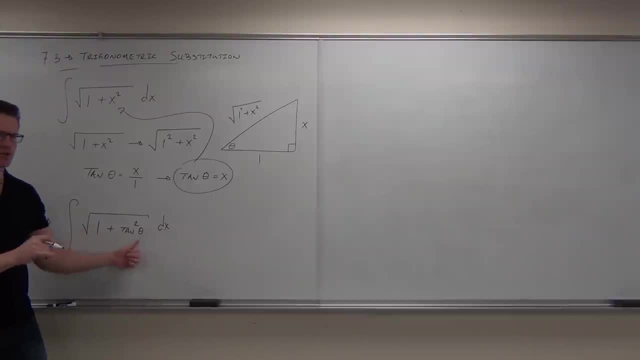 No, No, This is an issue. These have to match. Your variables have to match. So what in the world do we do with that dx? It's really similar to doing a u substitution- Really similar. So we have tan theta here. 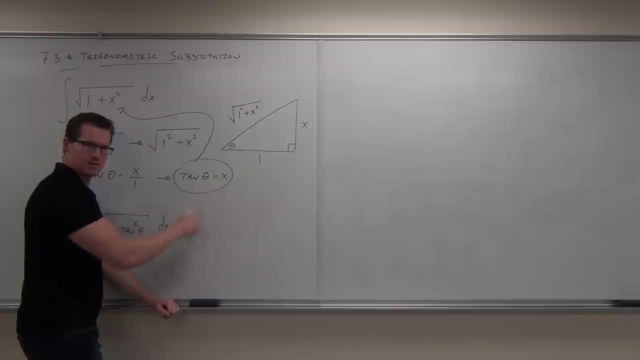 We have x. Can you figure out what dx is? Take a derivative. Take a derivative. What's the derivative of Secant squared? So secant squared theta equals how much Dx? Ah, Now we know. So this part becomes our dx. 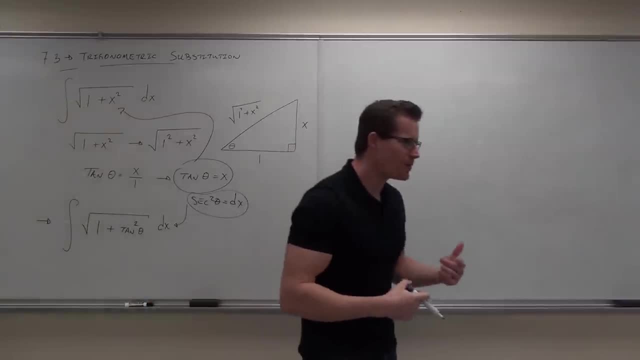 I'm going to work over here, but it is. it's not a really complicated idea, but it's kind of it's new for you. I know it's brand new, So I want to make sure that you guys are okay with exactly what's going. 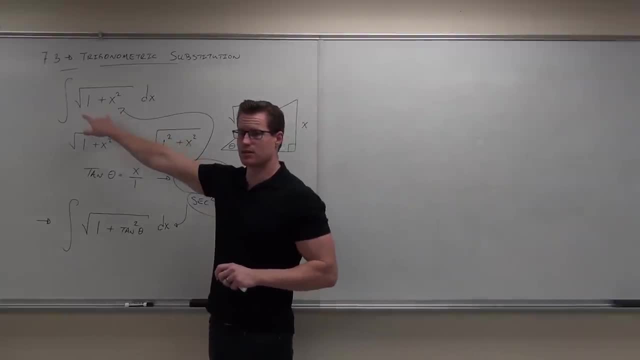 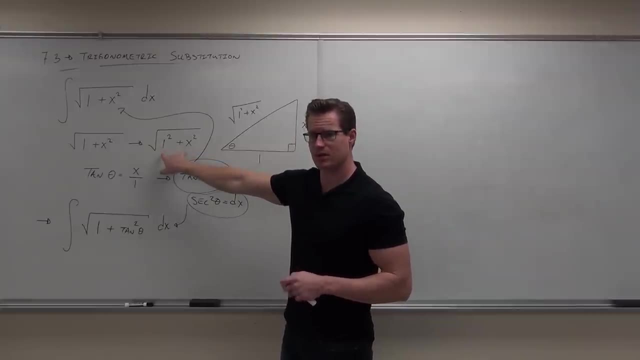 on here before we go any further. You understand we can't do this the way it is correct Can't do it, So we pull it off. Do you understand that this is a hypotenuse of a right triangle? It's got the plus there. 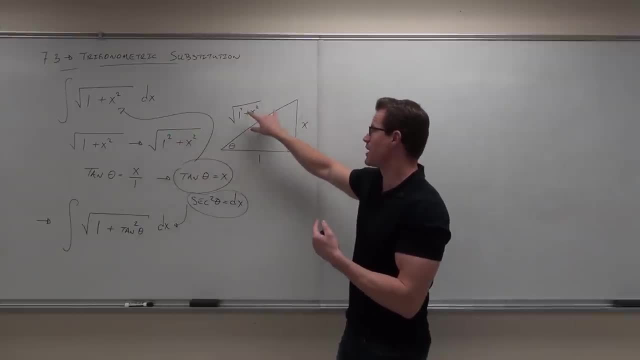 It's a leg squared plus a leg squared, and then we take a square root. That is the distance of a hypotenuse. If we do that, it gives us one leg and the other leg upon which we can make some sort of a trigonometric function. 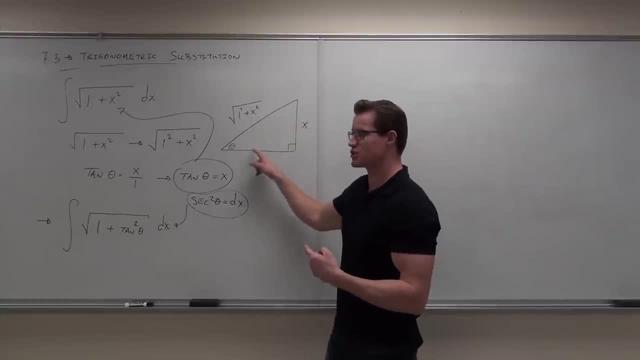 a relationship amongst those two sides. Tangent is the appropriate relationship here. It's nice. We don't want to do cotangent. It'd be 1 over x. That'd be silly. I want to do tangent and get x over 1.. 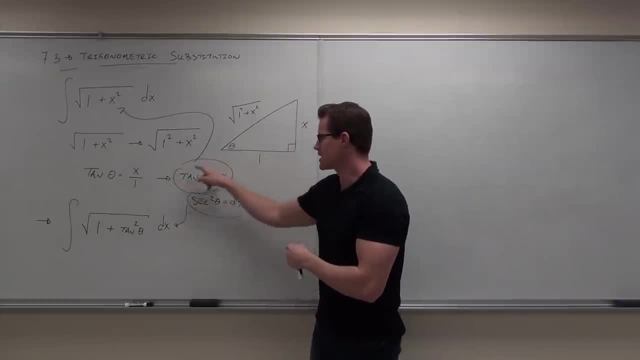 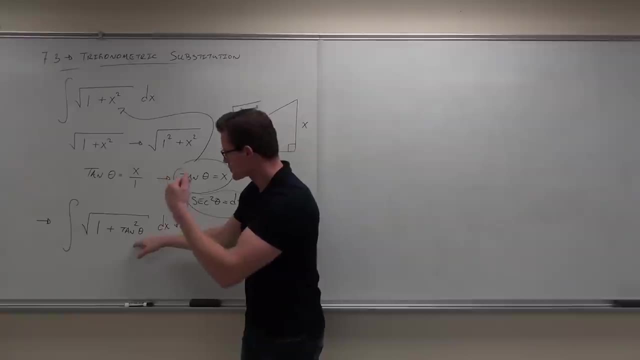 That way I have a nice substitution. So tangent equals x, tan theta equals x. We plug that in for x, So 1 plus tan squared theta. We still have a square root. Dx is an issue. We've got to change that. 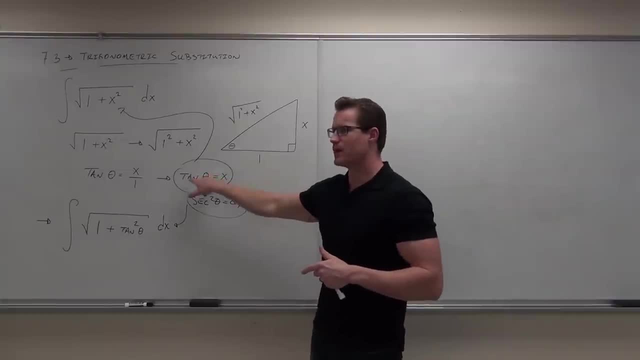 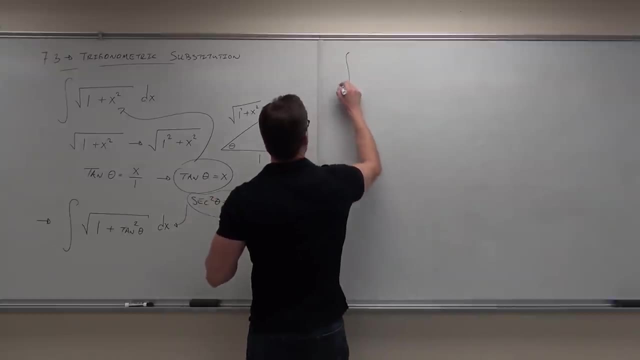 So, just like you did on a u sub, you still take a derivative. So tan theta equals x. No, no, no, Let's do: secant squared theta equals dx. Then we get okay cool integral of square root: 1 plus tan squared theta. 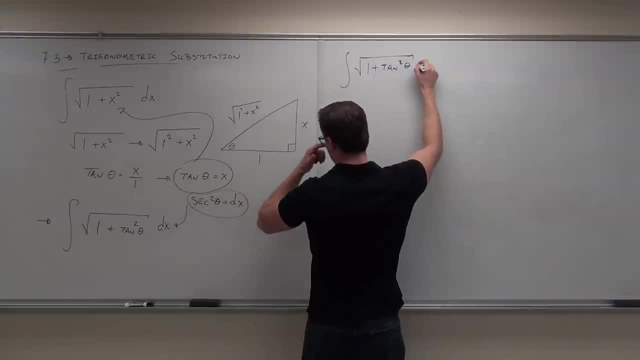 What's else? Secant squared theta. Secant squared theta. what, That's nice, This part, that is my dx. So instead of dx I've got secant squared theta. Oh, you know what? I forgot my theta. 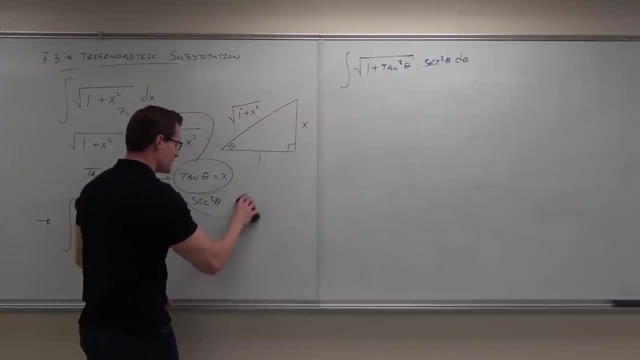 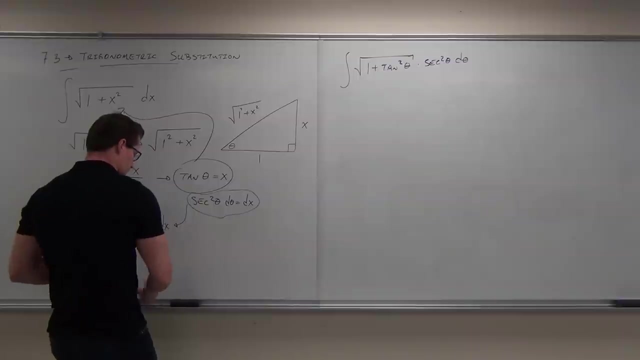 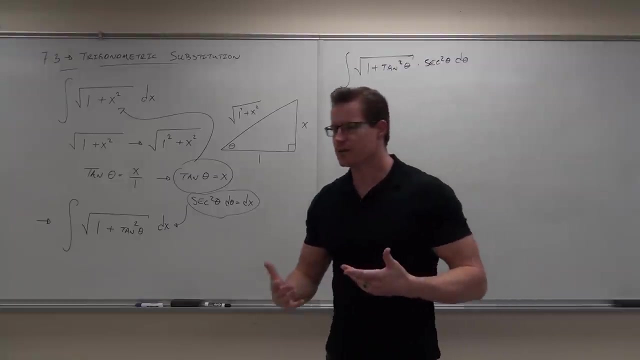 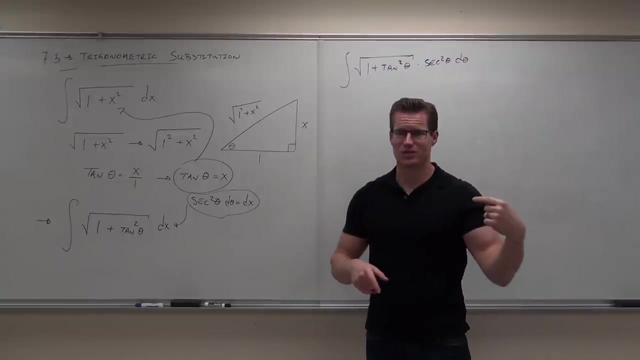 Why didn't you guys catch me on that? We were sleeping, My goodness, Do y'all feel okay with that one so far? Look what it does. As soon as you do this, that changes into from 7.3 to 7.2, just what we did. 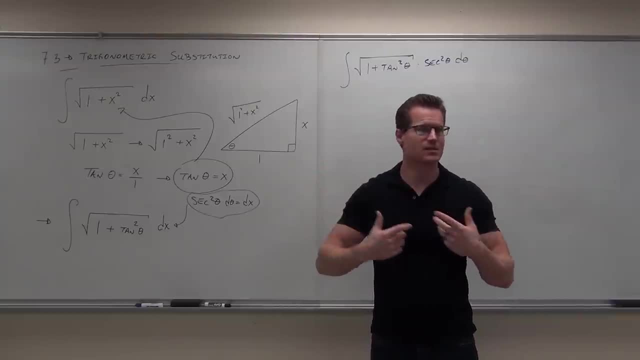 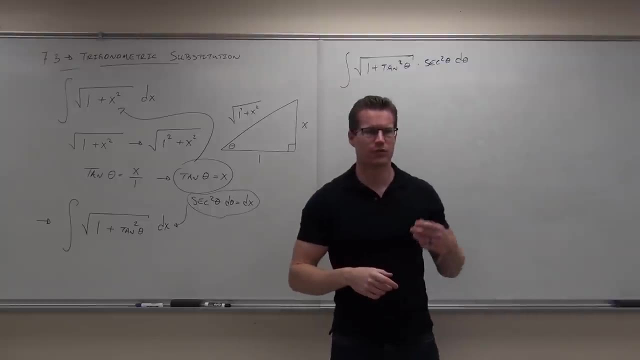 You just did stuff like this, didn't you? In fact, this is even nicer because it already has an identity built right into it. It's already going to match up. That's what we've got. We pick one of three trigonometric substitutions. 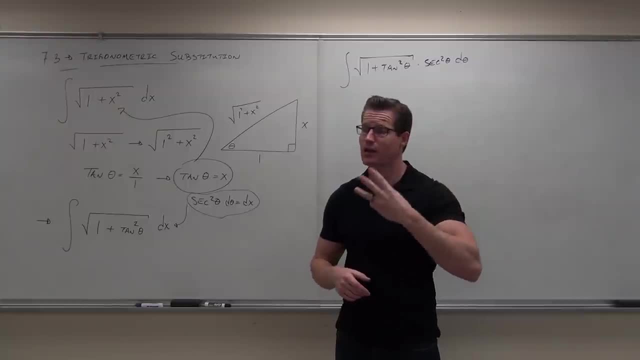 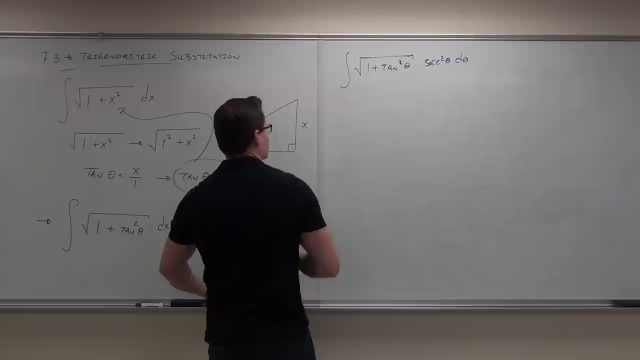 We pick tangent, we pick secant and we pick sine. If you've got those three, the identity's already there. It's really, really nice. You guys ready to do this thing? So tell me, what is 1 plus tan squared theta? 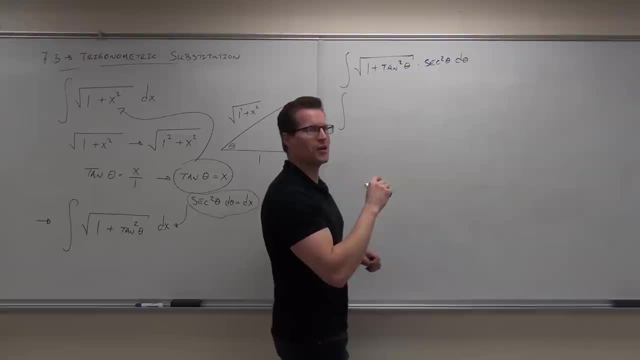 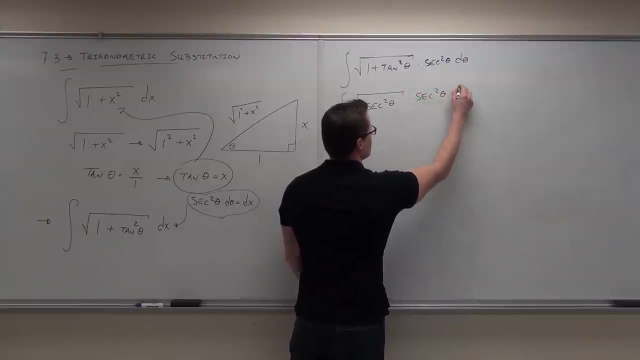 Secant squared theta. Okay, we do need to know that one. all right, Do we have a square root? still, Yeah, 1 plus tan squared theta is Secant squared. Secant squared theta Times. secant squared theta d theta. 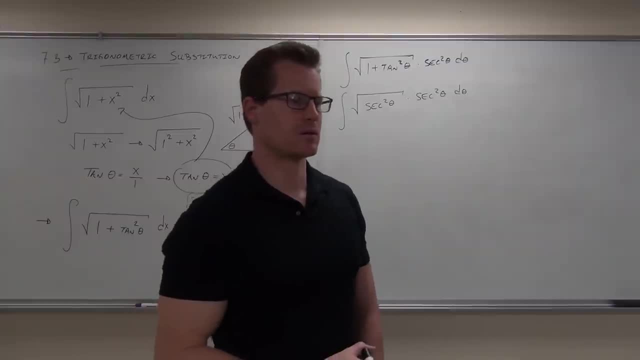 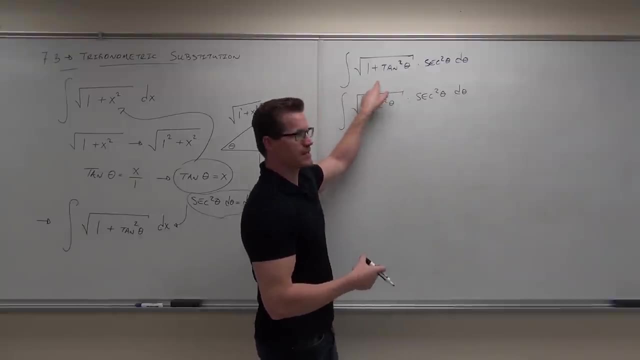 Give me something nice that happens: Square root The. what now? Square root Square. yeah, that's exactly right, This has to happen. So this is nice because we have one of these identities which you are going to have. Look, it's being squared right. 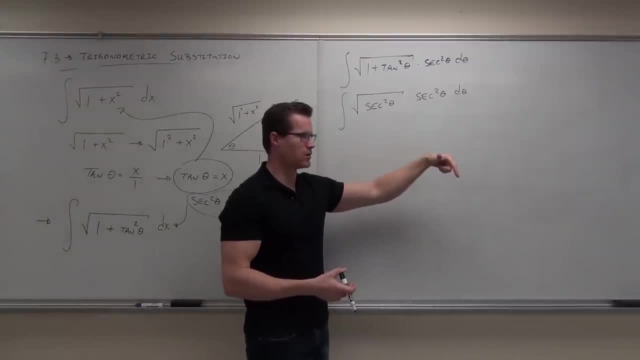 It's squared, So you're going to have a constant plus something squared. You can factor that out, You can make it work so that with identity, your square root gets rid of your square. That's fantastic, We love that. So this becomes secant theta times, secant squared theta d theta. 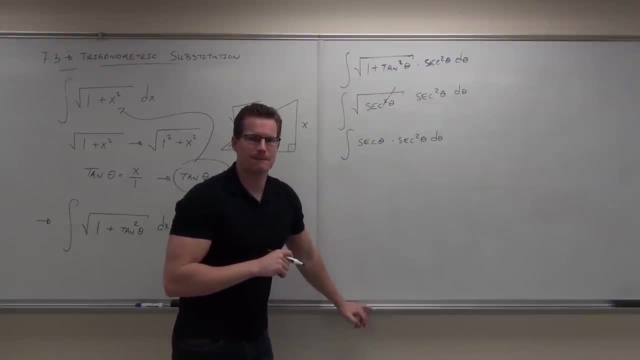 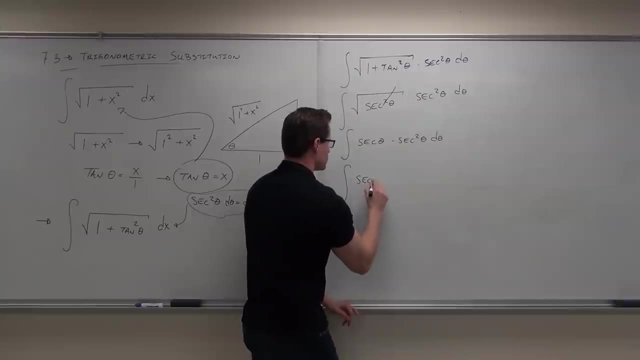 What are you going to do now? Share the Probably, combine them. Oh goodness, We've actually seen this one before in class. Do you remember We did? This was the? This was a horrible Actually. no, no, it was secant to the fifth. 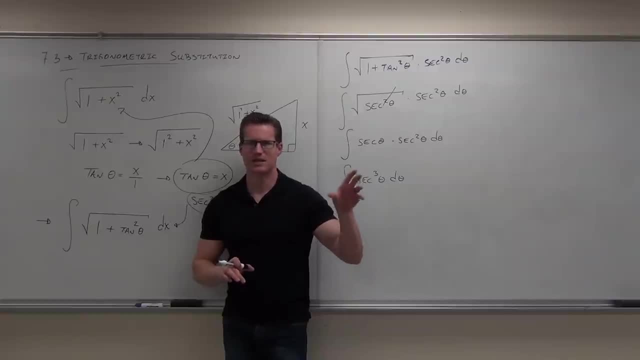 That was really horrible. Do you remember doing that one? We split it off, We used an identity, We did a whole bunch of stuff with it. We ended up adding the integral back and dividing. Remember that, So I'm not going to do that again. 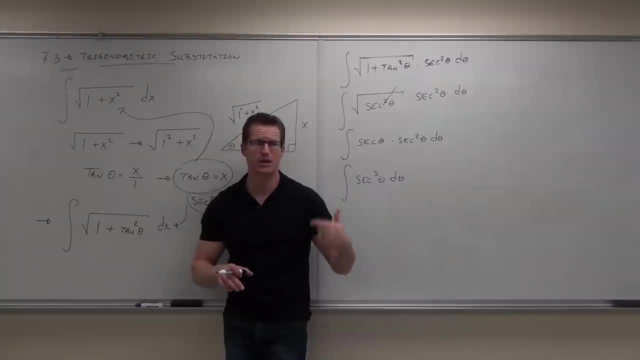 This is already in the video. If you want to refresh your notes or something, it's already back there. I don't remember if it was 7-1 or 7-2.. I think 7-1.. I think it was. integration by parts is what we did. 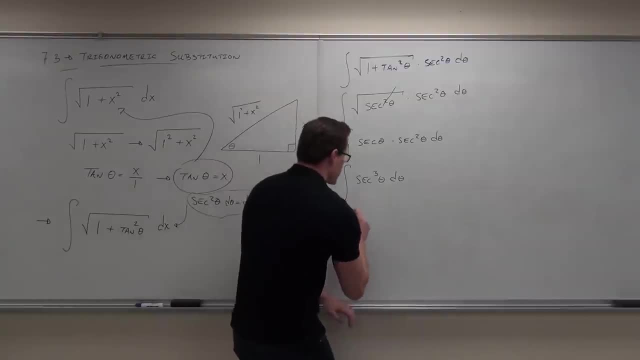 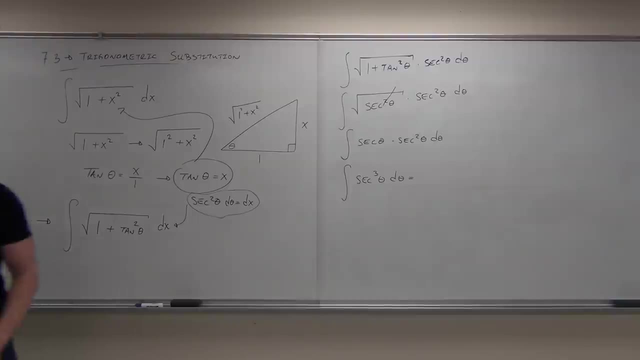 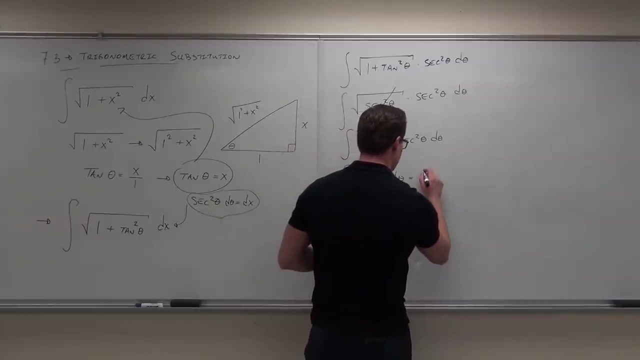 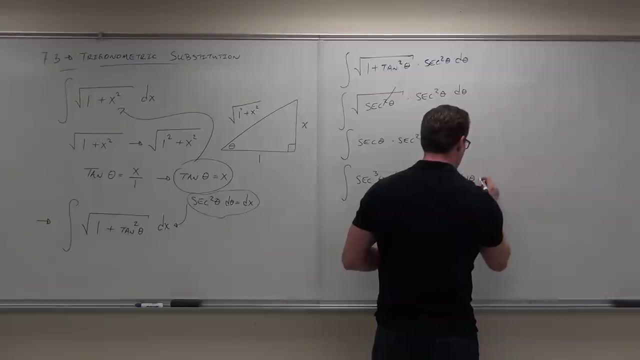 So it's already back there. But anyway, this integral becomes: Was it 1 half? Oh yeah, That's where I couldn't find it. Yeah, 1 half. 1 half secant theta, tangent theta plus 1 half ln. absolute value. 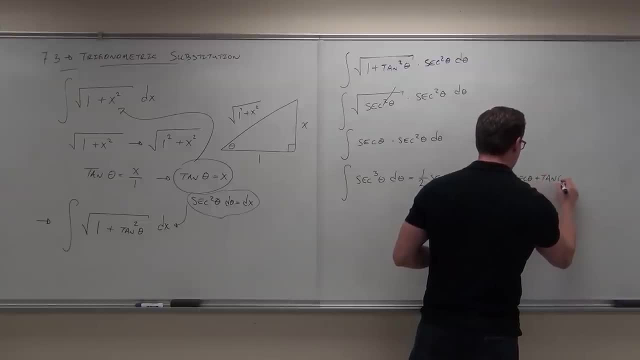 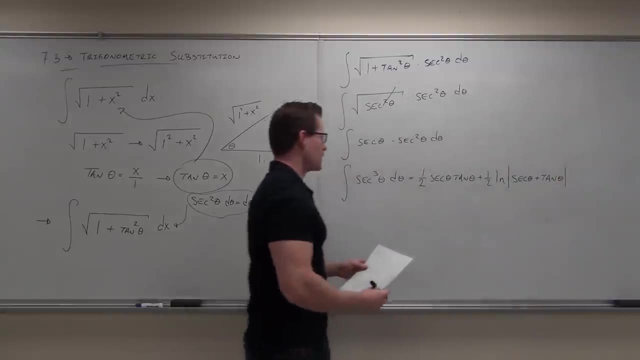 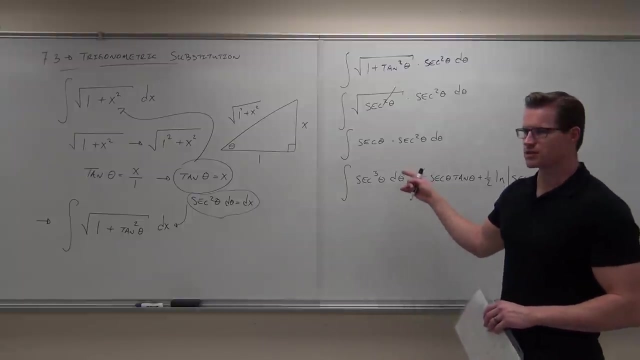 of secant theta plus tangent theta. No reduction formula here, It's integration by parts. if you really want to prove that that is the way it is, You'd split off the secant squared. You take the integral of the secant squared. 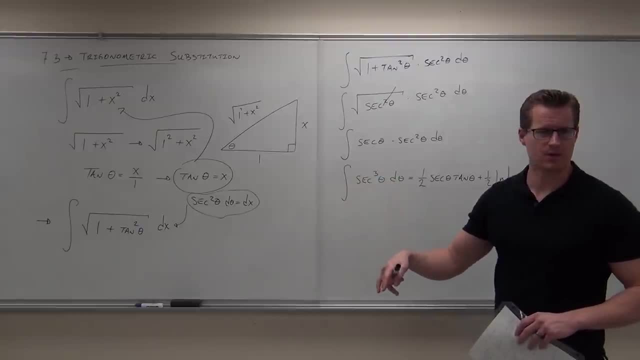 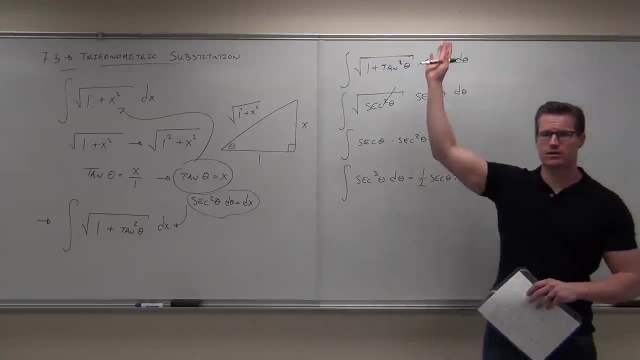 It becomes tangent. And then you do your integration by parts. You guys remember that one. I'm not going to show it, It's already on the video. We've already done this one. Could your hands feel okay up to at least this point. 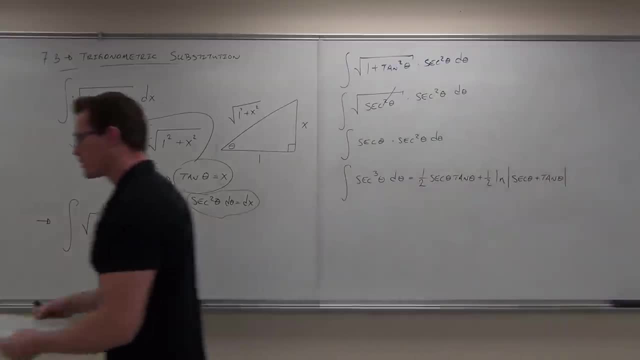 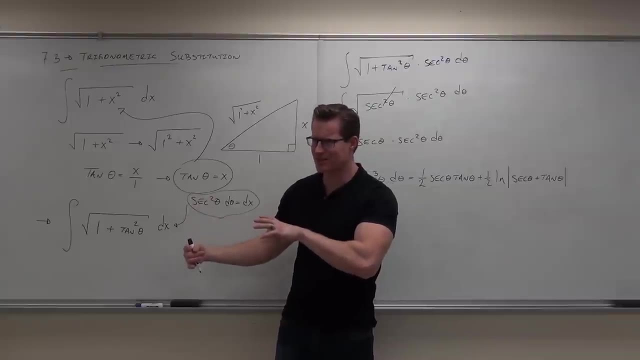 This one we've done before, So I don't want to rehash it. What I do want to say is: okay, let's take a look at my integral. Firstly, I don't know. I think this is really cool. Do you guys see how interesting this actually is, that we can do this? 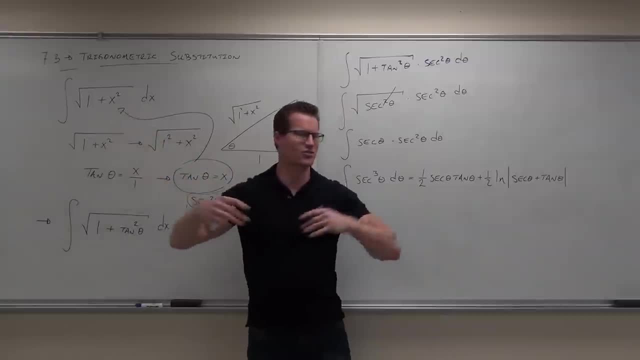 We're using a triangle to do an integral. It's crazy, It's out there, It's kind of fun. Here's the problem. What variable do I start with Theta? What variable do I have now Theta? That's a problem. 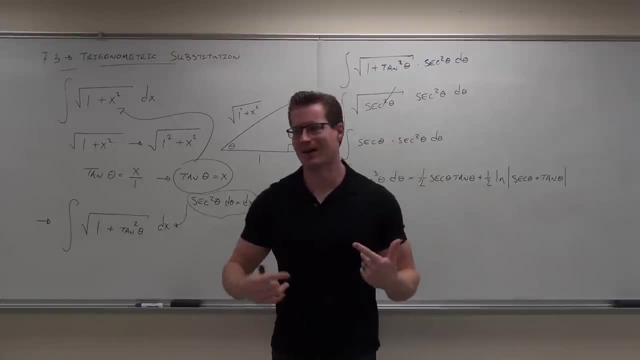 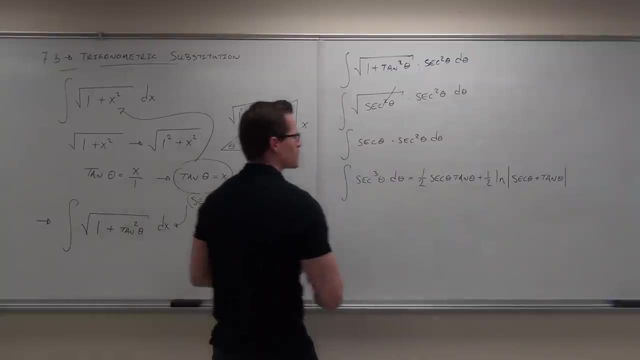 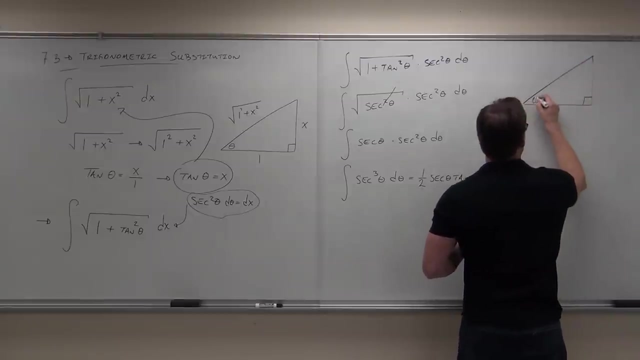 So you're not done right here. Don't just put a plus C and go, I'm done, You're not done. But the rest of this is not that hard. You see, we've got this triangle that we created. Do you remember when you did a U-sub? when you did a U-sub? 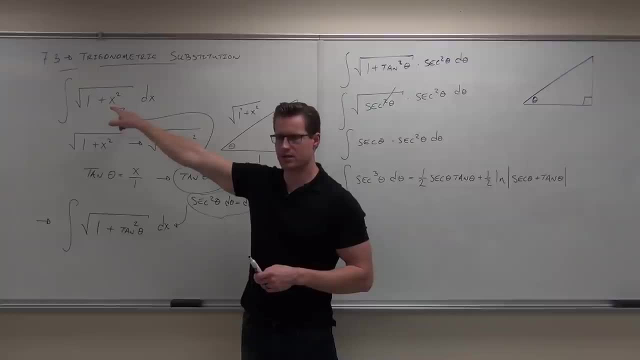 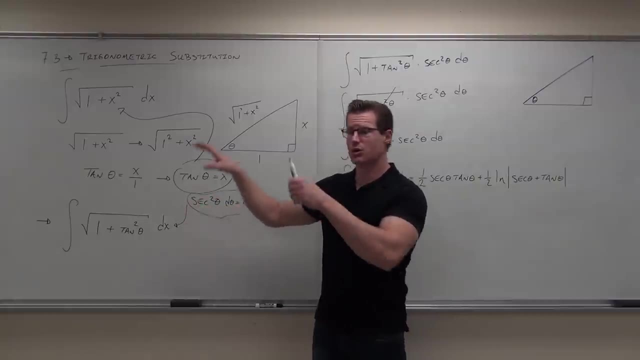 You used the substitution to change a part of your integral correct. Then, when you got done, you substituted back in. Remember that Same thing happens here. We used our triangle to do a substitution. Now we're going to use our triangle again to substitute back. 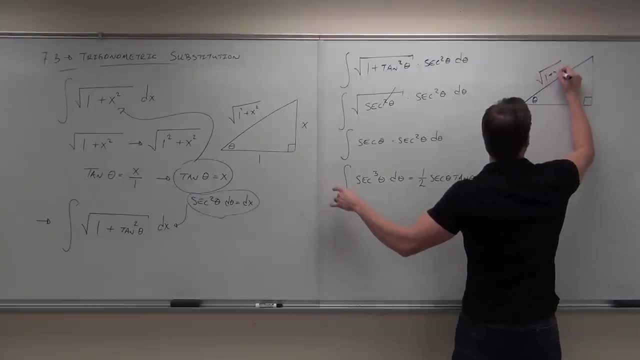 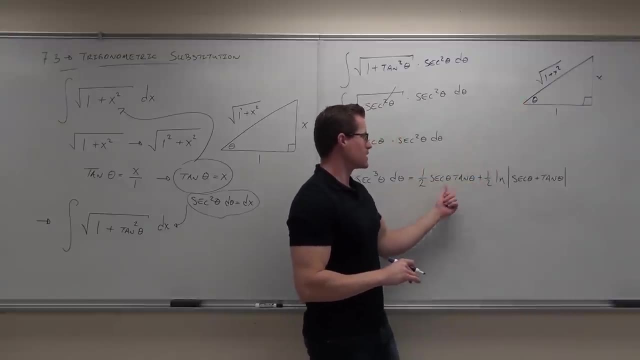 So if our triangle is the square root of 1 plus X squared, and this is X and this is 1, here's what I want to know, That's theta, Here's what I want to know. Can you tell me all of these trigonometric relationships? 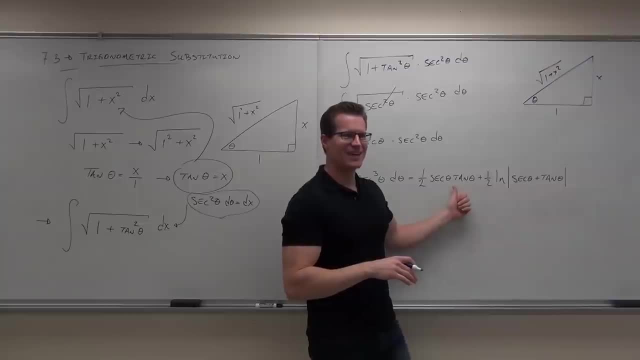 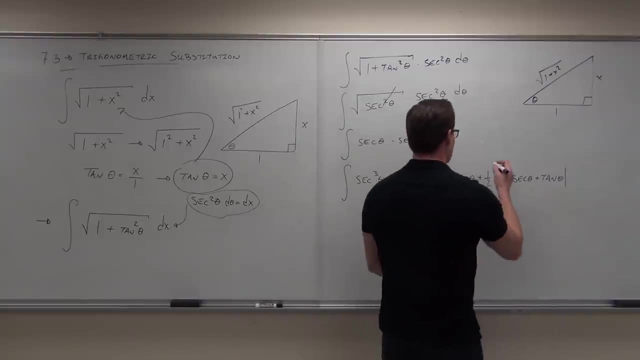 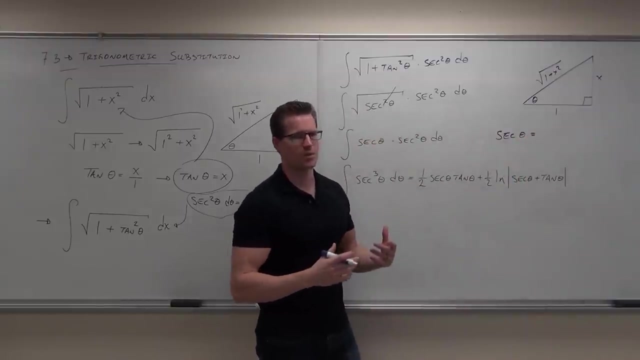 Just put that anywhere, It's fine. Can you use this triangle to tell me all these trigonometric relationships? Yeah, Yeah, So let's list them out. Can you tell me what secant theta is? Now, you've got to be good at this. 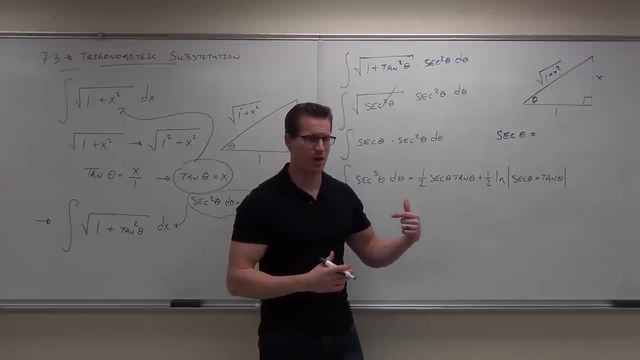 You've got to know that tangent is opposite over J squared And sine is opposite over hypotenuse And cosine is adjacent over hypotenuse And you have to know what cotangent and cosine and cosecant are. So tell me what secant is. 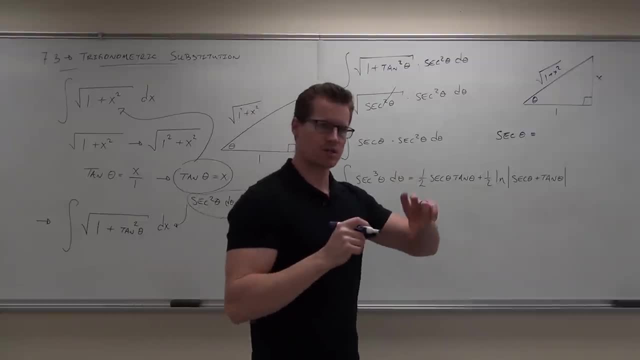 Hypotenuse over adjacent. Very good, Because cosine is adjacent over hypotenuse, Therefore secant, the reciprocal of cosine is reciprocal of this. So what was it again? Hypotenuse over adjacent Hypotenuse. What's a hypotenuse? 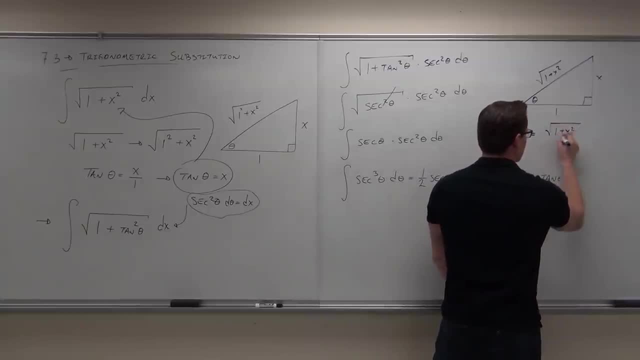 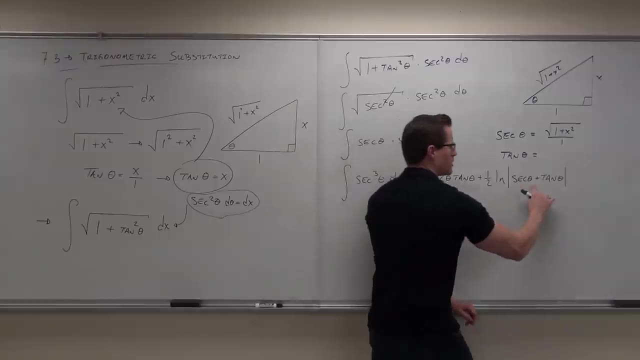 1 plus 4 over 3 plus 6.. 1 plus 4 over 3 plus 6.. 1 plus 4 over 3 plus 6. Over 1.. 1. Let's also do tangent, So we're going to do all of our trigonometric functions right here. 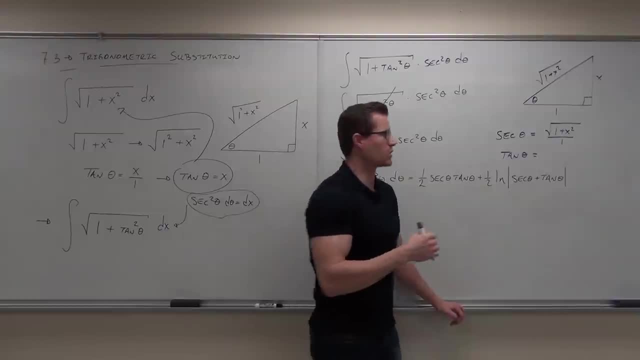 just right by our triangle. Can you do tangent X over 1.. Opposite over adjacent. Brilliant, Just opposite over adjacent. We've got X over 1.. Do your substitution, It's not hard. Tell me what's going to be here for me, please. 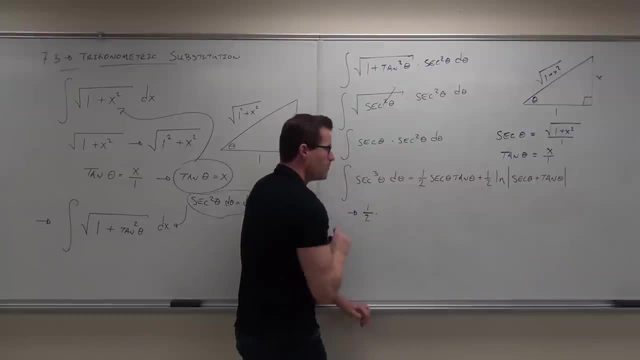 What's going to happen? One half, You've got a one half, Very good. What else Secant, Secant? What's secant? One Okay, Then what are we going to have? X Okay, Plus what changes over here? 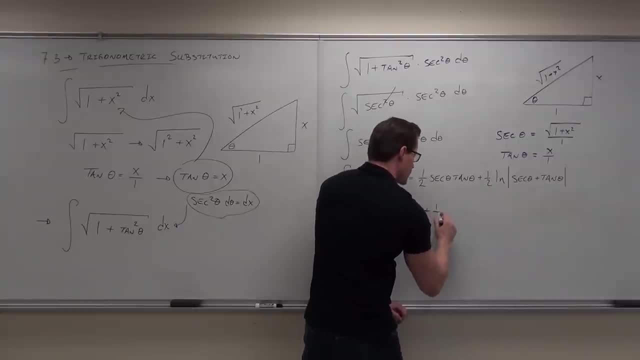 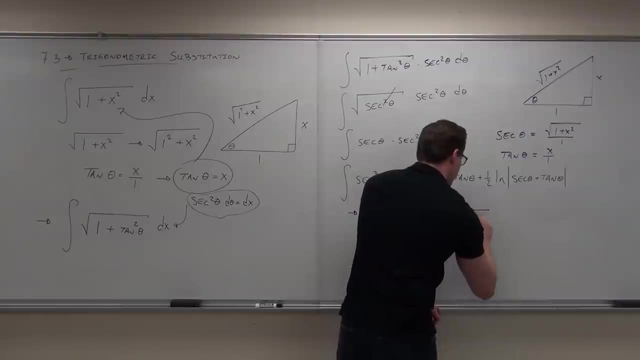 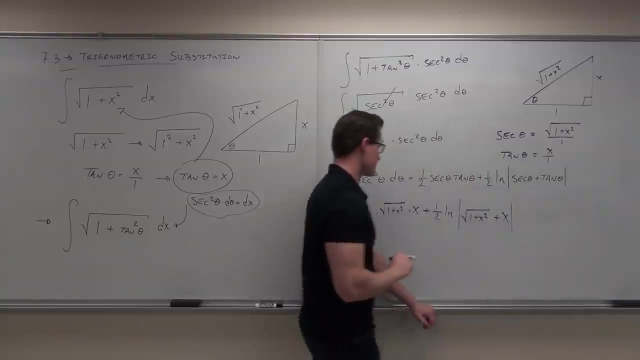 Does the one half change? No. Does the LN change? No? Does the absolute value change? No? What's inside? 1 plus X Times X, Not times X Plus X. Oh, it does, It does. Well, obviously you don't know what your x is. 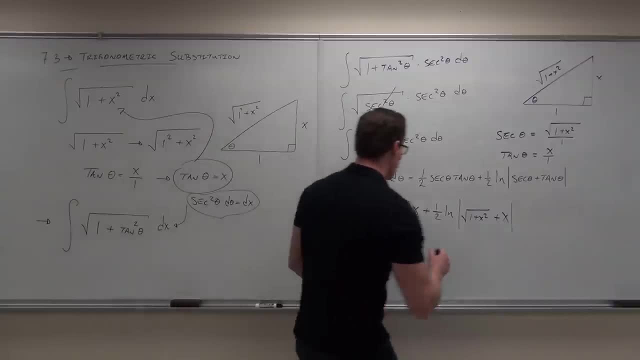 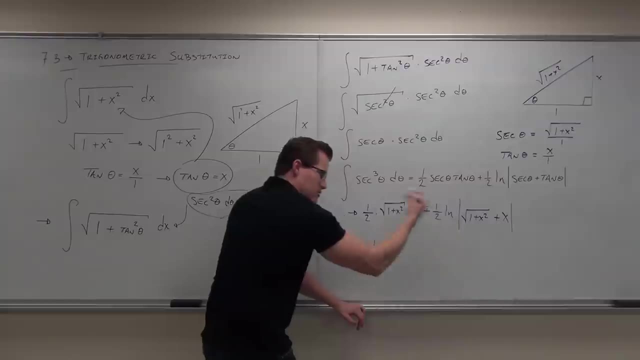 And then Plus c. Nice plus c Probably clean it up a little bit. I would, at least I would do 1 half x. Yeah, I'd do 1 half x. You could factor out a 1 half if you wanted to. 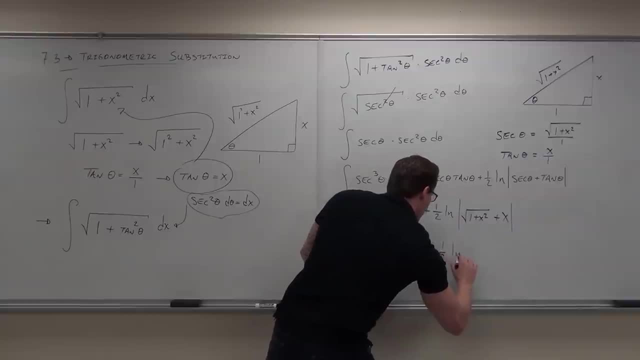 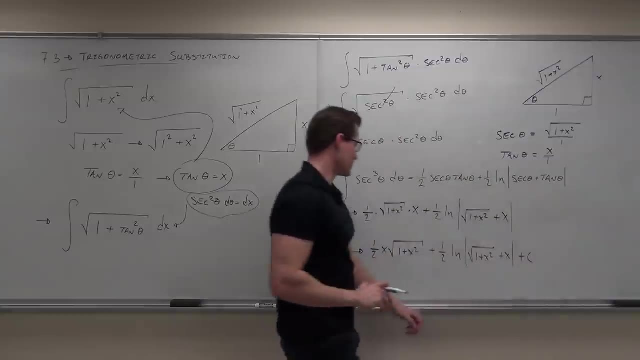 1 plus x squared and then plus 1 half ln absolute value, square root of 1 plus x squared plus x plus c. Oh, my goodness, let's check. Is it in terms of x, like we wanted it? Yes, So the idea kind of OK. it's a crazy idea. 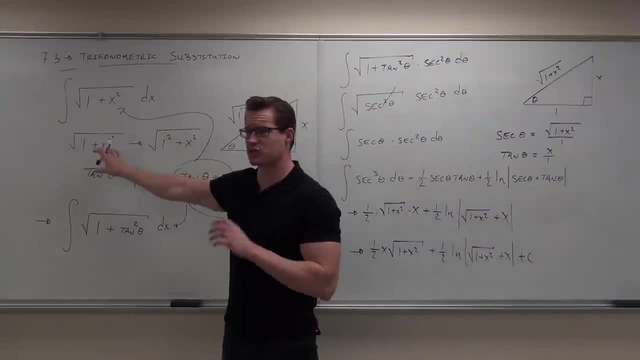 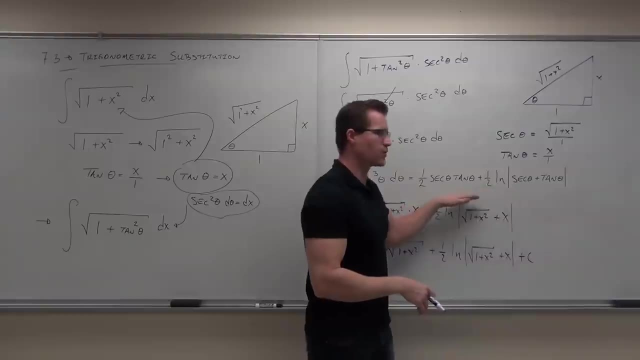 It's a cool idea. It's use a triangle to make a substitution based on a trigonometric function. Do the integral like you know how to do. It's just a trig integral. You guys should know how to do this stuff And then, at the very end, when you're all done with it, 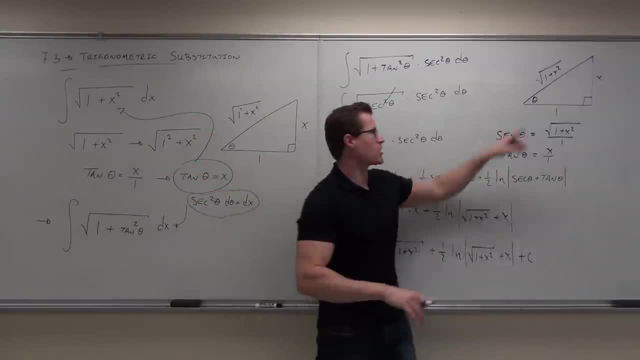 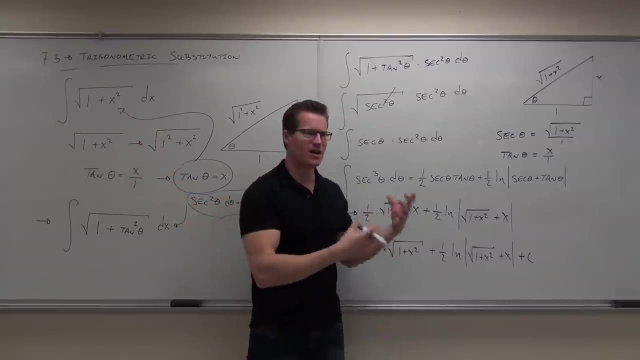 use your triangle again. So triangle to make a substitution, triangle to fix your substitution Show of hands, if that one actually made sense to you. Do you guys get the idea? Did you even know that was possible? Kind of cool, though, right. 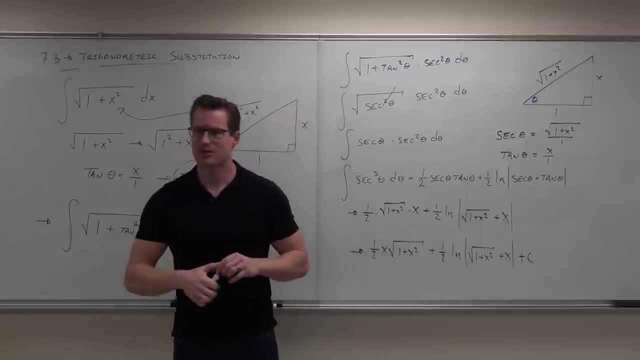 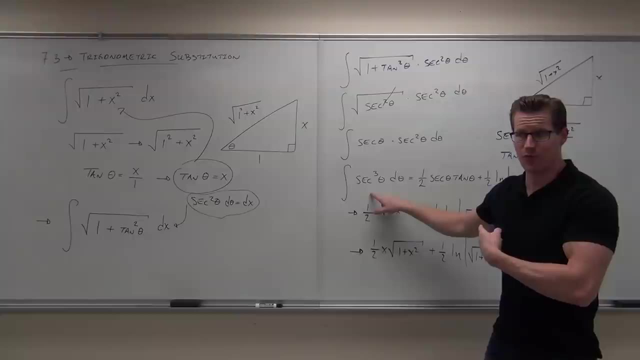 Do you want some more examples? Of course you do. yeah, Of course. Now, this made it look a little bit easier than it might be for you, because I skipped over this. I skipped over the secant cube. We did that one before, which you're fine to use that, OK. 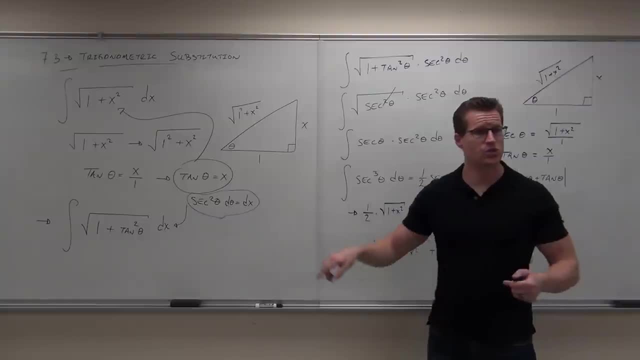 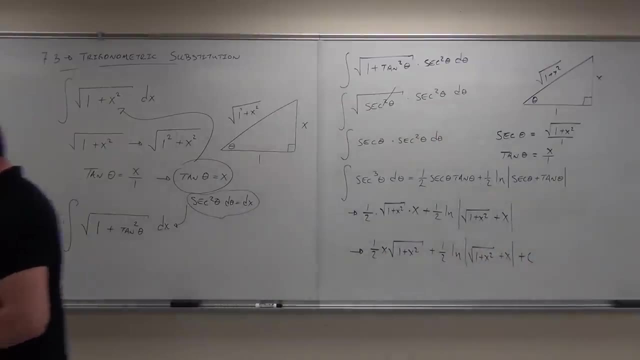 If you've done it before, look at it. OK, we've done that, But you do know how to do that. There's an integration by parts, So some of these are going to take you some time. Do you guys have any questions? 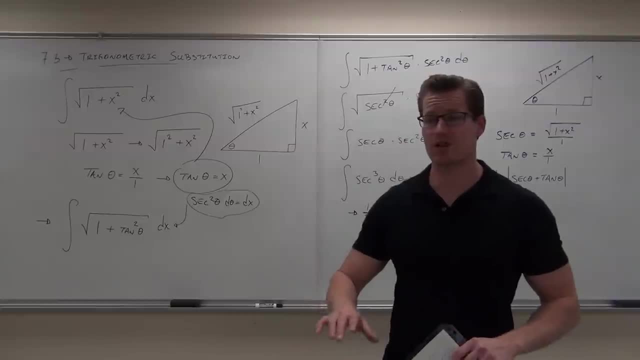 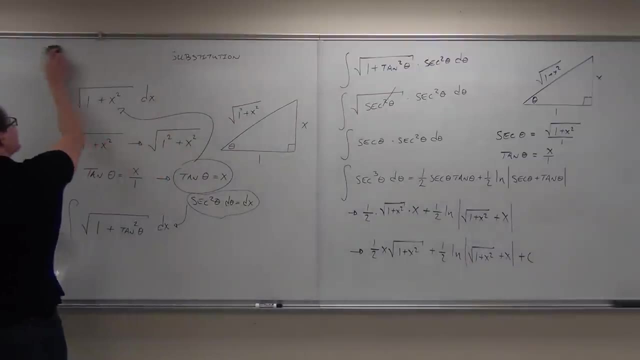 Because these problems take a little bit of board work, So I'm going to have to erase this. Any questions at all? before we Go on, You can ask if you want. All right, OK, So before we go any further, I want: 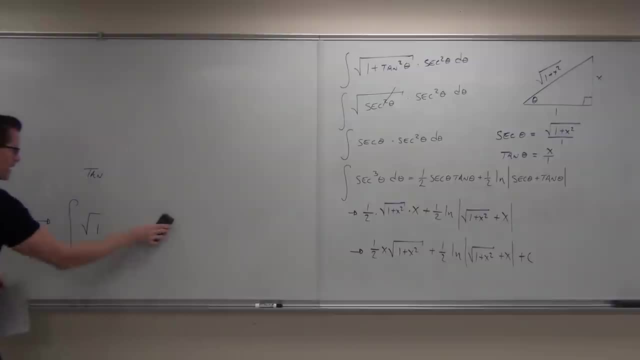 to give you a rundown about when we can use this and why it looks the way that it does. So we can use this when we have one of three situations. I'm going to give you the formulas Again. I don't want you to just blatantly memorize the formulas. 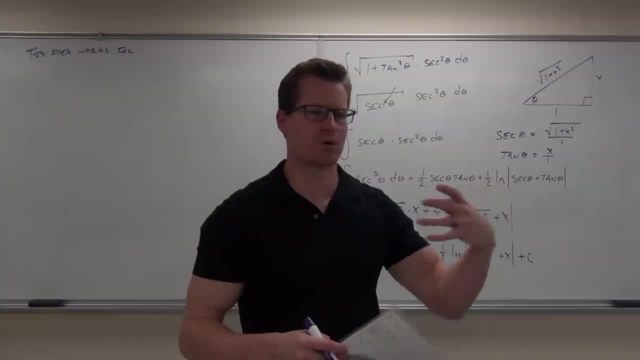 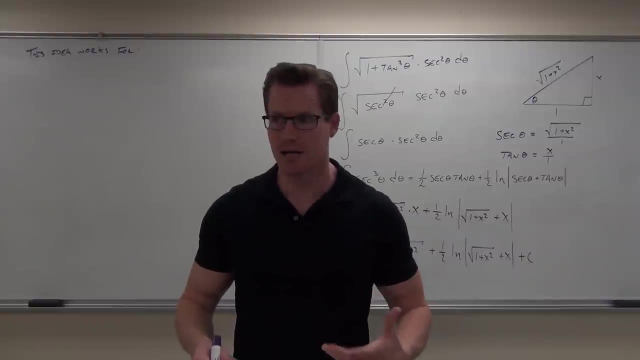 You will, OK, You will memorize them, But I want you to understand why they are the way they are, Because it's really silly to do this stuff just by what's my formula. It doesn't make any sense. I want you to get why it works. 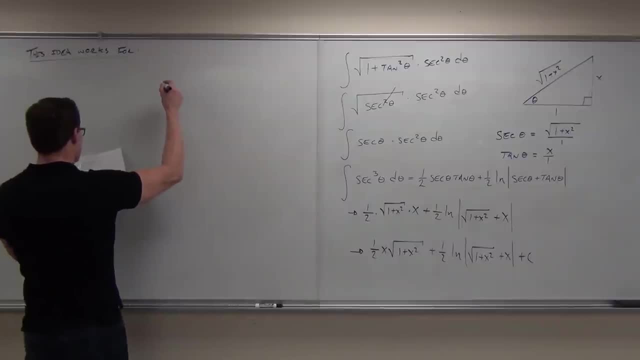 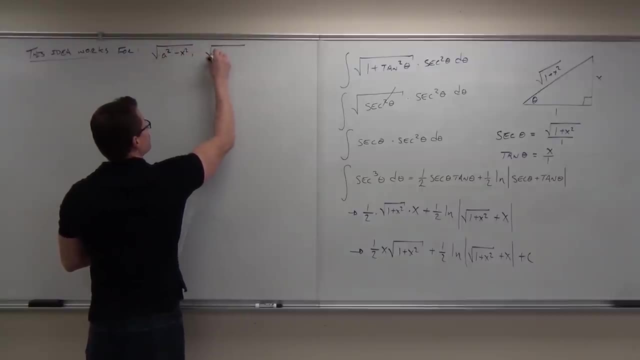 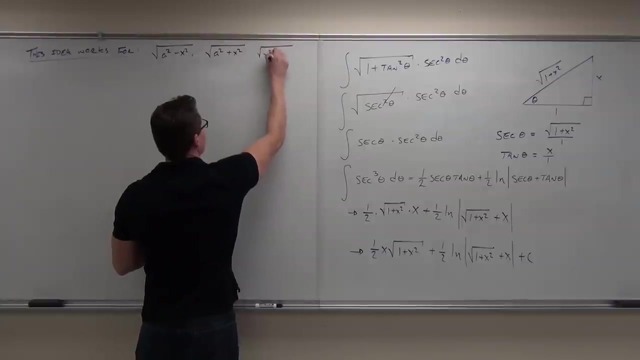 And that's important. So this idea does work if we have one of these three things: If we've got a square root of a squared minus x squared, or a square root of a squared plus x squared, or a square root of x squared minus a squared. 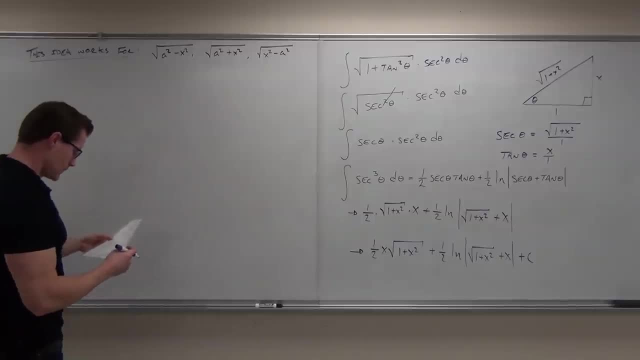 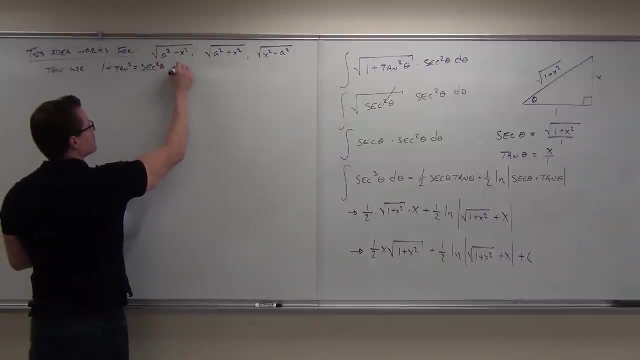 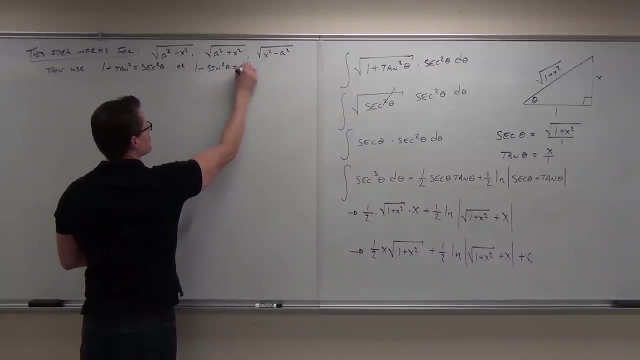 Our first one was of this form. Now, after we do that, we'll be using one of our Pythagorean identities. So then we use Either 1 plus tan squared equals secant squared in one way or another, And or 1 minus sine squared equals cosine squared. 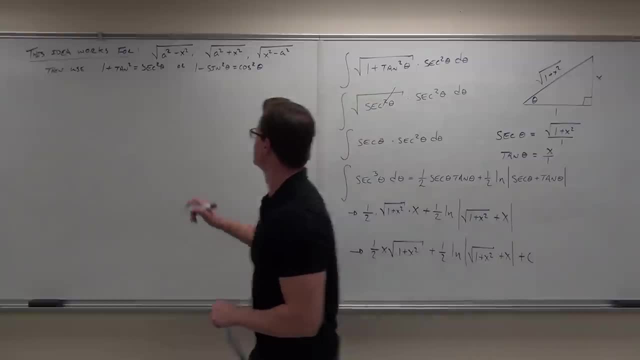 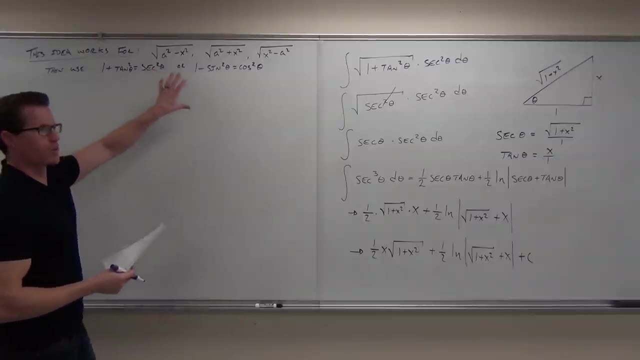 Say what You stand up with. the theta: Oh, darn it, Thank you. So here's the big three. I'm going to look at these in more detail. We're going to understand why they are the way they are, why the formulas actually work. 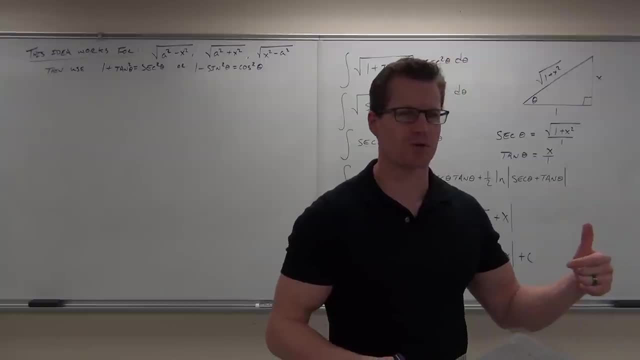 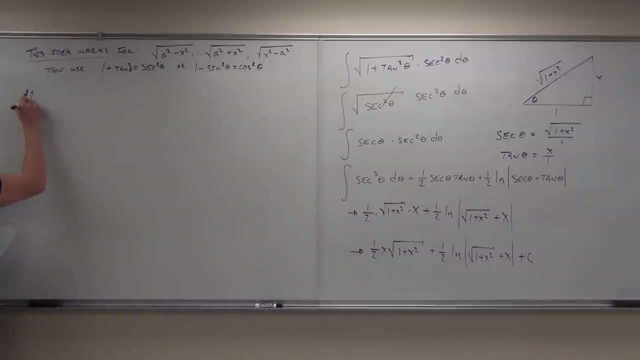 And then every time we go through one of these trig integrals- trigonometric substitutions for integrals- I'm going to rehash the same thing until it kind of sticks with you. So here's number one. Let's look at this. 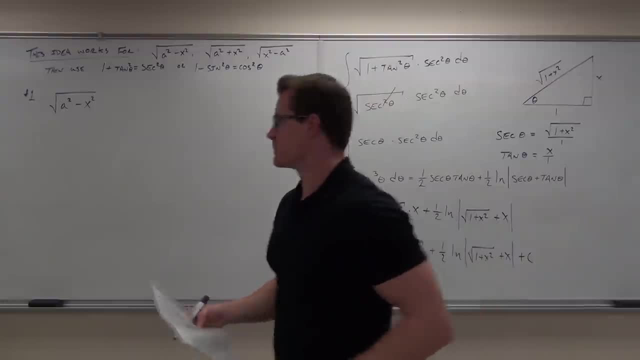 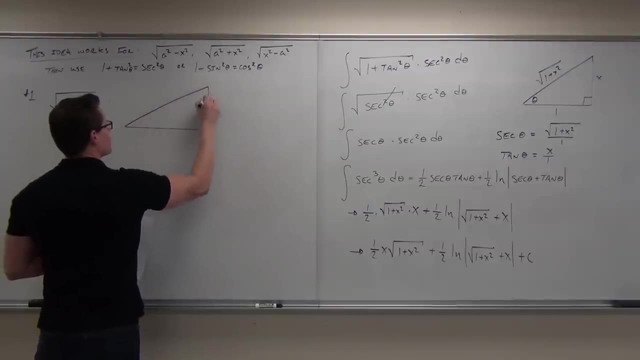 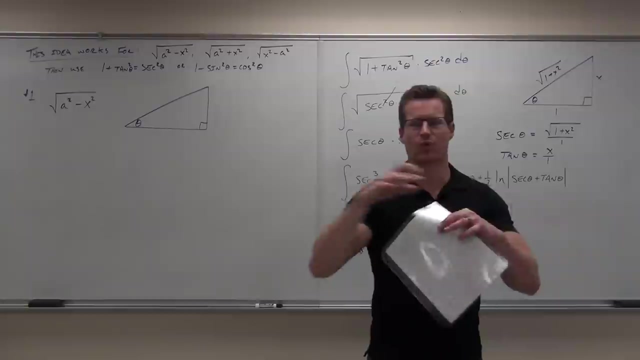 If we were to create a triangle out of this thing? I always draw my triangles in the same orientation. That way I have it fixed in my head. I don't want to get random triangles up here. It's got to be the right triangle, of course. 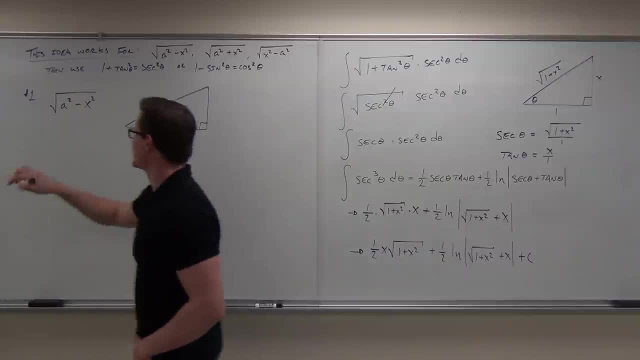 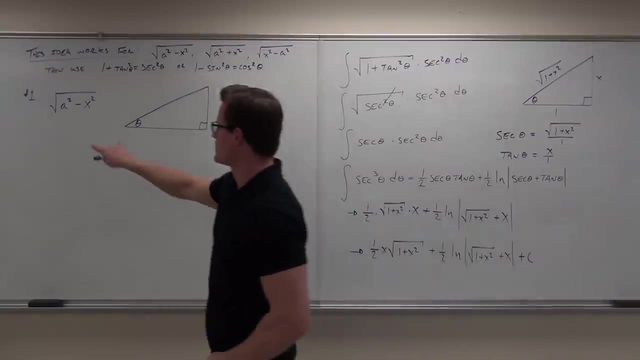 I always draw it this way. Maybe you can do the same thing. I want you to think of what this actually is. It's going to be part of the Pythagorean theorem, But think about the pieces up here. Would this have to be the length of the hypotenuse or the length of the side? 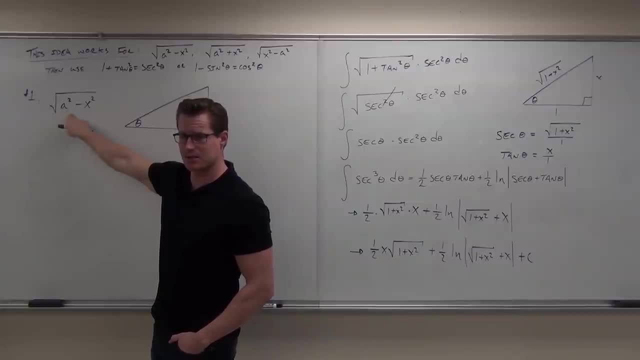 What do you think It's got to be a side because it's got a minus in there. Does that make sense? Pythagorean theorem says the hypotenuse is when you take the sides and add them. A side happens when you take the hypotenuse and subtract. 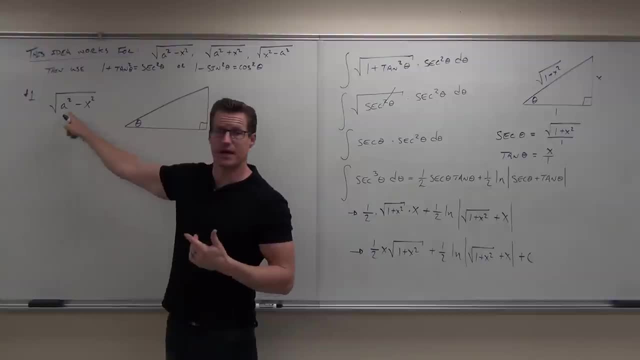 So what we know right now is that this is going to be the length of a side. You guys all understand the idea: It's got to be a side. Now think about which one of these would be the hypotenuse. If this is a side, one of these pieces has to be the hypotenuse. 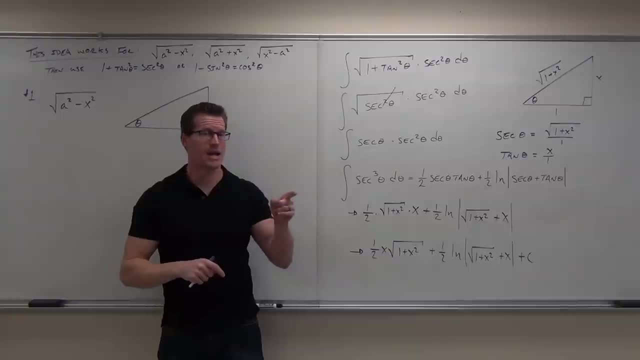 What letter has to be the hypotenuse? A has to be X, can't be, because the hypotenuse is the longest side, correct? So if this is the longest side, if X was the hypotenuse, I'd get a negative inside my square root. 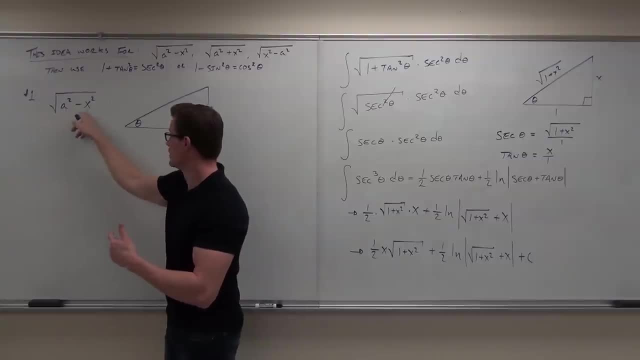 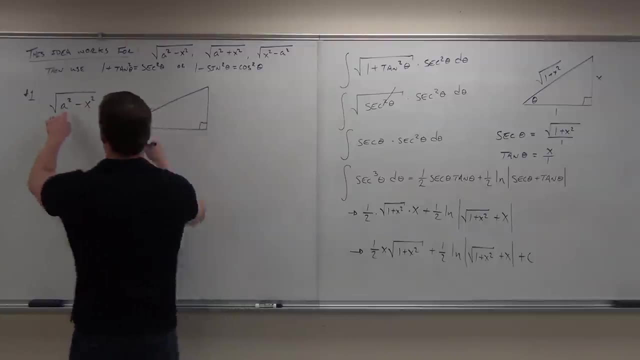 I can't have that. Are you with me? So we look at this and go wait a minute. If this is a side, one of these is the hypotenuse, the bigger one. the first one has to be the hypotenuse. 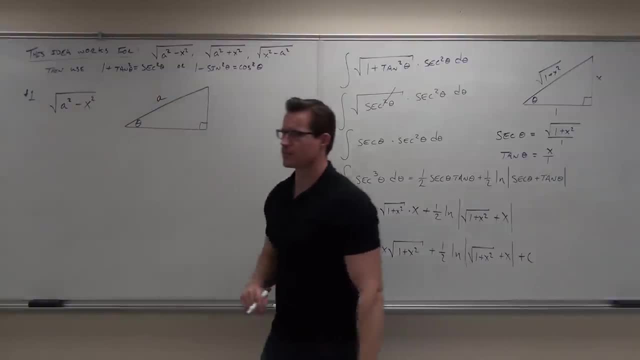 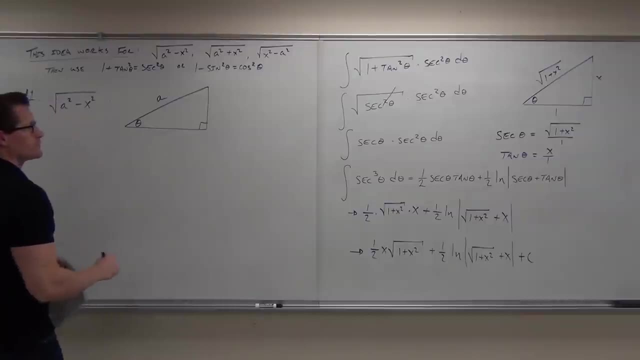 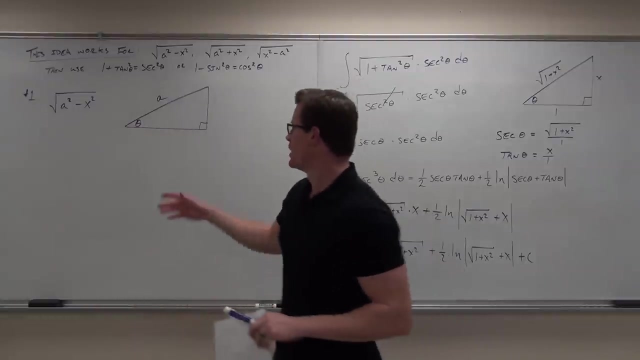 That's got to be A. Now here's your major idea for this whole thing, for this whole lesson. Once you figure this out, it's not hard. I mean, shoot if it's got a plus. that is the hypotenuse. 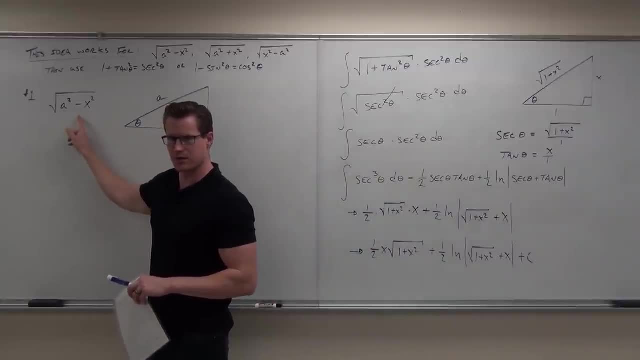 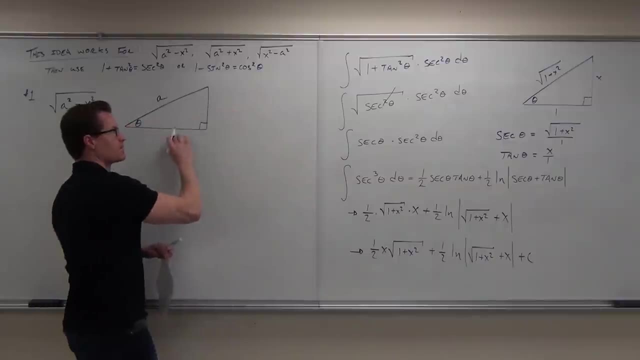 If it's got a minus. one of these is the hypotenuse. Is that clear for you? It's the first one. the bigger one is the hypotenuse. Now, here's your whole goal. Your next goal is: you're going to make these sides in such a way that you get X over A. 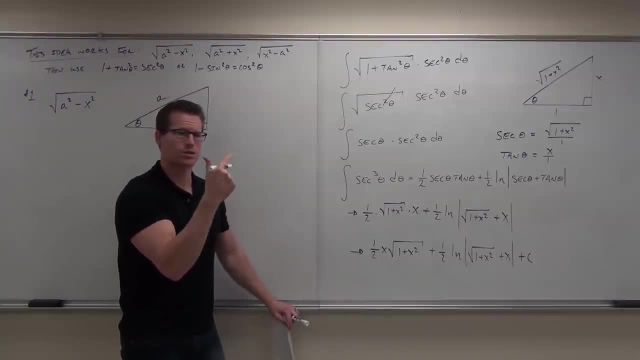 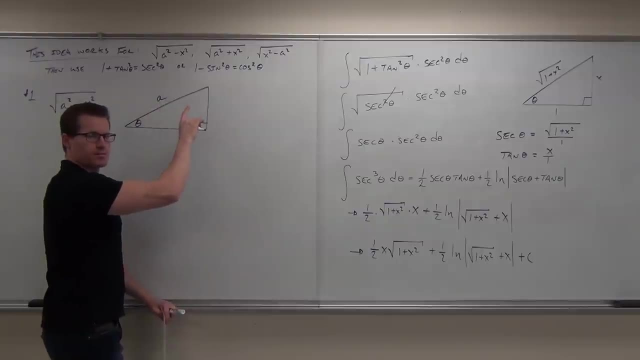 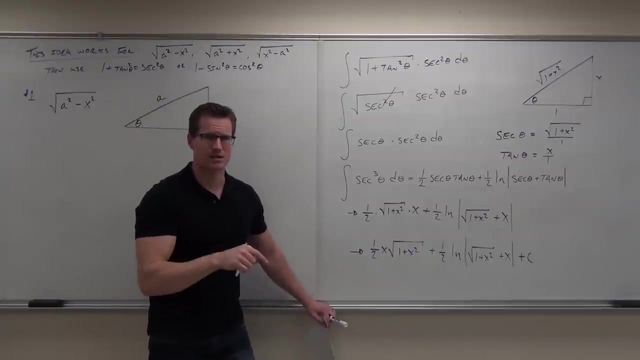 X over A for either tangent or sine or secant. Those are the only three that we're going to use: tangent or sine or secant, So we figure out where the hypotenuse is. Then what we do is we make our sides in a relationship so that tangent or sine or secant gives us X over A. 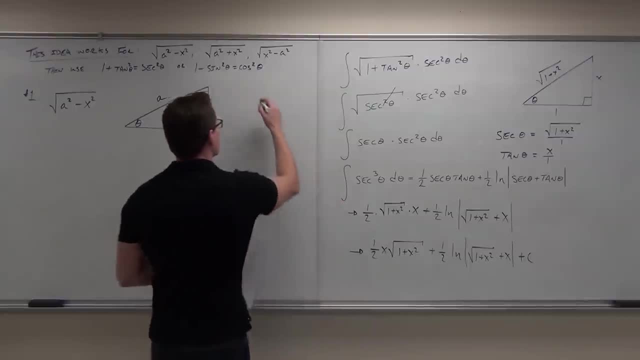 Is that clear for you? I'm going to write that out and make a little note here. So notice that you get to choose right. Either this is going to be X, or this is going to be X, Either this is going to be square. 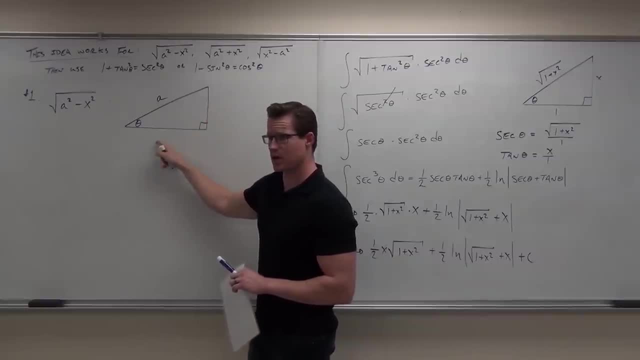 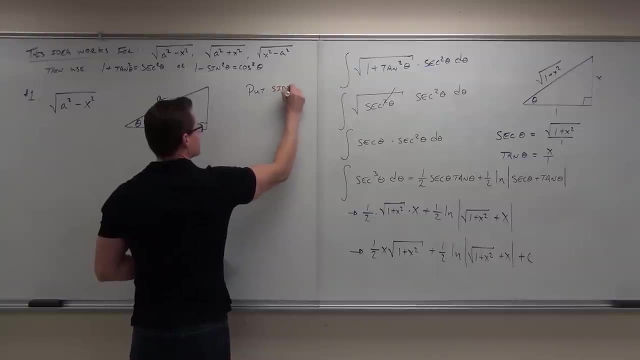 A squared minus X squared or this is going to be the square root of A squared minus X squared. You get to choose, but only one is the correct choice. So put sides in a relationship such that we get X, X over A for tangent or sine or secant. 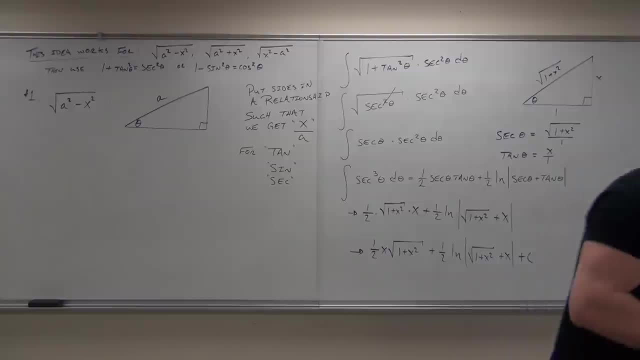 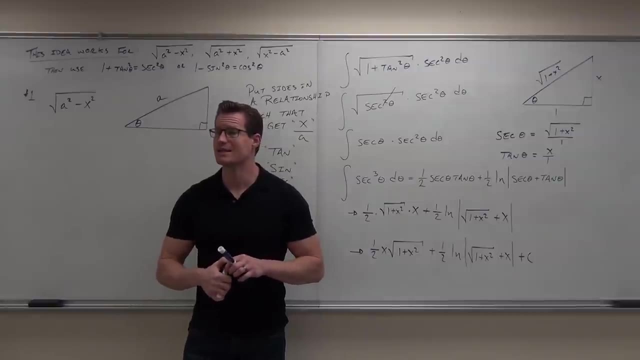 These are the three that we use. We don't use cosine, We don't use cosecant, We don't use cotangent. We use tangent sine or secant, And the reason why we do that is because The identities are really nice for those. 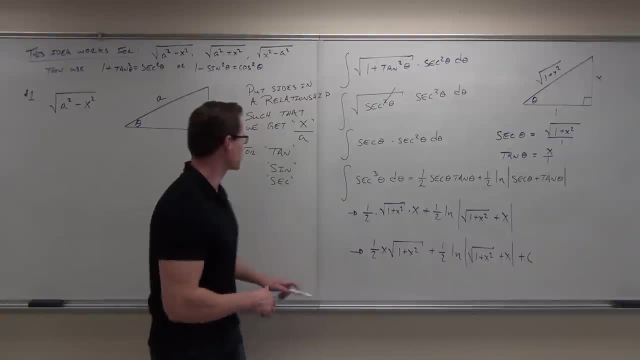 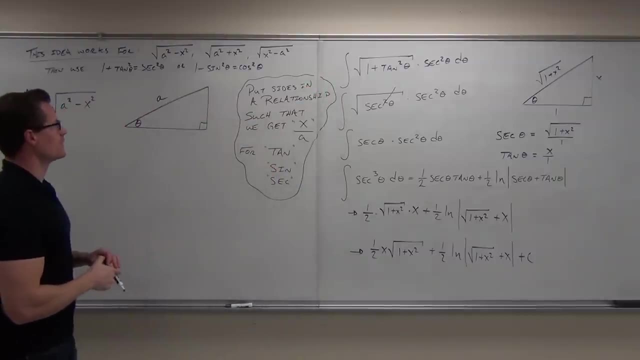 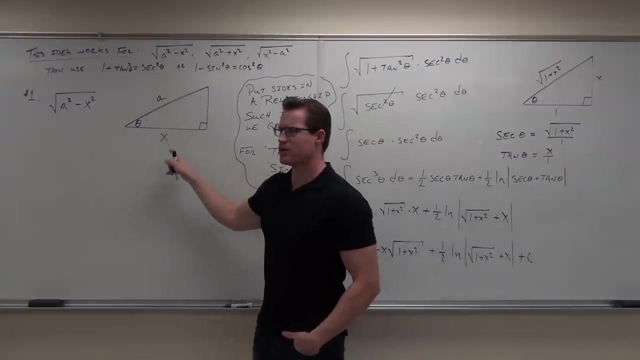 It makes it easy. Are you guys with me on that one? So let's try it. So this is our idea. We want this. Let's give one of them a try. If I do this, If I put X here, The only way I'm getting X over A is if I use. 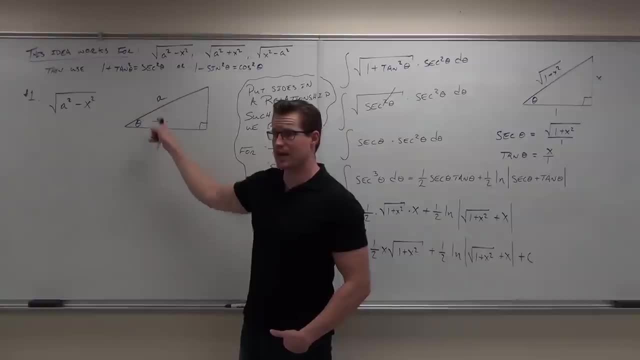 What please? You've got to know your trig Cosine would give me X. is cosine tangent, sine or secant, Then that's a bad choice. So we figure out our hypotenuse first. We have two options. 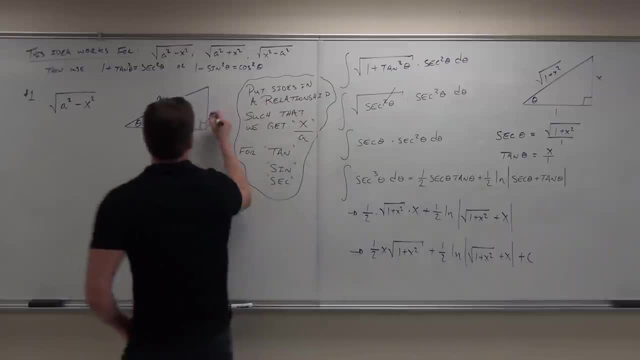 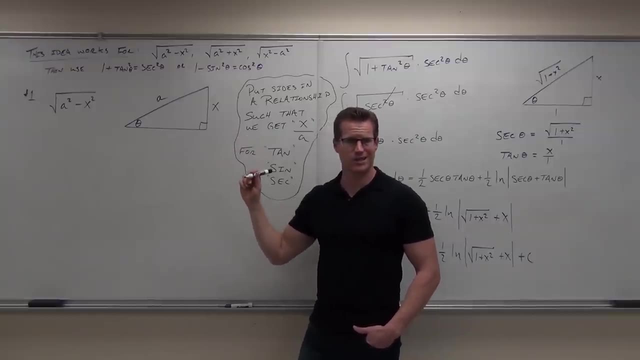 X either goes here or X goes here, Or the side goes here or here. If X goes here, If X goes there, Can I make X over A with either sine or tangent or secant? Which one Sine, Brilliant? Just fill up the rest of the other side with whatever it is. 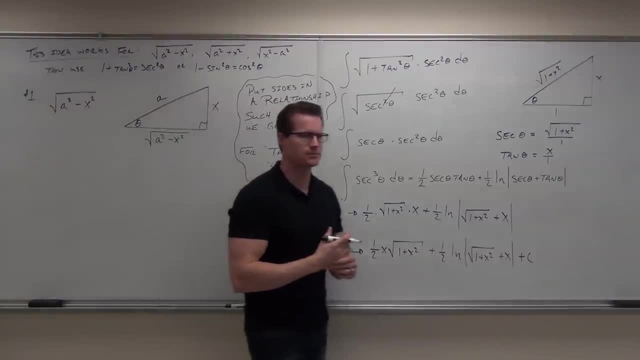 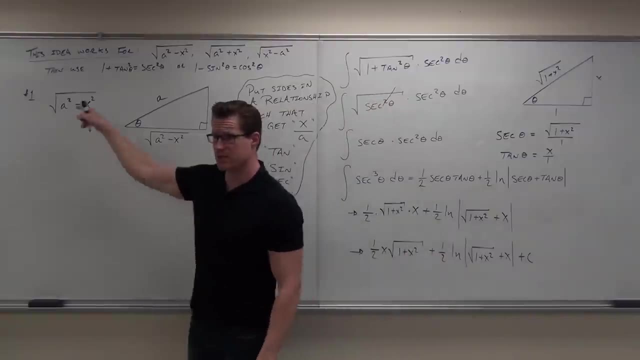 A squared minus X squared. That's the idea. That's the idea. Show of hands. if you understand the idea, You see most classes or most books just tells you: hey, if it looks like this, we're just going to do: sine equals X over A. 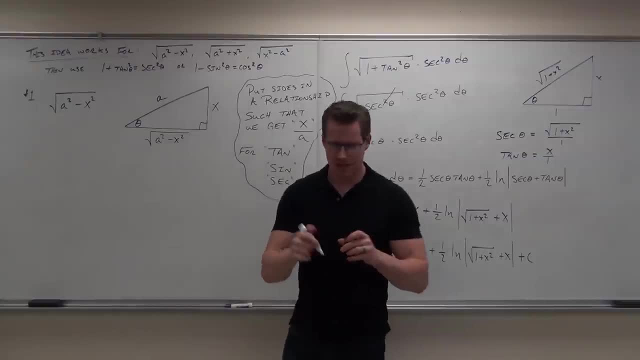 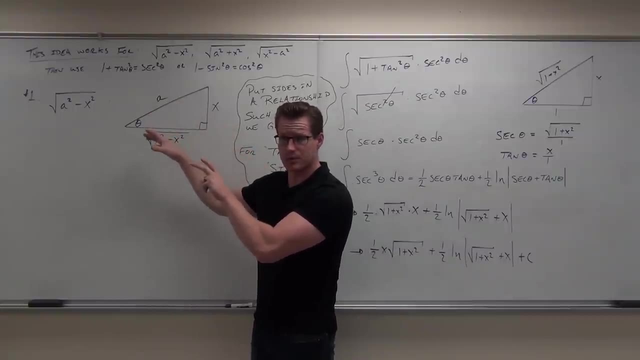 That doesn't tell you why. The reason why we're doing this is because, when you create your triangle, we're going to do it in such a way that this gives us something nicer, Something without a square root. That's what we want. 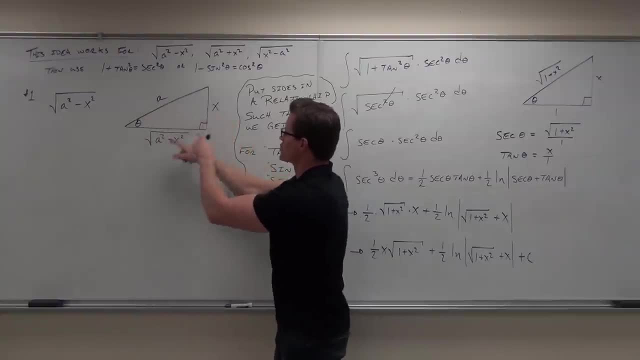 Something easy. So if I've got an A for my hypotenuse, I get my choice of X. I'm going to choose it in such a way that tangent, sine or secant gives me X over A. Then we write that appropriate trigonometric function. 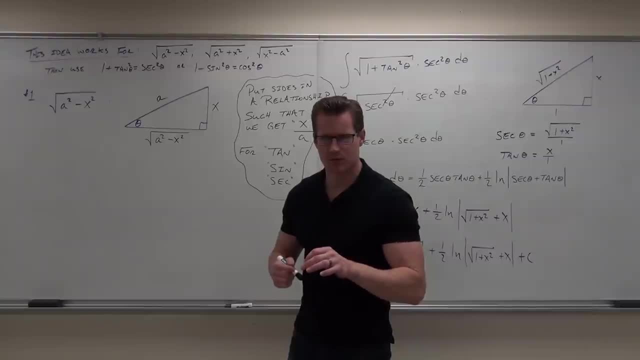 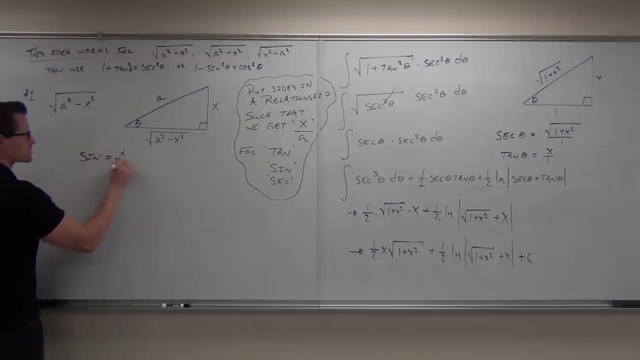 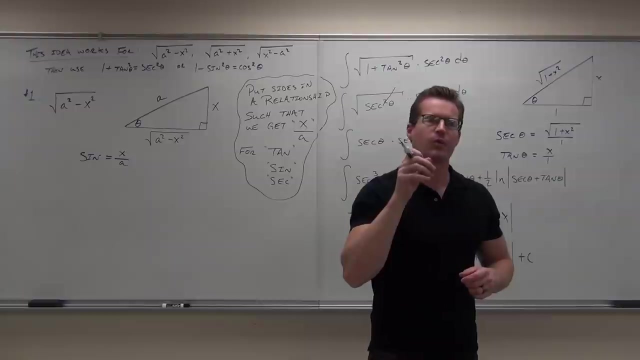 So which one are we going to use? Mine, Are you still with me? Yeah, So we go. OK, cool Then. sine equals X over A, Sine equals X over A, And we always solve for X. We solve for X because that is going to be our substitution here. 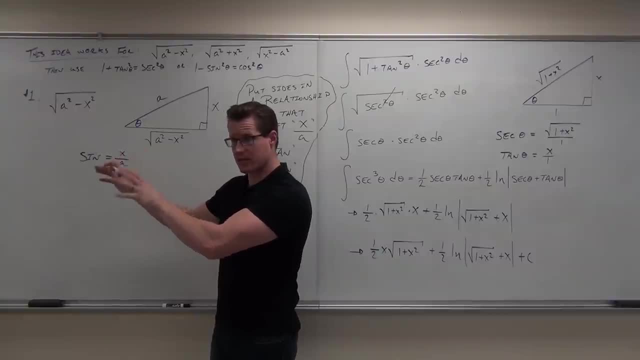 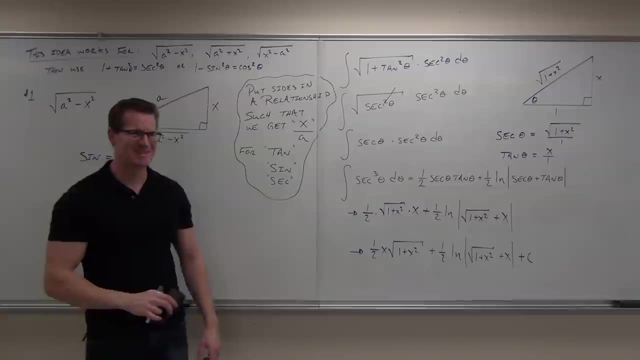 You guys with me. We don't have X over A's. generally We have X's. What do you think, Nathan, I keep forgetting. I'm so excited. I love doing this. I keep forgetting my thetas. I'm so norgy. 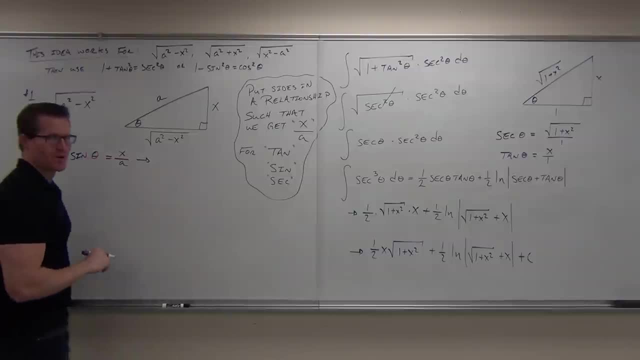 It's not such a good idea to forget your theta. I know It's ironic, right, But since I'm the teacher, ha ha, ha ha- I get to mark you down. It doesn't mean you're right. 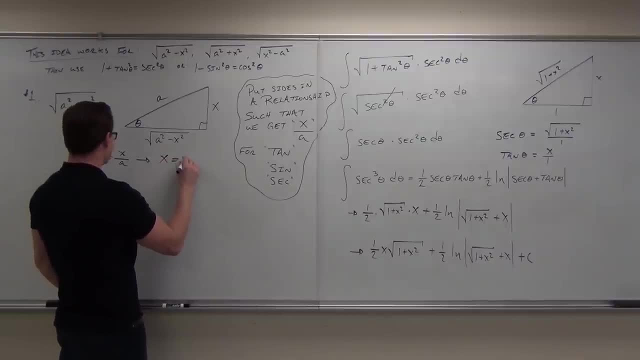 It's true. It doesn't, But that is true. That's what I have you guys here for, right To catch me on all this stuff. So if we solve for X, just multiply by A. this right here becomes your substitution. 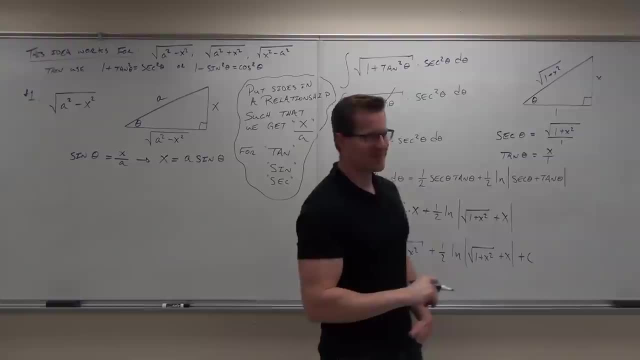 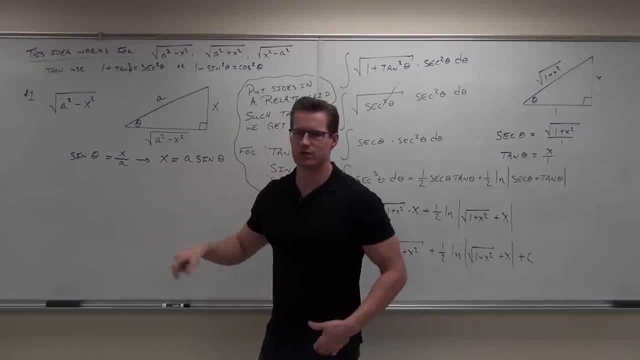 Now, you are going to get very good at this, And what you're going to understand is: you're going to get very good at this, And what you're going to understand is that when you see something like this, all you have to have is: X equals A sine theta. 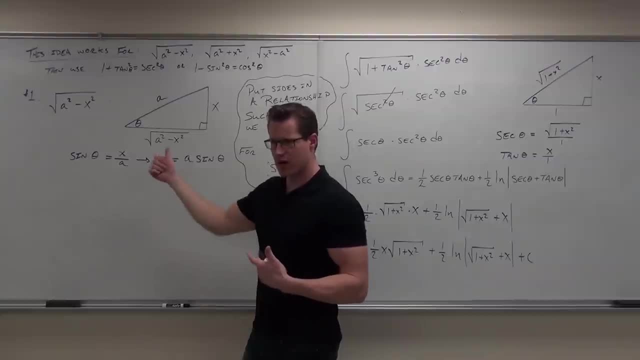 You're going to have to draw your triangle every single time. I still do it for myself, especially because at the very end we're going to have to substitute back in. So you're going to need that triangle, So draw it. Get used to the idea of drawing your triangle. 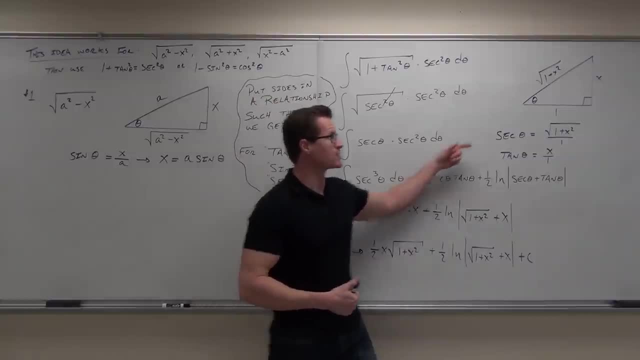 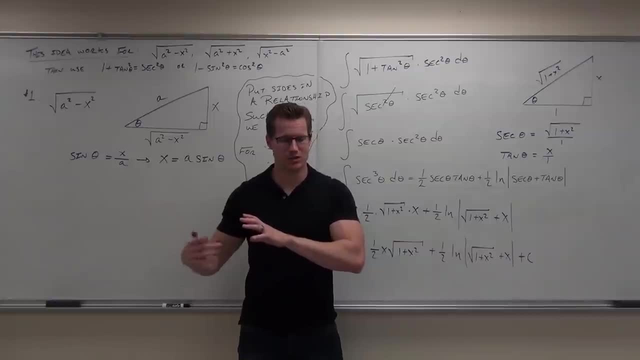 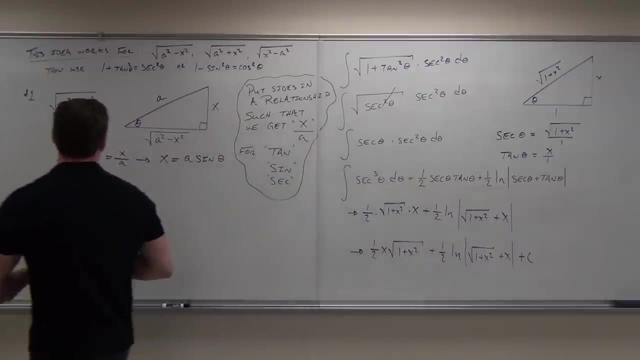 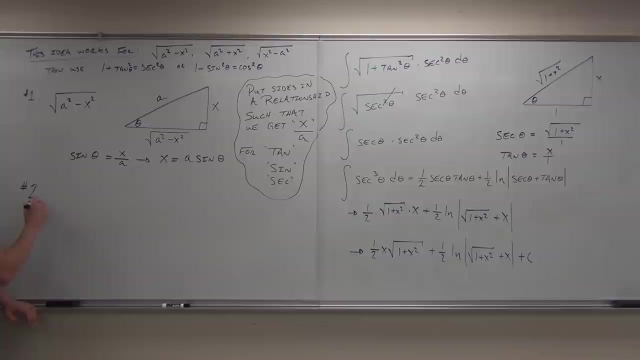 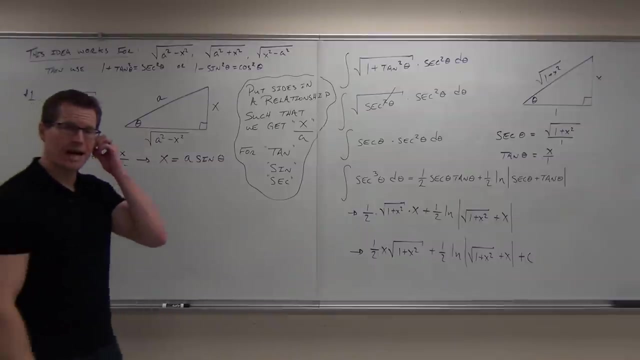 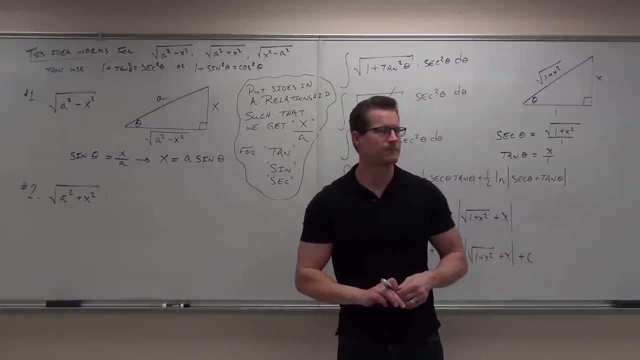 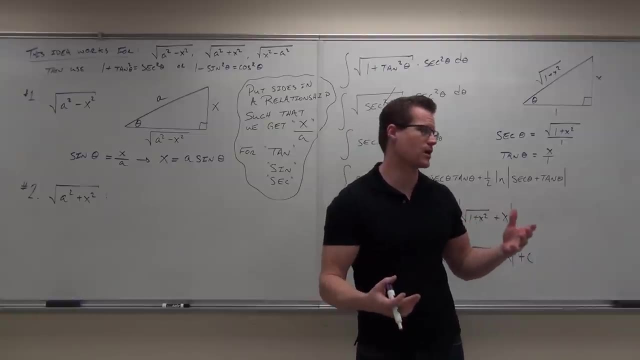 Michael. So we just get the other three functions, because they're just difficult to use in this way. Right, You don't need them, we use the ones that work all the time. Those ones are the tangent, the sine and the secant. 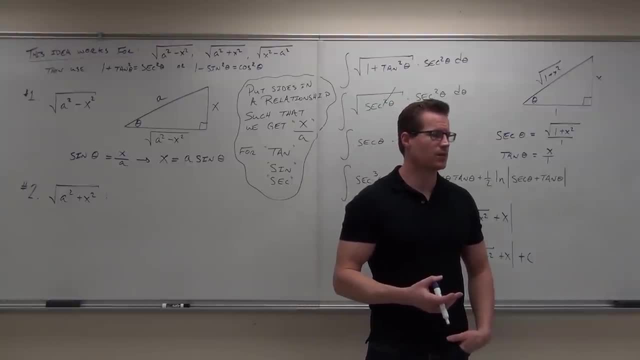 Could you do it with the other ones? Probably, But we don't because these ones work. These are the big three. This one takes care of tangent and cotangent. This one takes care of sine and cosine. This one takes care of cosecant for us. 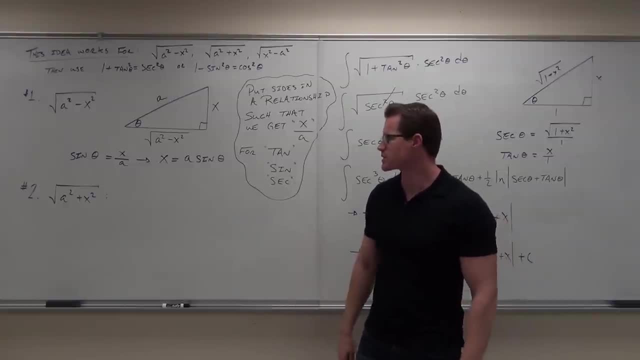 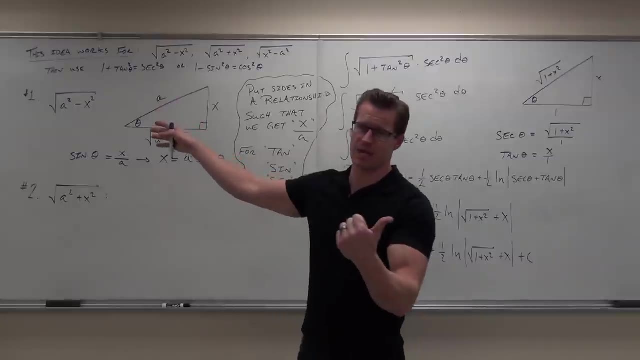 So otherwise we'd have the different identities. These ones work really nice. You guys, ready for the next one? First thing we do every time we see one of these that we can't fit on our table, that we can't do a substitution for, that we can't do a integration by parts for 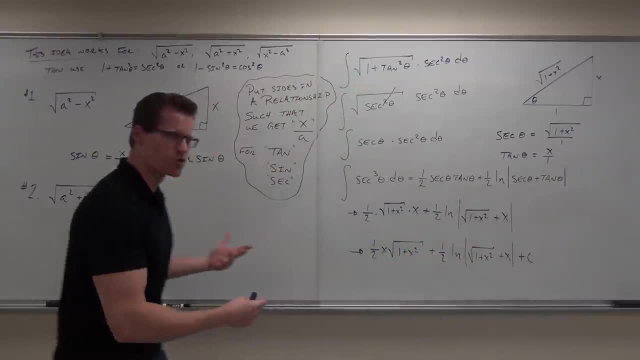 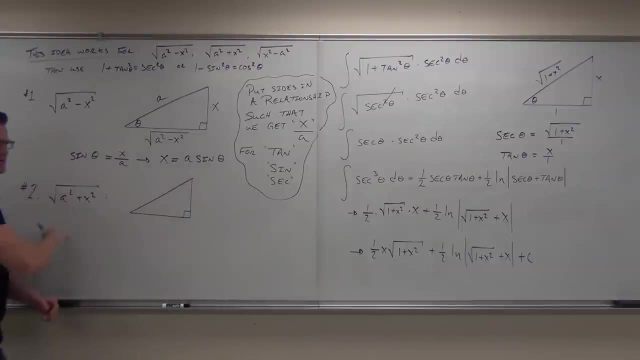 and it's not trigonometric. we do a trig sub. That means you're going to draw a triangle, So we draw our triangle here. You've got to be very good at telling me whether this piece is a hypotenuse or a side. 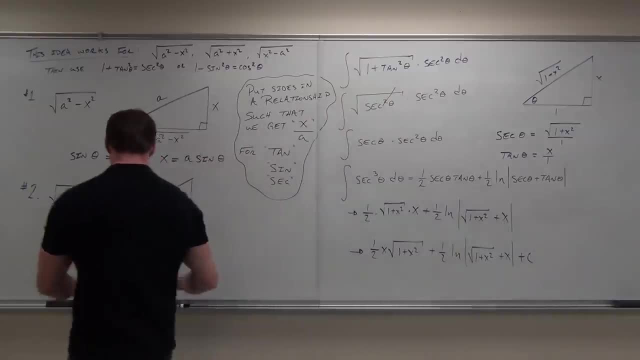 What is that? one Hypotenuse? Very good, So this makes it actually pretty easy. Our hypotenuse is a squared plus x squared. Now We need to put our sides in a relationship We're either going to have. by the way, what are our two sides here? 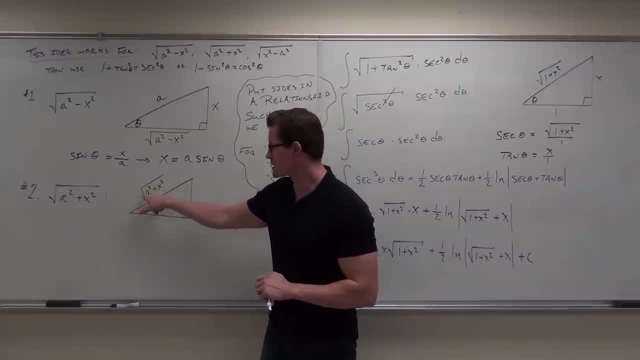 A and a. Good, It's not a squared, It's a. So if this was a nine, you'd be putting a three. Does that make sense? Okay, So we have a and x. Where's the a going to go? 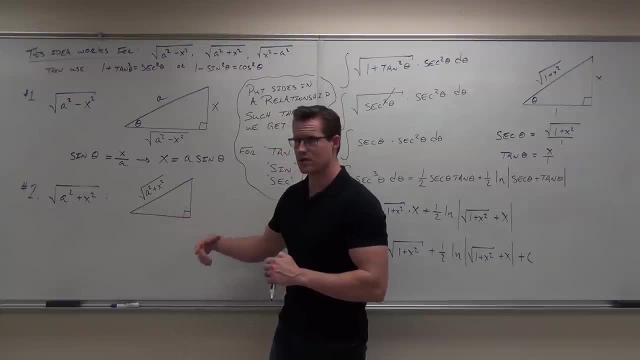 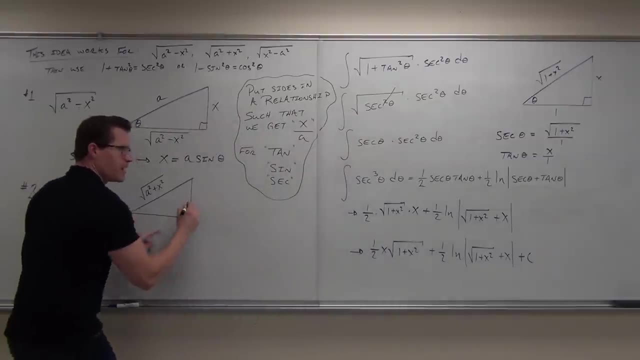 Opposite or adjacent Adjacent. Good, Because I'm trying to make. I'm not trying to make sine or secant here, because those have to deal with the hypotenuse. I want that, I want tangent, I want the relationship. 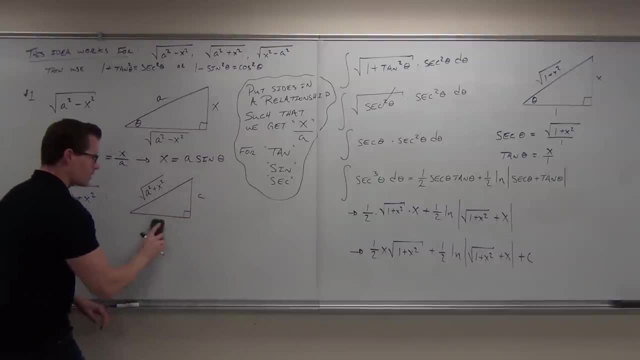 I don't want a over x. That would be a bad idea. What I want is x over a. So in our case our substitution would be: tan theta equals x over a. You okay with that one? Solve it for x. X equals a times tangent theta. 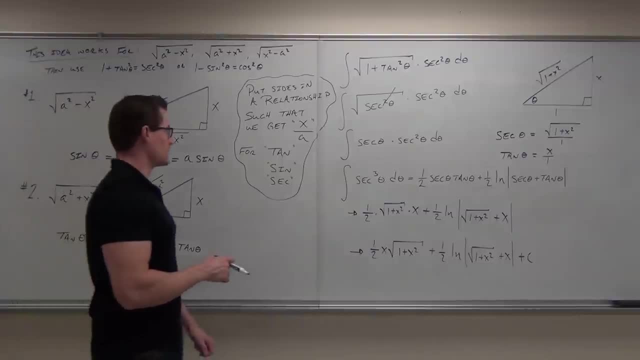 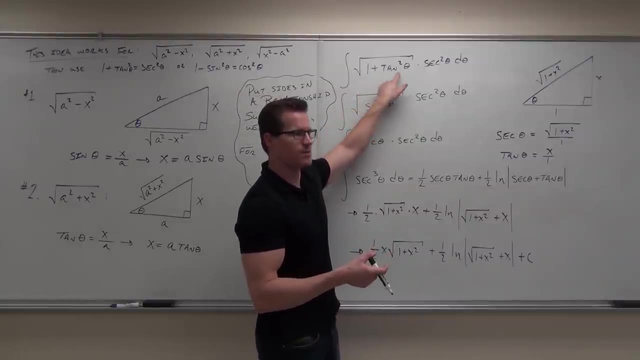 If you look back at the example which I left on the board, like parted on the board when we did this, when we did our substitution, that was it. X was one times tangent theta. That's what we had here. Then we squared that. 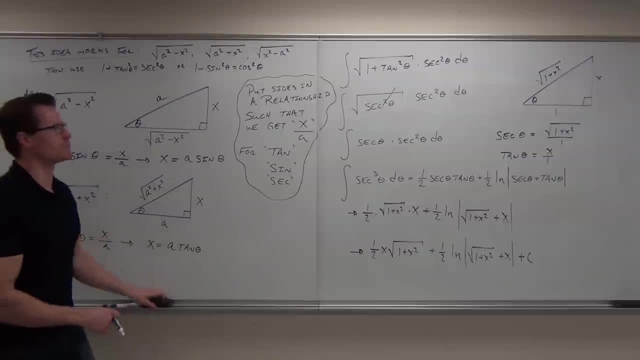 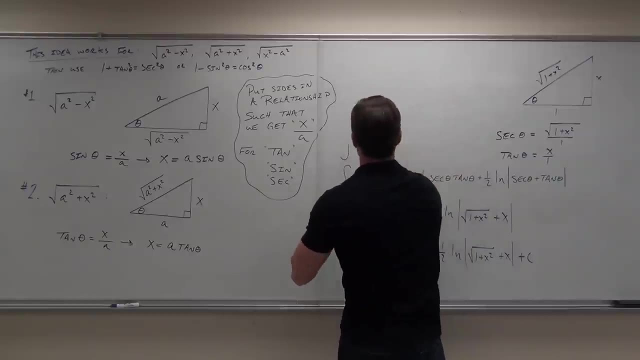 Still okay with it. Let's talk about the last one then. Then I'm going to have to erase all this. So if you have any questions, you let me know. But again, I don't really care if you memorize these ones. 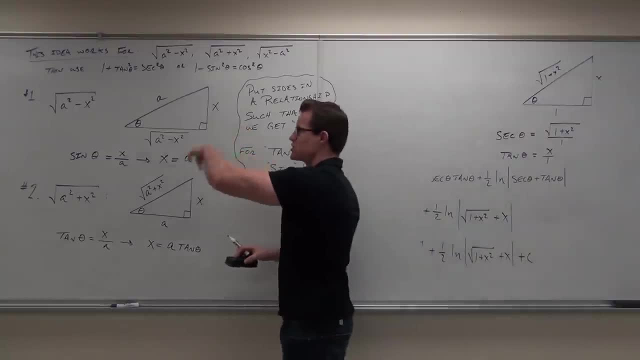 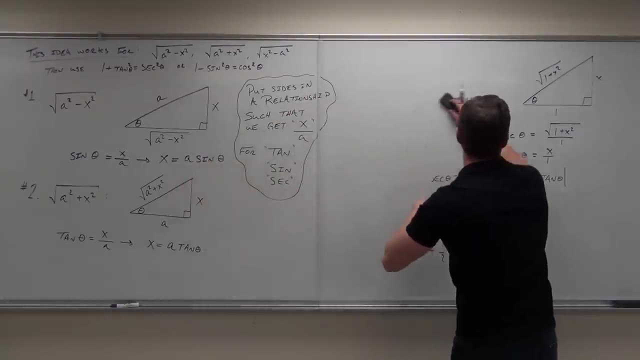 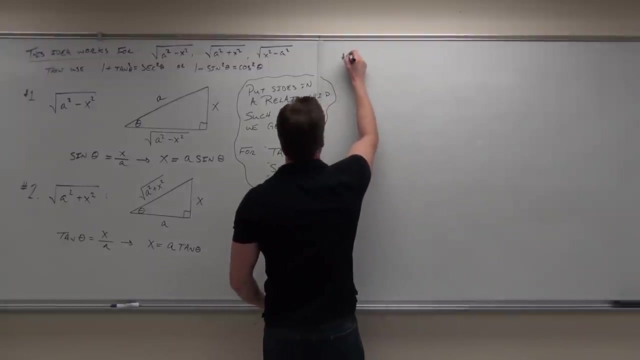 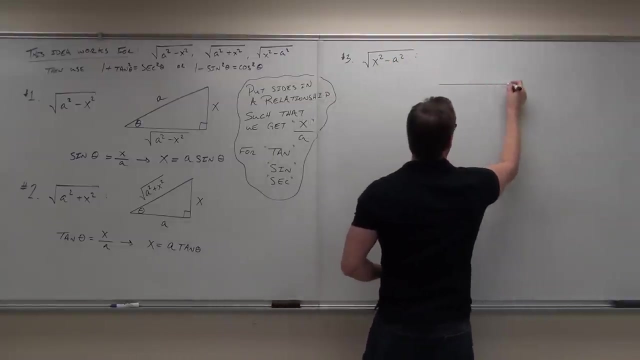 The way I'm hoping to teach you is that the relationship of a triangle- a triangle- has to make sense. Then you don't have to memorize the formulas. You can just do it whenever, without having to look at it as a formula. Okay, that was pretty good. 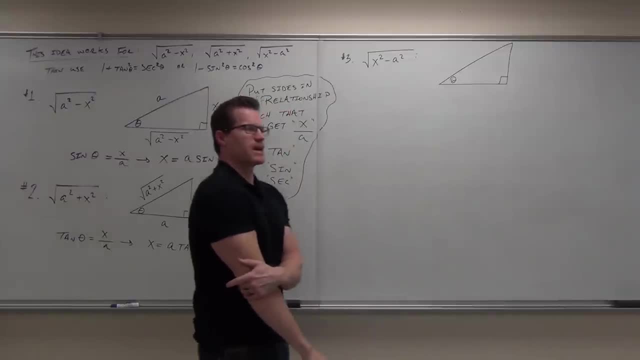 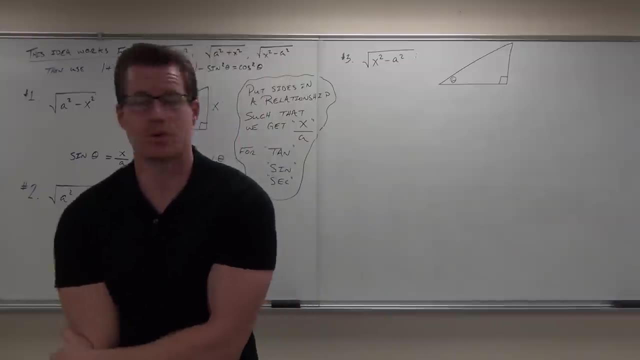 Okay, let's think through Square root of x squared minus a squared. Would you say that x squared minus a squared is a hypotenuse or a side? What do you think? Side- It's got to be a side. So it's either going to go here or it's going to go here. 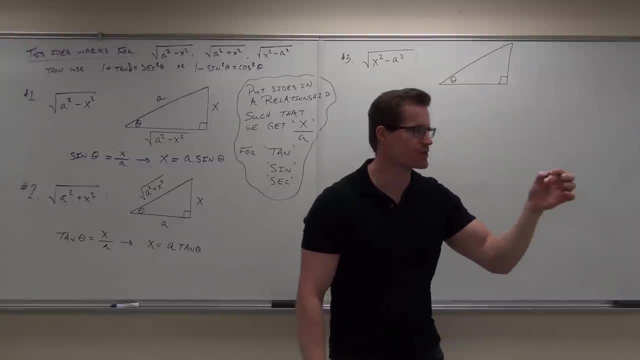 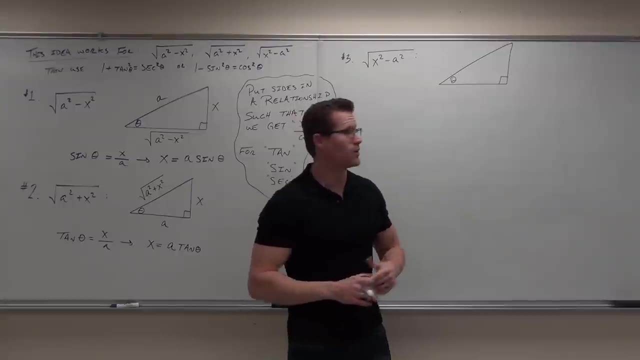 I don't know yet until I determine what the hypotenuse is. So let's talk about what the hypotenuse is. What's the hypotenuse? How do you know? it's x. Yeah, if it wasn't. if it was not a hypotenuse, this would be bigger. 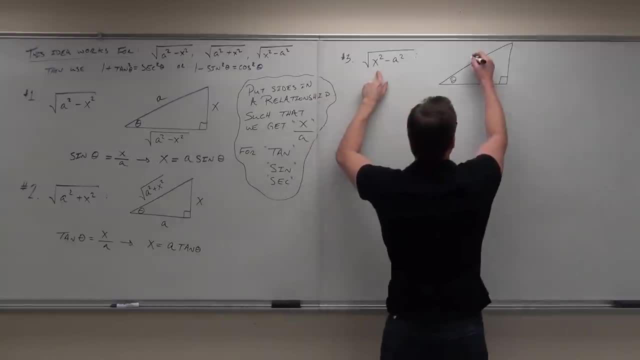 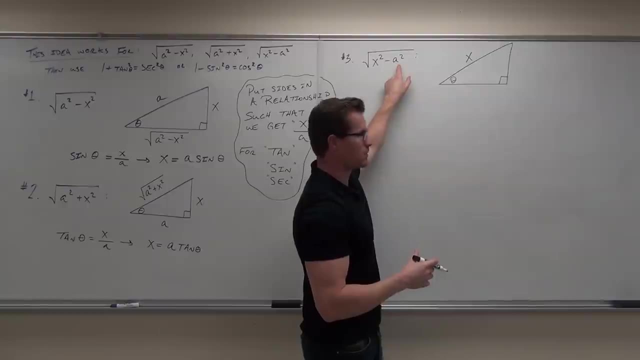 When I square those numbers, I get a negative. That's a problem. Okay, so x is the hypotenuse. Now we've got to put our sides, which are a. a is a side here, x is over here. 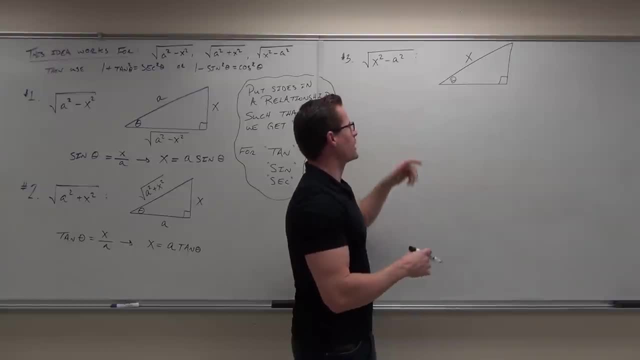 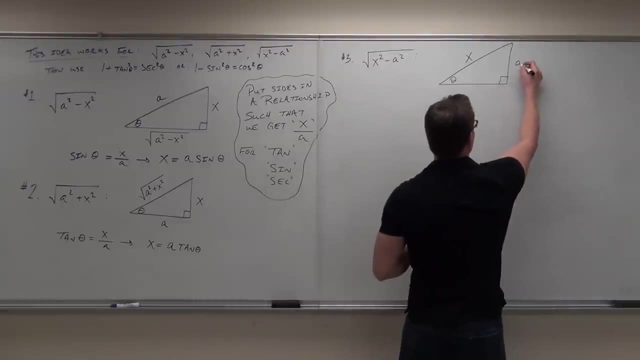 a is a side and this whole piece is also a side. All right, Where does the a go in this triangle Opposite over? Okay, let's try If I do opposite. Oh, no Side would give us a over x. 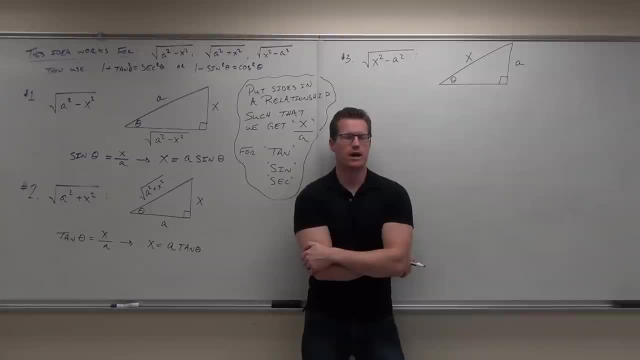 Do I want that? No, I want x over a, And I can only use a tangent, Sine and secant. So let's see which one of those work. Would tangent give me x over a? No, Would sine give me x over a? 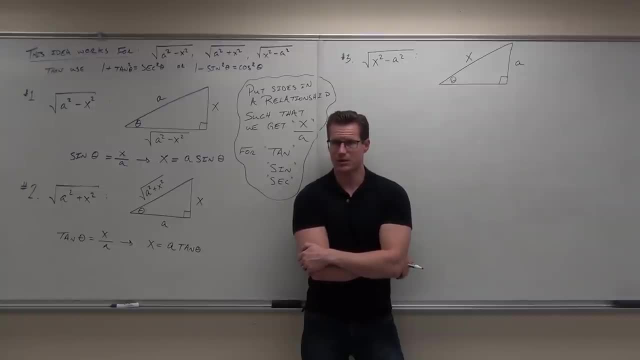 Secant, Okay. so if that doesn't happen, what's it going to be? The a is going to be, It's got to be secant, And the only way to do secant is to move the a from here to there. 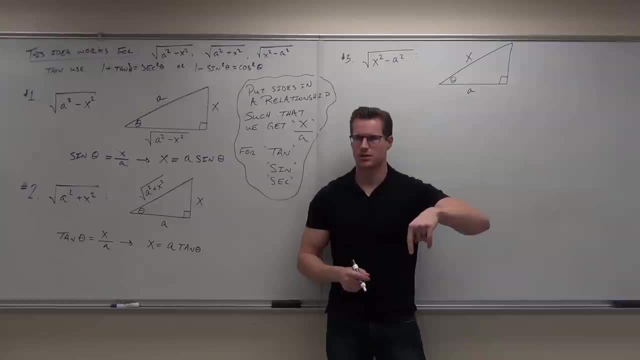 Secant is hypotenuse, over adjacent. So if I say, hey, the x is the hypotenuse, guess what? I'm using Secant, Secant, Hello. that's the only way it works. So if x is the hypotenuse, I'm using secant. 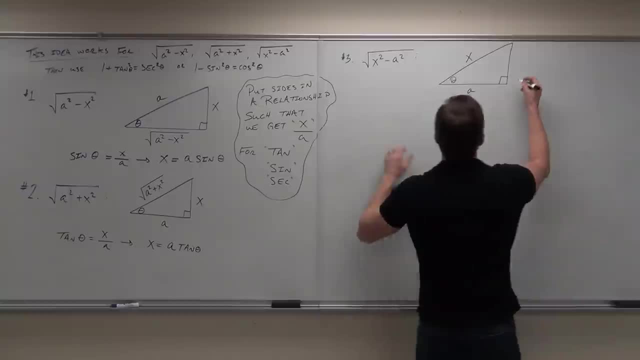 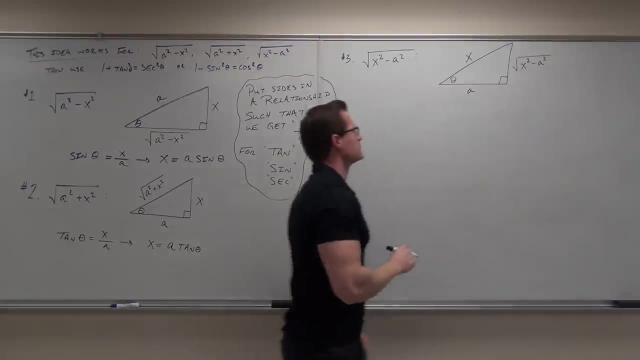 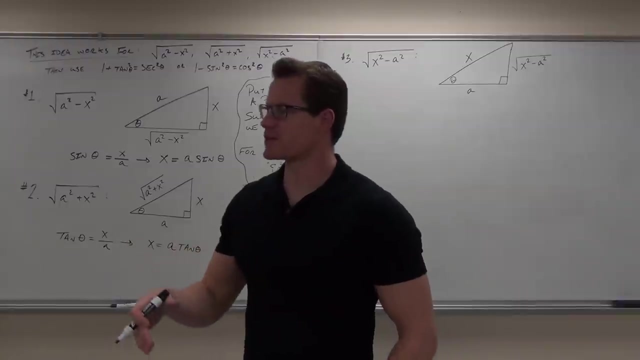 Does that make sense? Yeah, Then this is x squared minus a squared. In this case you go okay. well, let's make our trigonometric substitution. Let's make something so that our trig function gives us x over a. 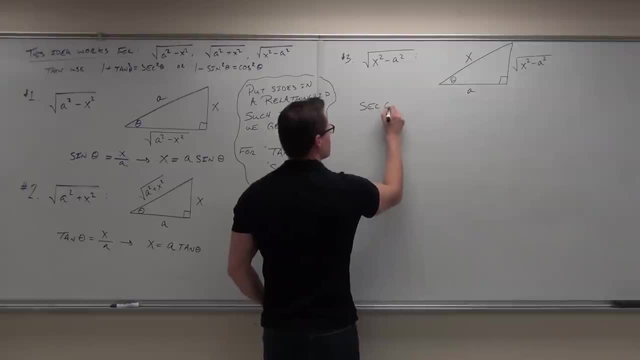 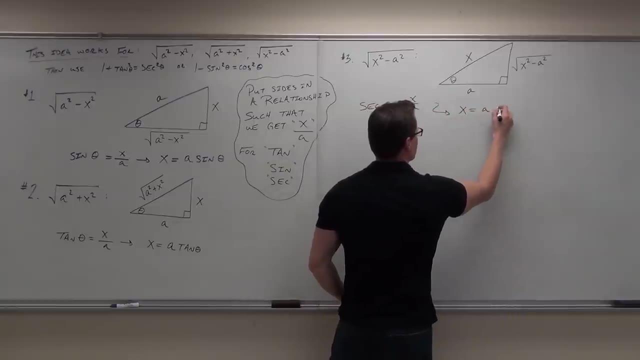 The only one that works here is secant, So secant theta is x over a If we solve for x. If we solve for x, our substitution becomes x equals a secant theta. In each of these cases we've used a triangle. 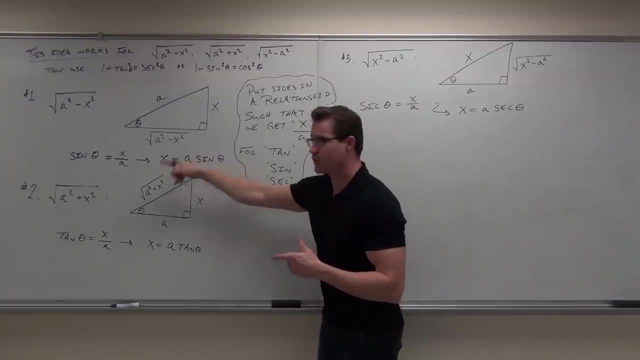 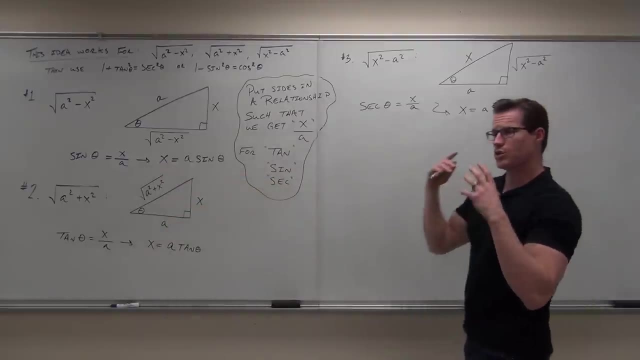 We've created a trigonometric substitution. After this, we take a derivative of both sides That lets us change our dx into a d theta, dx, d theta, dx into a d theta. We do our substitutions and then we have a trigonometric integral which we just covered, that section for. 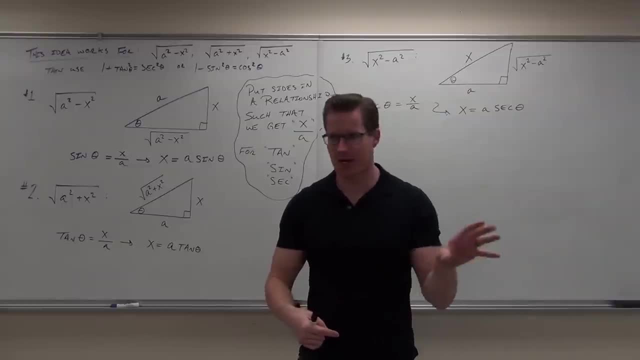 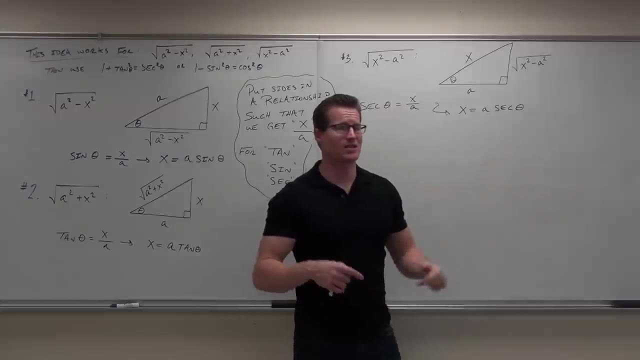 Get the idea Kind of cool right. Well, can't you forget What do you get at the very end of your integral to do Triangle. Yeah, So we use a triangle to do this. We're going to use a triangle to undo this as well. 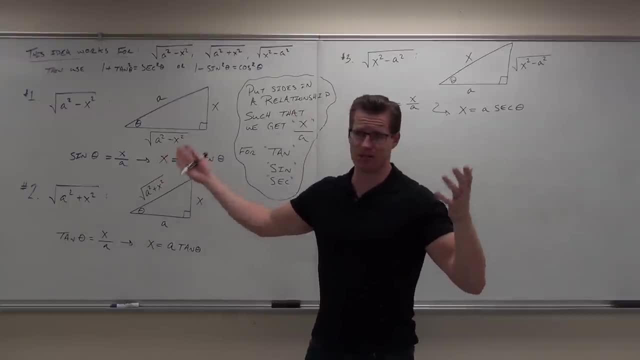 It's time for some practice. This is it. This is the whole idea. If you get this idea, you're done. All right, It's practice. It's not as easy as I made it sound. All right, Right now it's like: oh, this is a piece of cake. 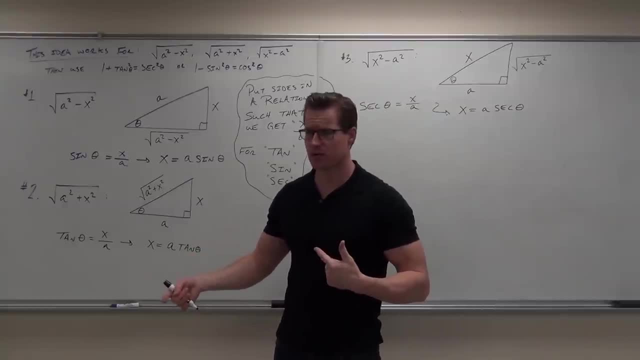 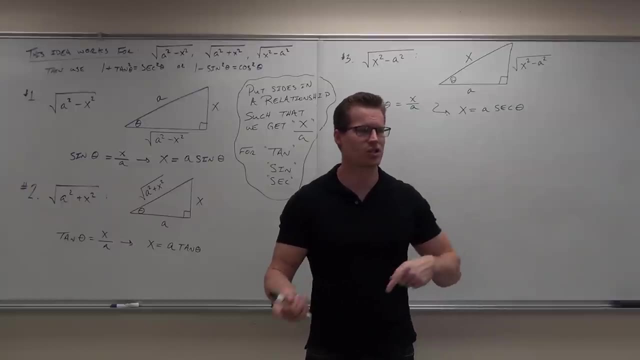 They do get a little tough. Mostly it's just working with the trig and not the substitution. You guys should be almost pros at that just after looking at this. It's typically the trig integral that gets like: oh man, because you're going to be. 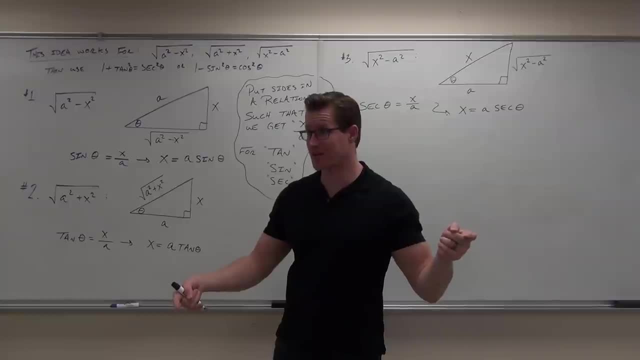 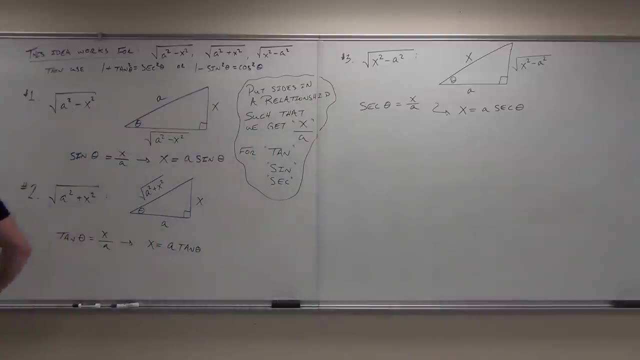 doing the last section stuff again. Lots of practice here. You guys ready for some practice, Exciting A little bit. I'm so excited, I don't know. It's fun for me. Will we be able to do the whole section, just knowing this. 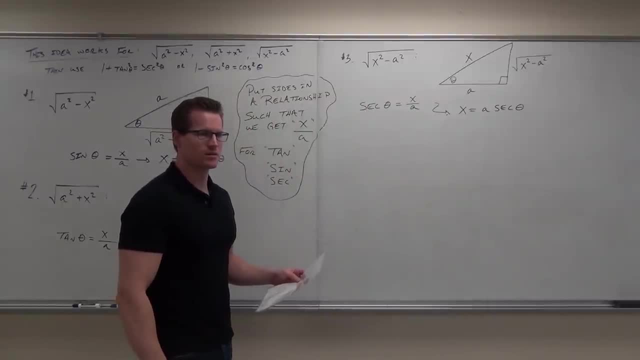 Will you be able to do the whole section just knowing this? Yeah, Is this pretty much like the bread and butter of the whole thing. This is trigonometric substitution. Second, bound for the homework. Yeah, That's pretty great. Seven, three. 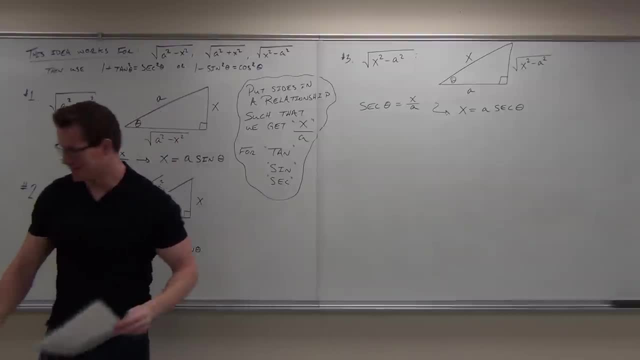 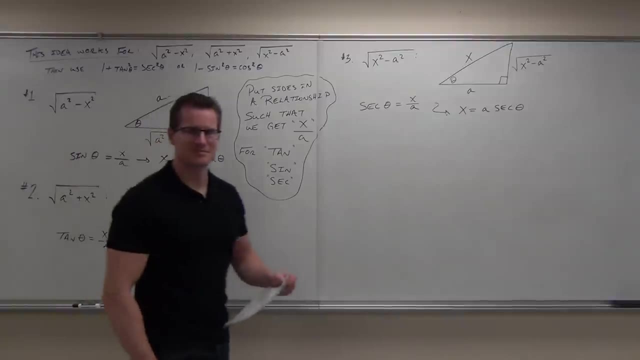 This is pretty much seven, three. Pretty much it. OK, Yeah, Which I think, Unless there's anything else that doesn't happen. Yeah, That's it, So we can do our homework after. Yeah, Why don't we just end right now, then huh. 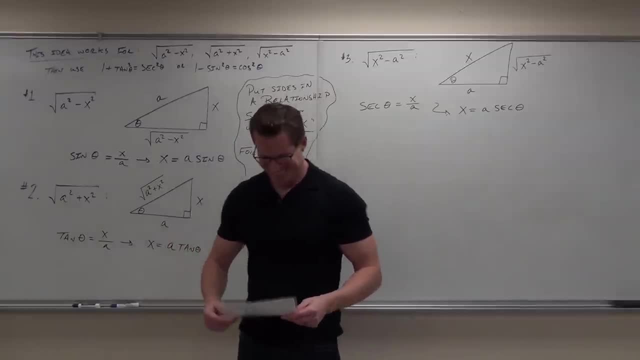 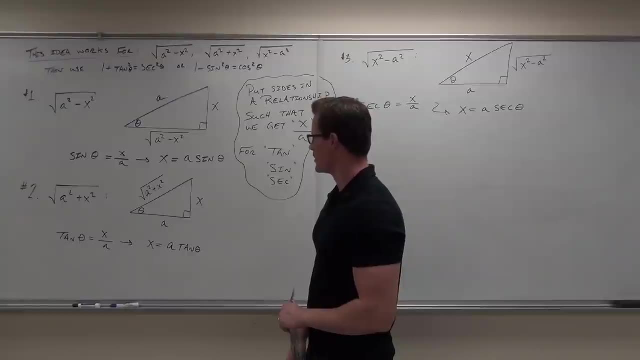 No examples whatsoever. Fantastic, You know. one more thing that I want to put up here for you that I didn't put up: If you're going to do this substitution, you're going to be getting a sine squared. See it, If you get a sine squared, then you're going to be using this one. 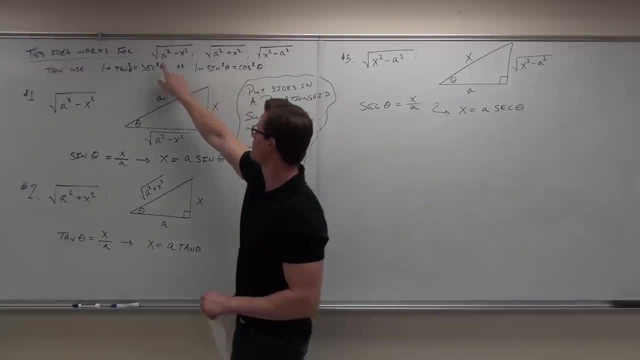 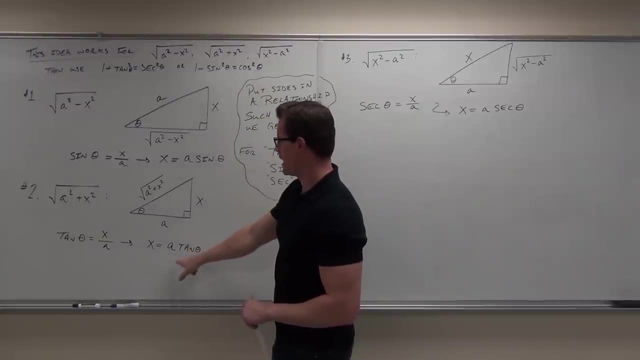 You follow me. You're going to have something minus a sine squared. You'd be using this identity. If you're going to have a tangent up there, you're going to have something plus tangent. You'd be using this one. Does that make sense? 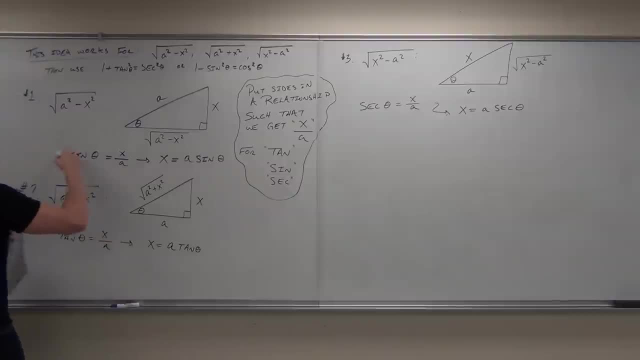 So let me write this for you here. So once we have this, the substitution we would have is one minus sine squared theta. Sine squared theta equals cosine squared theta. This would be the identity we'd be using. Once we have a one plus tangent squared theta, you'll be using one plus tan squared theta. 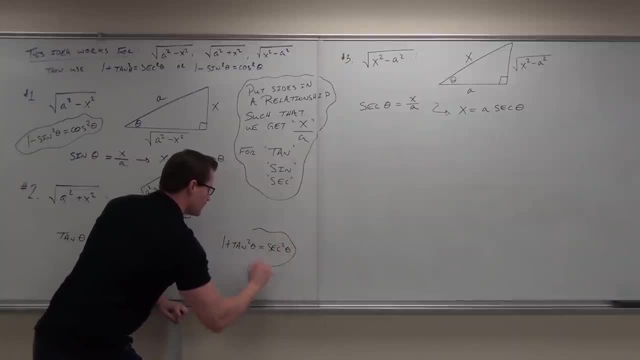 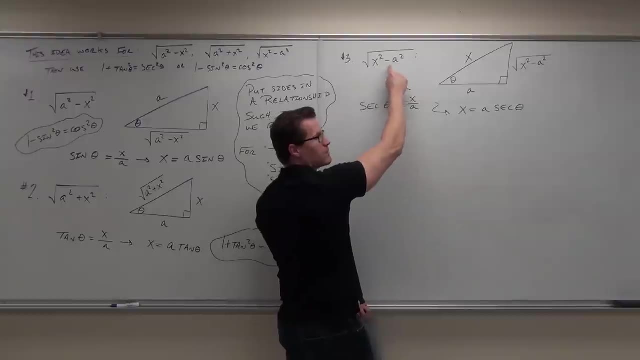 equals secant squared theta. This one, if you have a secant, look at this. If you made the substitution, you'd have secant squared minus something. You have secant squared minus one. We'd use secant squared theta minus one. equals tangent squared theta. 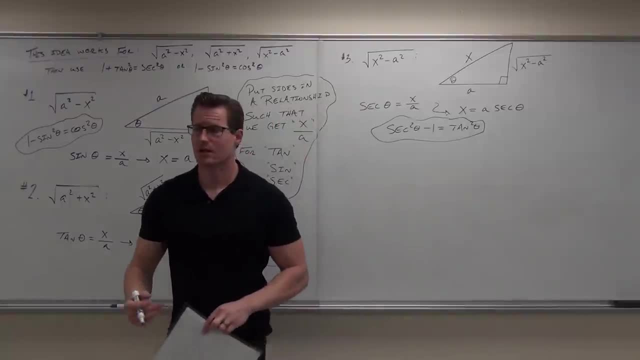 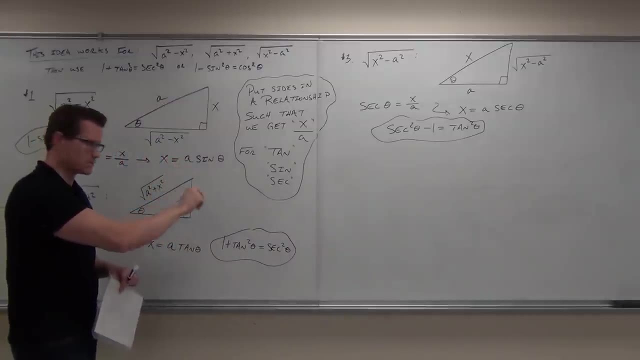 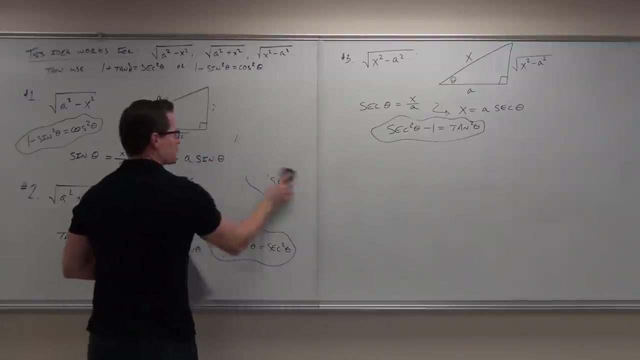 And those would be the follow-up identities that you're going to use here. Now let's practice. Do you have this written down, everybody? Yes, no, Yes. Let's practice Again. I don't care if you memorize the formulas. 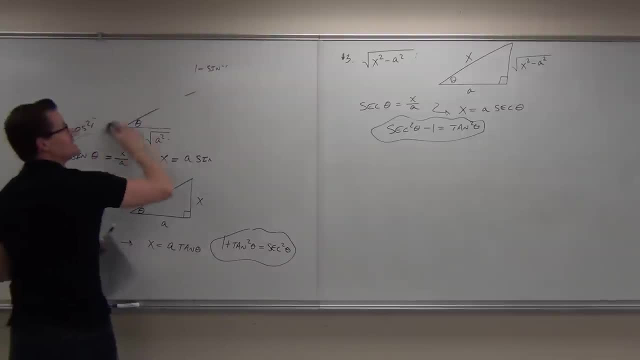 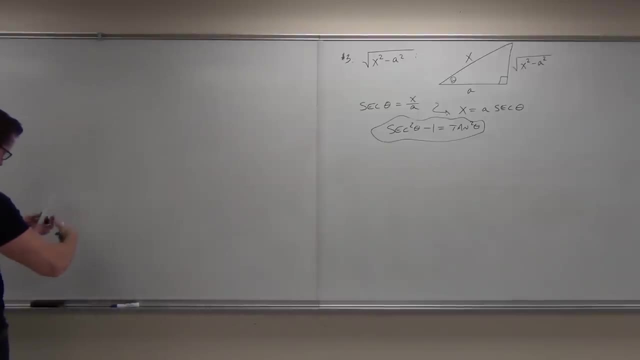 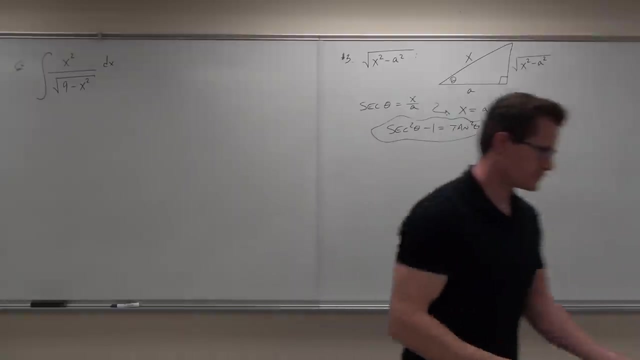 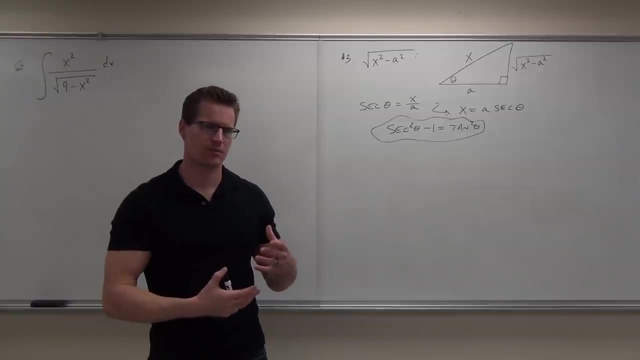 It's going to be obvious what you do If you understand the idea. So let's do some. how about this one? Go through these integrals, not just that we're in a certain section for trigonometric substitution. Go through them and see if you can actually do them without it, like if I give it to you. 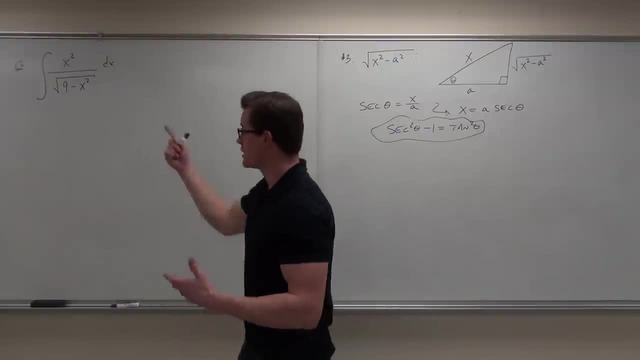 on a test. I'm not going to tell you what to do, So go through it. See if you can do it with a substitution. If you can cool, Do it. See if you can do it. integration by parts, if it's really quick. 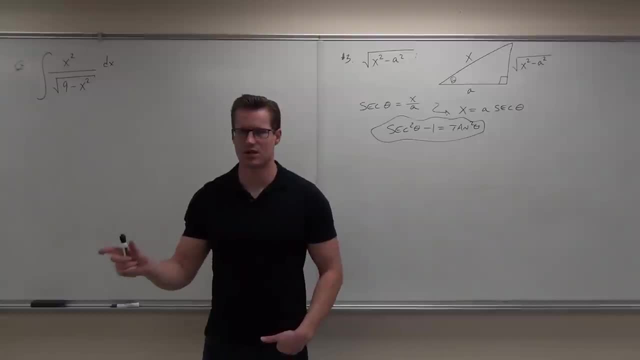 Okay, I can do that. See if you can do it with just basic trigonometry. if it has sines and cosines up there, Do it Go to trigonometric substitution, of course, if you have something like this. But try some of those things. 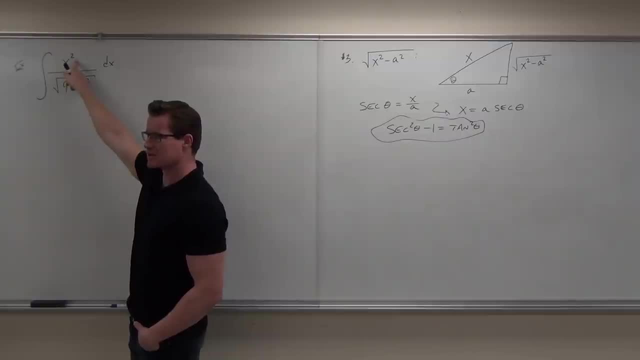 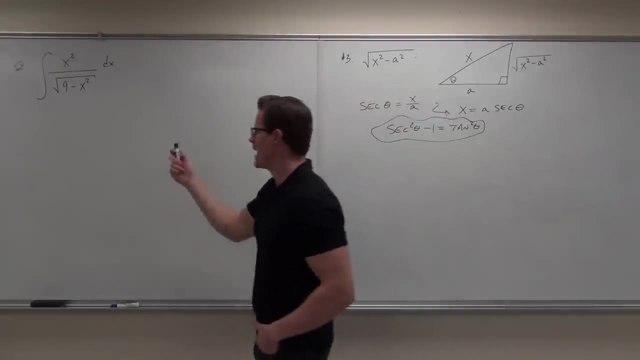 Like, if this was just x, If that was just x, I'd go for it. I'd go for a substitution. I wouldn't start a trig sub because it would be easier than that. Does that make sense? Okay, in our case, we have well, nothing but a trig sub here. 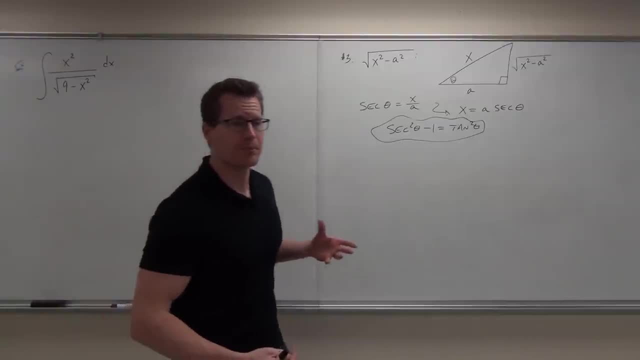 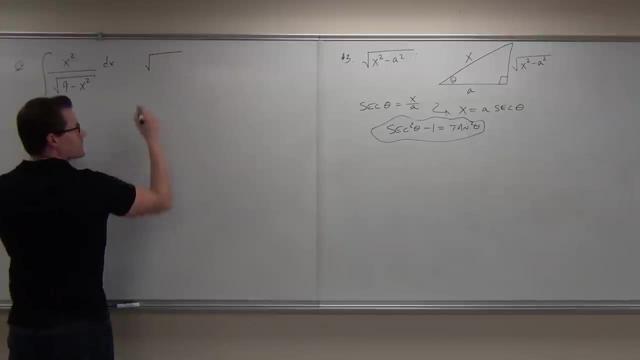 What piece are we looking at to substitute? Yeah, so let's take a closer look at the square root of 9 minus x squared. But you know what? I'm not going to think about it as 9 minus x squared. I'm going to think about it. 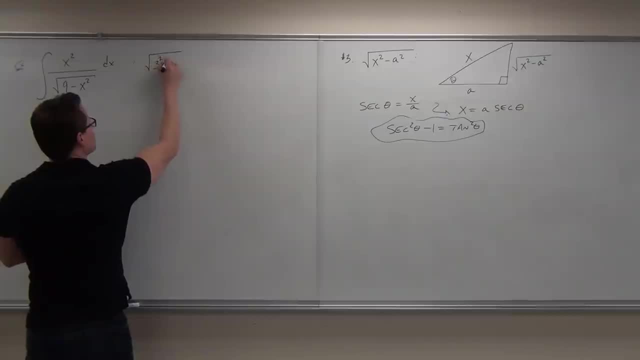 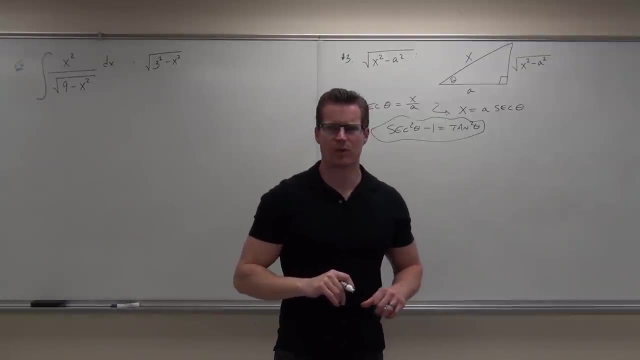 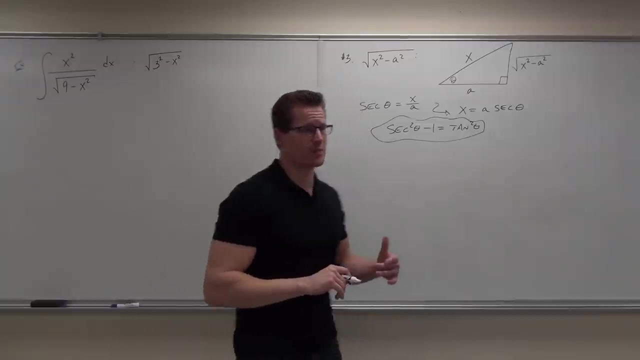 I'm going to think about it, as Almost begs the question. well, wait a minute. What if it wasn't 9?? What if it was 7?? Could you still do it? Yeah, You've got to think outside the box, though. 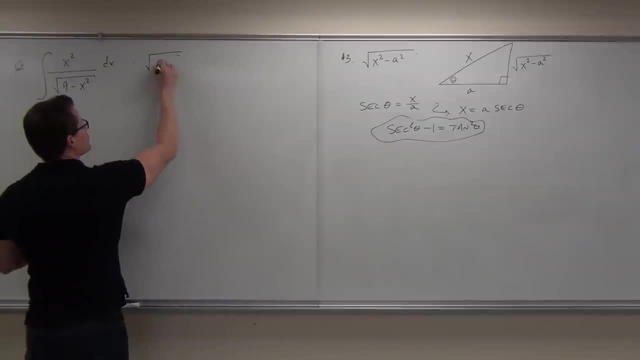 If this was a 7, you could do something like the square root of 7 squared. That would give you 7.. Does that make sense? It's harder. Generally. we get those perfect squares, which is really nice, But you don't have to. 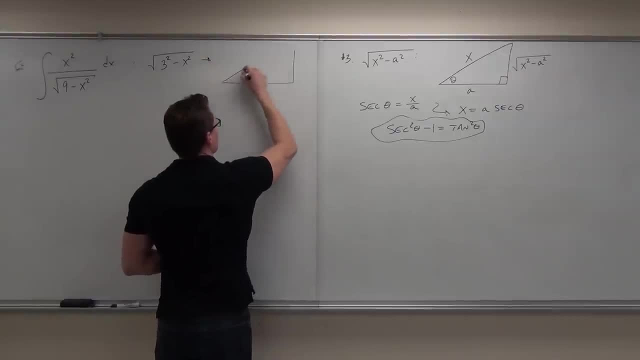 Okay, here's where the rubber meets the road. Basically, all you have to do is know how to draw your triangle- I mean, not just a triangle, but know how to put the sides on the triangle. That's the key thing. 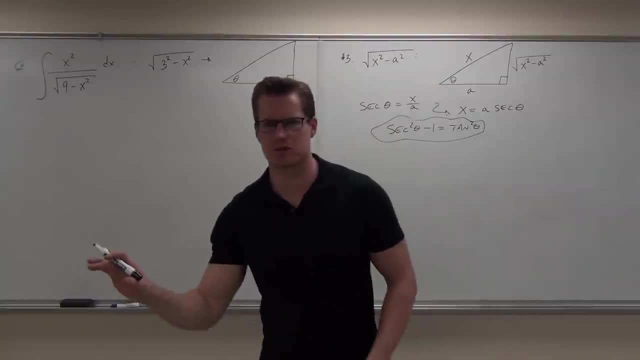 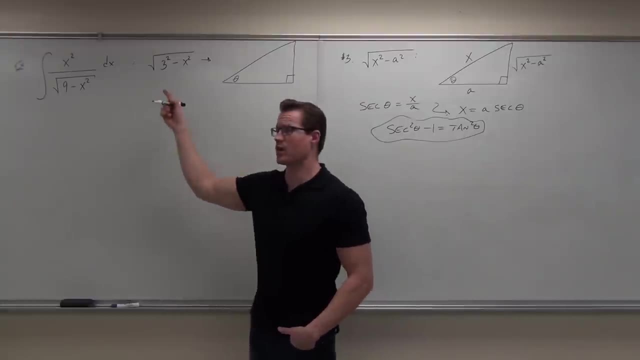 If you can do this correctly and make the appropriate substitution, everything else falls into place really nicely, So let's walk through it. I don't want you to just look at your notes and memorize the formula. I want you to think through this. 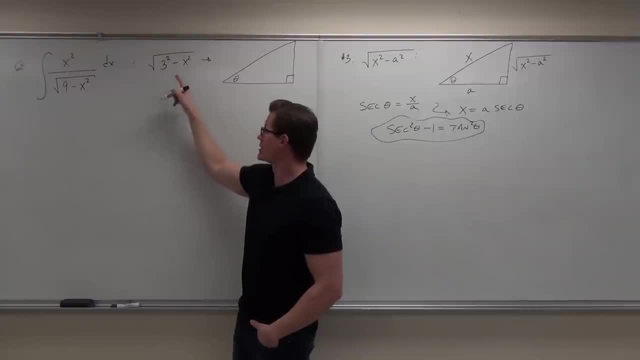 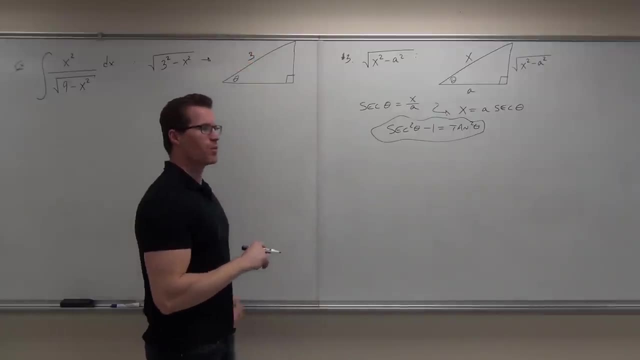 Would you say that this is a side or a hypotenuse Side? It's a side for sure. Can you tell me what the hypotenuse is here? 3. So create a triangle. That's 3. Tell me what one other side is. 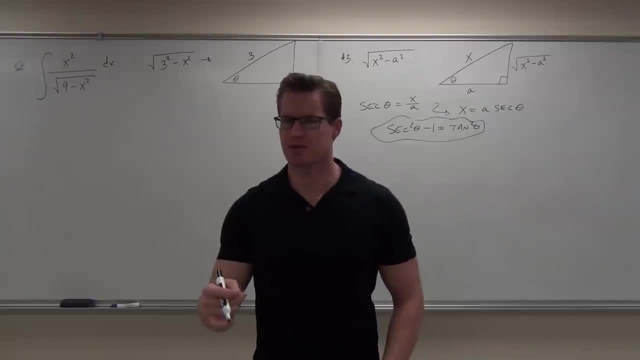 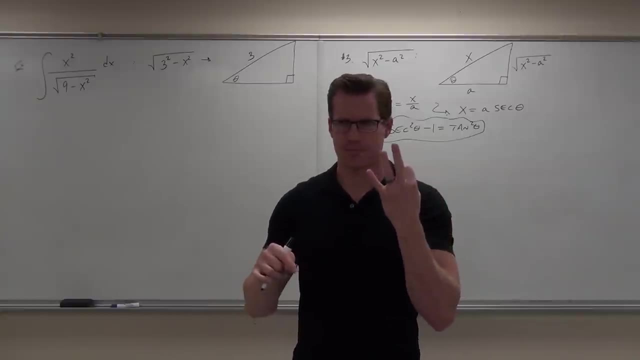 X. Now we want to put this in a relationship so that we get x over 3. with what three functions are we looking at? Sine and sine. Okay, I heard a lot at once. Hopefully you said sine, tangent and secant. 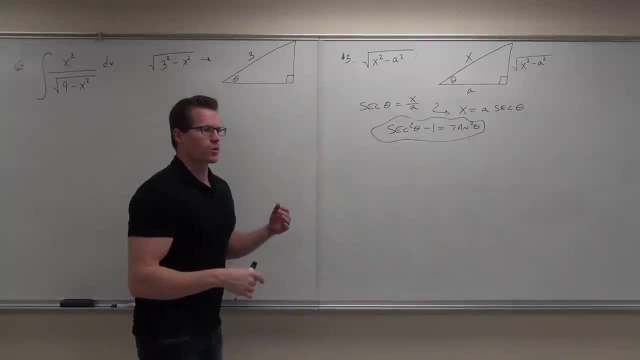 That's right, Sine, tangent and secant, Let's see which one would work for us. Is tangent going to put x over a? for us? No, Tangent would put whatever You're going to have a square root somewhere. 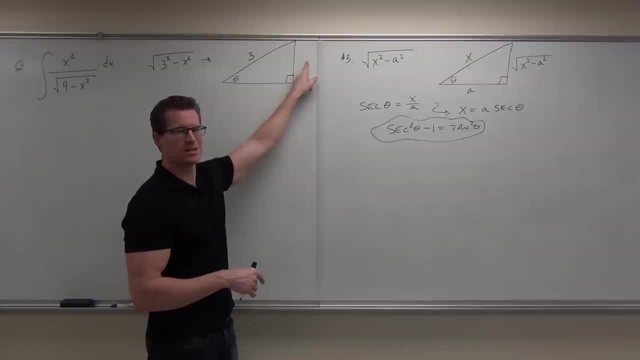 That's not good. Would secant work for us? No, No, secant could put 3 over x, but not x over 3.. I don't want to do that, So what's the only other option for us? Sine. 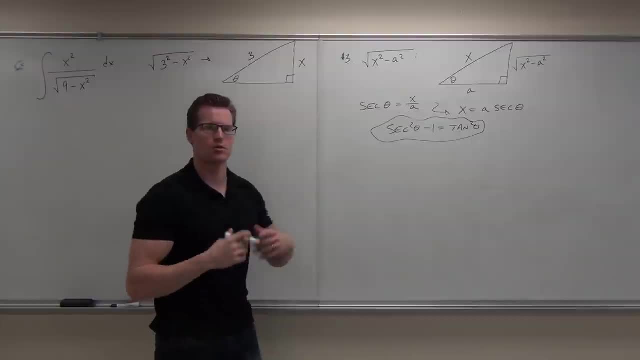 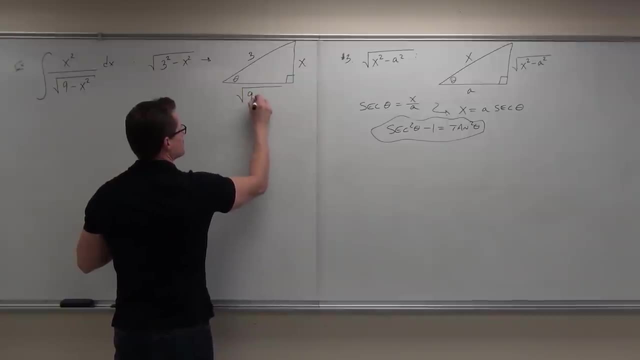 Sine, So you need to work with sine. X would have to go there to work with sine. Does that make sense to you? Yeah, The other side. now we change it back to 9.. Square root of 9 minus x squared. 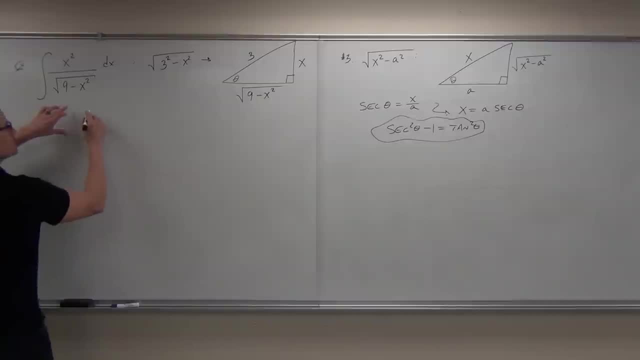 Let's go for this, Let's do our substitution. So the first thing we've got to do is: what's our relationship? again, One more time, What do we have? 3 sine theta equals Good. So sine of theta equals x over 3.. 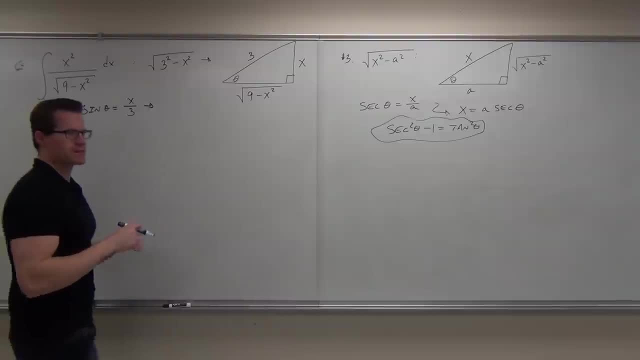 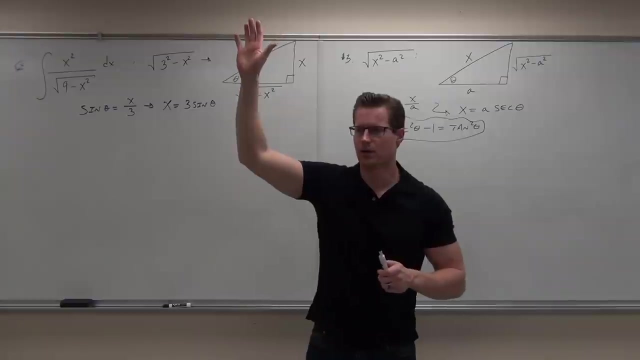 equals x over three. that makes sense, doesn't it? Sine of theta equals x over three. opposite over hypotenuse. Therefore, x equals three sine theta. Quick show of hands. if you're okay with that one, Cool now what else are we gonna do right now? 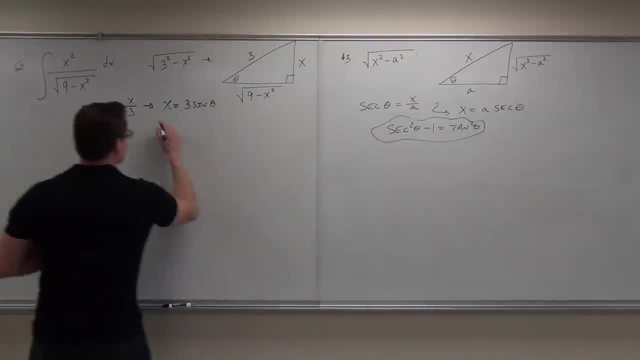 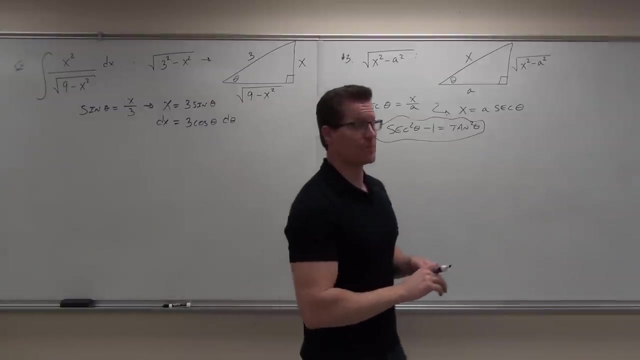 that we've done our substitution Dividing- Yeah, that's a great idea. So dx would equal Three cosine of theta. D theta, I mean d theta. So hey, we've got our substitution. Are you guys okay with this so far? 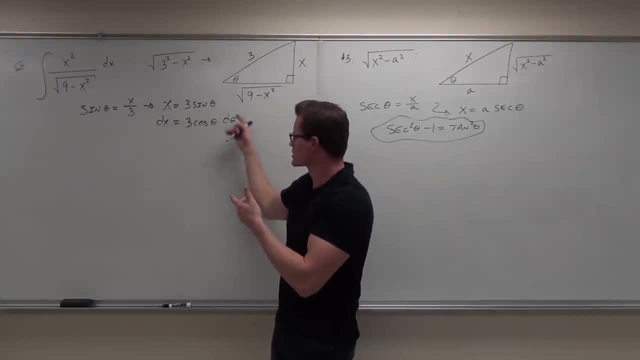 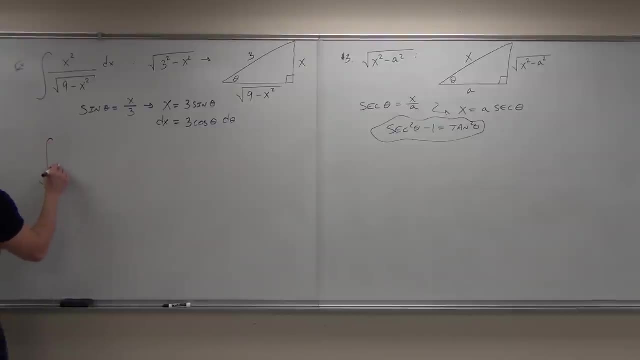 We've got x equals three sine theta. no problem, Take a derivative: dx equals three cosine d theta. Now we get to substitute with all this stuff. So let's see how it works out for us In this type of process. 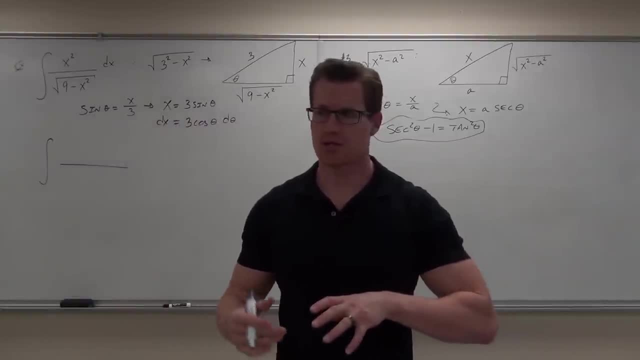 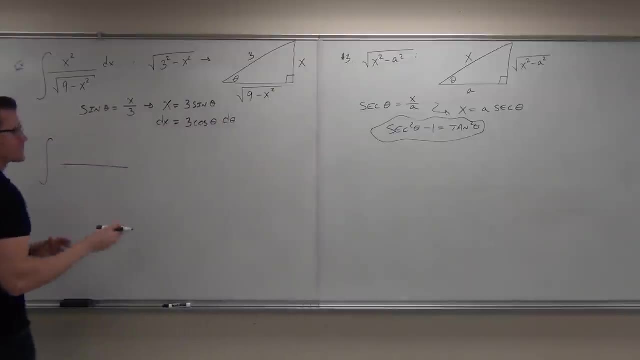 everywhere you see x, you're gonna have to substitute. There's gonna be no elimination of x's because you're getting rid of all the x's with your thetas. So tell me what's gonna be on the numerator, please. We gotta move a little quicker here. 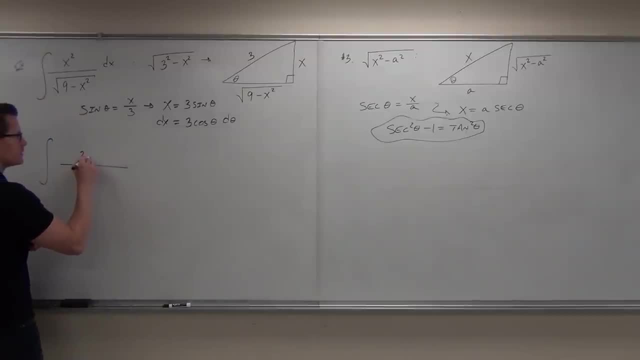 What's that? Three sine squared Three. what Sine of three sine of theta? Okay, so three isn't three gonna get squared here. Yes, Yes, it's part of your x, So this whole thing gets squared. 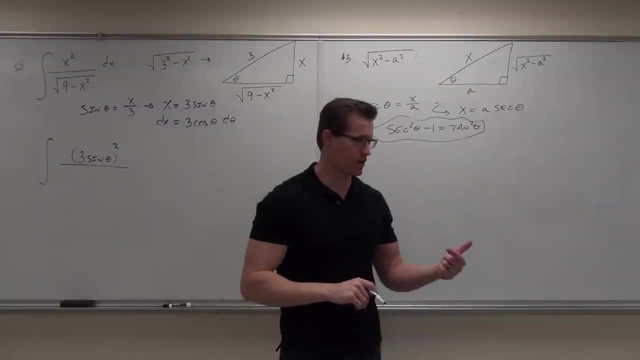 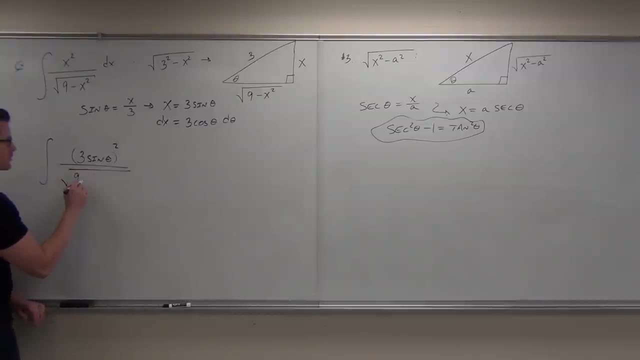 If you put three sine squared theta, you missed out on your constant. You missed that Denominator: Square root of nine minus Nine's still there. very good, What's Minority of sine of three? Three sine theta? and then what? 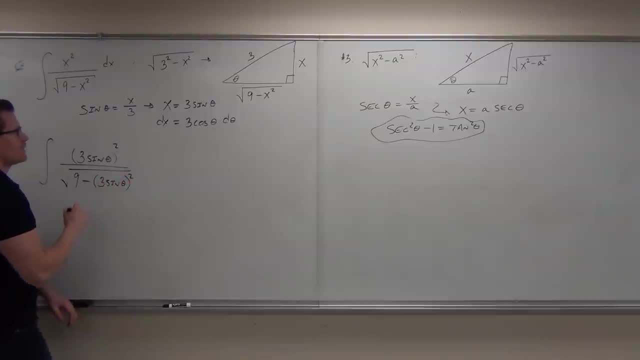 All squared. All squared, very good, I like it. And then, oh man, we got a d theta as well, I'm sorry, dx as well. What's the dx become? Three cosine of theta d theta. Okay, honestly, if I did this at the start of class, 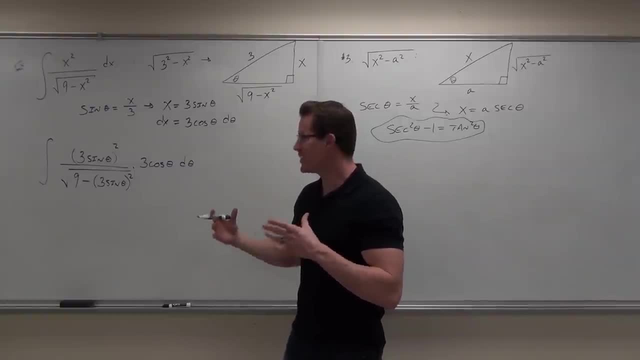 you'd probably be like what in the crap is going on here, But let's see if it makes sense now. Are you guys okay with a triangle? It's just a triangle. you gotta be okay with triangles, They're fun. Make up the relationship so that this fits okay. 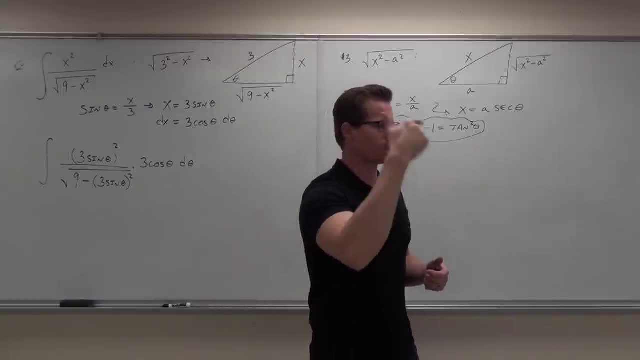 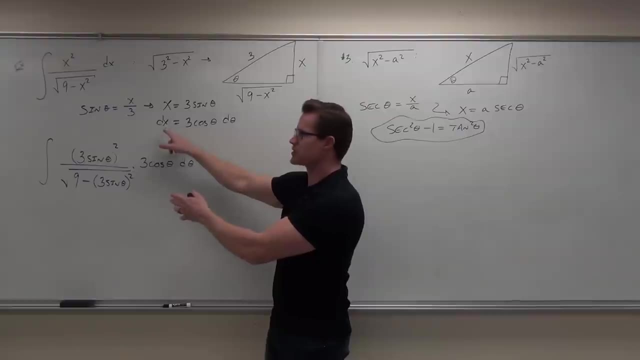 and that you get a trigonometric relationship. you want Sine, tangent, secant where you get x over a. That's the whole deal. Once you get that, everything else works out real nice. So we got well most of the time. 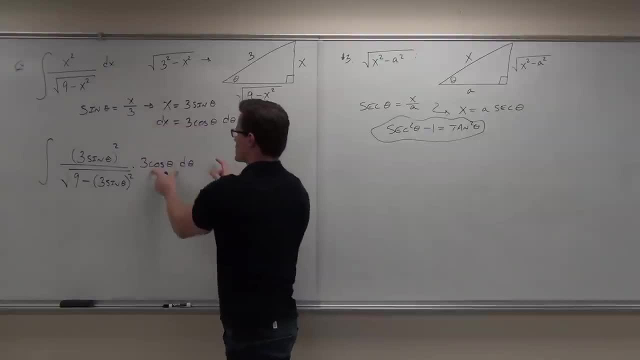 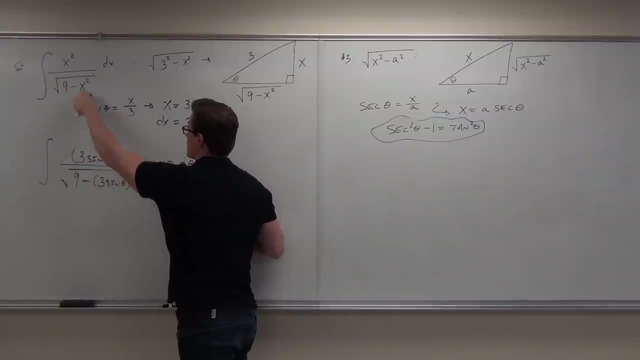 We got dx equals three cosine d theta. That's where this comes from. We got x equals three sine theta Square. nine cool minus minus three sine theta squared. Now it's just a matter of simplifying. Don't try to work with it now. 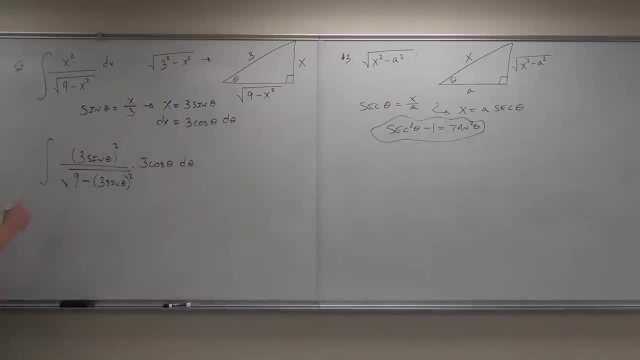 Simplify what's going on here, So let's do it. This becomes nine times sine squared theta. This becomes the square root of nine minus nine sine squared theta. And this is still three cosine theta, D theta. We're just doing some algebra right now. 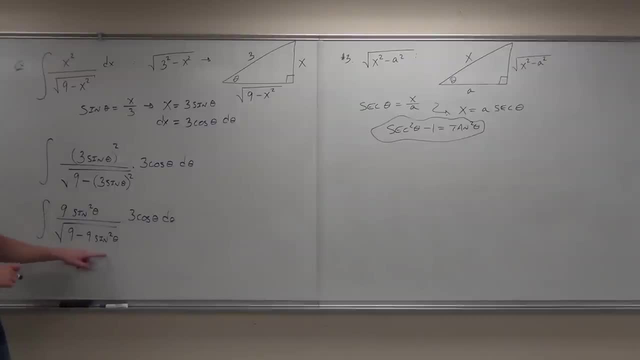 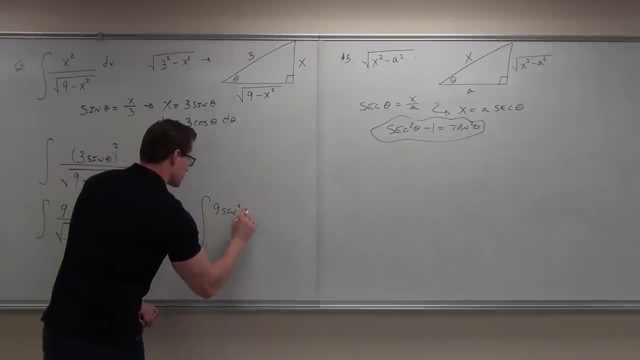 Now here's the issue. This is almost, almost an identity, but it's not. Why is it not an identity? The nines are there. Well, let's factor the nines. Yeah, let's factor that out. So nine sine squared theta over square root of nine sine squared theta over square root. 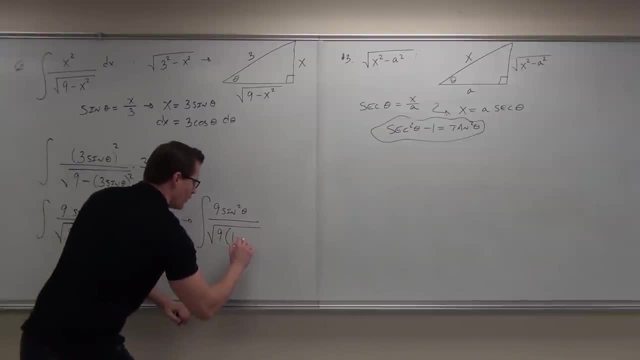 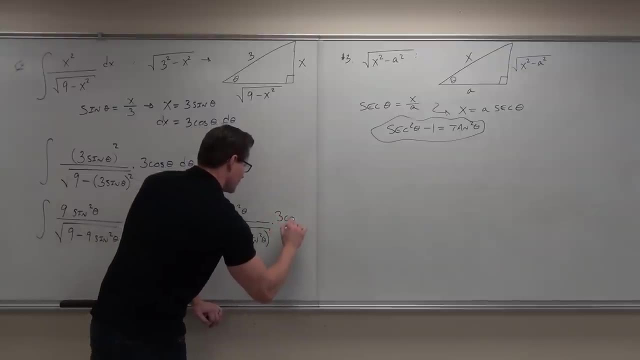 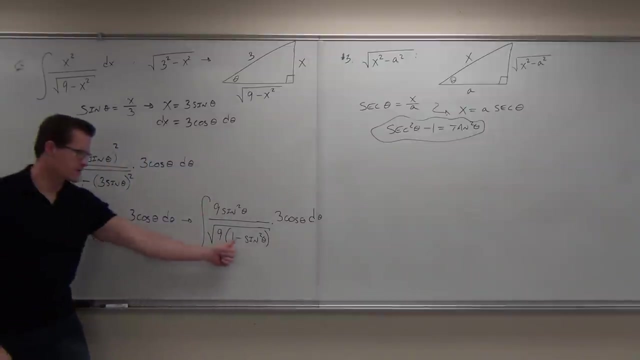 of nine. If we factor those nines, I get one. oh beautiful, Look at that. Love math, Cool, That's the same This: we factor out the nines, We got one. minus sine squared theta, we got three cosine theta d theta still. 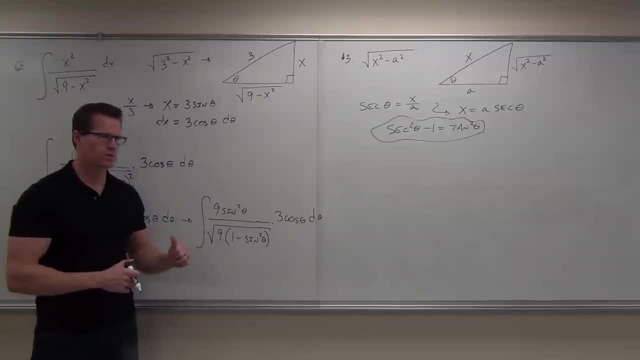 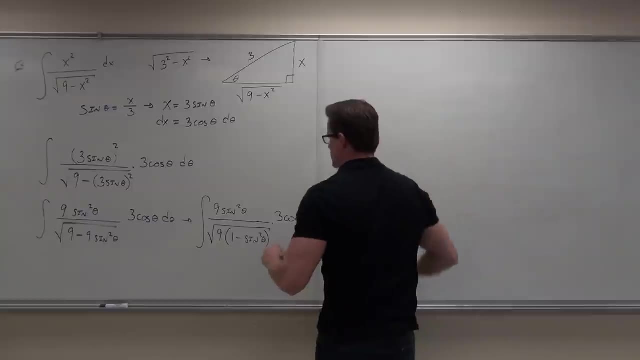 You guys still okay with it. Tell me what happens when I have a product within a square root? What can I do with that? Pull it out. You know we're going to have products within square roots, So let's see if we can do this. 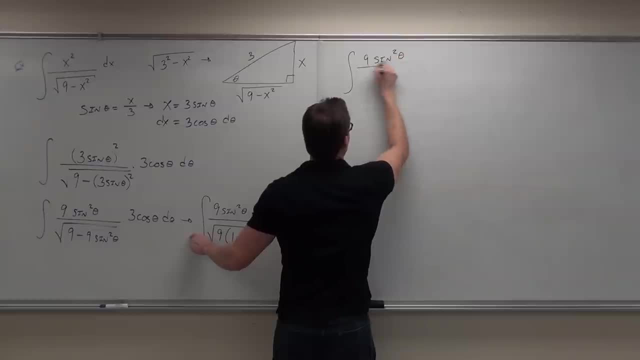 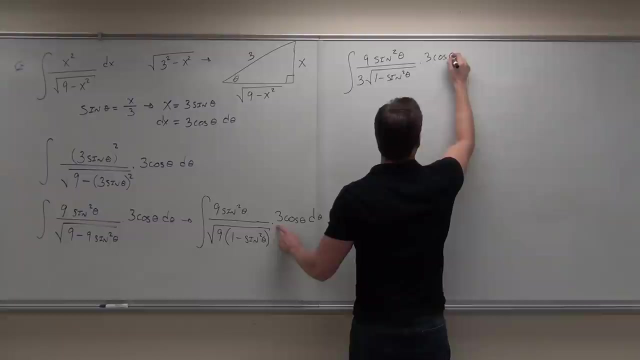 We've got nine sine squared theta. We've got what's the square root of nine And then the square root of one minus sine squared theta. and then we've got up here a three cosine: theta d theta. Threes are gone. 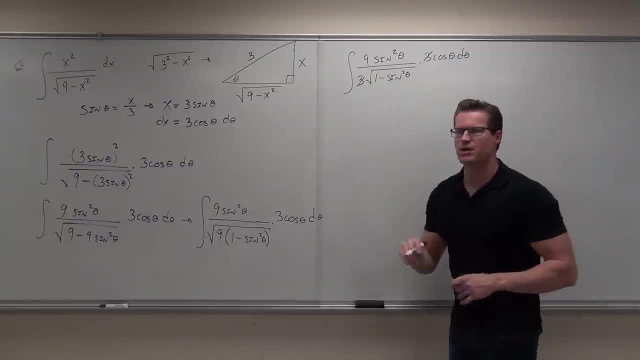 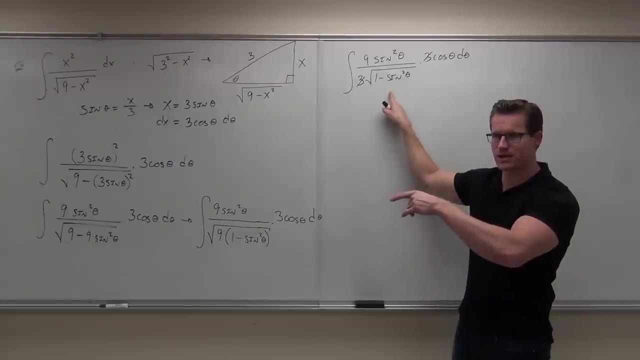 Three here, three here Also. check it: one minus sine squared theta. This is why we did that substitution, because this will work for us. So one minus sine squared. what is one minus sine squared theta? Cosine squared theta. 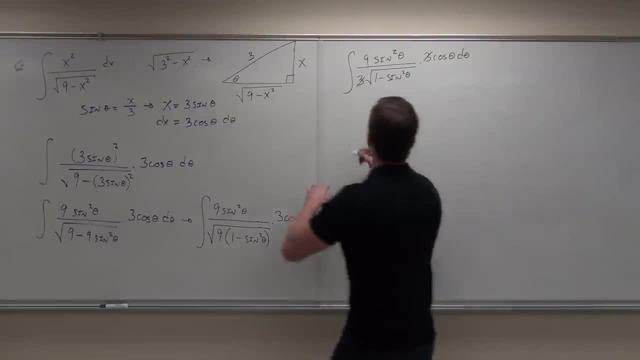 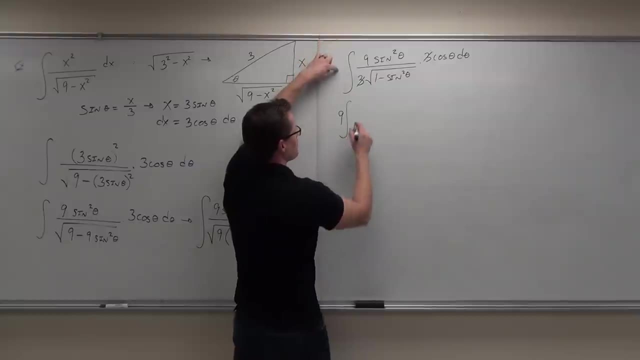 That's why we use sine. okay, Because that works nicely for us Also. what else is gonna happen? Pull the square root of r. Okay. so nine is here. I've got sine squared theta. I have square root one minus. 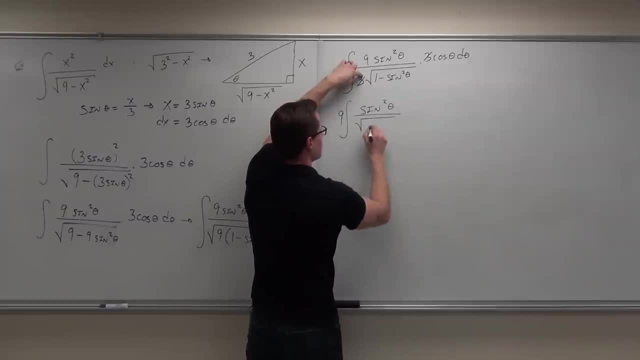 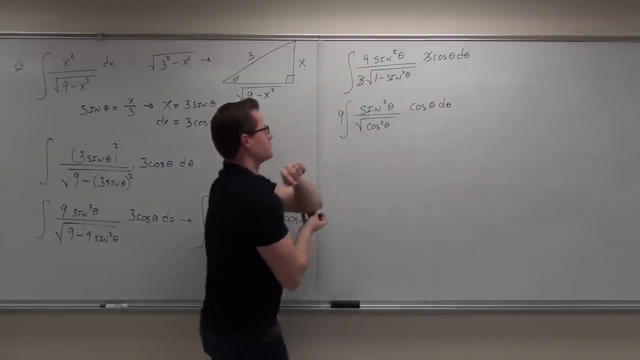 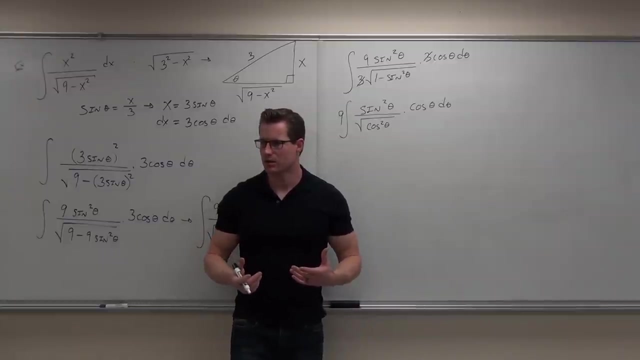 oh, sorry I messed up. I've got cosine squared theta times cosine theta d theta. We still okay so far, It's getting nicer notice. have we done any calculus right now? No, Not really at all. All we've done is manipulated. 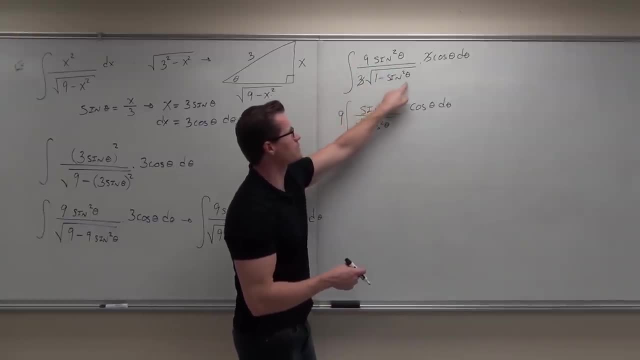 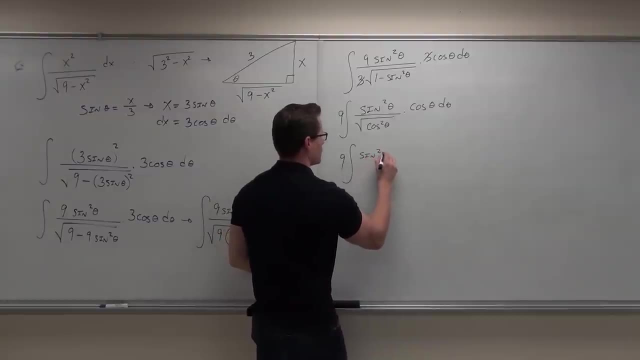 So we've got nine out front. threes are gone. this is cosine squared theta. it's still in the square root. tell me what happens with that square root. It cancels, It cancels And then the cosine cancels. 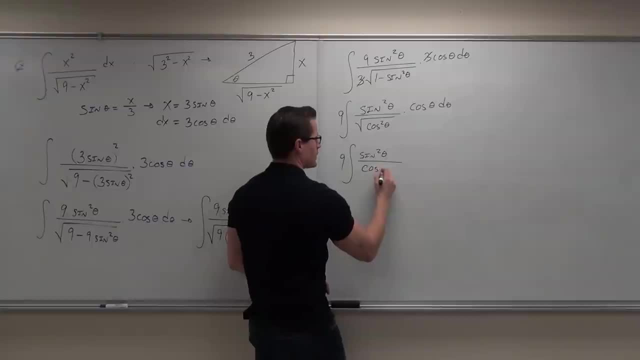 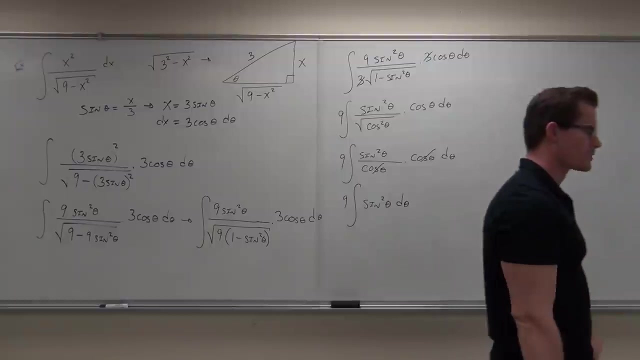 And then we get sine squared. yeah, So we have cosine theta times, cosine theta d theta. Those are gone. We have nine integral of sine squared theta d theta. Can we do the integral of nine square nine, sorry, nine, integral of sine squared theta. 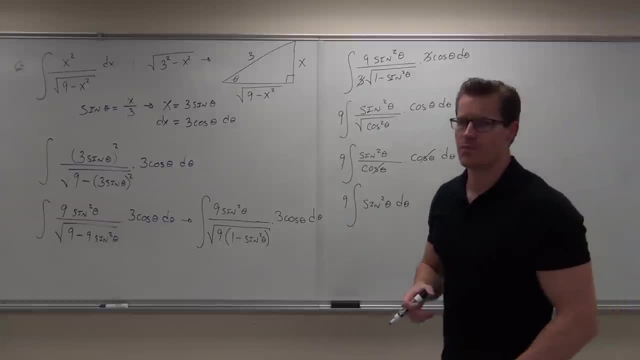 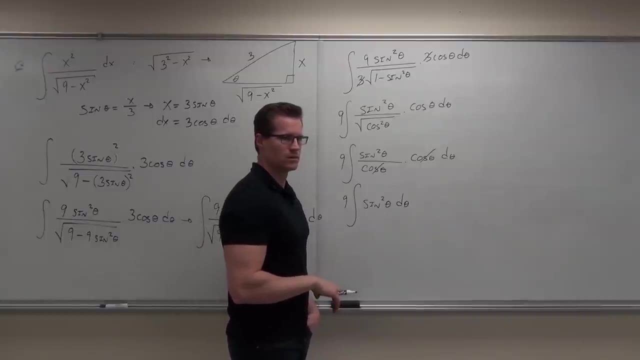 Theta, How would you do it? Reduction, Reduction, You could do, reduction formula, you could. How could you do it if you didn't want to Half angle? yeah, very good, sorry, I didn't hear you. So if I did half angle, we could do one half. 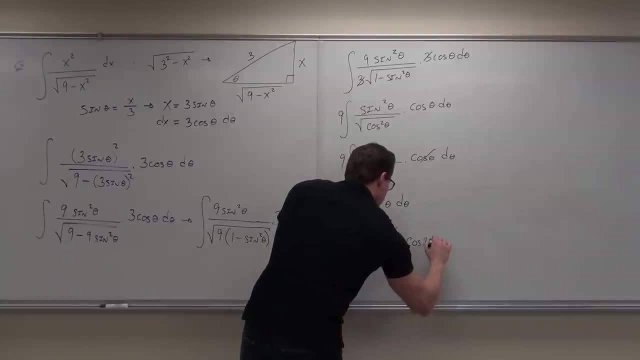 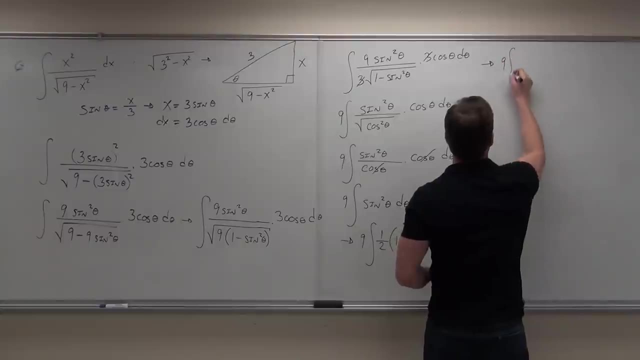 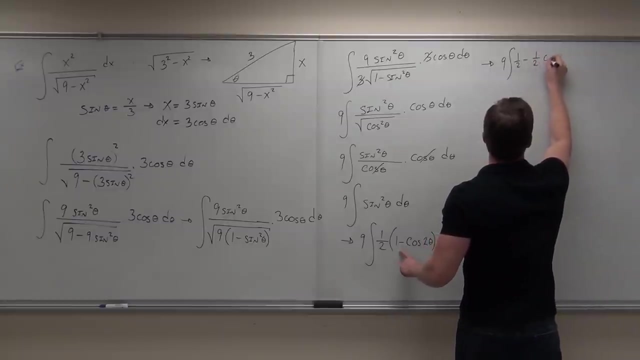 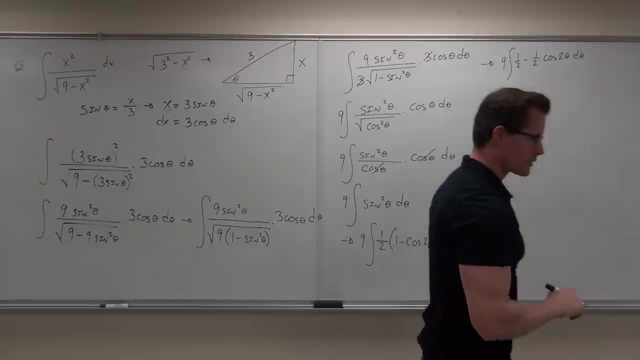 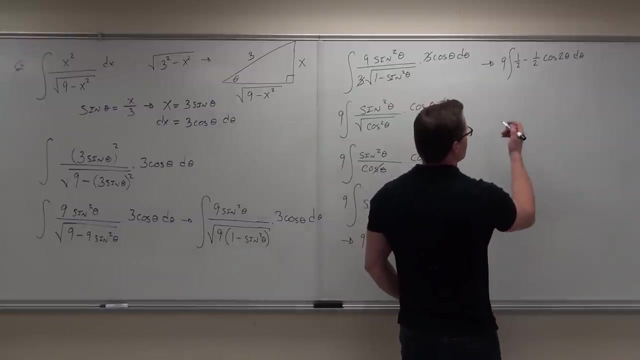 one minus cosine two theta d theta. One half minus one half cosine two theta d theta. Stop me if you see a mistake. I know I'm working kind of quickly here. What else? Pull that one half out, You could. you could pull the one half out. 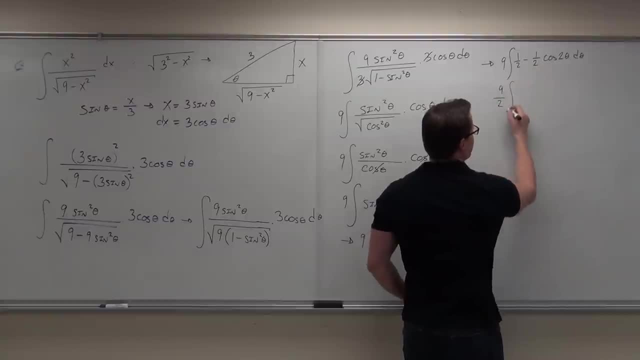 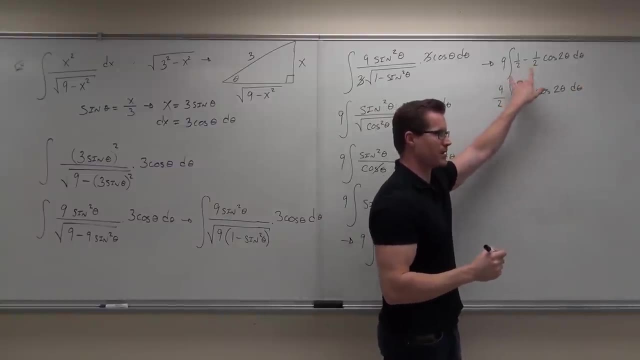 then we're gonna have nine halves if I factor the one half out. one minus cosine two theta d theta. Don't just pull this one half out, though. you'd have to factor to make that happen. Why didn't you do it on the earlier stuff? 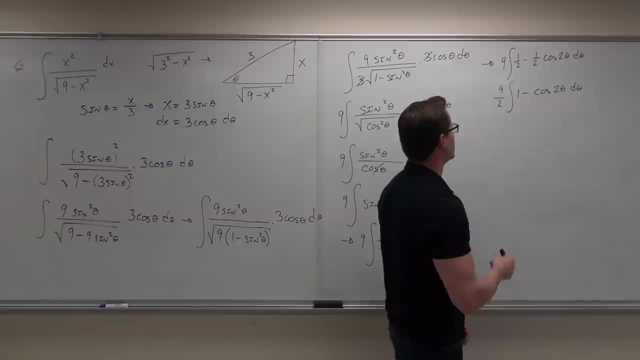 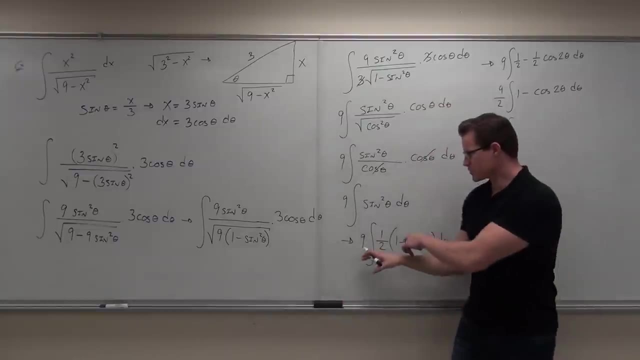 You could've. yeah, you totally could've. I don't know why I didn't. Oh, you're trying not to do it right there? Yeah, you could've done it right here. just pull the one half out. I didn't see that you were right there. 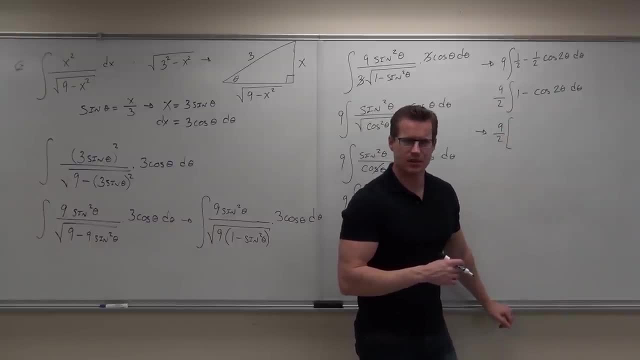 Can you take the integral of one. What is that? It's not x. no, Keep in mind. this is why it's important: Theta, What's the integral of cosine two theta, Theta, One half sine. theta over two times two theta over two. 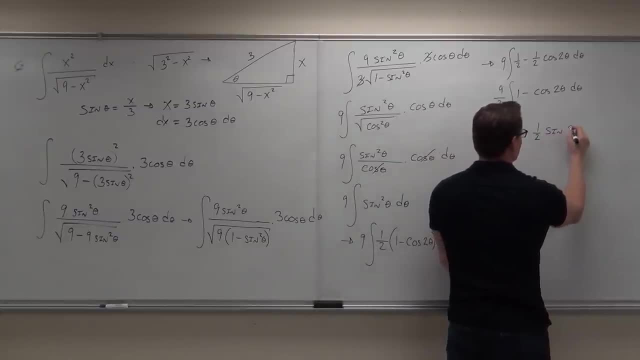 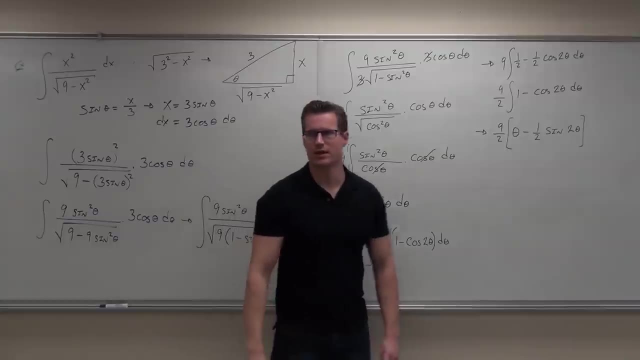 Good. So theta minus one half sine two theta, Are we still okay? Mm-hmm, Okay, we're going a little long today. I'm sorry for that. Do you guys want to finish it right now? Yes, Okay, so well, I bet you do. 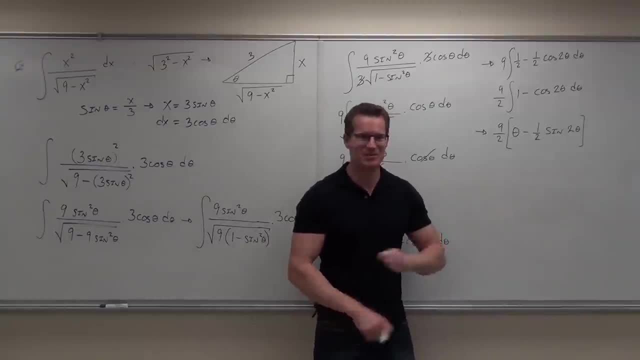 We had no class coming in, so we're good. Whoo, let's go another hour, Okay, No, no, no, no, just joking. We're not doing that. I'm hungry. I'm hungry, I'm wasting away. I lost three pounds in a week. 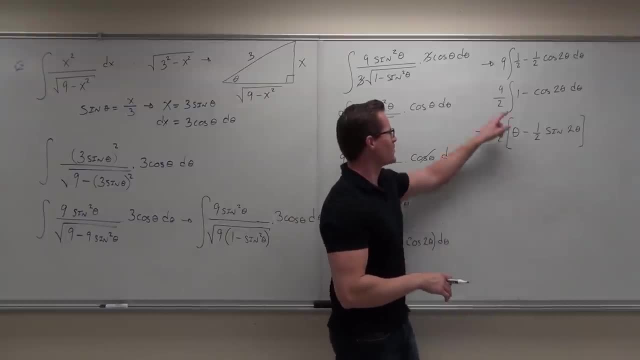 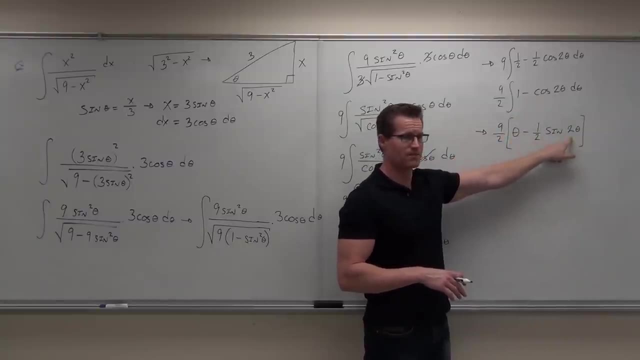 I know a new movie and it's been created. This anyway, this is not important. So, theta, don't you feel sorry for me, I have to do math. and a movie One half sine two, theta, we still all right with that one. 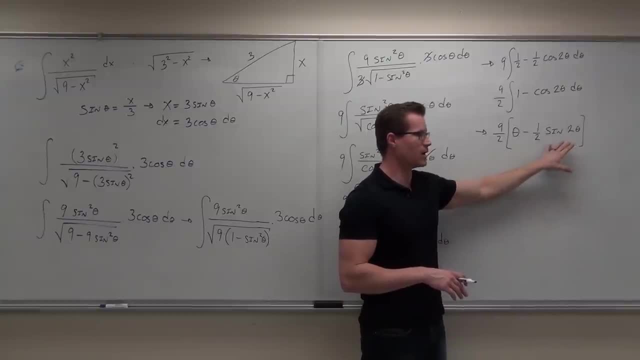 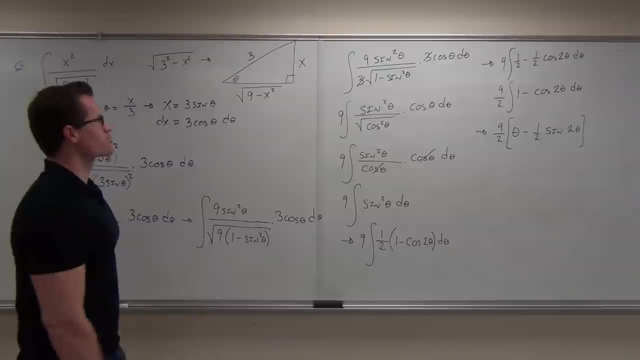 Mm-hmm. Now here's the issue. This is done, calculus is done, But we started with: we have: use your triangle. You're always going to use your triangle. So here we go, Here we go. Let's start with it. 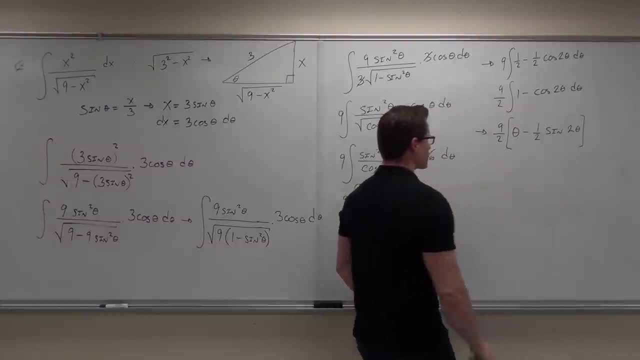 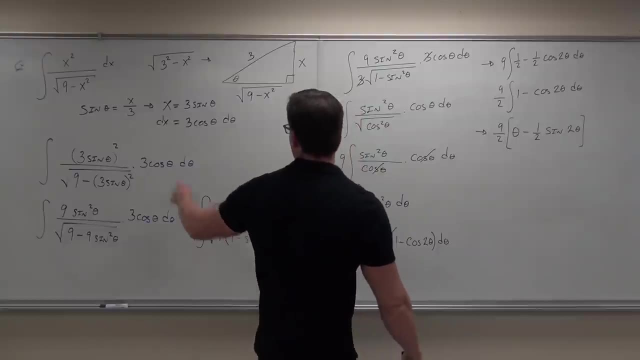 What do we know about this thing? We know it's sine- oh goodness gracious- Theta. it's all for theta. Well, we know that sine theta. let's start with this, okay, Because you can't have any thetas left. 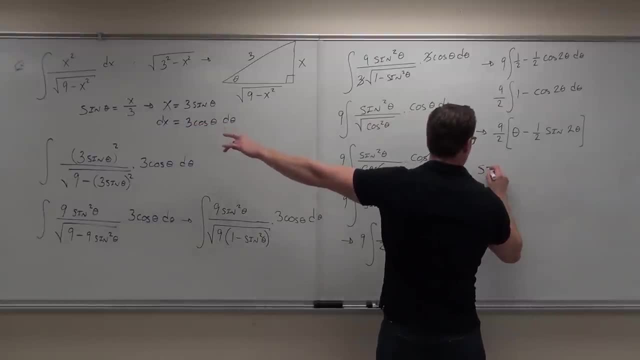 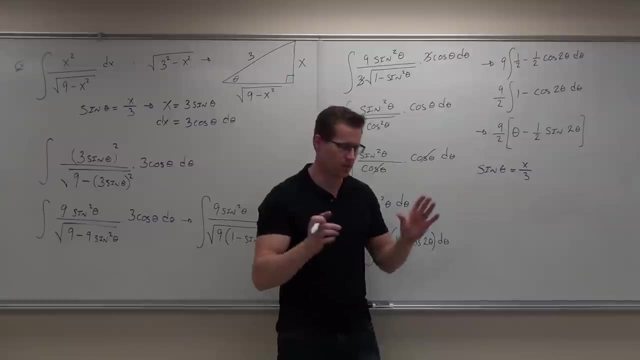 You gotta have all x's. We know that sine theta equals x over three. We know that, Okay. We know that, Don't we? Mm-hmm, Okay, cool, So keep it simple, Use this substitution again. 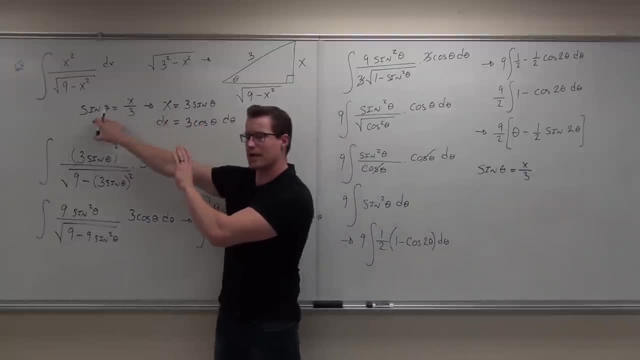 Sine. this is why we write this one. We don't go directly to this one, Because oftentimes we'll have to use this Sine. theta equals x over three, If that's the case, the only way we can solve this. 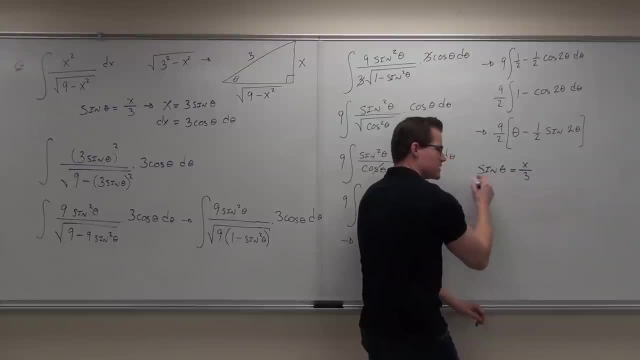 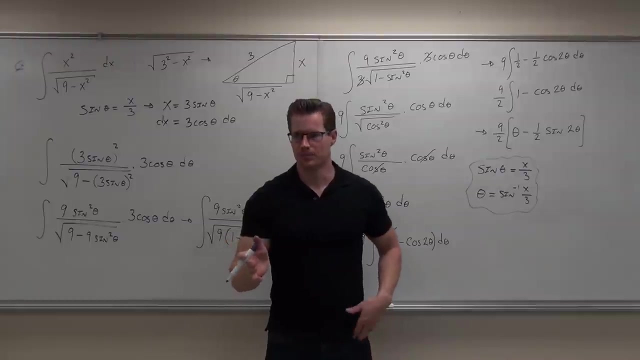 is say: well, let's take a left inverse of sine, on both sides At least. if we do this, sine theta equals x over three, if, and only if, theta equals sine inverse x over three. That's one little piece. Here's the problem, our main problem. 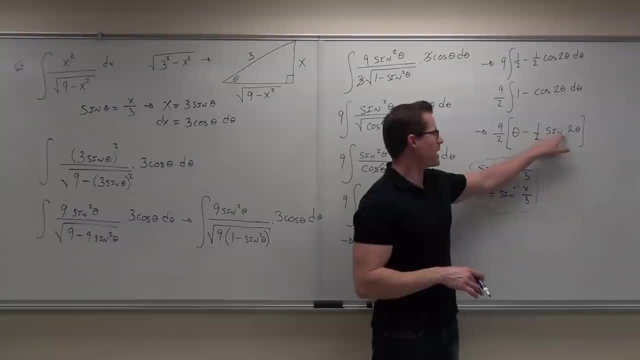 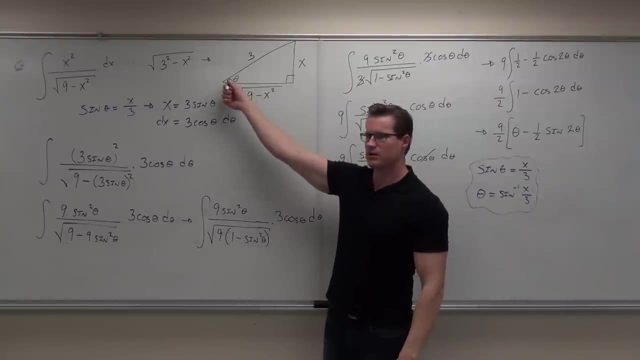 Our main problem is that sine two theta. that's a problem. If I look at sine two theta, is that two theta? No, No, you don't just get to pull out a two or multiply something by two. You actually have to have the actual theta. 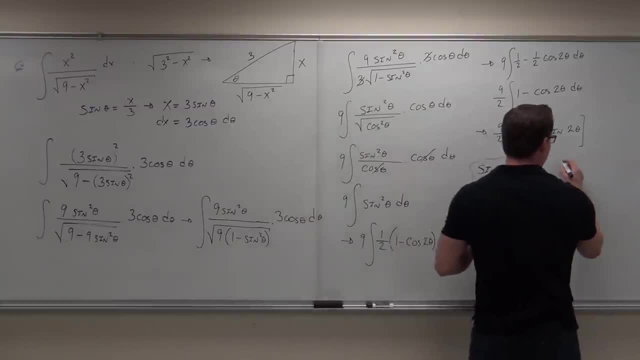 So when we look at sine two theta, we need to know that that is the same thing as two sine theta, cosine theta. So sine two theta, That's a problem. That's cosine theta. Hey, look at that. Do you recognize that identity? 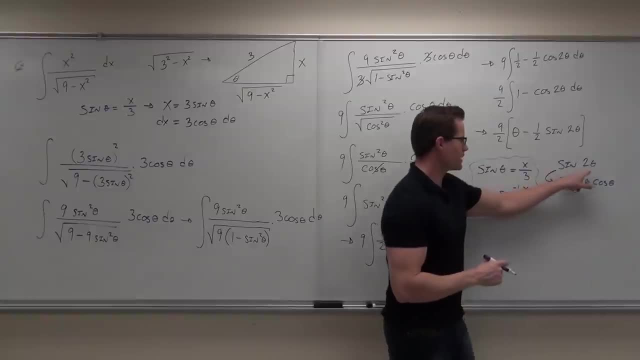 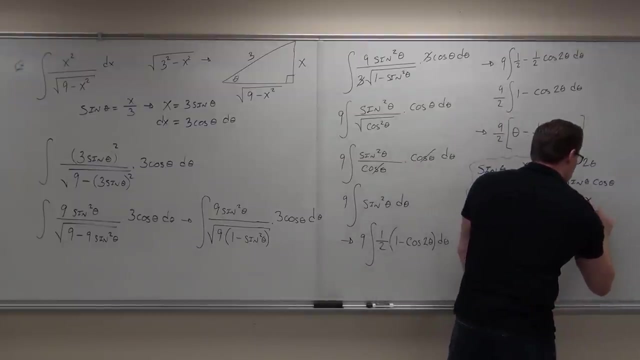 Sine two theta is a double angle, So sine two theta is the same thing as two sine theta. Now, now it becomes easy. Can you do sine theta? We already know that one Sine theta is x over three. Let's do cosine theta. 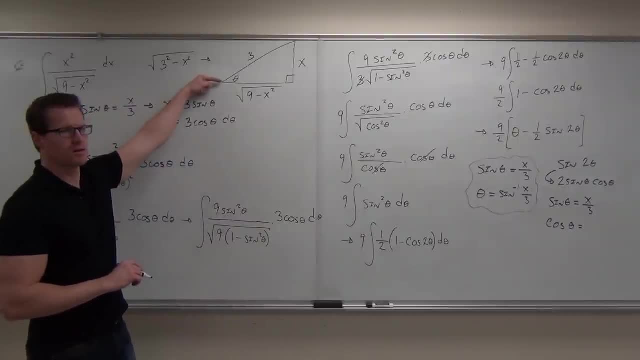 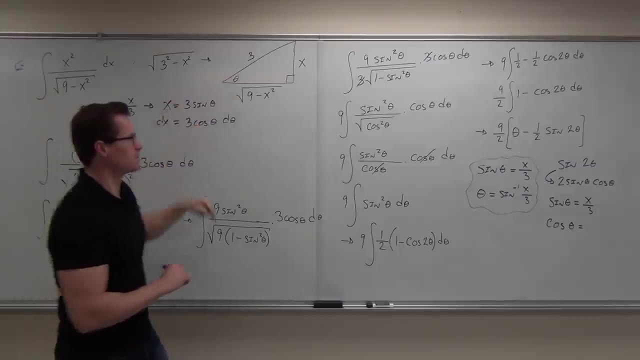 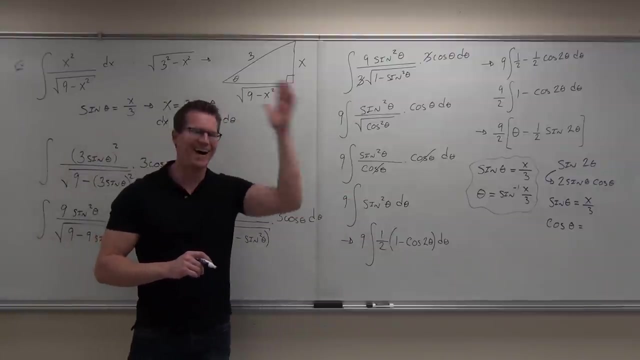 Let's look back at our triangle for cosine theta. How much is cosine Theta Adjacent over hypotenuse? x over nine, nine, nine, So add some catnip: Adjacent over hypotenuse, Adjacent over hypotenuse. 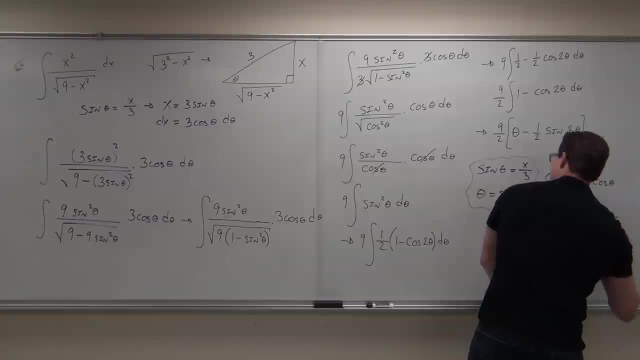 Good luck, guys. It's not that I'm doughy, but it's a good into it. We used to count, I'm sorry. Yes, Okay, I'm going to have to erase this. We're going to move over here. 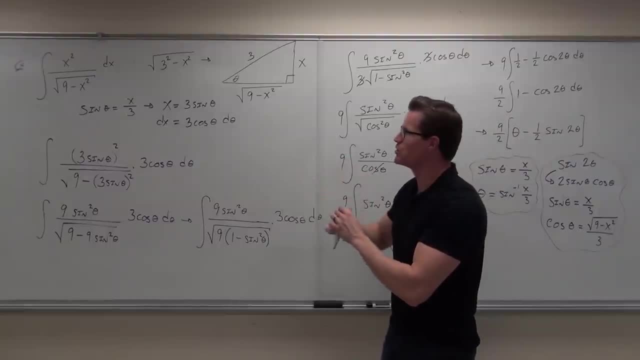 We're almost done, I promise, but I want to make sure that this actually makes sense to you. Are you okay with our triangle substitution for this? That was pretty. this is the easiest part, actually, is this, It's the easy. 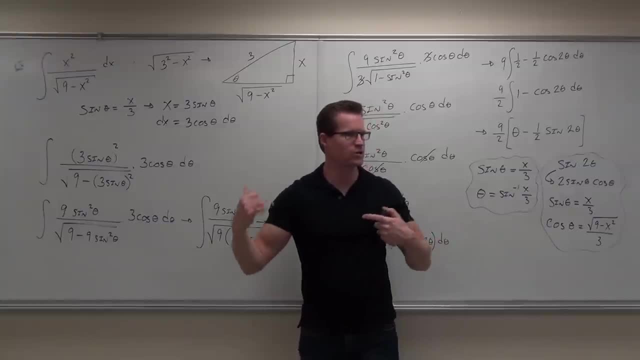 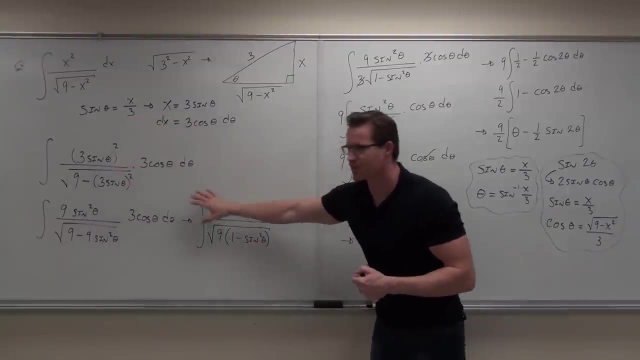 Now that I've taught you how it actually makes sense, you don't have to follow the formula. Hopefully you understand hypotenuse sides. put them in the right relationship, get whatever trig substitution is necessary. Everything's simplification, all of it is simplification. 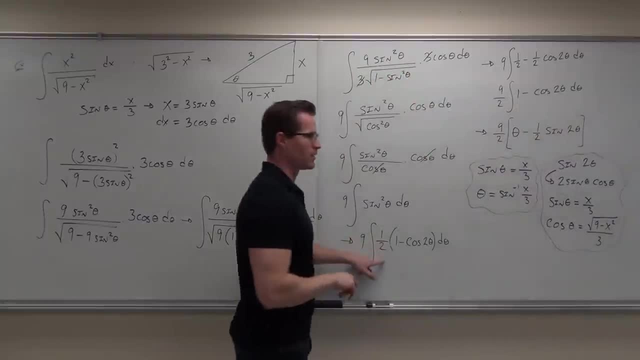 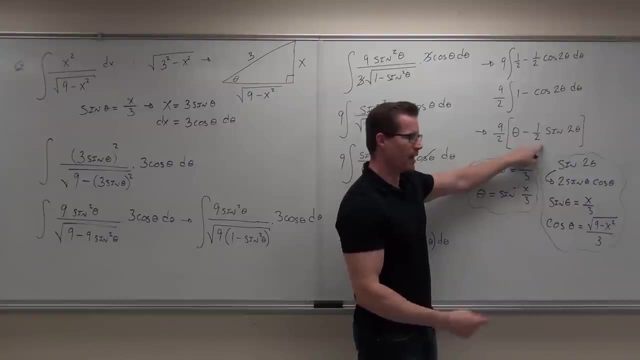 until right here. Then we have a little bit of calculus. You know how to do that already. That's your last section. You get all the way down to here and then you go: ah, junk, Now we've got to substitute back in for any thetas that we see. 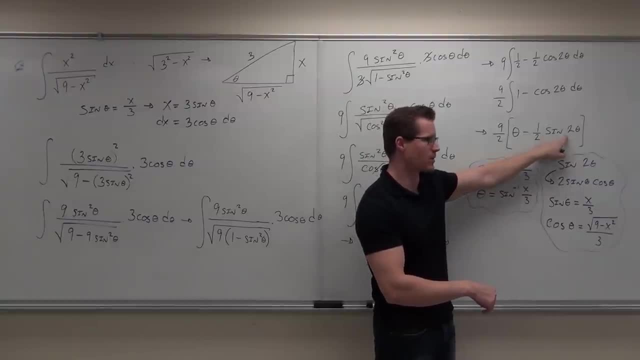 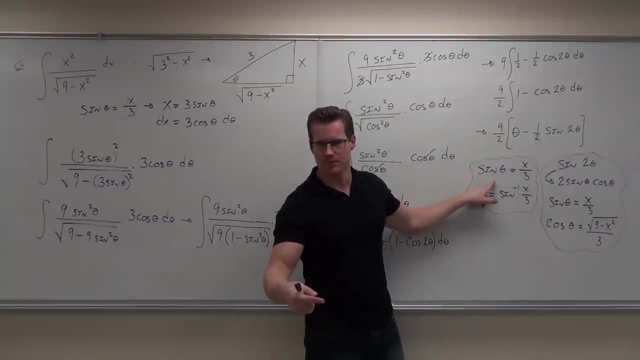 Some of them are easy, Some of them are take some time, okay, So check it out. Theta: whenever you have just a theta, you are going to have an inverse trig function. So if sine theta equals x over 3,, 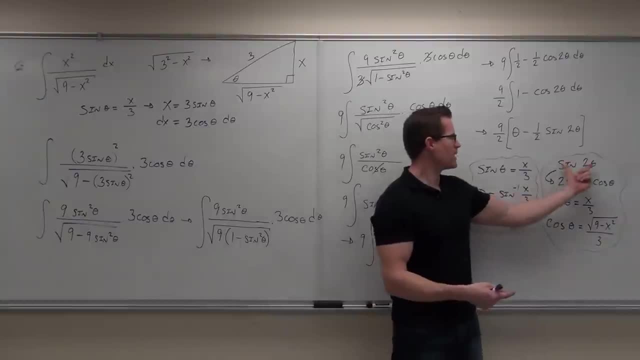 theta is sine inverse of x over 3.. You got it. Sometimes you'll need an identity Sine 2 theta. no, you can't have that. You get 2 sine theta, cosine theta. Well, sine theta would be x over 3.. 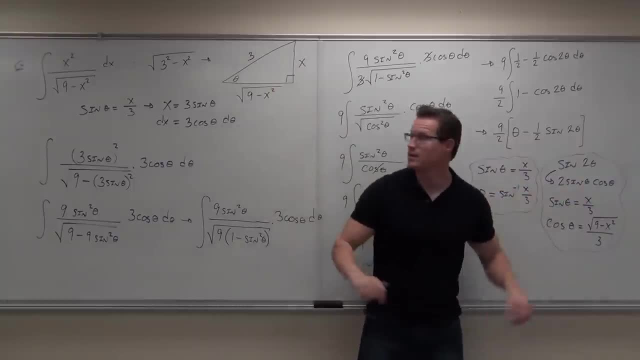 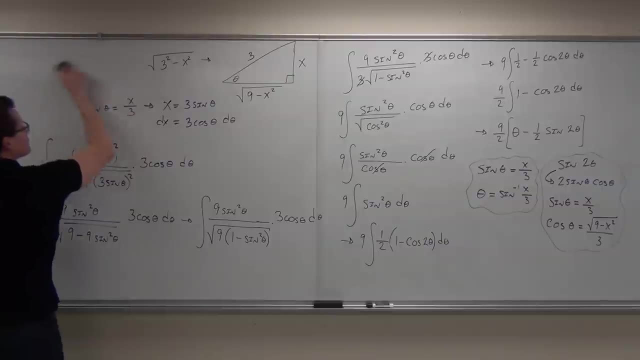 That's one more triangle. Sine is x over 3.. Cosine theta is square root of 9 minus x squared over 3, and now we're going to put everything back together. So Nine halves We've got theta minus one half, sine 2 theta. 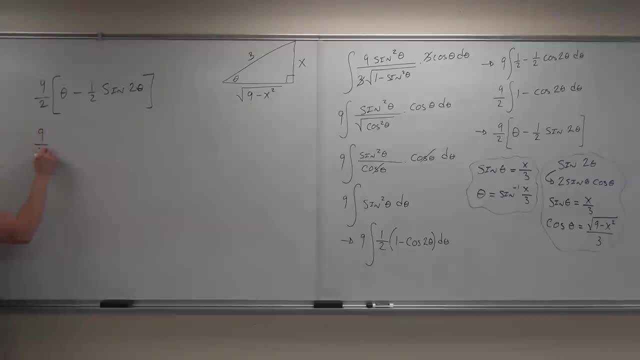 I'm going to draw it out to make it hopefully very clear for you. This is nine halves theta minus one half times 2 sine theta cosine theta by the identity that we just used. So the one half is here. This is 2 sine theta cosine theta. 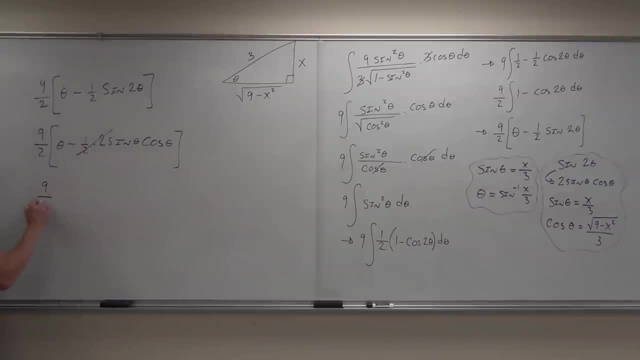 Understood. One half and two are gone, So we get nine halves. Theta is sine theta. Theta is sine theta. Theta is sine theta. So we get sine inverse x over 3 minus sine was x over 3, cosine was square root of 9 minus x squared over 3.. 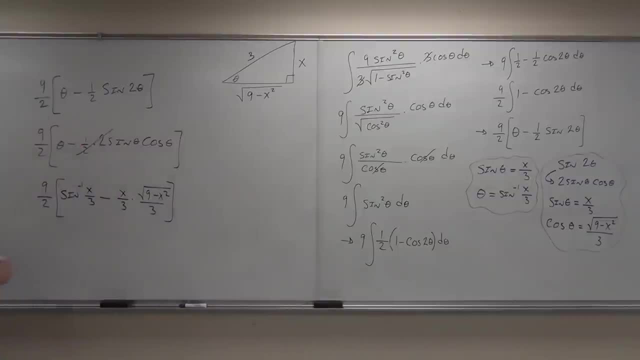 We'll make it just a little bit nicer. looking here. You could factor out a one ninth, but don't do it with this 3, because that's part of your angle now. You can't change that. So Sorry, not angle. 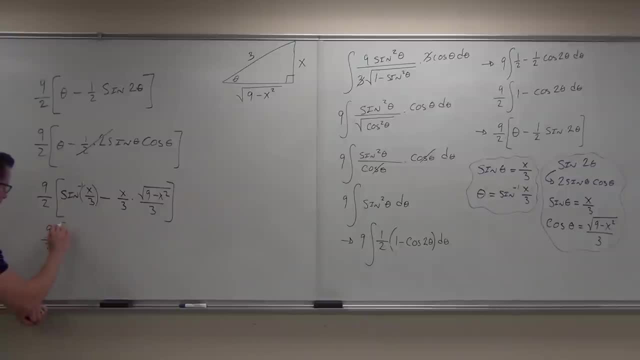 That's a relationship. So nine halves. We have sine inverse x over 3 minus x times the square root of 9 minus x squared over 9.. And then finally, plus C. Oh my goodness, Yay, Is the triangle the hard part. 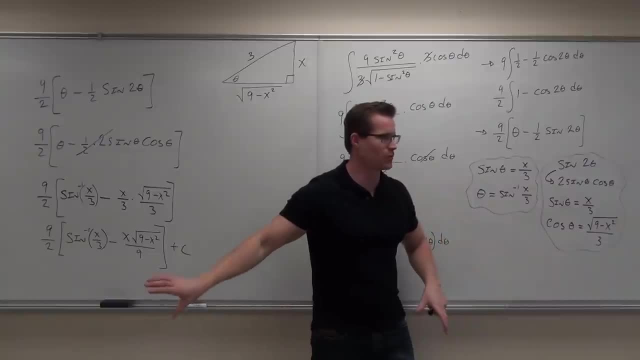 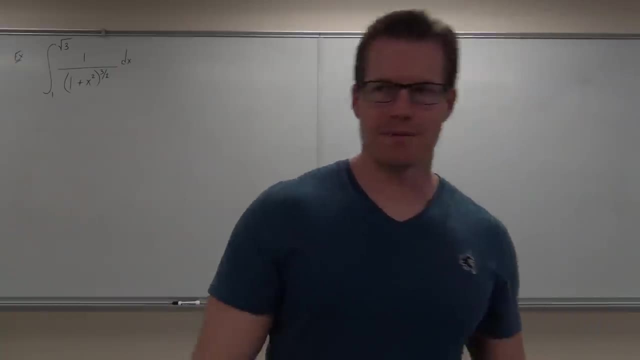 No, No. It's all of this junk that hopefully afterwards I need to show fancy. Do you feel okay with what we've just done? Fantastic, All right. Three more examples and we're done with section 7.3.. Again, we're going through some of these, these integrals. 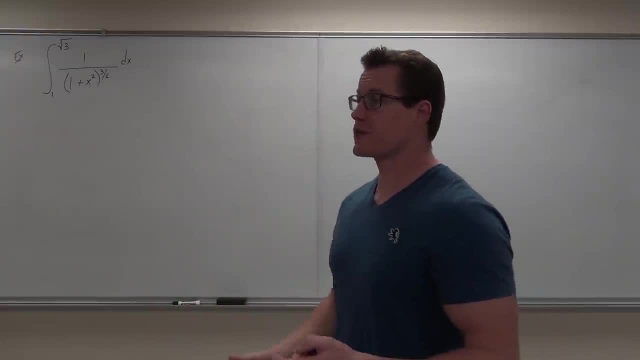 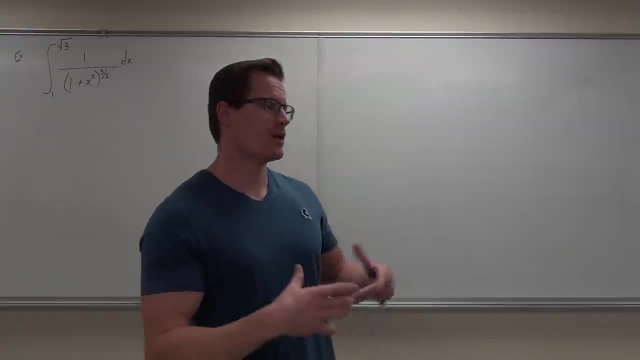 that we can't otherwise do without this thing called trigonometric substitution. So the idea is: look for a square root in your problem. Sometimes you will have to create a square root in your problem If you look for a square root in your problem. 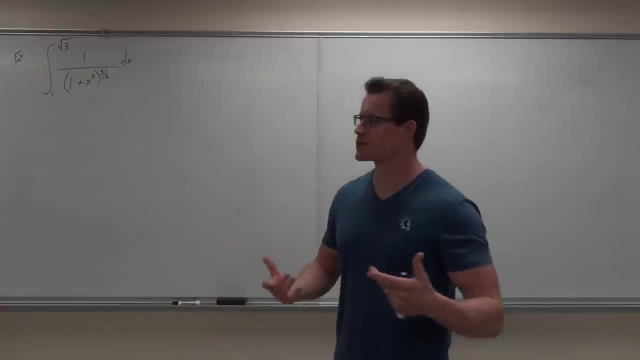 that fits the Pythagorean theorem of a right triangle. we could do the substitution, So let's take a look at this one. This one's not going to take us too long. I just want you to see a couple of other techniques that we're going to use here. 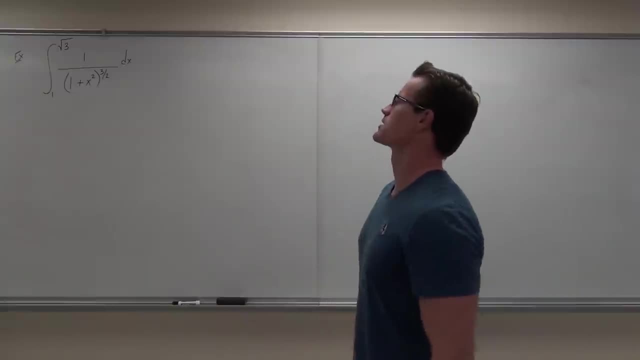 So integral from 1 to the square root of 3, of 1 over 1 plus x squared to the 3 halves. Do we have a square root in this problem? Yeah, It might be a good idea to write it like that. 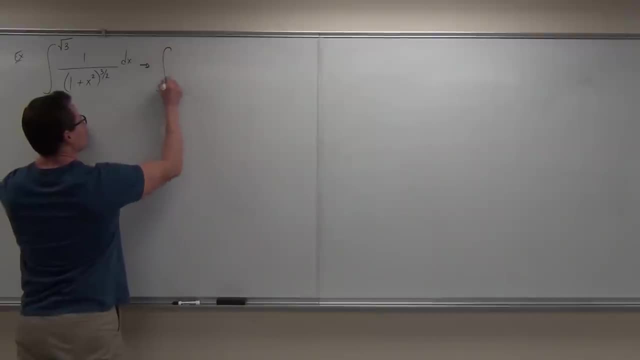 So, instead of just like this, just take a second and rewrite it so that we have that square root. So, instead of 3 halves, what does that 3 halves actually mean To the cube Square root of the third power Square? Okay, 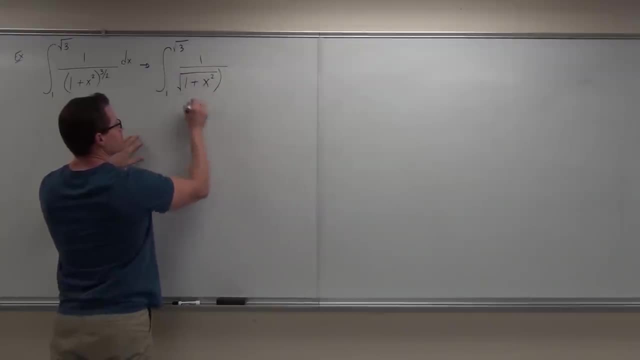 So I'm going to have a square root like this, And then what I'm going to do is I'm going to have that 3 outside. You should know from your algebra that you can have the 3, the power 3, inside or outside. 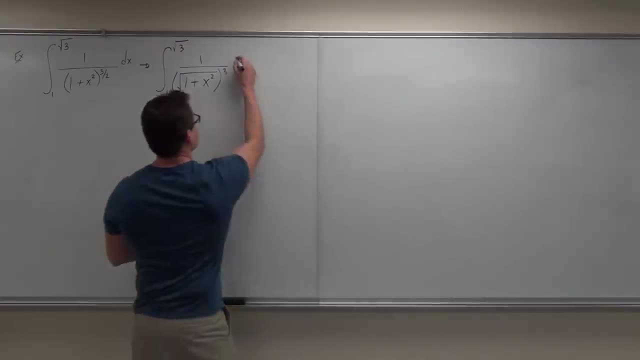 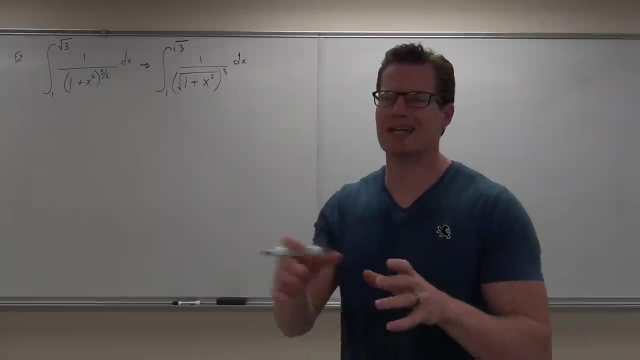 We're going to choose the outside. That way, our substitution is actually possible. You guys okay with that so far. Now we should be to the point where you can make up your own triangle here. So give me the idea. Let's walk through this one. 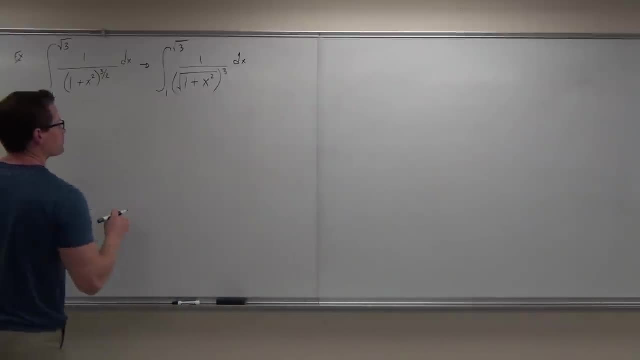 I'll have you do the next one on your own. What's the idea? What are we trying to do? So we want to find the legs? Okay, So we want the legs And the hypotenuse. Let's look here. 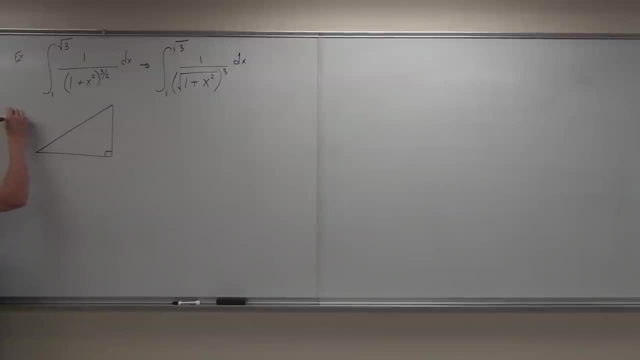 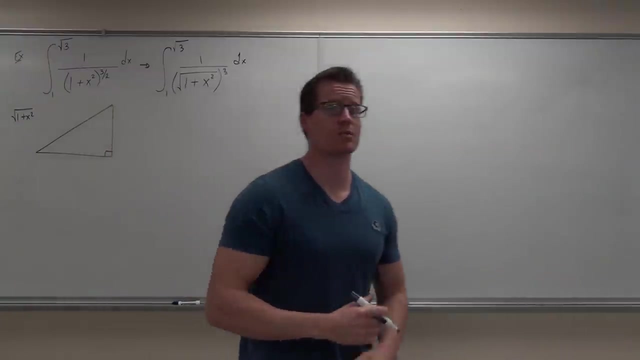 We get the square root And what I'll do is I'll have a square root of 1 plus x squared. That's going to give me something here. So we're trying to make the square root of 1 plus x squared be either one of the sides. 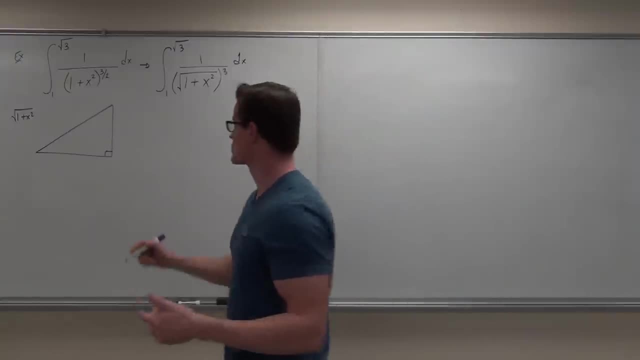 one of the legs, or the hypotenuse. Now, one thing I'll always do is I'll try to write whatever this number is as a square. That way it gives me the side of one of the legs of the legs. So instead of 1, I know it seems a little bit trivial, but I'll put 1 squared. 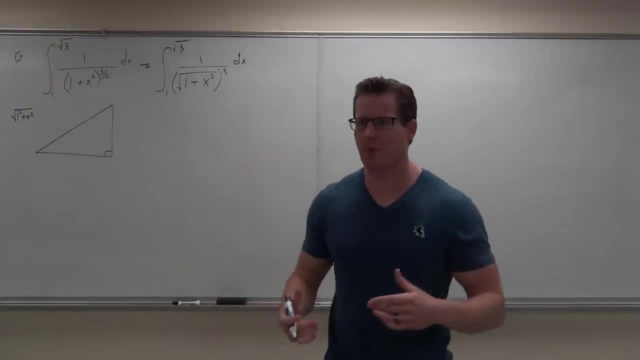 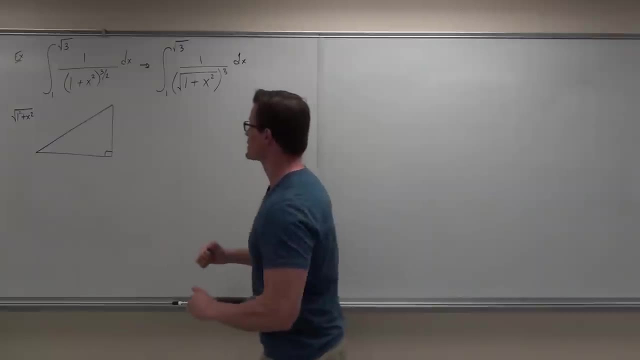 If it was like 4, I'd put 2 squared 16, I'd put 4 squared. That way, I'm not accidentally putting the wrong number on one of my legs. Does that make sense to you all? Okay, So let's think about it. 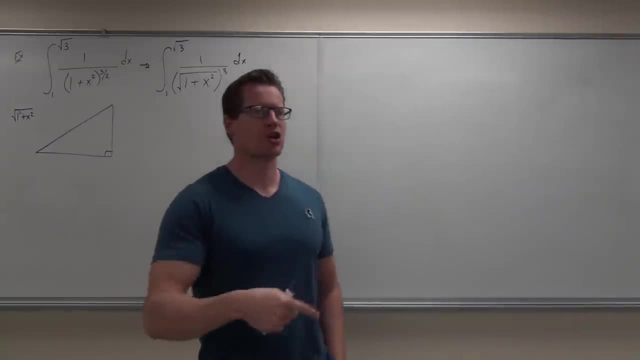 We've got the square root of 1 squared plus x squared. You guys should know right now what that is, whether that's a hypotenuse or the length of a leg. What do you think that's going to be A hypotenuse? 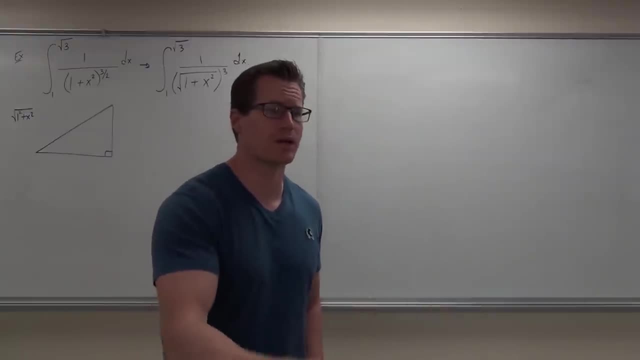 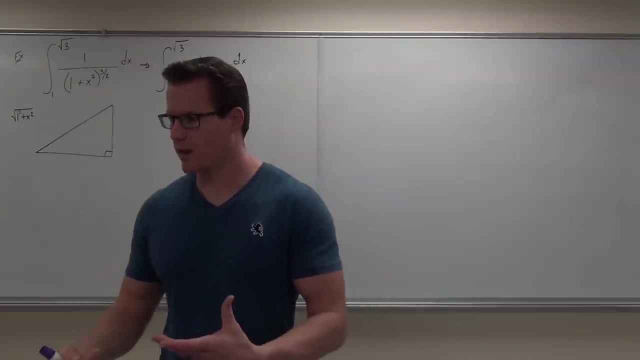 How do you know automatically what it is? A plus? Okay, If it's got a plus there, it's got to be the hypotenuse, Not because it's a formula, but because we understand what the Pythagorean theorem is. 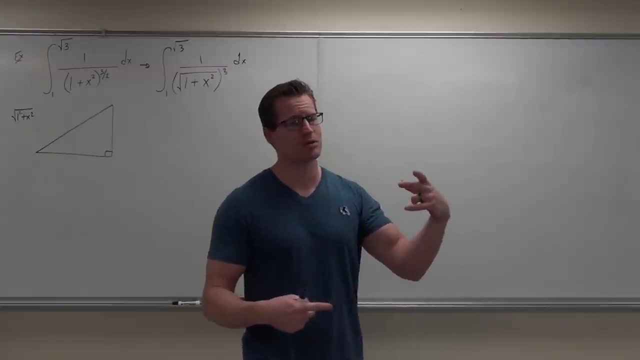 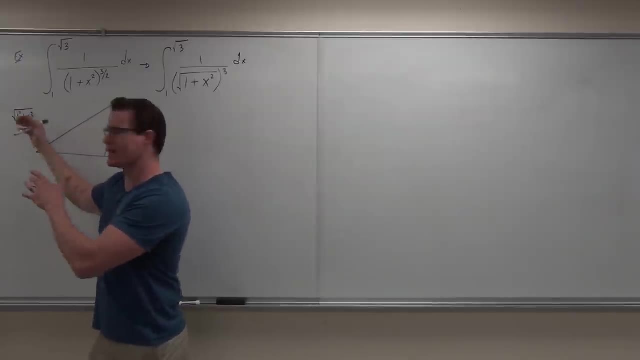 The Pythagorean theorem says that the length of a hypotenuse is 1 leg squared plus another leg squared, and then you take the square root of it. So there's no way that can be a leg. This has to be the length of the hypotenuse. 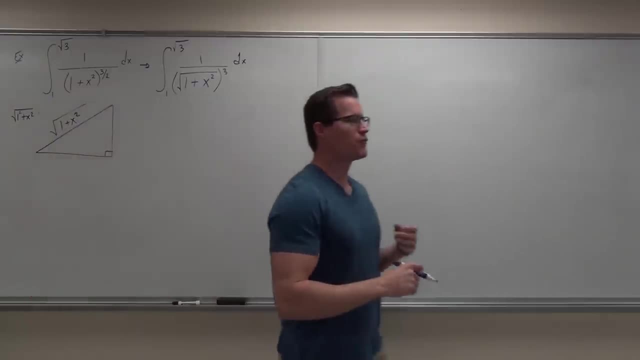 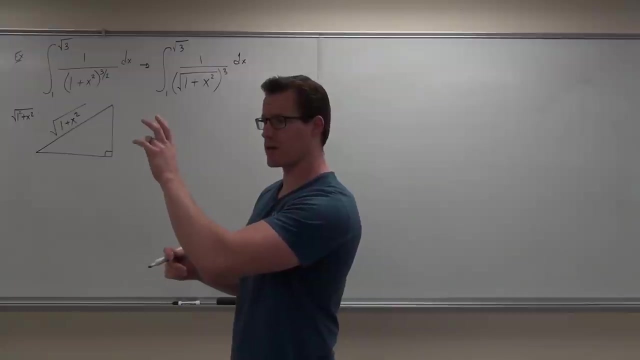 Does that make sense to you? If we have a minus, well, that's the other case. Pythagorean theorem says: for the length of a leg you're taking the hypotenuse squared minus another leg. So what we know is: if we had a minus, 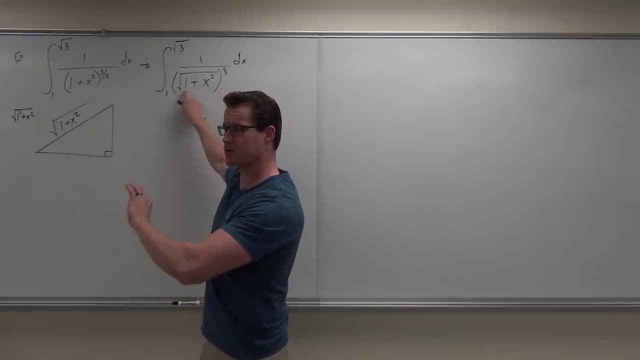 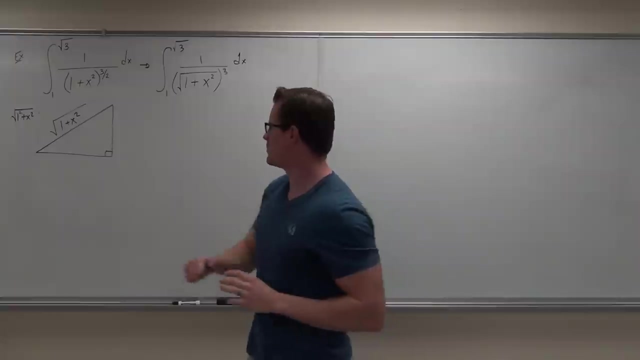 right here. this would give us the length of the hypotenuse and this would give us the length of the other leg. This would be the length of the last leg itself. So let's go through this. How much do you know about what trigonometric identity to make? 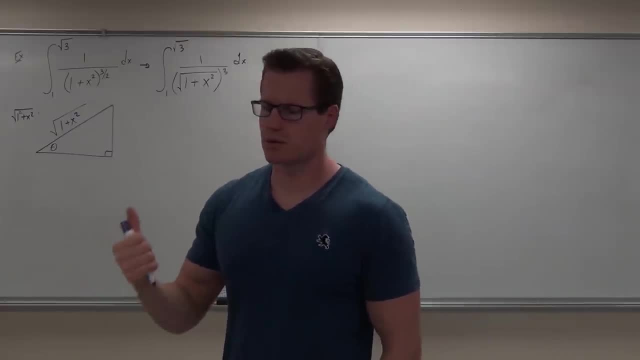 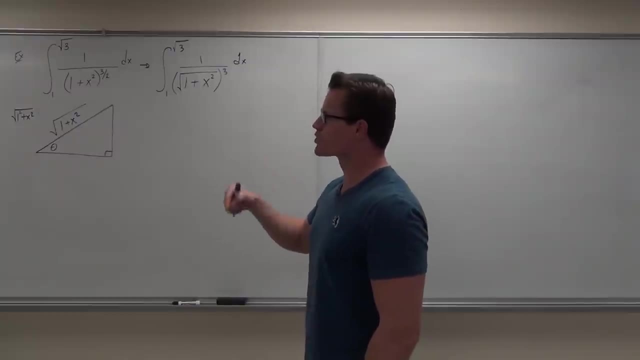 Which three do we always use? Tangent, Tangent, Tangent, Tangent. Good, Those are only three, because those are identities that work well for this. Now, what we're trying to get out of this is x over a constant. 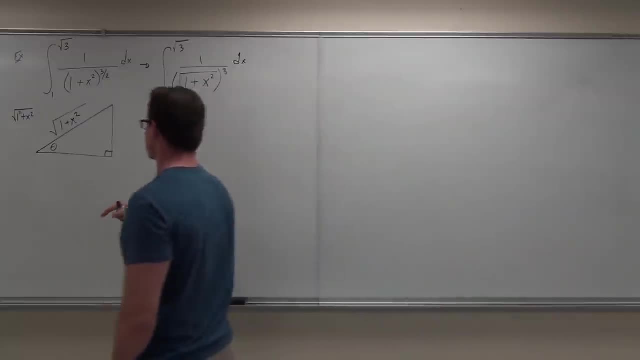 X over a is what we say, So we've got to use either tangent or sine or secant to make this happen. In that case, we're going to pick x for here and 1 for here. So we look at the length of our sides. 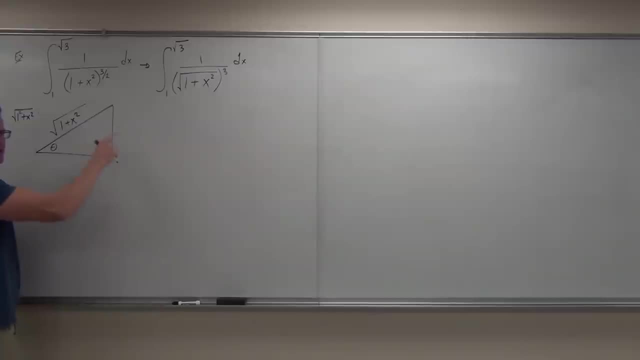 We've got x and we've got 1,, x and 1.. Where's the x going to go Here? Option 1, option 2? Option 1.. Option 2.. Oh, try it, We'll put x here. 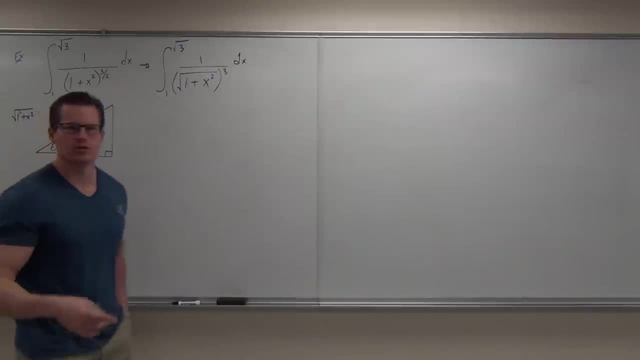 Oh wait, no option 1.. If I put x, well, let's think about why. though Don't just fall into the pattern and look at the formulas. I hate that. I don't want you to memorize all of them. 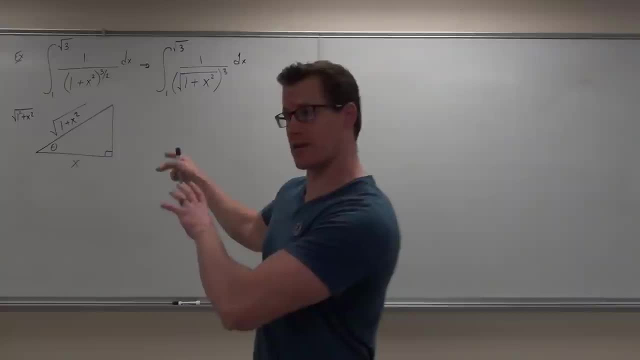 All the formulas? okay, because what if you forget a formula? That sucks? If you understand the triangle, it will make this easier. Let's look at this. Firstly, do you all understand why this has to be the hypotenuse, yes or no? 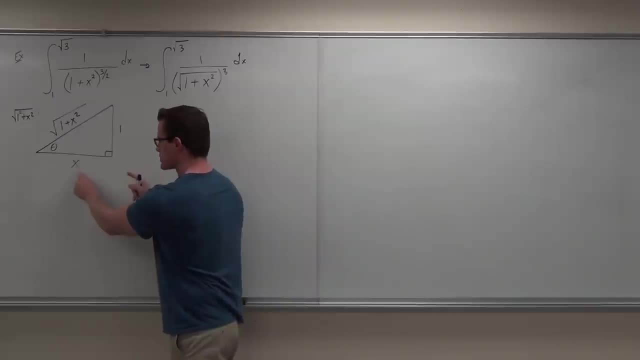 Okay, if that's the case, either this is 1 and this is x, or this is 1 and this is x. If I have this, is there any way in the world I'm going to want to use sine or secant on this triangle right now? 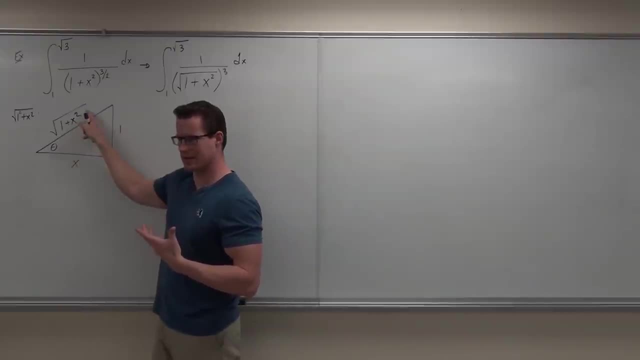 Sine, Sine, I'd have this. I'm trying to get rid of that. That's the whole idea. I don't want to talk about that. How about? how about secant? I'd have this. I don't want to use that either. 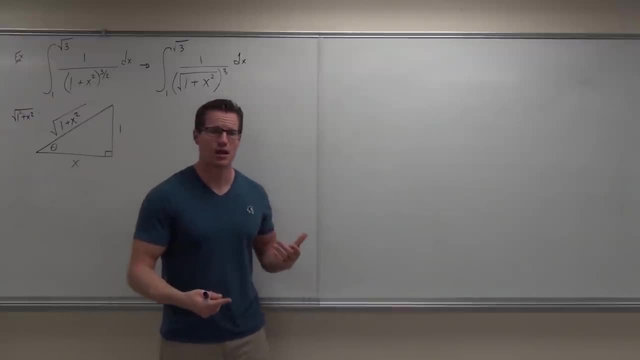 I want to relate the easiest two sides, the x and the constant. but I want to do it in such a way that I get x over the number, not the number over x. So is this going to work for us? No, Tangent would give us 1 over x, but well, let's make it nicer. 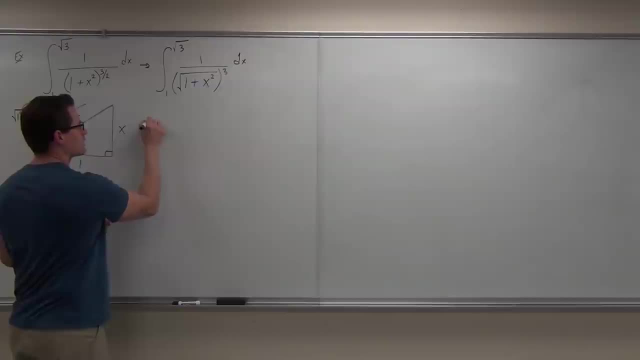 Let's put x here and 1 here. Now, if I take tan theta, I get x over 1, which means that x equals tan theta Typically. what we'll do is remove our constant over here, since it's 1,, no big deal. 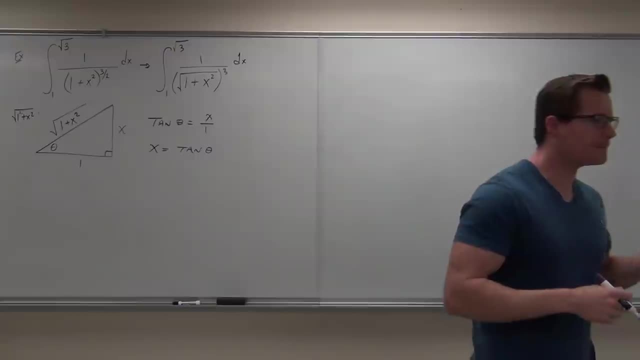 Okay, keep on going. What now? We've got x equals tan theta. What's the next idea Before we plug it in? because we have two things that we're going to be doing here. What else are we going to do? 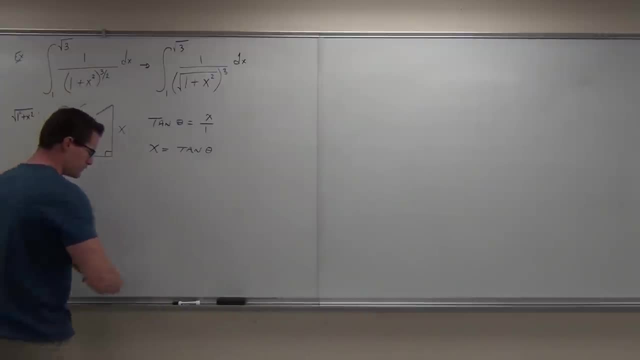 Say what? Let's do that If we take the derivative. you see, when we do this, we're going to be changing this into some sort of a function involving theta, but we also need to change our dx into some d theta. 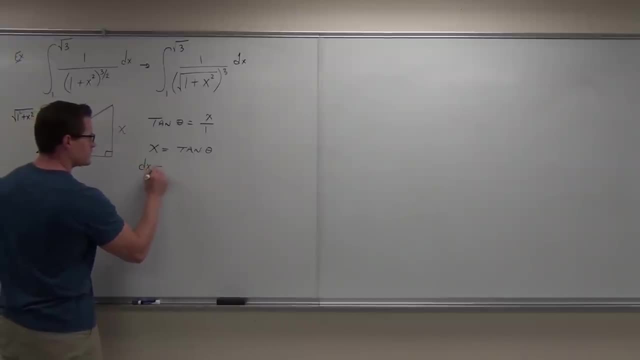 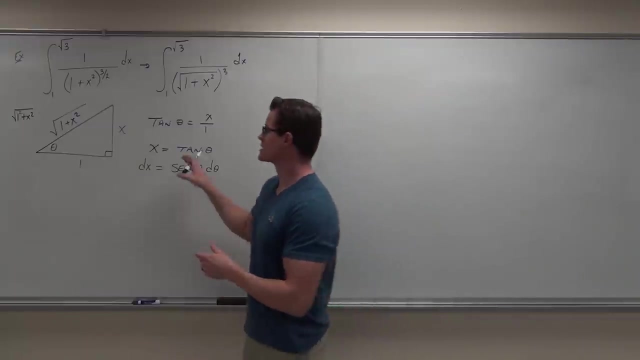 So, in order to do that, we take our derivative. we get dx equals. oh, everybody, tangent d theta, d theta. Perfect Guys. so far, we're so good. Go ahead and make the substitution, Let's see. you guys do it. 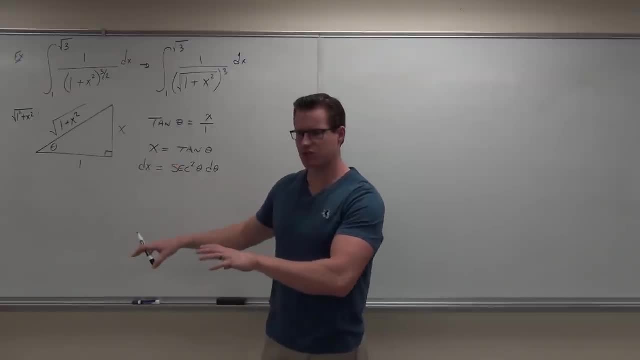 Go from here, plug in what you need to plug in. I'll do the same thing on the board. I just want to make sure you can do it on your own, okay, So go, I'll give you about 10 seconds. 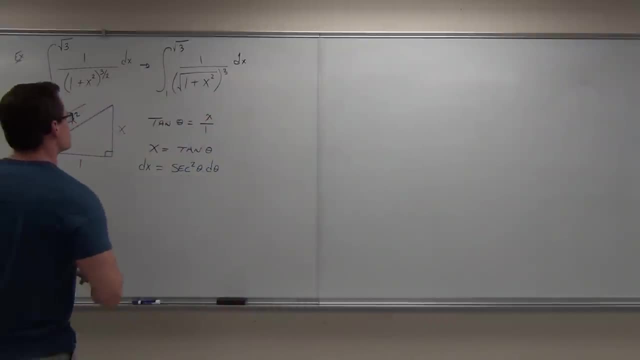 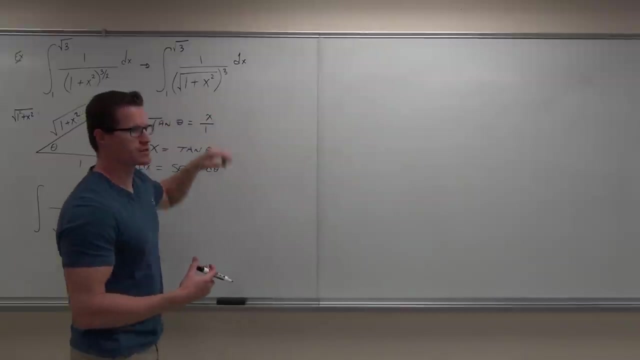 then I'll put it on the board. Make your substitution Notice. when you're doing trigonometric substitution, the square root, it's never going to change. The idea is that we're changing just this variable x because when we square it, when we square whatever, 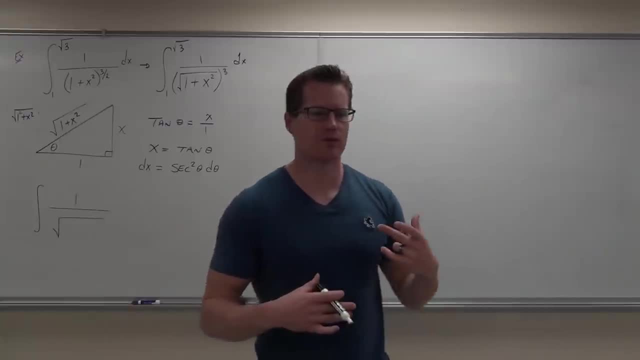 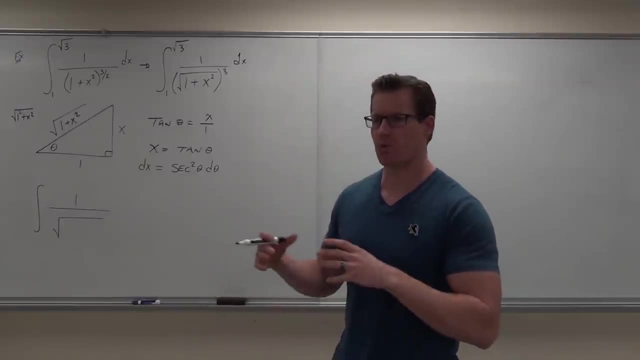 that variable is of the substitution. we're going to get some sort of 1 plus or constant plus that we're going to be able to make an identity out of like 1 plus sine squared or 1 plus tangent squared or 1, one of those things. 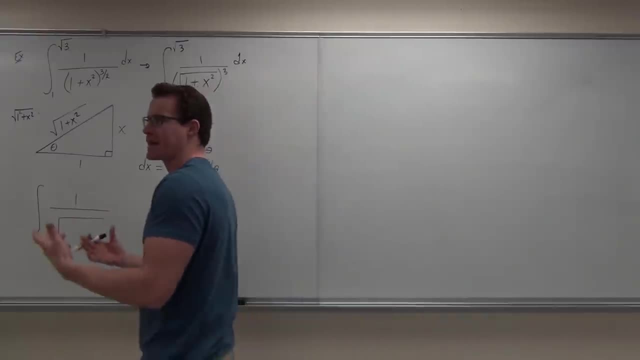 actually it's 1 minus sine squared, sorry, or 1 plus tangent squared. that automatically fits one of the identities that we have in hand. So does the 1 change? No, No, And the plus doesn't change. What's the x become? 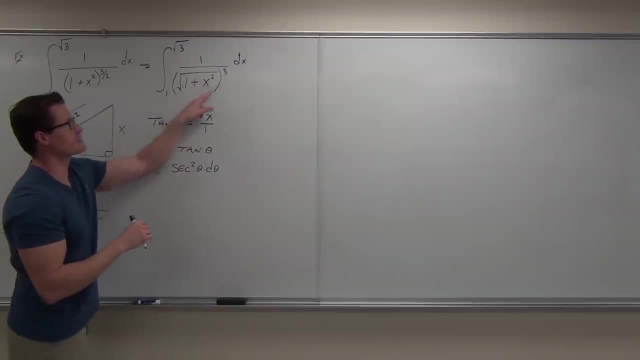 Tangent squared theta- Good. So if the x is tangent, then this is tangent squared theta- Very good, And we still have that power of 3.. Let's make sure we're not losing anything. Now the reason why we did our derivative right here. 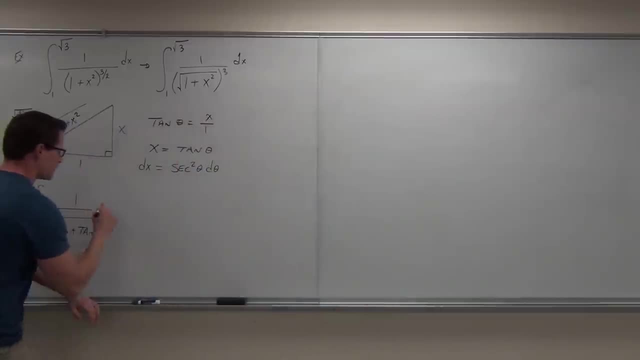 so we can also substitute for our dx. What's our dx become? Let's make sure. Do we have all thetas and a d theta Looks like it. We're pretty good to go. There's one thing I haven't done yet. 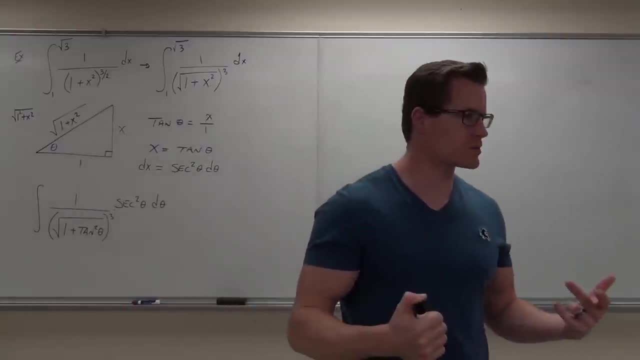 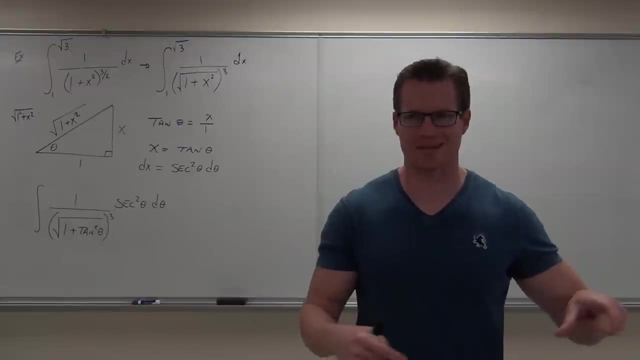 and this is kind of up to you. I like doing this. Some people don't. Some people like to wait to the very end. I like changing bounds. I like to, because sometimes I'll forget to re-plug in my substitution. That kind of sucks. 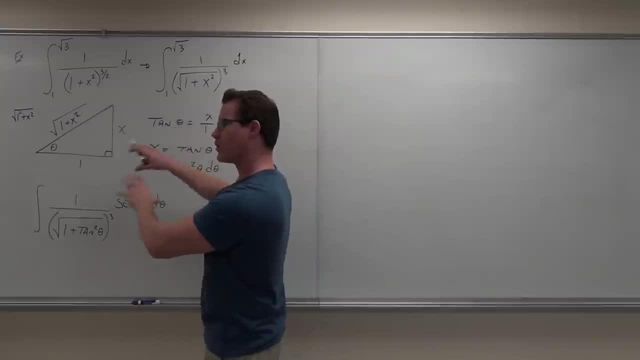 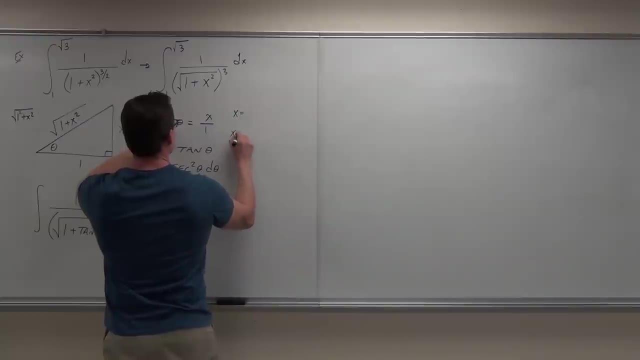 So right now I'm going to go ahead and change bounds. We do that at this step. We don't want to wait until later. Do it right now when you're doing your substitutions. So right up here we have x equals square root of 3 and 1.. 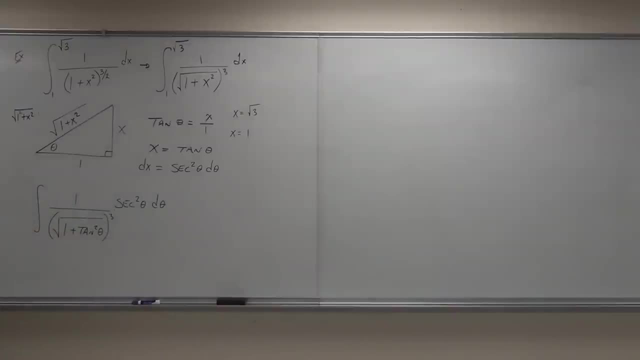 Write that down. So if that's the case, if x equals the square root of 3, then what we would get is tan theta equals square root 3 and tan theta equals 1.. Please note, I'm doing this on purpose. 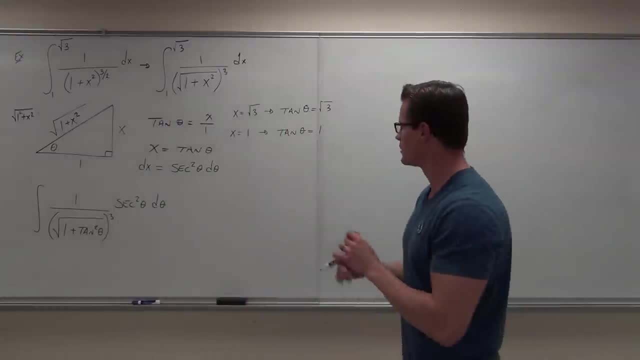 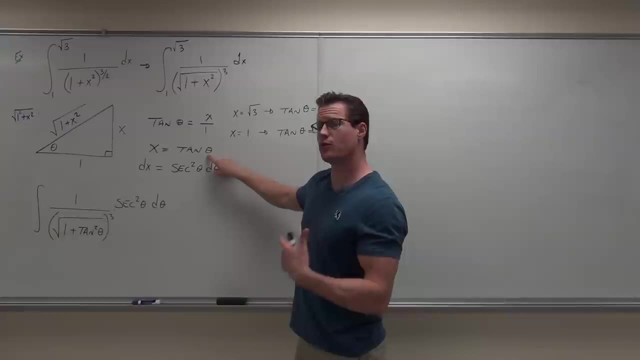 I want to make sure that you guys see how to actually change the bounds in this scenario. If you have, x equals the square root of 3, look at where the x is. X is not theta. What we're trying to do is solve for theta. 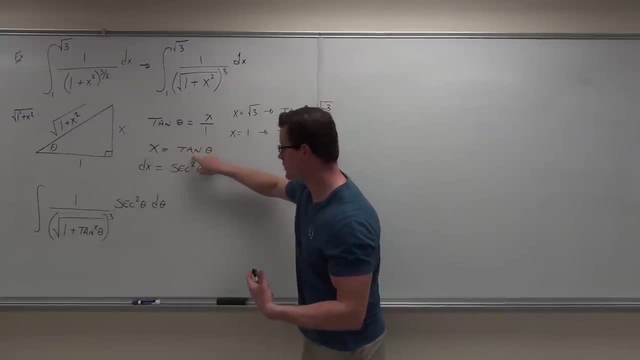 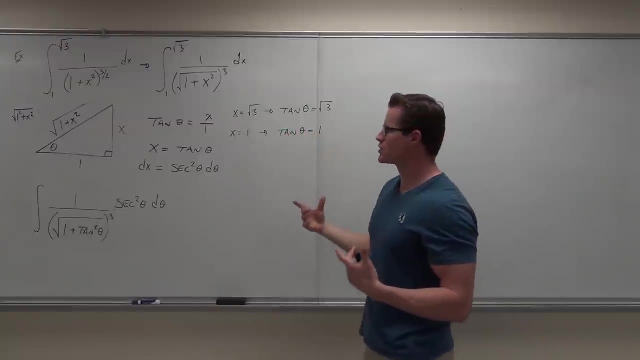 Does that make sense to you? So we have the square root of 3 equals tan theta. We would have 1 equals tan theta. You guys follow this idea. Well, now what we're going to try to do is put our integral. 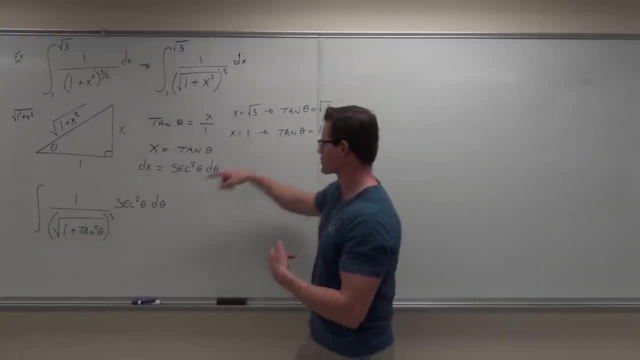 in terms of theta, not tan theta. We don't want 1 and square root of 3. here again, What we're going to have to do is use an inverse tangent to figure out what that is. So basically it says: okay, cool. 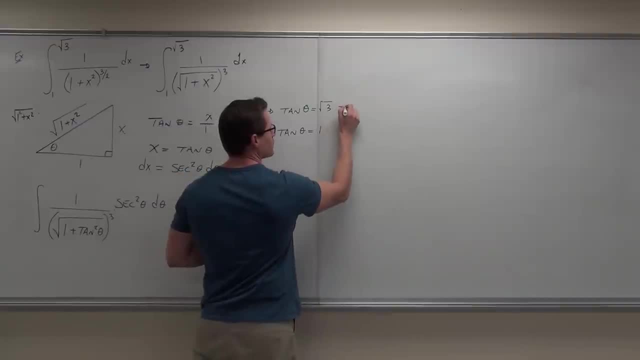 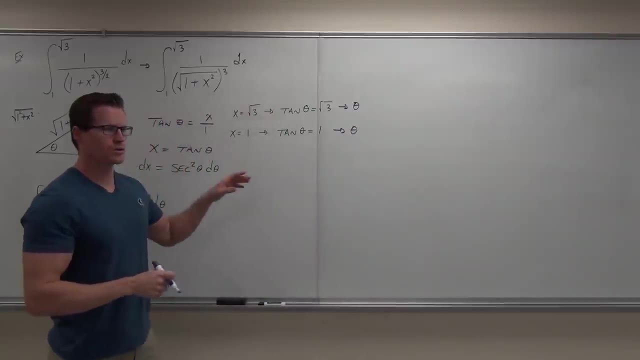 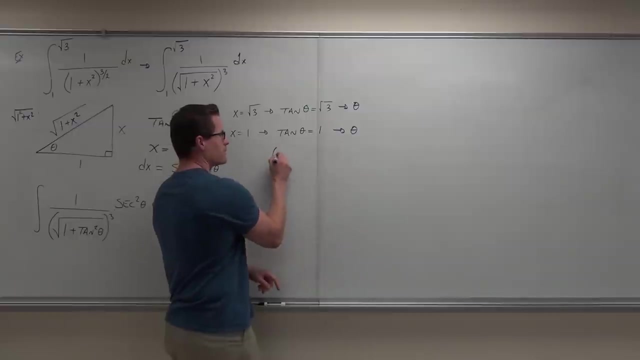 I'm glad you got this. Now go one step further. Figure out how much theta is, So recall I'll do this on one of them. Have I lost you? I don't want to lose you yet. Recall that this is true if, and only if, this is true. 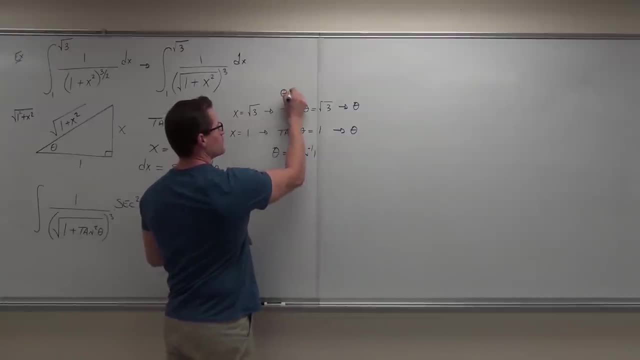 Do you remember doing that? This is true if, and only if, this is true. So basically, it's asking: A: what angle does it take For tangent of that angle to equal 1?? And same thing here: What angle does it take for tangent? 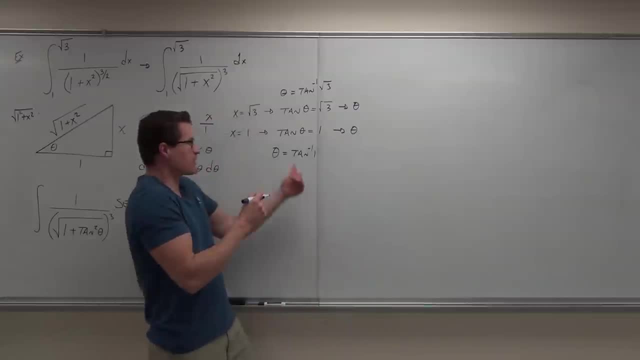 of that angle to equal the square root of 3? Do you guys know what it is Or can you think of the inverse? What's tan inverse of the square root of 3?? What's tan inverse of 1? Pi over 3 and pi over 2.. 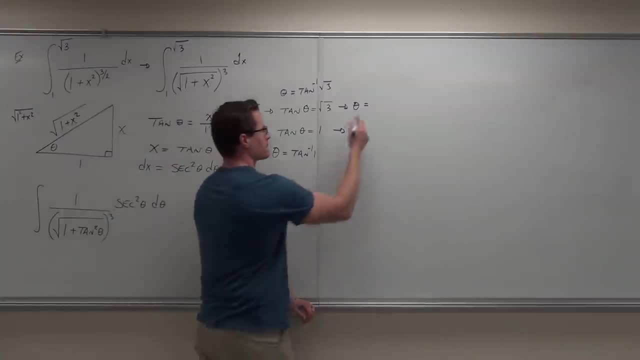 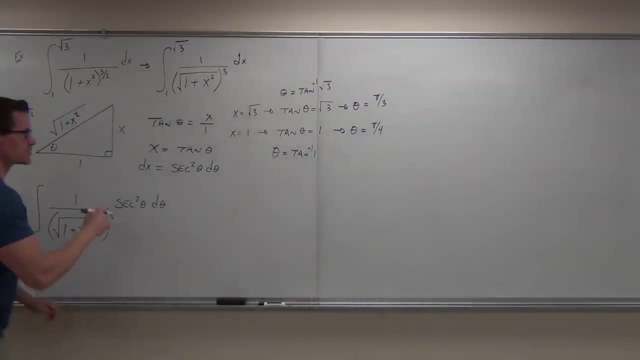 Pi over 3 and pi over 4 and 4.. And pi over 4, yeah, That's a nice order for us too. So this becomes pi over 4.. This becomes pi over 3.. Let's make sure that you guys all have this. 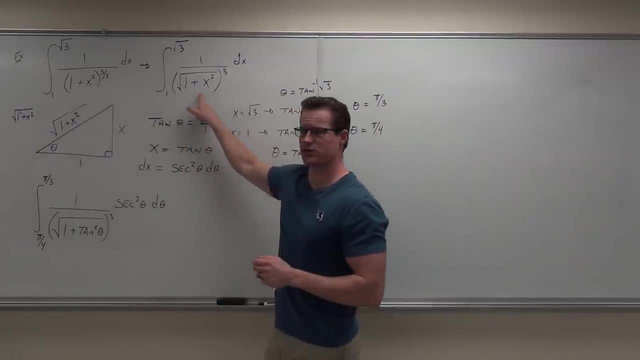 Are you okay on writing this as a square root to the third power, Yes or no? Yes, You guys are dead today. huh, My goodness, I know it's Monday, but geez, More activity. I'm excited about this stuff. 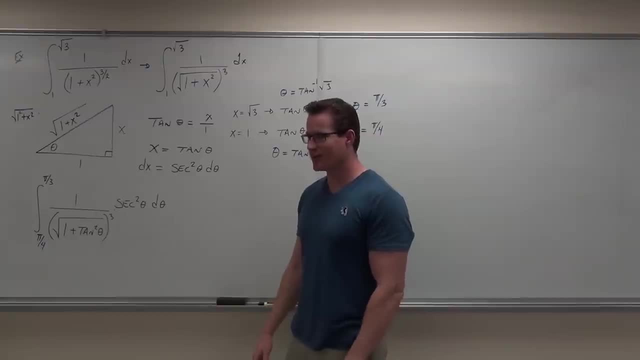 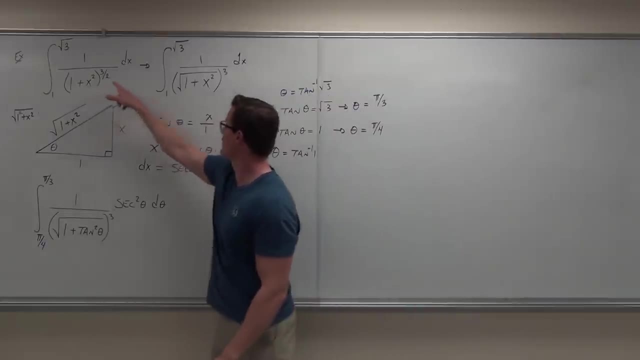 You should be too. Goodness gracious. This is fun, I guess. Come on, people, You're talking about math Jedis already, Geez Okay. so are you okay with writing that as a square root to the third power? 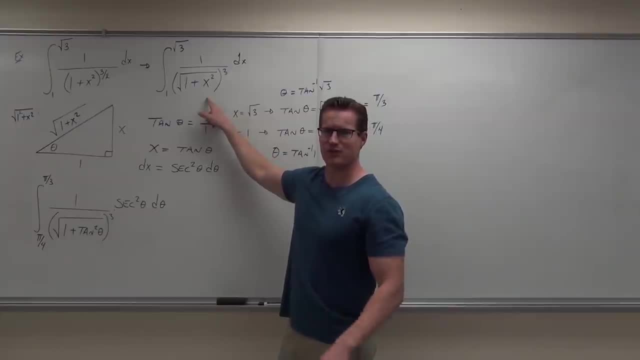 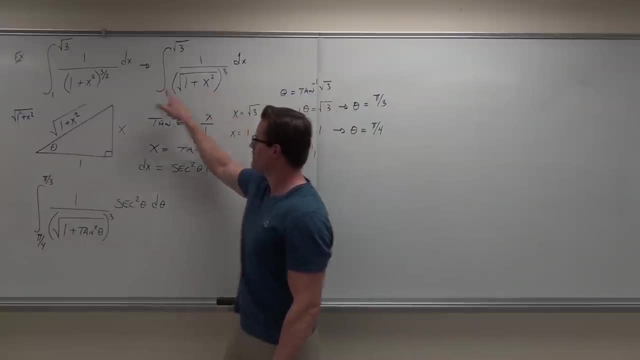 It still wasn't any better, was it? Mm-hmm? Yes, People in the video think you guys are lame right Right now, Right on, All right, Anyway. so this is now that I have potency. we talked about why we're trying to make our sides. 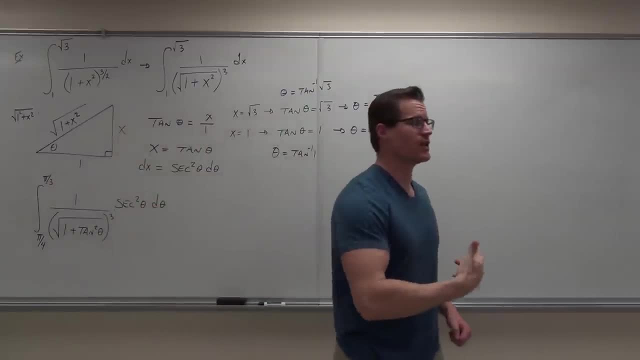 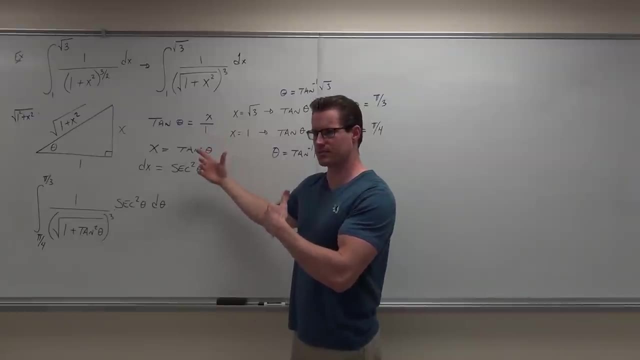 in a relationship that work with tangent or sine or secant. They give us x over a constant. We've done that with tangent, So tan theta equals x, no problem. Now, if you have a definite integral, change your bounds here. 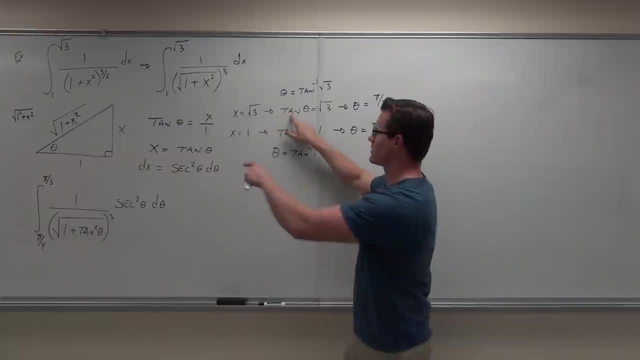 If we change our bounds, x equals square root of 3, okay, Tan theta equals square root of 3.. That's what we're getting. That means that you're going to have to do tan inverse or square root of 3 to figure out your angle. 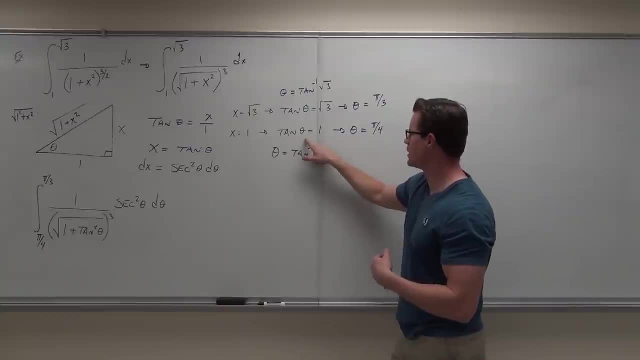 In this case, we get pi over 3.. In this case, where tan theta equals 1,, pi over 4. Tan of pi over 4 gives you 1.. So we've changed our bounds from pi over 4 to pi over 3.. 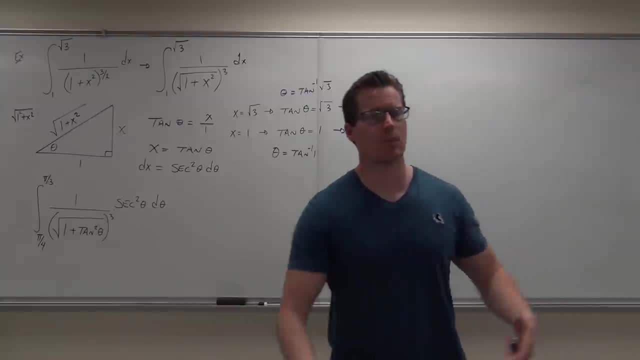 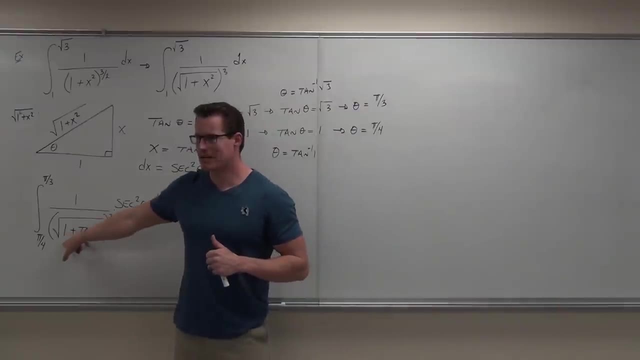 And it's still in order, which is nice for us. Okay, next step, Come on, Tell me what we're going to do. I think the square root from the bottom, From the bottom. So we're going to use our identity. 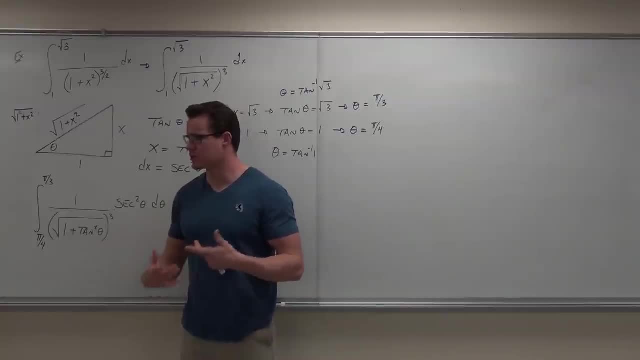 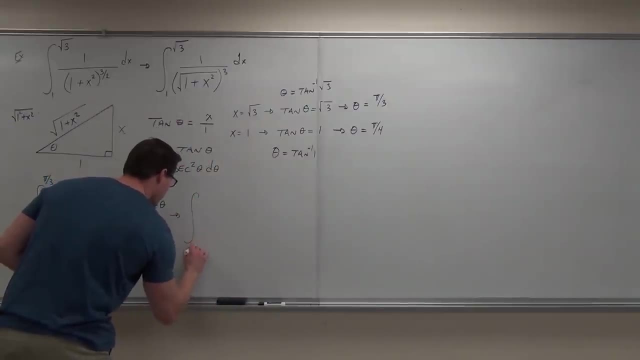 Get rid of that thing. This is always going to happen. if you do your trigonometric substitution appropriately, You're going to have an identity. You're going to have an identity that you'll use. So we'll have pi over 3 to pi over 4 to pi over 3.. 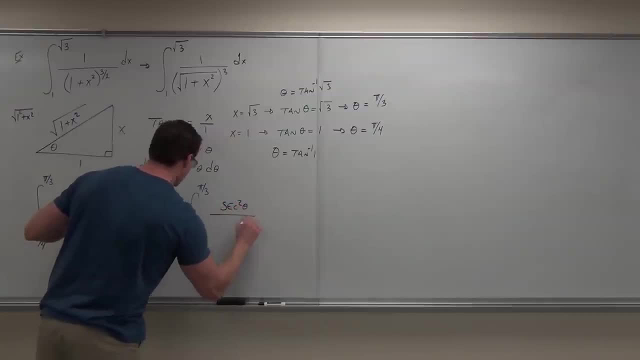 Got a secant squared theta over. tell me what this is going to be exactly. what's still there? Square root of 3 plus 1.. Okay, square root is still going to be there. I like that. What else? Square root of q. 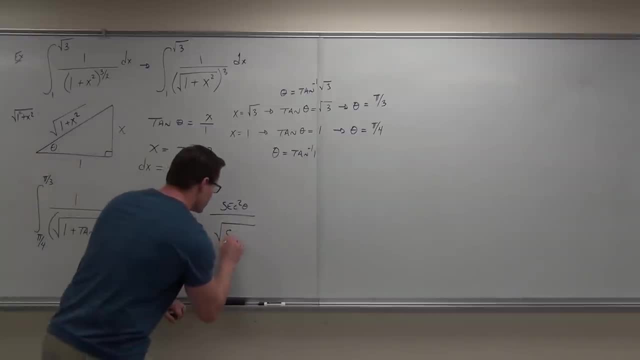 This is an identity. This is equal to secant squared theta Square root of 3 plus 1.. And what else? Q? Don't forget any little pieces here. Cool, almost done. What's the next thing that we're going to do? 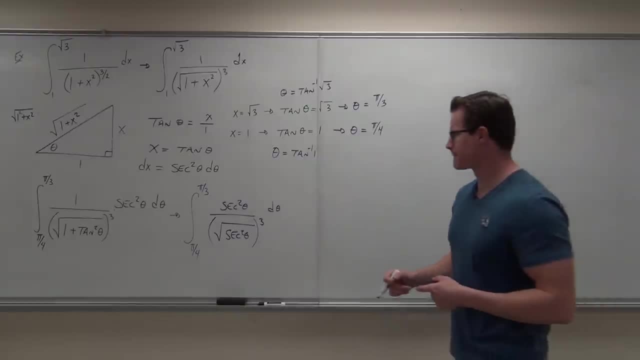 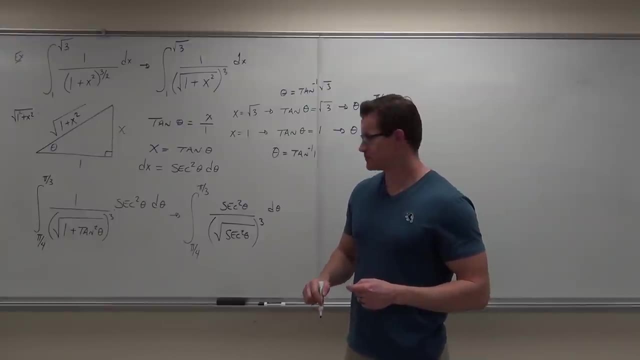 Quickly come on. You could take it out of the square root. You'd end up with 1 over the square root of secant, squared theta to the second, And then the square roots would cancel out and you'd end up with 1 over the secant. 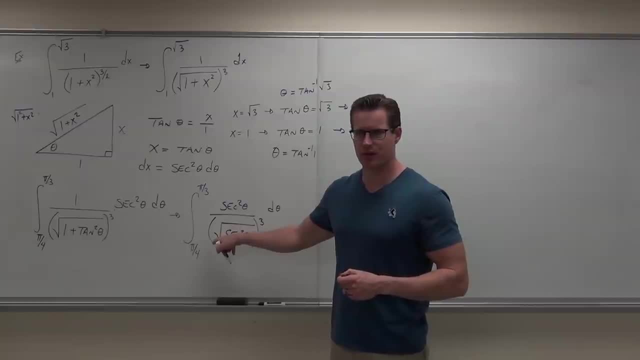 So let's simplify this part. Let's do that: Square root of something squared, what happens? Take root of square root Down. So we got pi over 4.. We got pi over 3. We got secant squared theta. 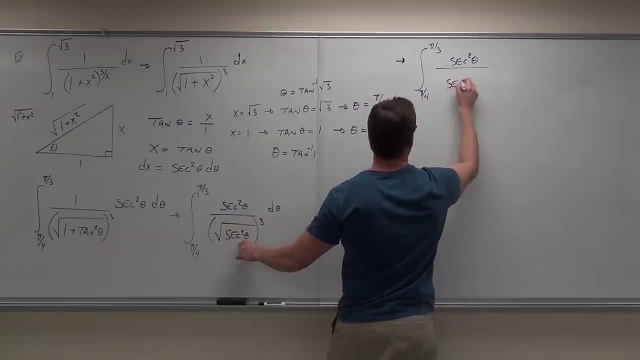 We got the square root of secant. squared is just secant, but then I have it to the third power. So this gives me secant theta to the third power. Are you still okay so far? Notice all the simplifying you're doing. 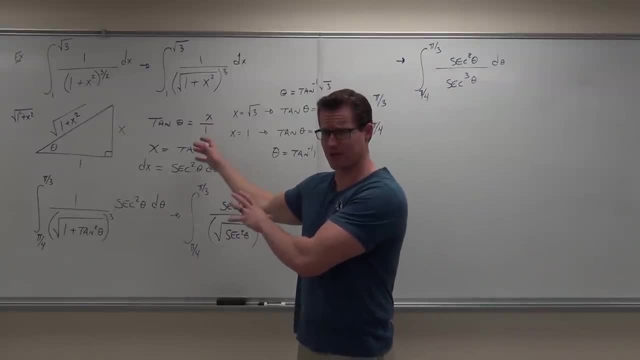 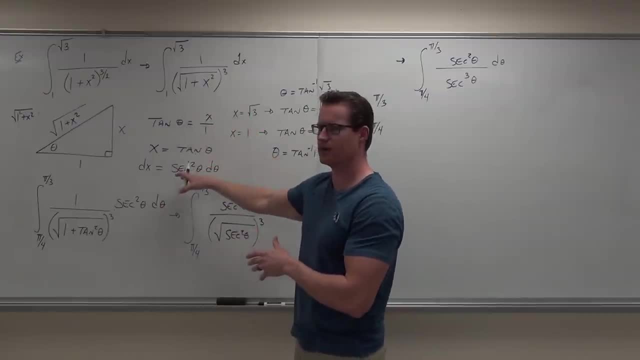 Have we actually done any? maybe a derivative here? huh, Maybe a little bit. That's pretty easy. We're just really simplifying a lot of this to make it nicer for ourselves. So pi over 4,, pi over 3.. 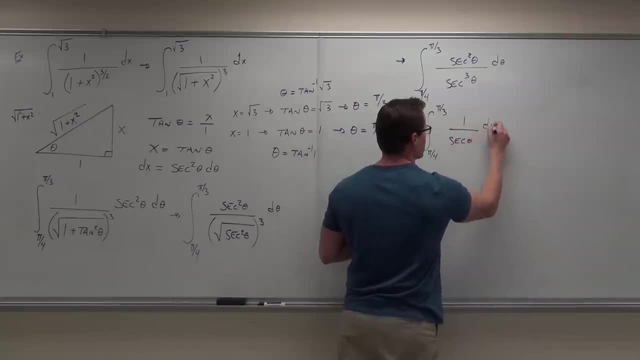 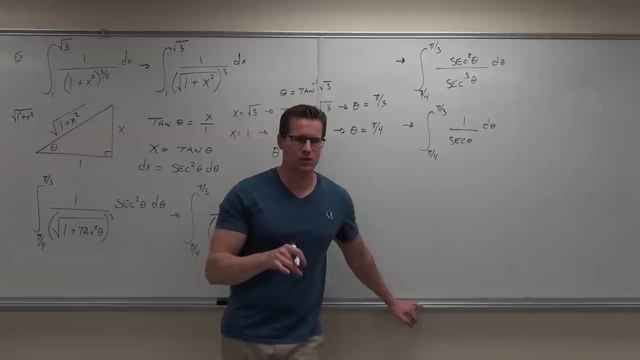 We're going to have 1 over secant theta, d theta. Don't get hung up on this stuff. Think back to what I told you about trigonometric integrals. How trigonometric integrals work. is this If you have sines and cosines? 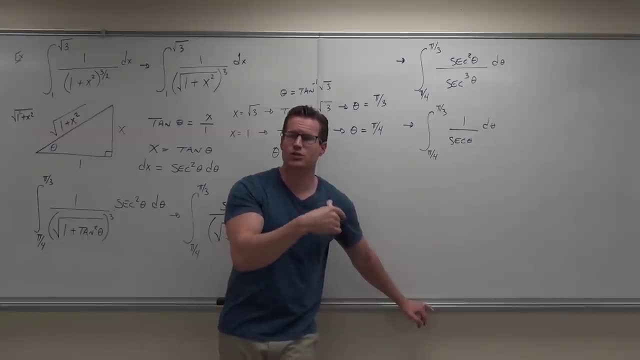 I told you how to deal with those. right Yeah, If you've got tangents and secants, I told you how to deal with those. If you have cotangent and cosecant, I told you how to deal with those. If it's not one of those things, try changing it into. 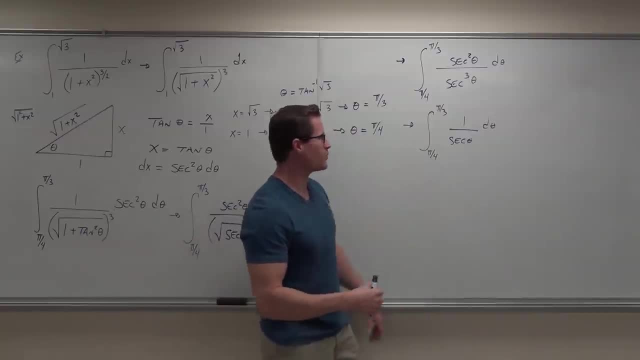 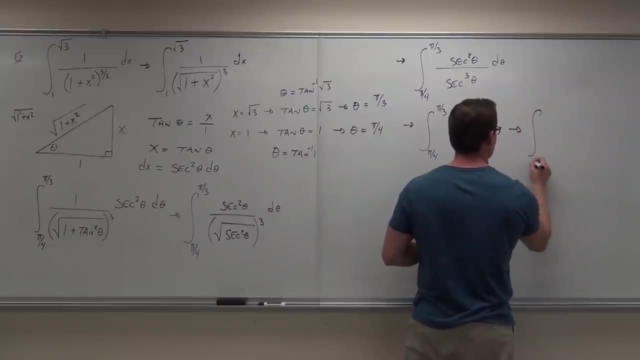 Cosines, Sines and cosines. Try changing that Man. what's 1 over secant? Well, let's think about 1 over secant is cosine. So pi over 4 or pi over 3, no problem. 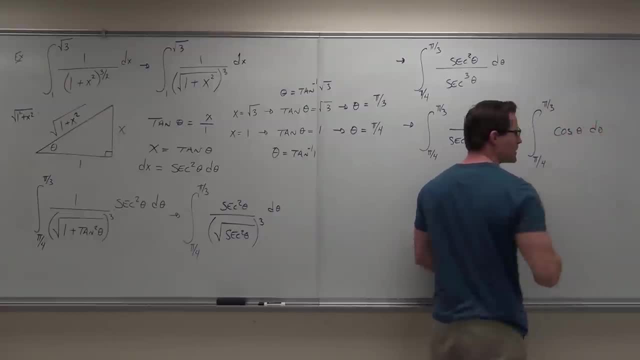 This is just cosine theta and all of a sudden we have a very, very easy Integral to do Everybody. what is the integral of cosine theta? What do you think, Sine theta? Perfect, Oh, you got everyone now. 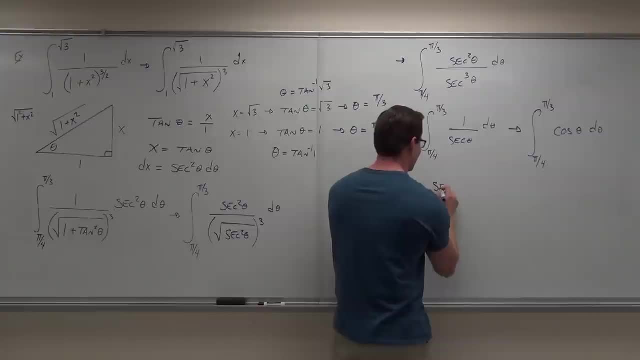 Oh my God, We woke up Sine theta. Now here's the question: Do I have to go back and change everything into x's again? No, This is why you'll want to change bounds here, because if you don't, you're going to have to use your triangle. 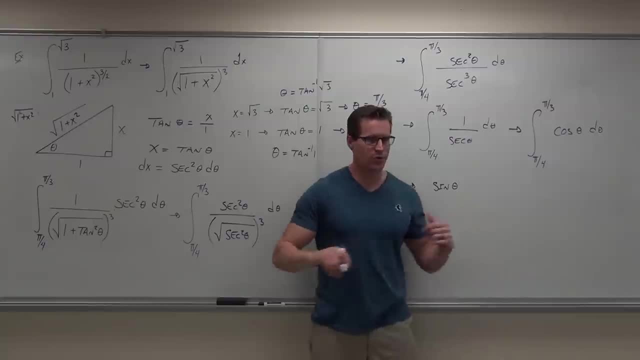 You have to go back and change this back into x's before you change it. Yeah, No, Before you plug in 1 to the square root of 3.. Did you just catch what I said? Yes, Okay, So if you change bounds, this is kind of nice here. 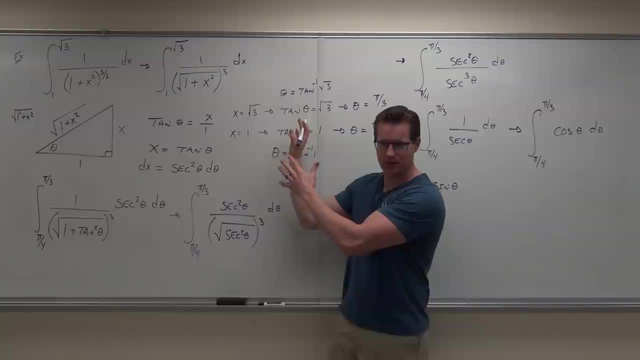 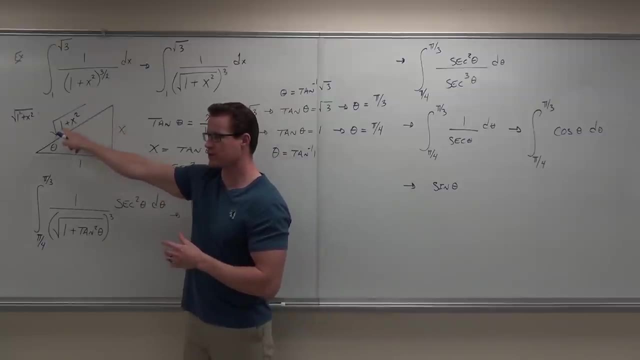 because you don't have to go back to your triangle. If you didn't do this right now, you'd be looking at sine theta. You would have x. look at this please. You'd have x over this square root of 1 plus x squared. 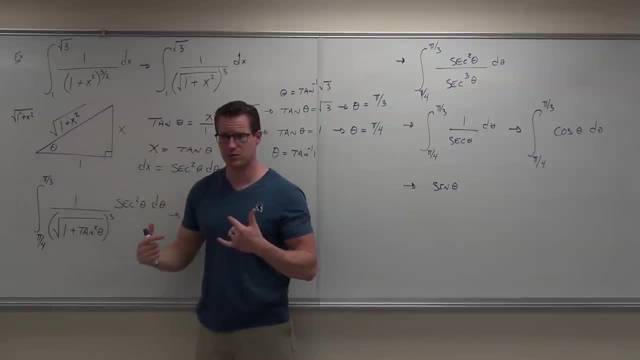 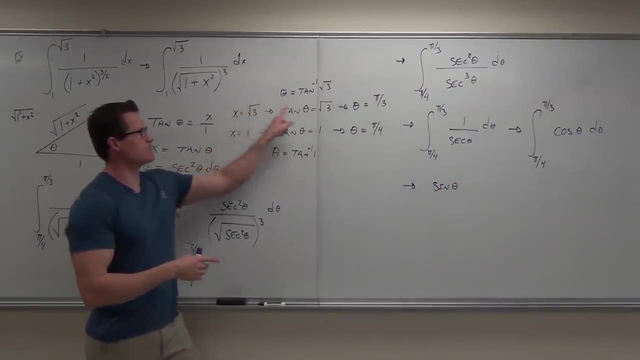 Then you plug in the square root of 3, and you plug in 1, and you'd subtract those two fractions. Does that make sense to you? If we change bounds, no big deal. We change these from x's into thetas. 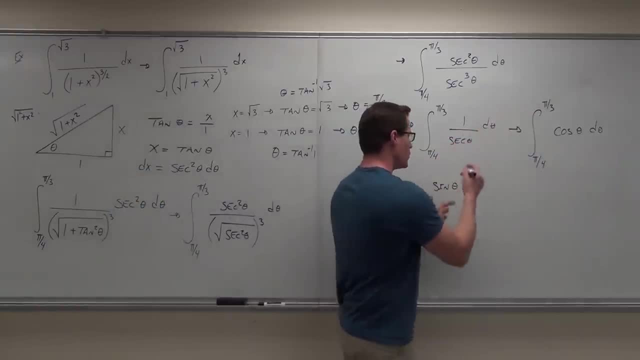 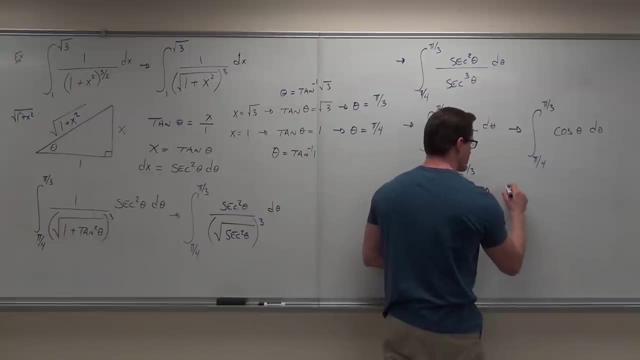 Hey, it matches now. So now these are in terms of theta. No need to plug it back in. We're just going to go pi over 4 to pi over 3.. What that means is we'll have sine of pi over 3 minus sine. 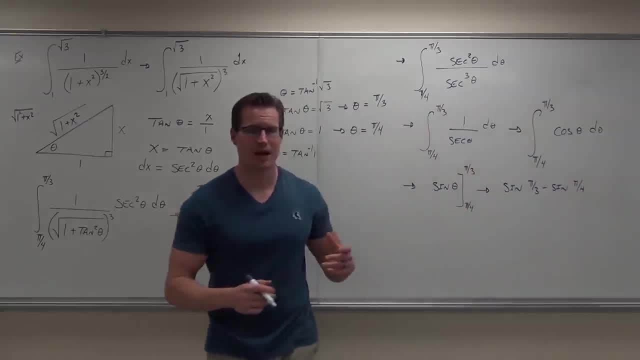 of pi over 4.. That should be pretty easy for us at this level. Sine of pi over 3 is what? Square root of 3, square root of 2, 2.. That's square root of 3.. All I heard was: ooh, ooh, ooh, ooh. 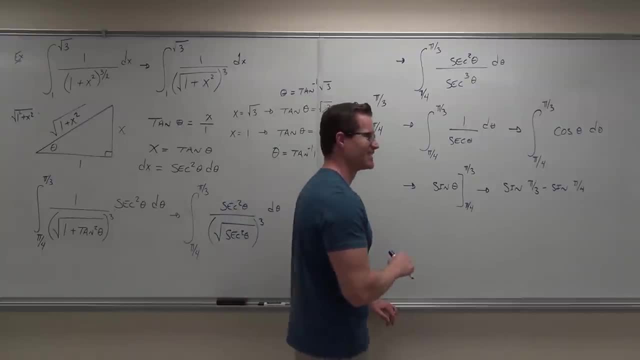 Square root of 3 over 2.. It's over 2.. That's good. Square root of 3 over 2.. Isn't the integral of cosine negative sine? No, it's not. We'll have to think about why. 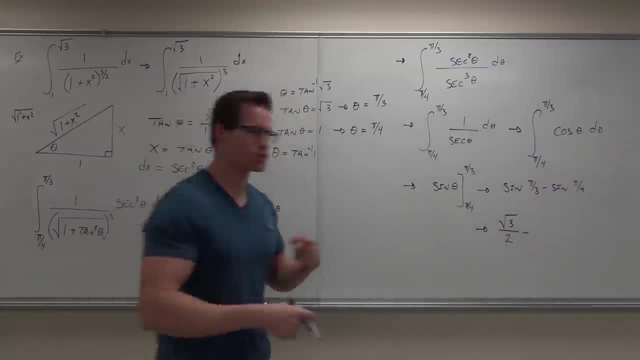 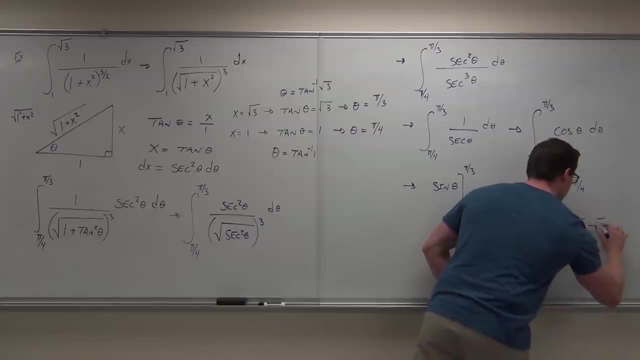 Okay, Square root of 3 over 2.. Very good, And Square root of 2 over 2.. Square root of 2 over 2.. Make them one fraction: Square root of 3 minus square root of 2 over 2.. 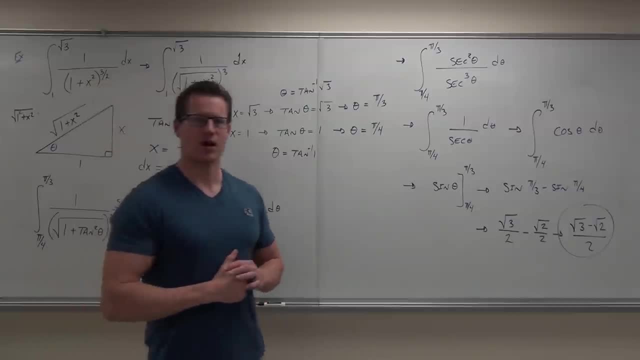 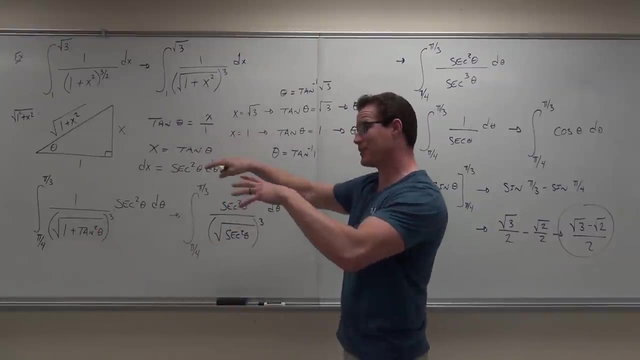 That's the idea. Took us a little bit longer than I thought, but show of hands. if that mode made sense for you, Good deal. Okay, Let's work on the next one. So definite integrals you might definitely want to try. 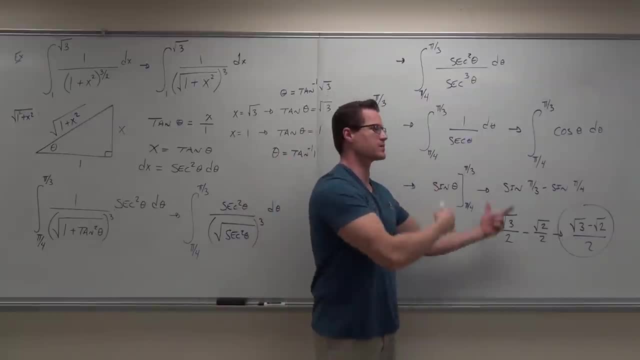 to change your bounds here. That way, you don't have to use your triangle to make your resubstitution Just a good idea. Are you guys okay? down to this far Show of hands. if you are, Very good, That's fantastic. 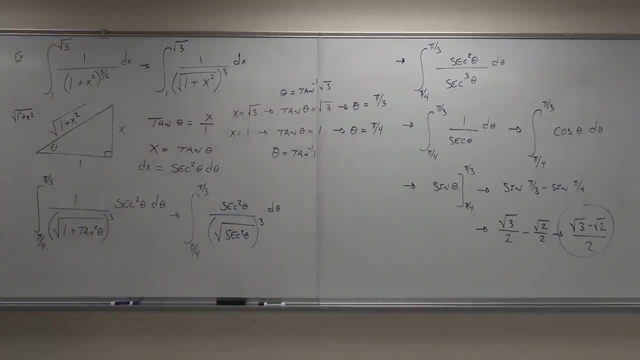 That's what I'm looking for. Let's do the next one: Questions, Comments, Concerns. Is it more understandable than the first time we went over? Yes, It's getting easier. Is it getting easier for you? I like definite integrals better. 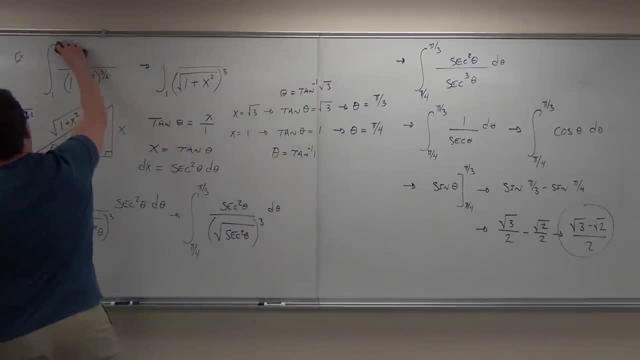 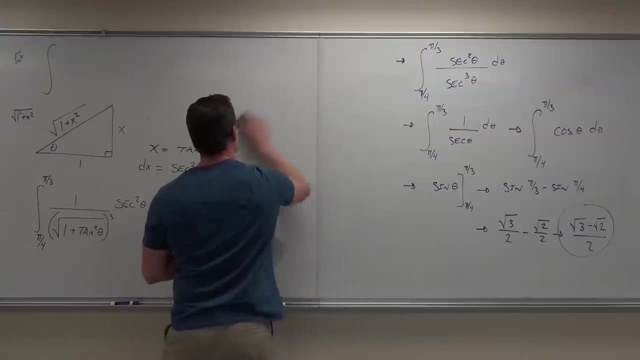 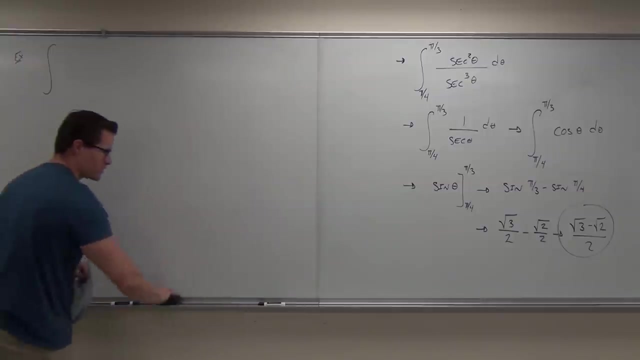 These ones, Yes, Ah, Why There's no resubstituting? That's why, That's why you change your bounds. Well, of course, Rob, now that you've said that I'm not going to give you more definite integrals. 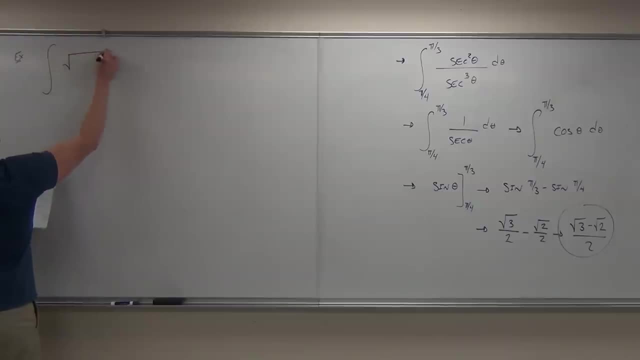 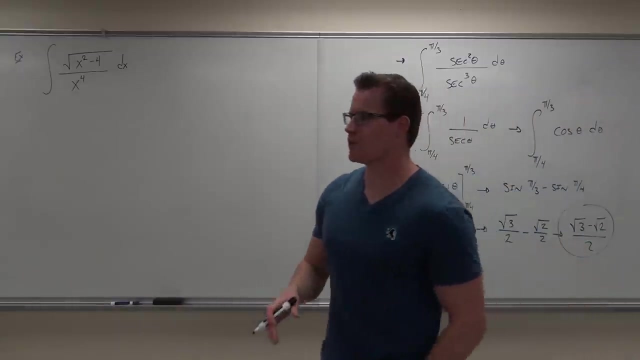 We're going to practice these ones now. You're welcome. Okay, here's what I want to do. I want you guys to try and do this problem basically completely on your own, but we're going to do step by step. So the first thing I want to do, I want to see if you understand that it's going. 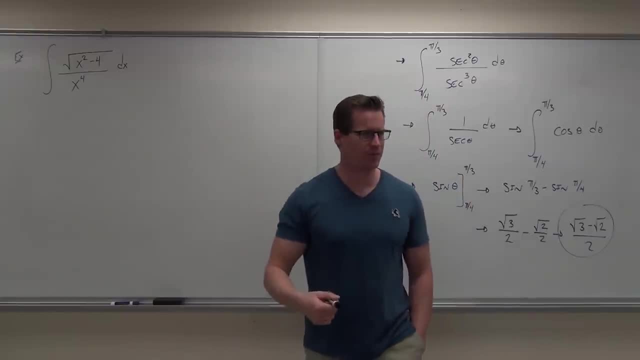 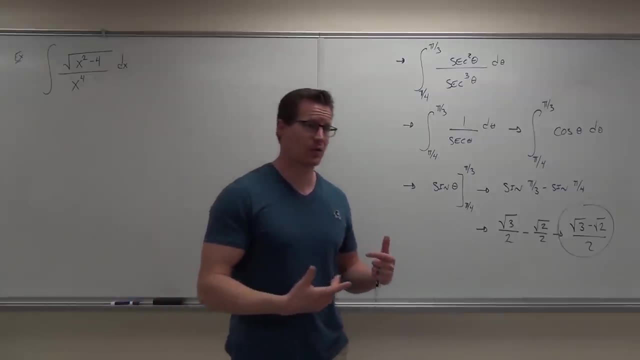 to be a trigonometric substitution. Can you see it just by looking at the problem. We're looking for, well, substitution, firstly, Substitution ain't going to work. We're looking, is it by parts? Well, not really. 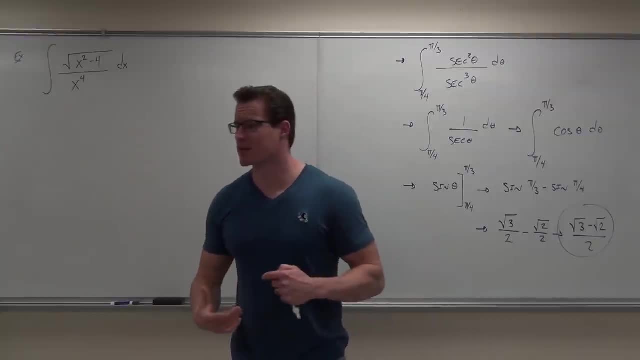 We don't have a product that's going to work for us very nicely. Is it a trigonometric integral? Well, not yet, but we're going to make our substitution, So I want you to pick the piece that's going to be the trigonometric substitution. 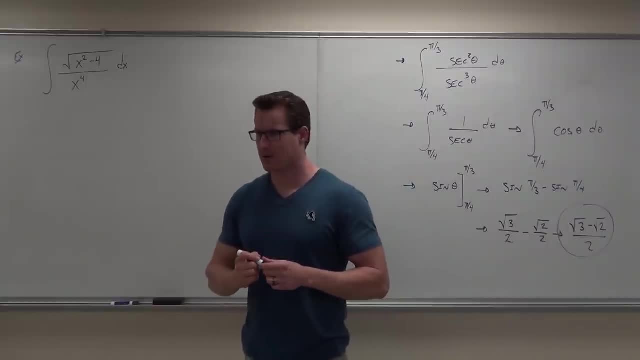 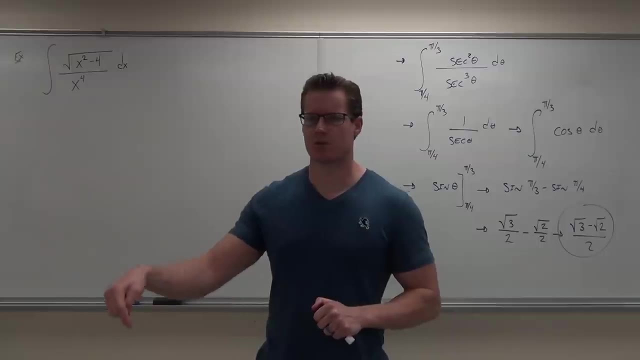 Go ahead and do that now. Pick the piece that you're going to use. It's always a square root, always. If there's no square root in the problem, you need to make a square root in the problem. You can do that algebraically. 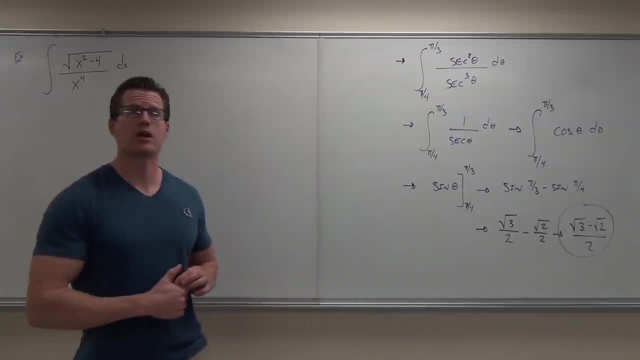 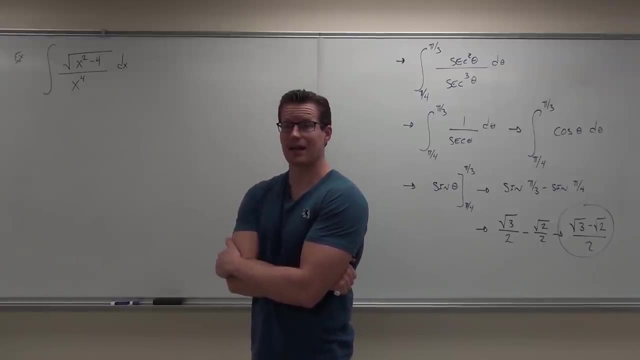 So pick a piece of that that's going to be your substitution. Make a triangle from it. Make a triangle, Think about it, Think about the piece that you just picked. Is that the hypotenuse or is that a leg, A leg? 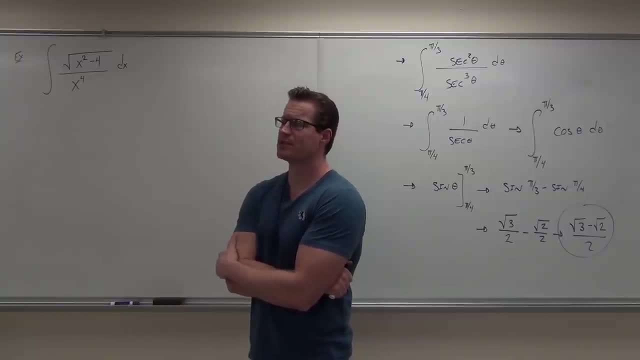 A leg. Okay, so you have it as a leg. Pick the appropriate piece of this- that's the hypotenuse- first. So label that out. Do it individually, Do it on your own. Let's see if we all get the right triangle. 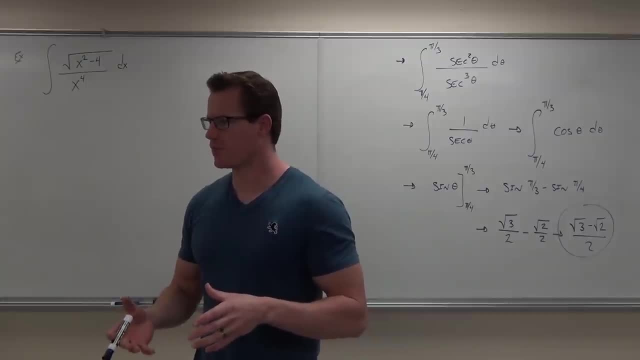 Did you guys know that making the triangle is like the most important point part here, Mm-hmm. After that, once you translate it to a trigonometric integral, it's pretty straightforward. I taught you how to deal with it. 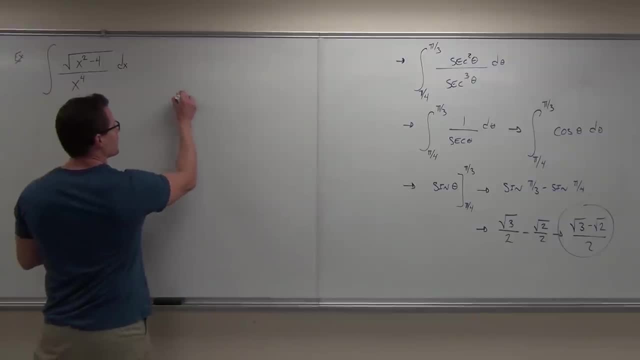 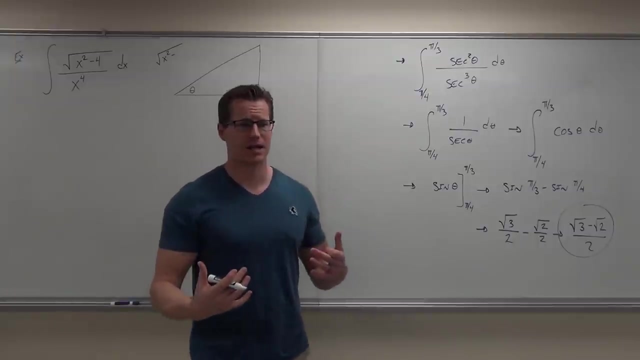 The triangle is important here. I want to make sure y'all got this. It's a right triangle. The piece you should have picked is x squared minus. I'm not going to write x squared minus 4.. What I'm going to think of it as is x squared minus 2 squared. 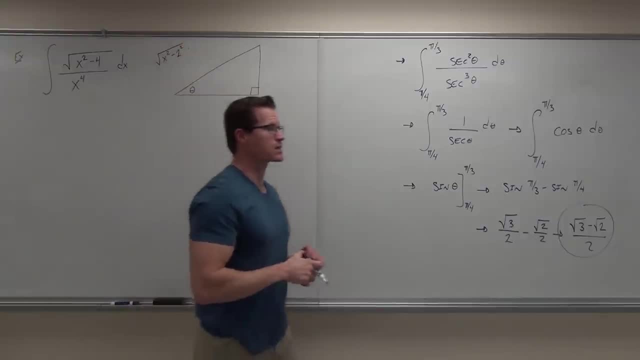 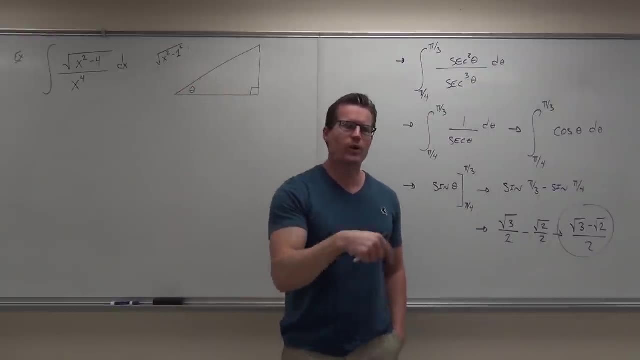 Okay, now let's think about it. Did you find out that this is actually the length of one of our legs? Yes, Okay, Now how do we start this? We're going to start with the hypotenuse first, always because then we can determine what. 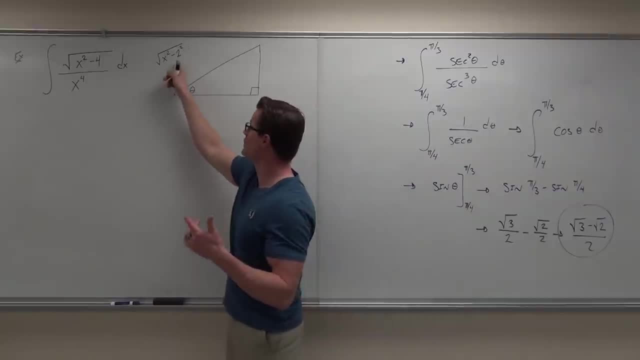 our legs are after that. So if this is a leg, then one of these pieces is going to be my hypotenuse. Everybody, what is my hypotenuse in this case? X? Very good, Yeah, it's always the one that comes first. 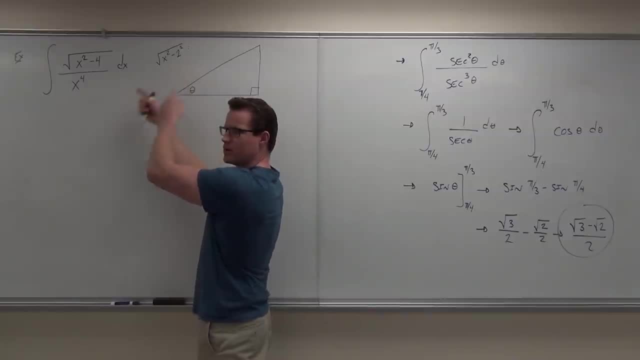 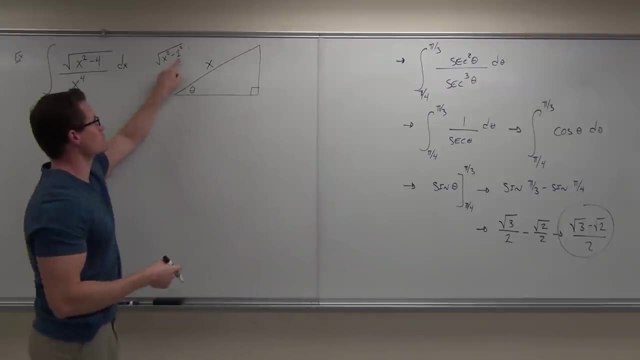 Otherwise you have a negative inside of your radical. it's not possible. So x is our hypotenuse. The reason why we write this as 2 squared rather than 4 is so that we don't accidentally put 4 here or 4 here. 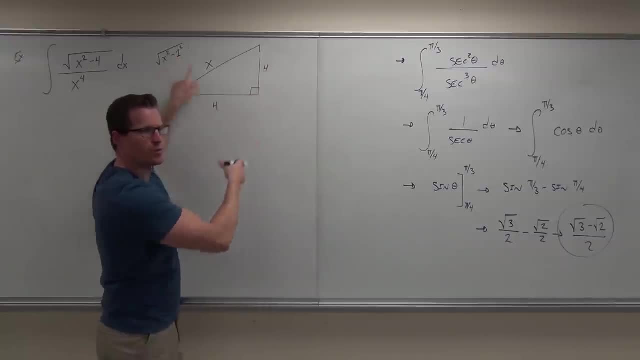 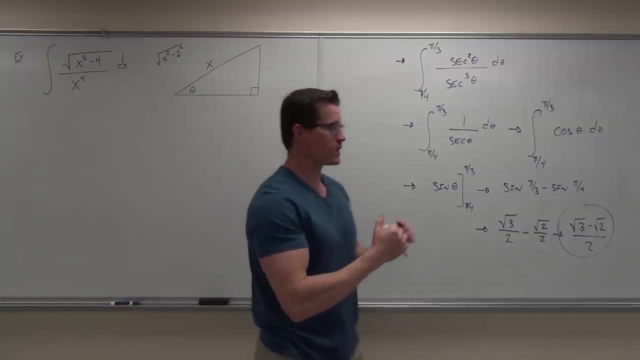 Okay, If we put 4 here, we put 2 here or 2 there, depending on which side that we need to use for this. Does that make sense to you? Okay, now we'll think a little bit harder. Which trigonometric relationship would we want to use here? 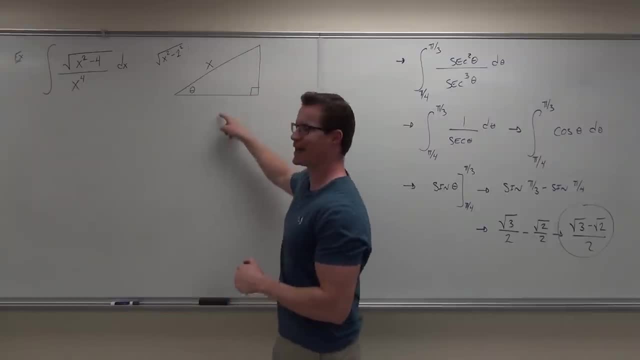 Would we want to use tangent at all? No, No, Tangent's going to have a square root in it and that sucks. I don't want that. Are we going to use sine? No, No, Sine would have x in it, but it'd be something over the x. 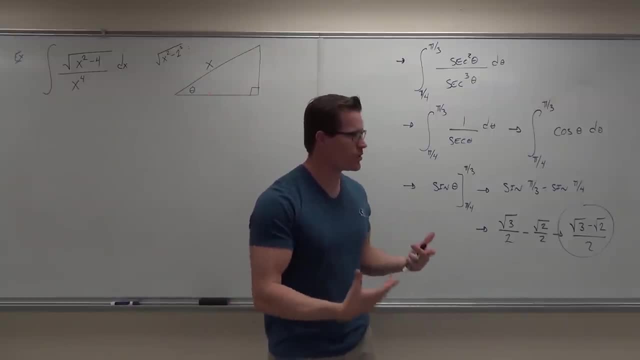 This is the way you go through. You actually think about these. Don't just follow the pattern. Think about what's going on here. Tangent sucks. It's got a square root Sine. Sine's pretty close because we could make it constant over x, but I don't want it over. 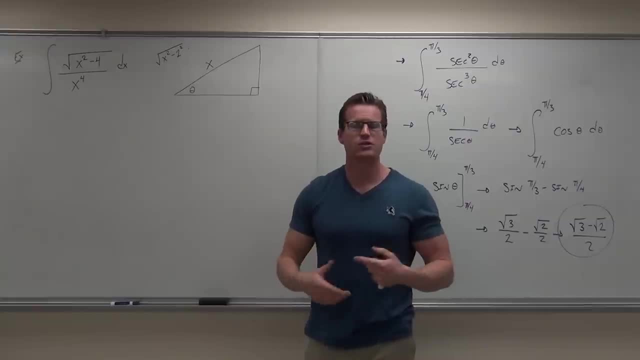 x. I want x over something. So the only other option that we have is Secant. So set up this triangle so that secant is going to work nicely for you. Where does the square root go? Bottom leg, right leg. 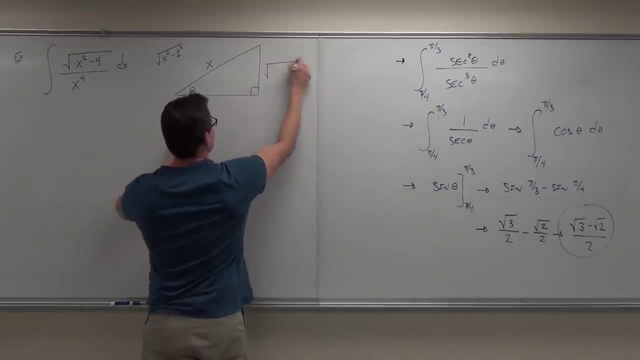 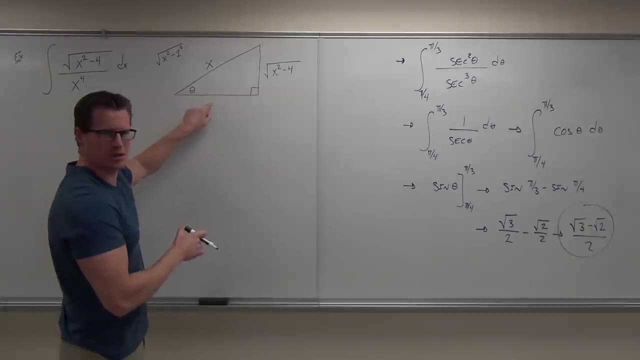 That way we get it out of the secant relationship. So the square root is x squared minus 4.. I'll put the 4 back because I don't have to worry about that anymore. And this one? what's this going to be? 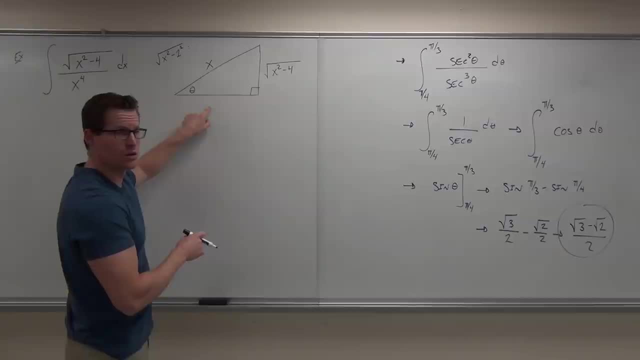 2. 2. 4. 2.. Do you understand why it's 2?? This is why we do that. Let's make sure this works for us. We have hypotenuse, Got it. We have one leg here. 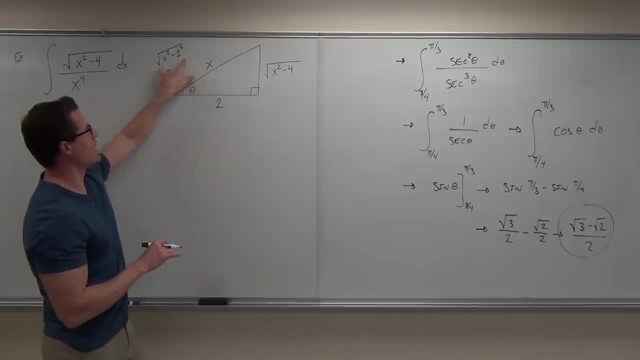 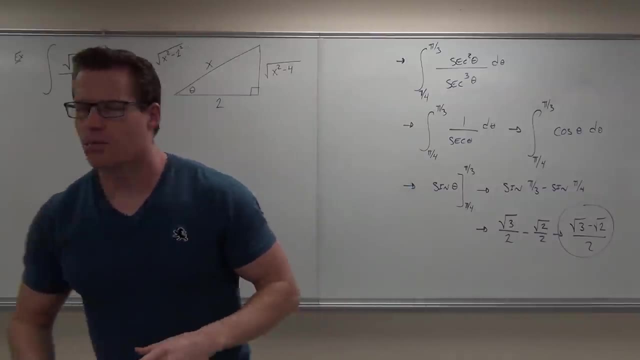 This is going to set up our secant relationship, And then we have this as another side Show of hands. if you feel, OK, Cool, OK, Go do the next step. If you haven't done it already, write the trigonometric relationship we just talked about. 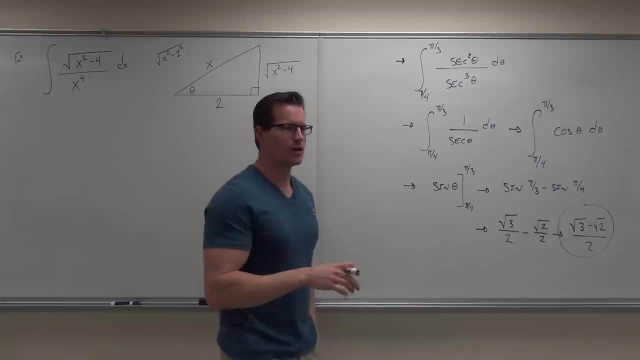 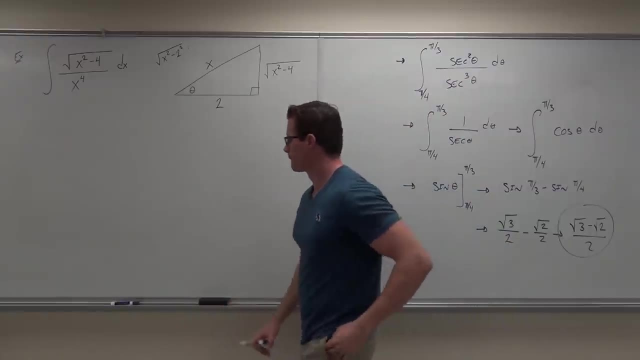 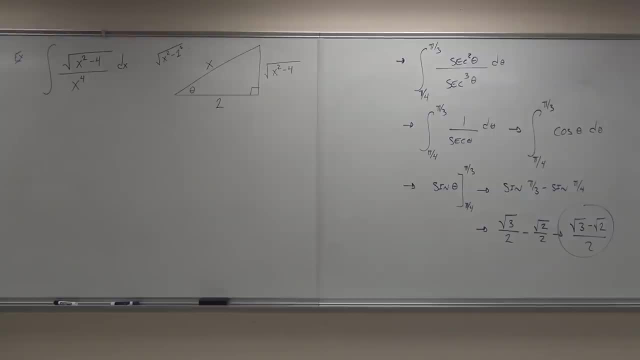 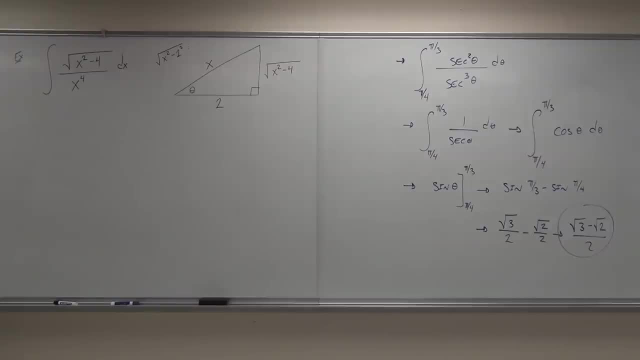 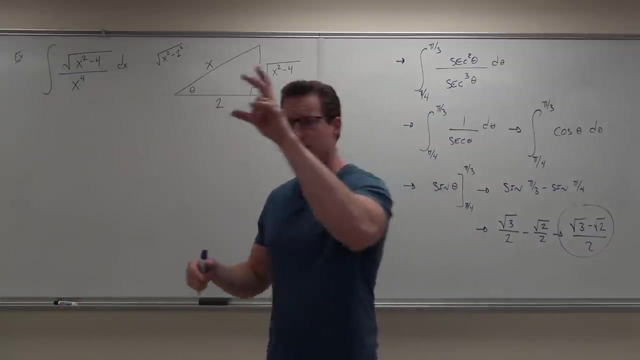 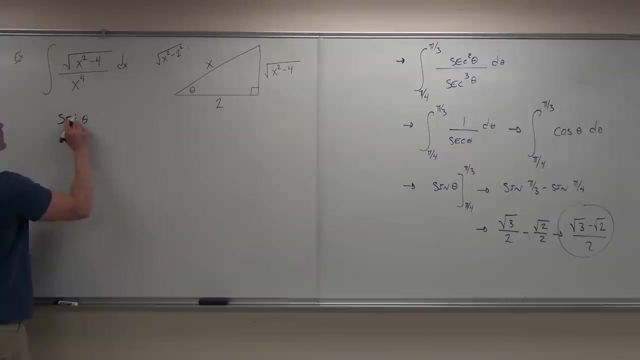 1. 1. 1. 1. Dr. Okay, which one works again. Secant Dr. Yeah, secant's going to give us hypotenuse over adjacent. So secant theta makes that relationship that we want. 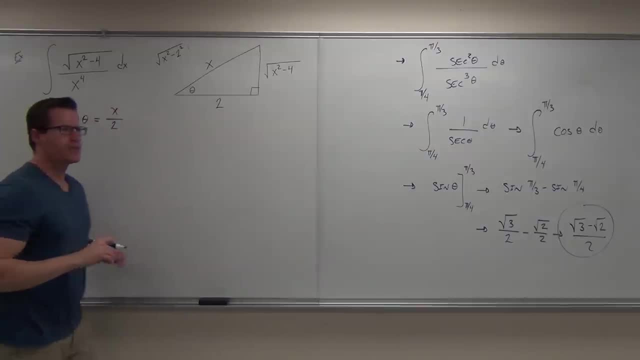 We want x over some sort of constant, Then what would we do after we get x over some constant? Solve for x, Dr. Yeah, solve for x, because that's going to be our substitution. I don't see any x over twos over here. neither do you. 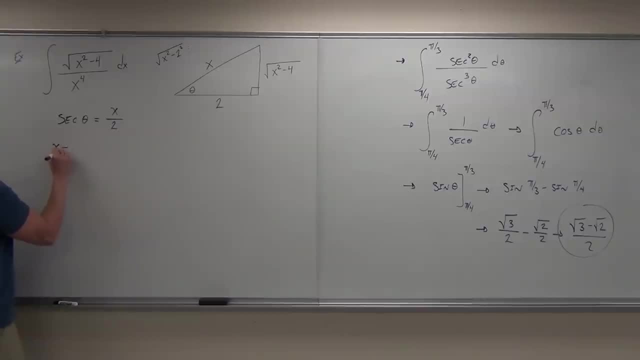 I see just x's, So let's make this: x equals two secant theta. Okay, everybody, what's the next thing that we're going to do? Take the derivatives Dr. Yeah. What do we have to substitute for our x's? 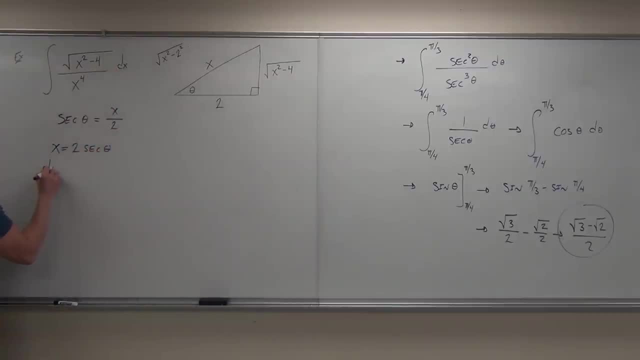 We also need to substitute for our dx, So by taking our derivative, by the way, just a question here: should you use a product rule here? No, Dr. No, it's a constant. Don't make things harder than they are. 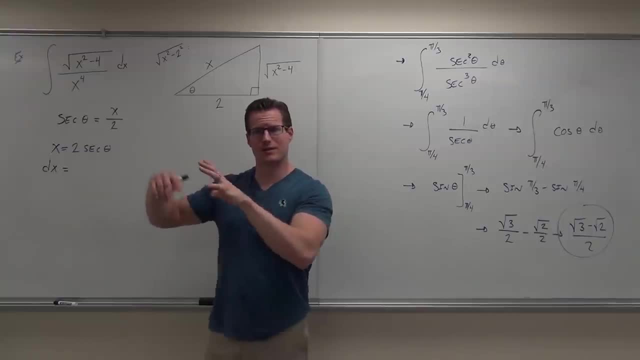 Don't do something silly, okay? I know that a lot of people think that this is going to be a really, really hard class, and in some parts it is, but don't make it harder than it is. If it's a constant, you wouldn't do this. 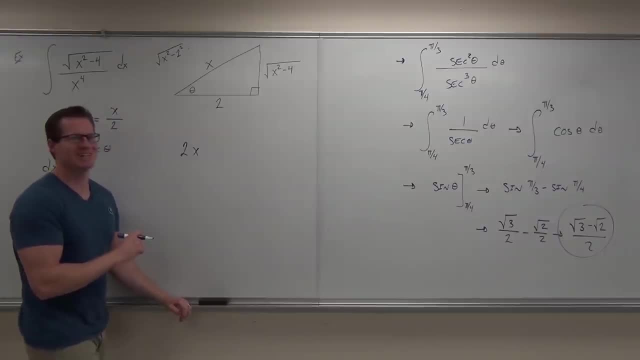 What's the derivative of two x Product rule? Let's do it, Dr. No, that's silly, right, That's a product, But that's a constant in front, It's a factor that happens to be a constant. So we do two, and then what's this become? 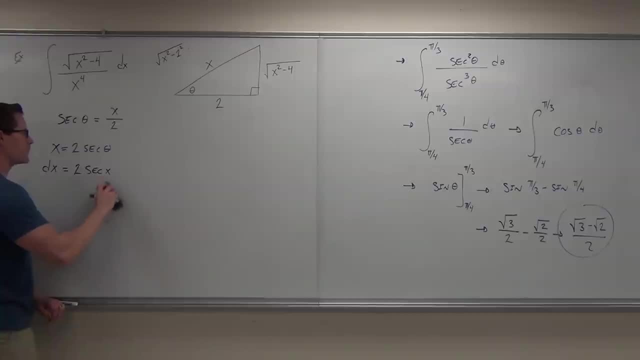 Theta, Dr. Oh, theta, That's good, Good, And then d theta, Very good. Okay, if you haven't done so already, make your substitution. have you all substituted on your integral Yes, Dr, Not yes or no? 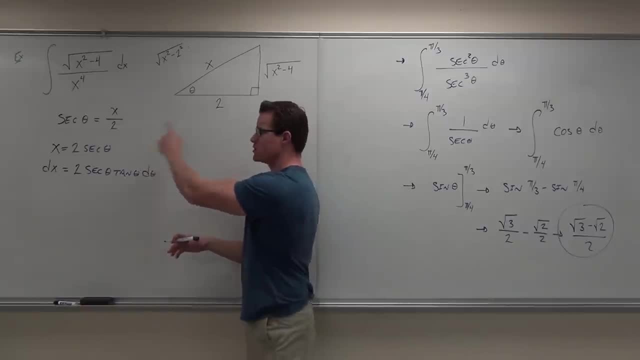 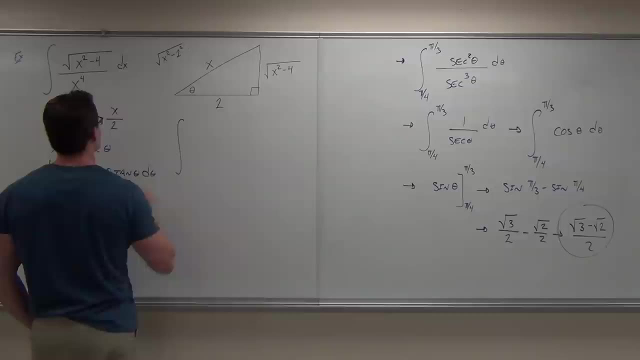 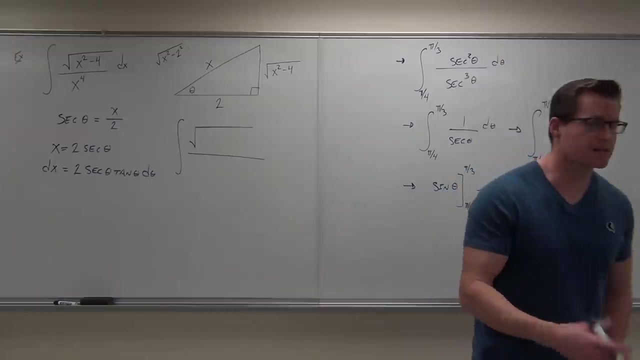 No, Dr, Have you made it that far? Okay, go do that. next, Do the substitution. Let's make sure that we're all 100% correct. There's a lot of pieces here, lots of stuff going on, so make sure we're all right. 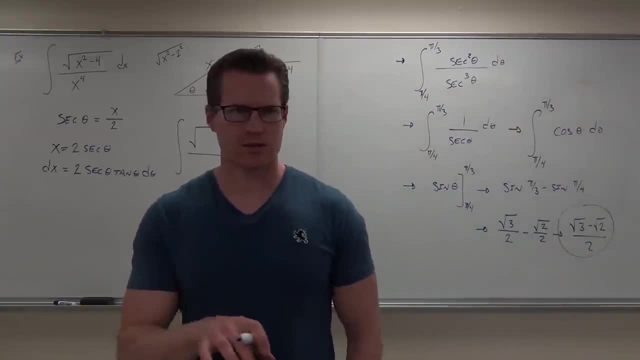 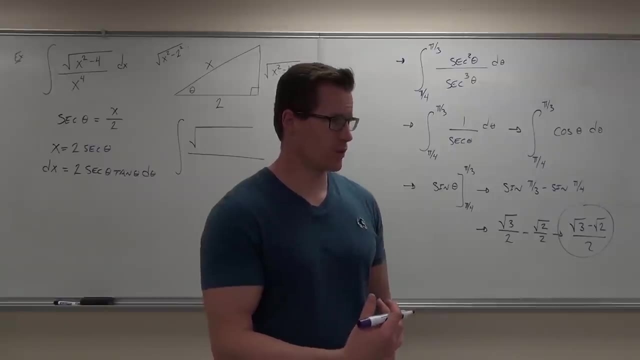 Where you have x, what are we putting in for x? Secant two: secant theta Dr. Oh, close, Don't forget that. two. If you get the constant there, is your integral going to work out? No, Dr, It will, but your constants are all going to be wrong. so make sure your constants 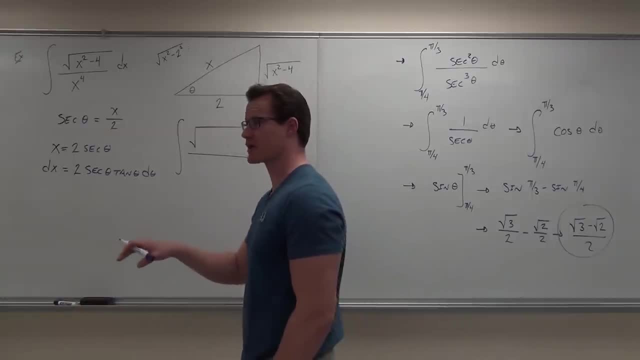 are correct. If it's two secant theta, make sure that goes in every place for x And your dx. make sure we have the correct thing for dx. So let me make sure you get the same thing I'm about to get. 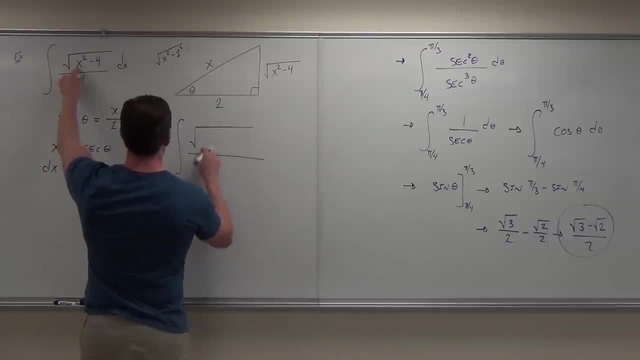 Let me have your eyes on the board here real quick, please. So x squared. I still have a square root, but x squared, no, no, no, For x squared, I'm going to have this whole thing squared. Notice, it's not this. 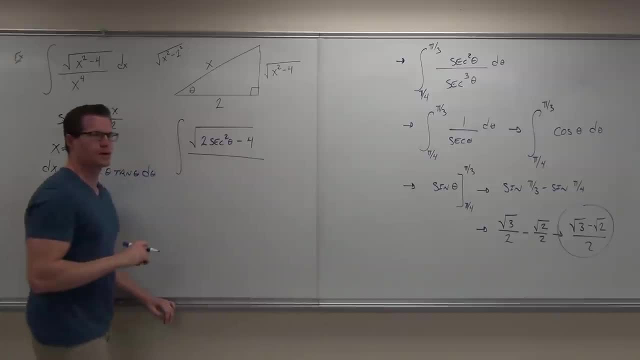 Do you see why not? Yeah, when I have x, this whole thing is the x. so when I square it, it's got to be like that. Did you catch that? That's going to affect this, because what happens here is, when you square the two, it. 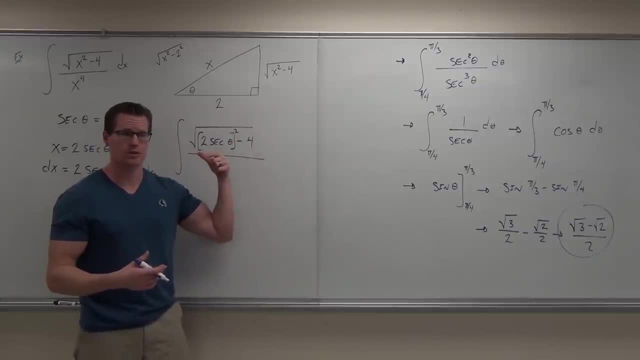 allows you something to factor out. You can take that four out of there, and that's what we want to do. Also to the fourth. well, it's now going to be two secant theta all to the fourth. Okay, So we got two secant theta, no problem. 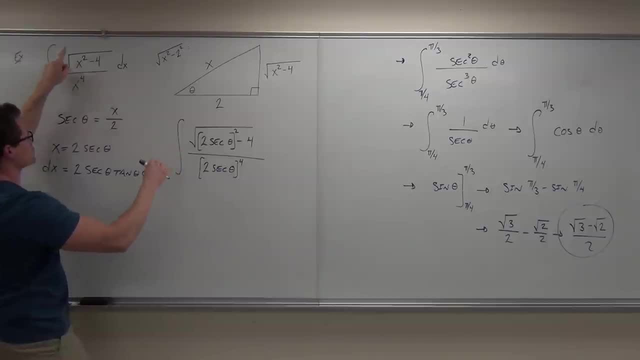 We got it squared, Minus minus four. four Got it. We got a square root around it. We got a two secant theta. now it's to the fourth power. and lastly, what else do I need up there? 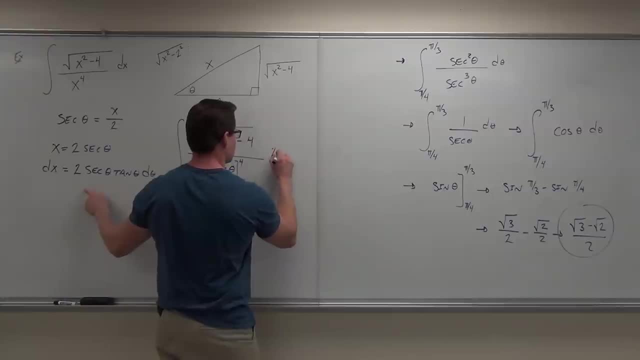 Two to the dx, Yes, Two to the dx. So two secant theta, tangent theta d theta. What I want to know is show of hands. if you got exactly that on your paper, I know you do now, before I did it. 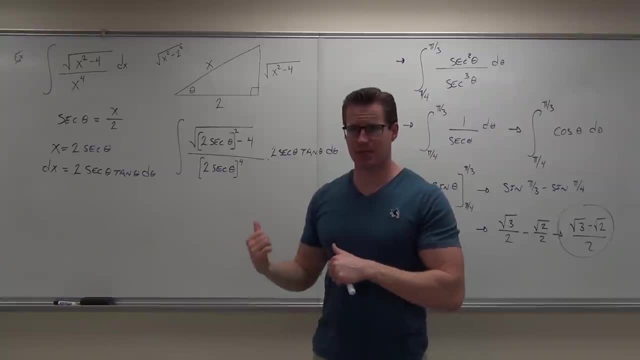 How many people had that? That's good. that's great. that's the first step. If you didn't, does it make sense? how to get that? Are you sure It's gonna take some practice? right, We gotta get this stuff down. 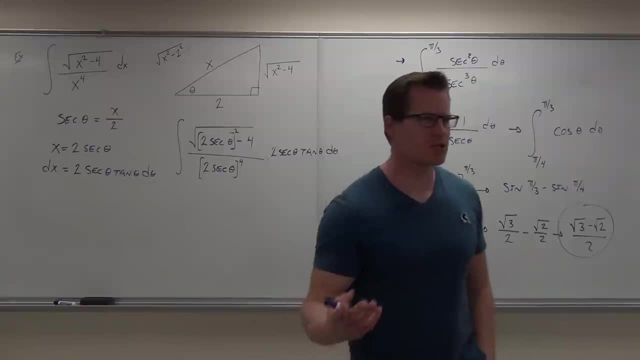 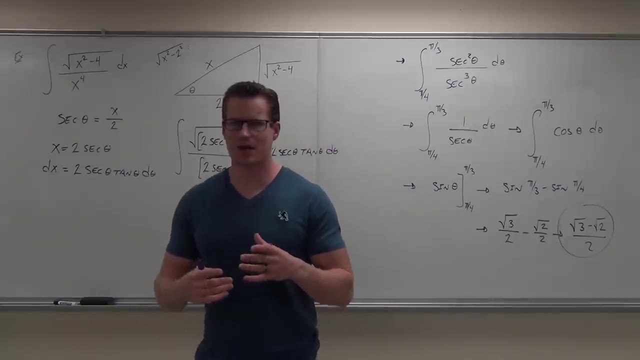 What's the next thing that we should do? Should we start doing substitutions and all that stuff right now? No, What are we gonna do? Simplify, Always simplify these things. Don't do substitutions or crazy stuff until you have this simplified. 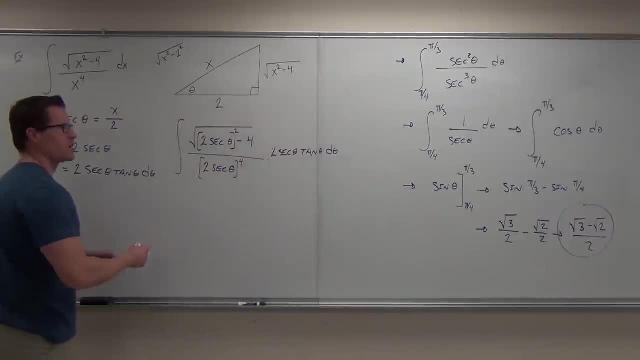 So if we simplify, well, it's just a whole bunch of algebra. I'm gonna go through it kind of quickly. If you have questions, of course let me know. But when we square this, this'll be square root of four secant squared theta. 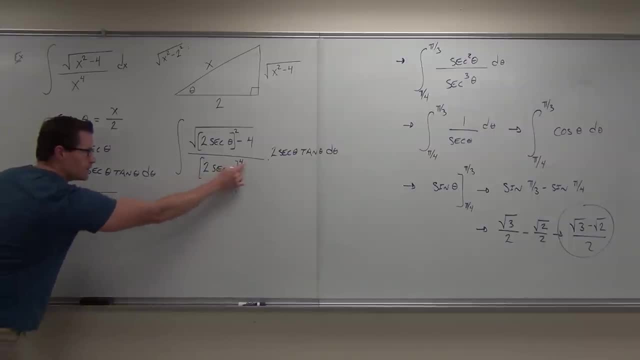 minus four, all over two to the fourth, is 16 secant squared, sorry, secant to the fourth theta. And then, of course, we still have a two secant theta, tangent theta. We can't afford to lose any of this stuff. 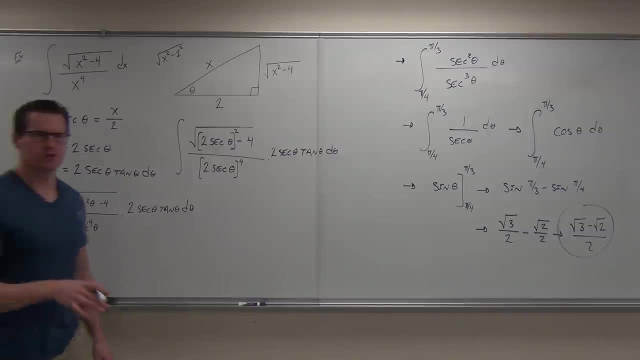 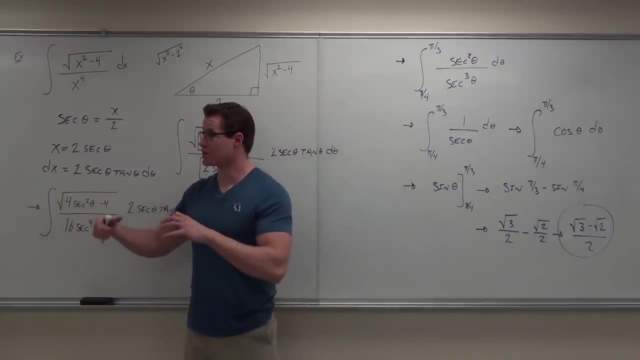 It won't work out. Next thing: what would you do if this was your problem on a test? Because it very well might be. What do you think Factor the inside of the? Yeah, what we know is that identities work with secant squared minus one, not secant squared minus four. 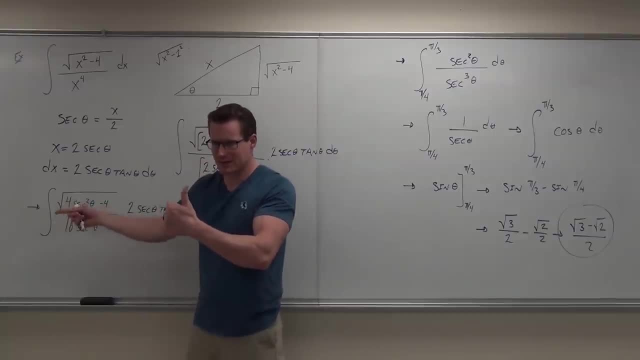 So when we have the same number here, that's what we have to have. That's important. We gotta have that. So if we miss the two here, you're gonna miss the four here. That's a problem. So once we factor that four out, 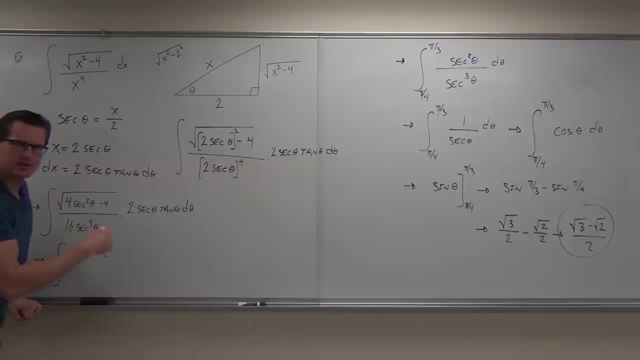 Let me pull it out of the two. Sure, I'm gonna actually do that step right now, okay, So watch carefully. So we have two factors correct. So what we get is a secant squared theta minus one If I factor the four and take a square root. 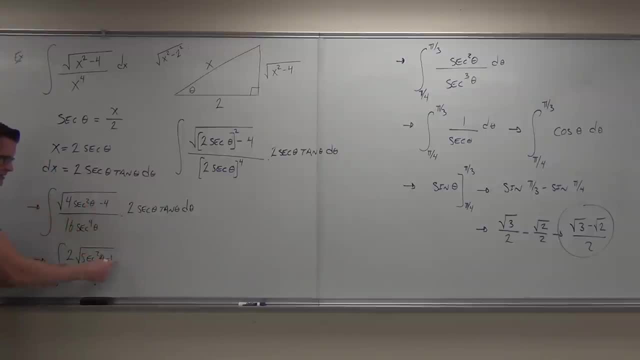 it's going to give me two. Does that make sense? Yes, This is this to me in my head. Is it to you in your head? Yes, Okay, so secant squared minus one. no problem, The four's factored, I take a square root. 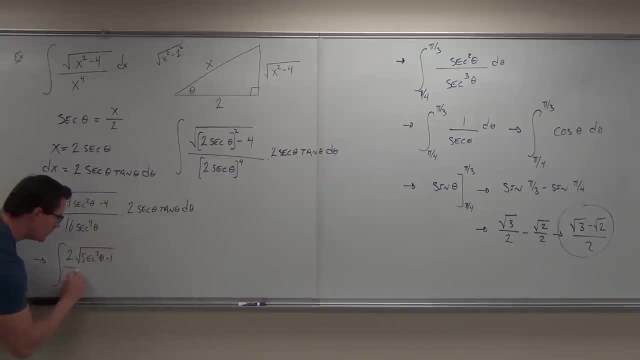 because we can separate square roots like that with products Over 16 secant to the fourth theta times two secant theta 10.. You'll notice that when I'm doing this I'm not doing a whole lot of math in my head. 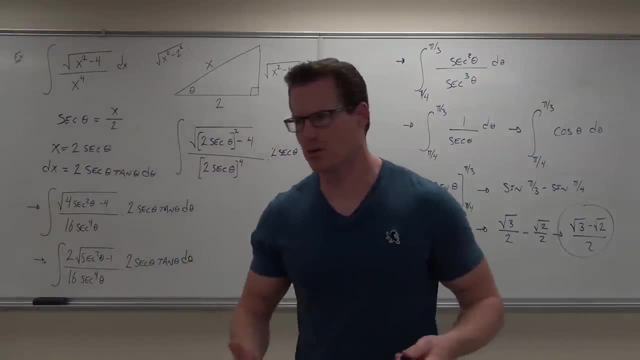 There's a few things, but not a lot, because I don't want to lose any constants. That's the big deal, Not constant? no losing constants, no losing negatives. Tell me some things I can do now. Pull out the 1: 8th. 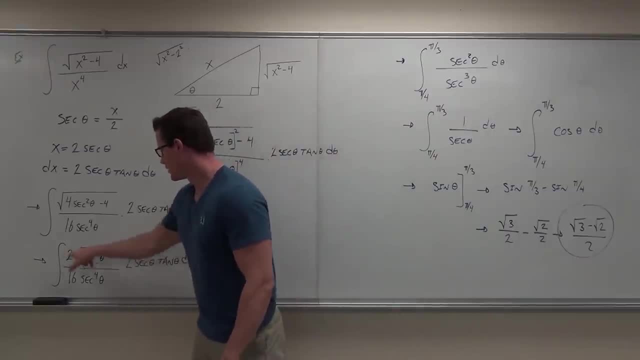 Turn it into a 10.. Okay, let's be careful about that. 1 8th, Oh yeah, yeah. 1 6th, It's gonna be a 1 4th. Pull out a 1 4th. 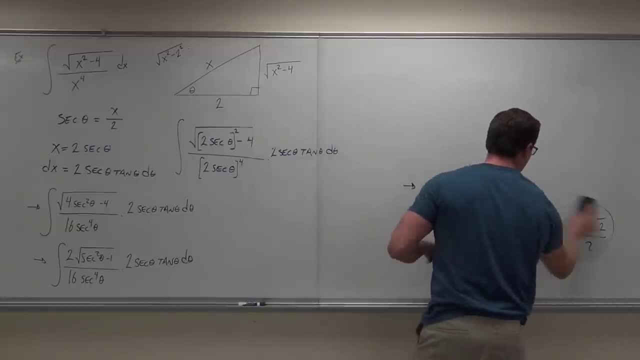 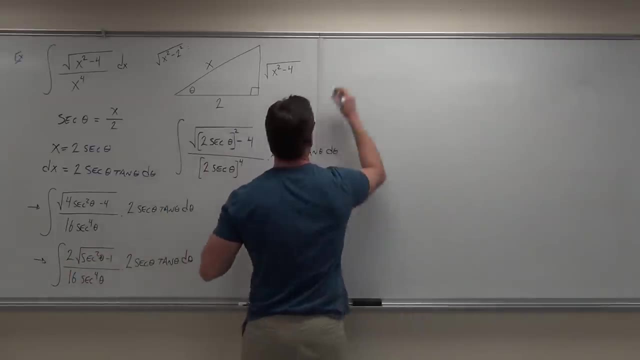 2 times 2 is 4,. 4 over 16 is 1, 4th, So 2, this is 4 over 16, 1, 4th comes out Integral of. so this is 1, 4th. all the constants are gone. 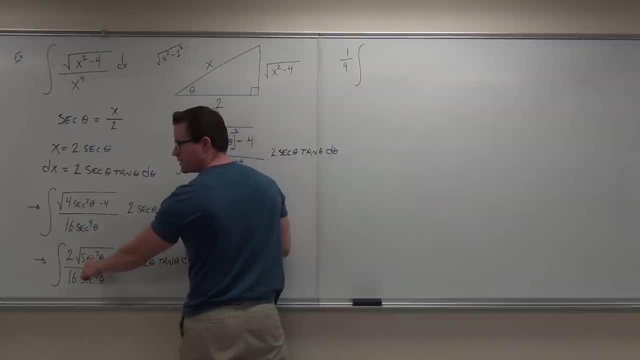 That's what we want. How much is secant squared minus one? Everybody, come on. how much is secant squared minus one? It should be an obvious identity, because that's what we were going for. That's why we did our substitution in the first place. 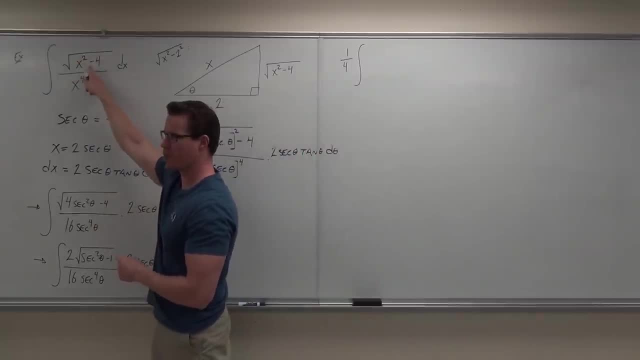 Once we get- hey, look at that, Something squared minus one, This will become a one. Something squared minus one, That's great. We want secant, because we know secant squared minus one is tangent squared. A square root of something squared goes away. 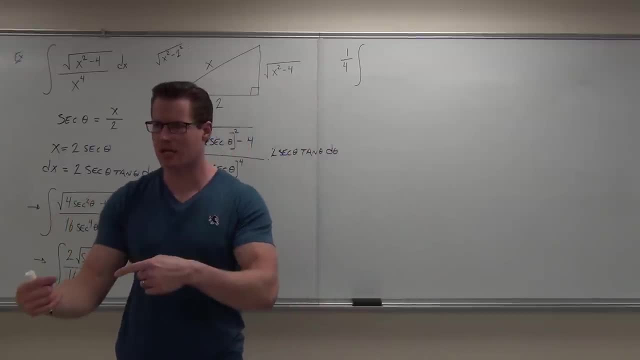 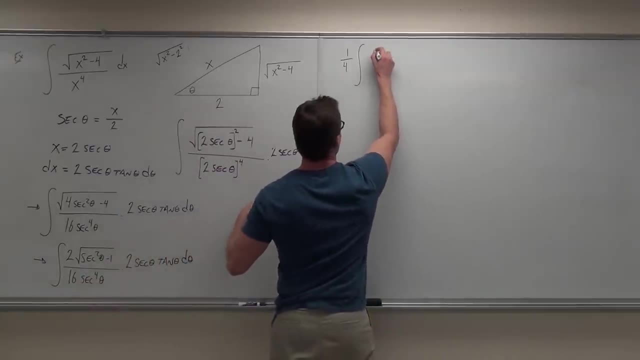 gives us just tangent. This is the whole idea, folks. That's why we're using sine and secant and tangent, because those identities are so nice for us. So we got- let's see, square root of tangent, squared theta over secant to the fourth theta. 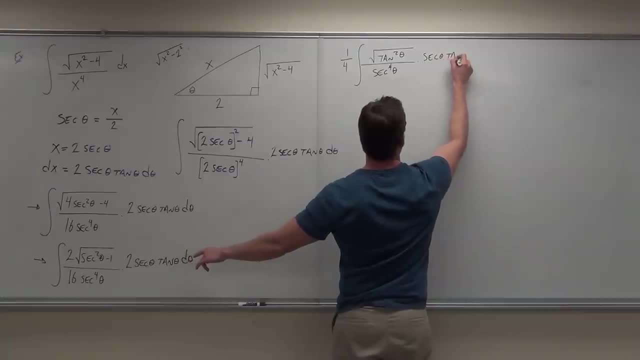 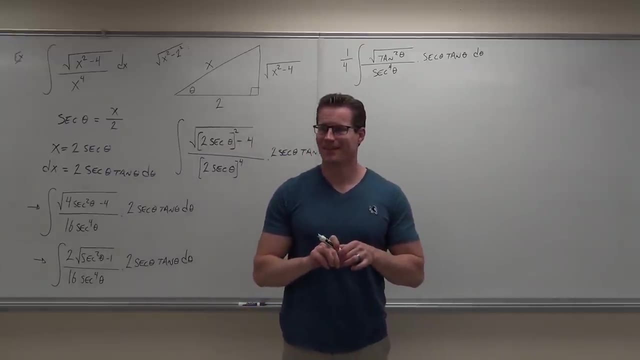 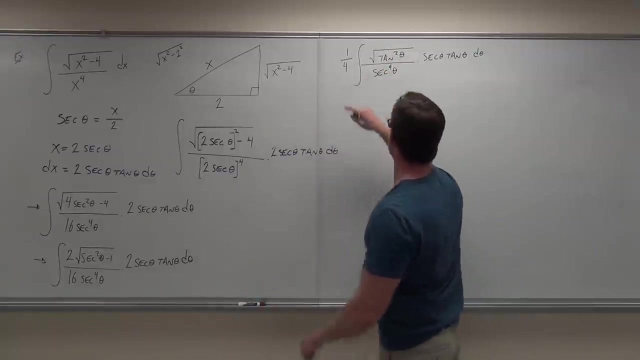 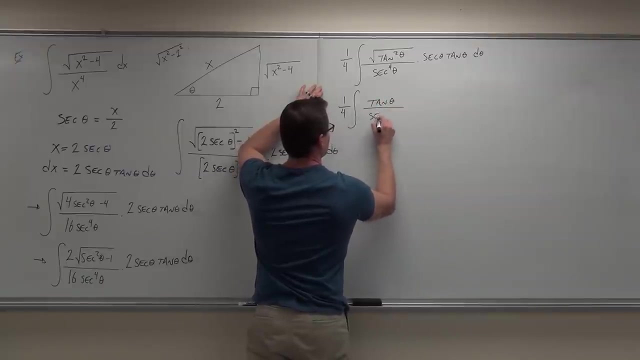 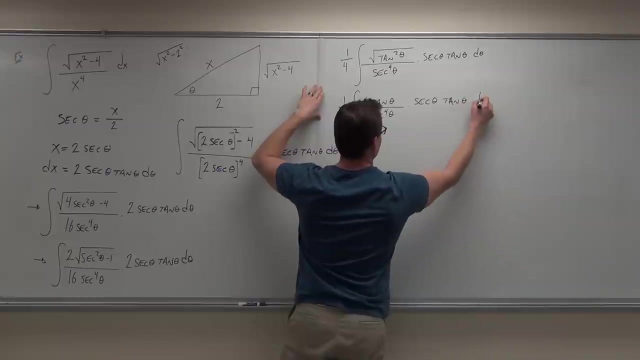 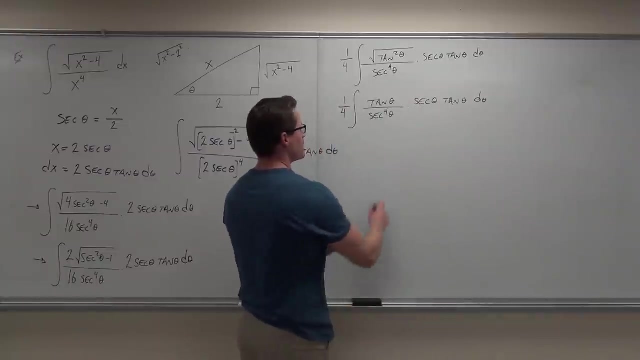 times: secant theta, tangent theta d theta. Are you all still okay? You sure What's the next thing you do? We're still simplifying. How much does this become A root of theta? What now? Let's do that. 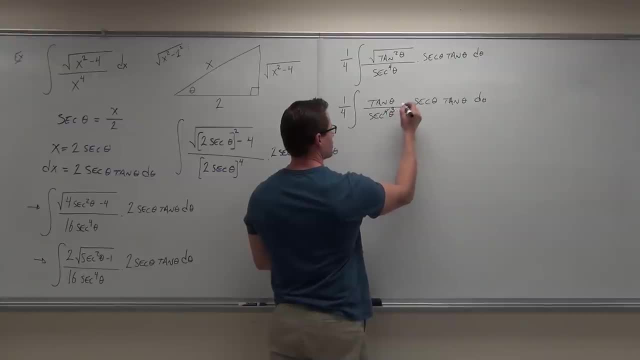 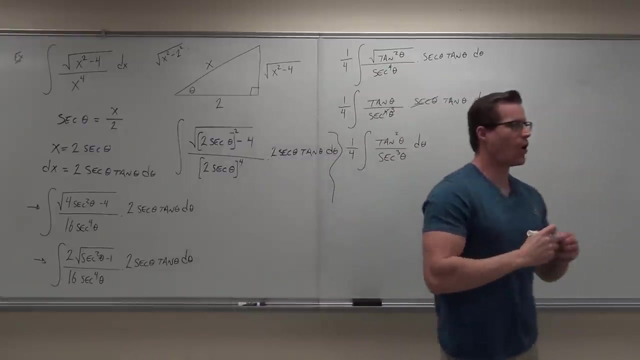 So this becomes to the third power: That's gone, So we'll have The one. fourth is still there. Yep, tangent, squared Over, secant to the third. Theta, d theta. What I want to know on a show of hands. 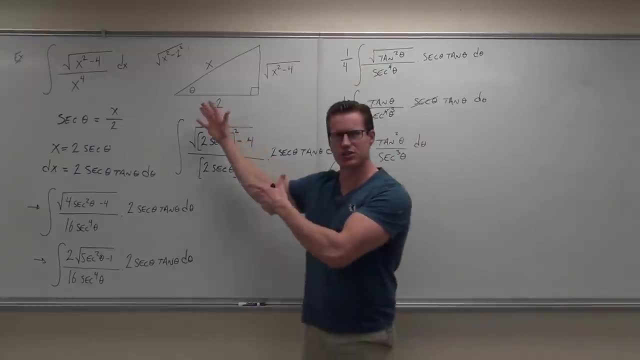 if you can make it down to that far on your own. does the triangle make sense to you? Is it starting to make a lot of sense? Can you do that? This is the idea up here, folks. This is trigonometric substitution. 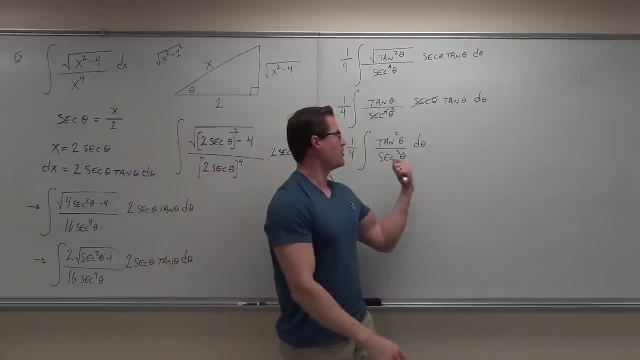 That's all it is. After you do this and you simplify it, that is your last section. Now, this is kind of cool, because we can do all of these problems. You won't be facing anything that you haven't at least seen before somewhere. 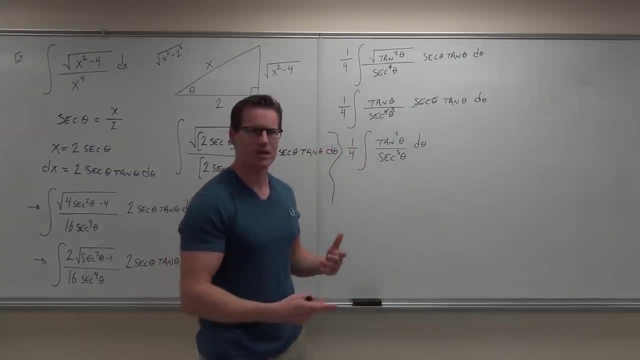 I've given you some pretty tricky ones in this class, so nothing should be above you. Okay, nothing's beyond you at this point. Now just follow the pattern. This does have tangents and secants, like I told you about, but are they being multiplied? 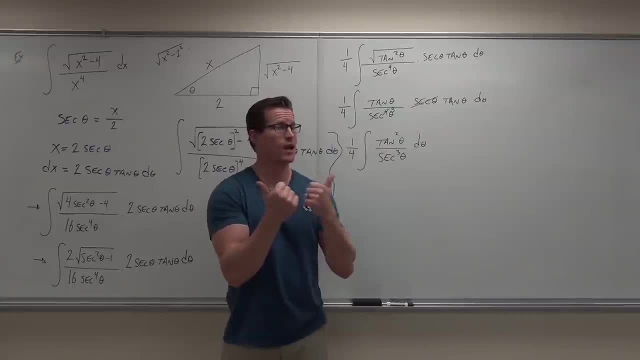 Okay, so it's not sines and cosines, It's not secant tangent, how we like it, It's not cotangent cosecant. If that's the case, then what are we doing with it? We're changing it to sines and cosines. 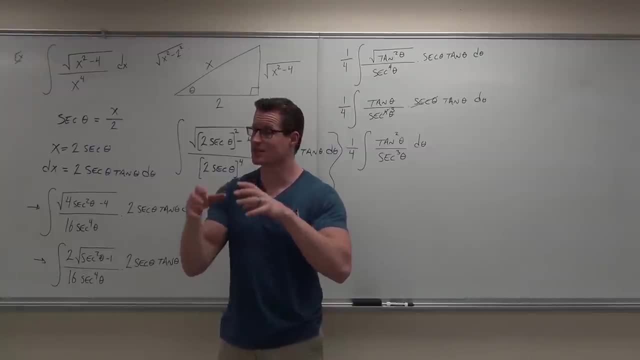 So we're going to be changing this to sines and cosines if we can. Does that make sense? If it doesn't fit, change it to sines and cosines and see what you get. Right now, there's no way I'm doing that integral. 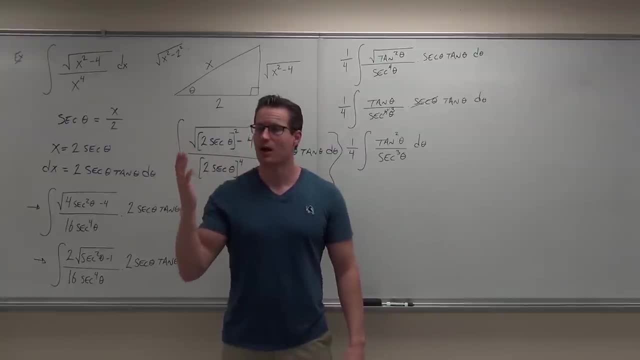 I'm looking like I have no idea. there's no way. But if I change it to sines and cosines and simplify it after that, maybe we got something. So let's try it. So, instead of 1 fourth integral of this bunch of crap, 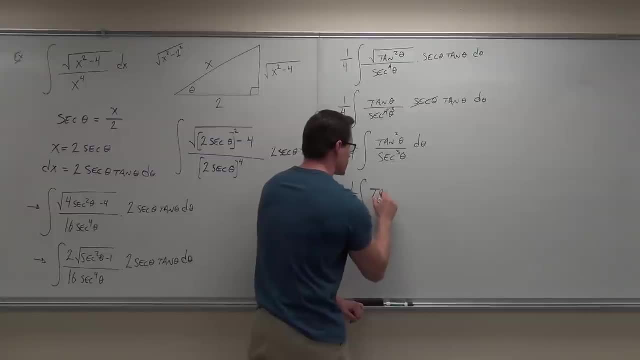 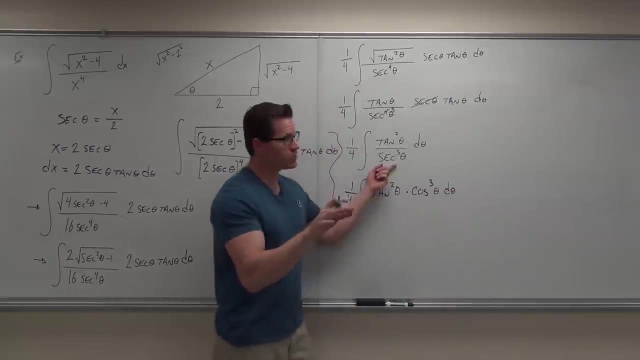 we're going to have 1 fourth this would be. I'll do this in two steps. This is tangent squared theta times cosine. to the third, theta d theta. You all should be okay that one over secant cubed is the same thing as cosine cubed. 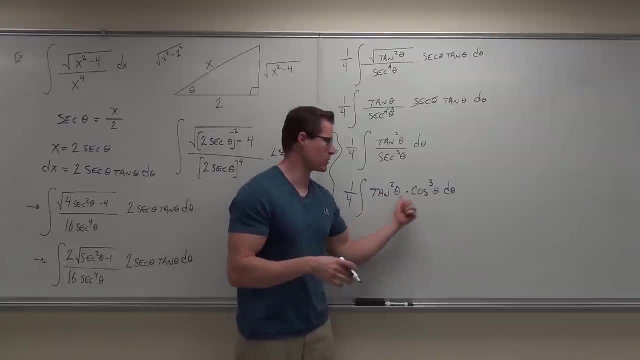 Yes, no, Yes, Keep going. I don't know anything that deals with tangent and cosine to you. Was that in your trigonometric integrals from last section? No, we didn't have tangent cosine, We had sines and cosines. 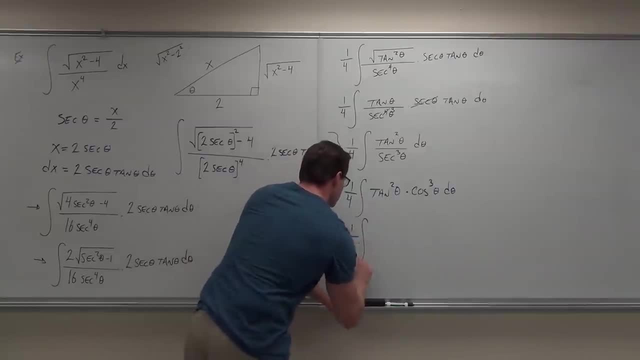 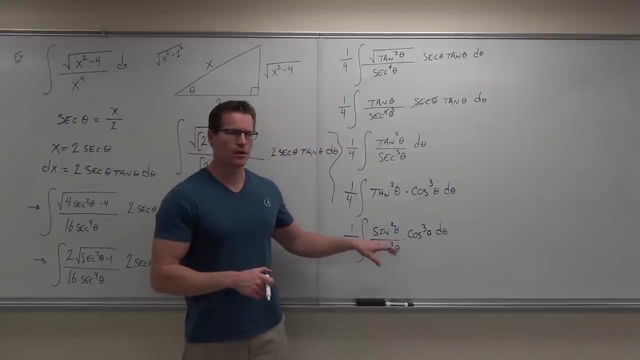 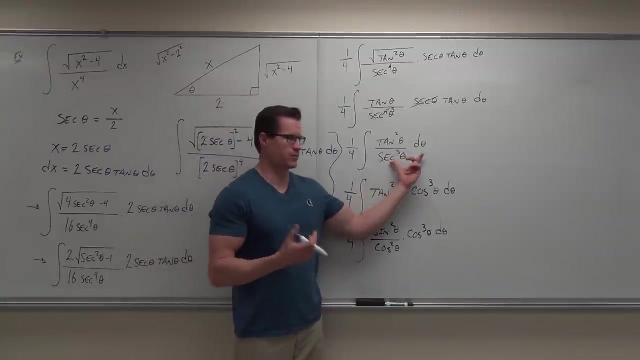 But if we do this, if we know that tangent is sine squared over, cosine squared theta, you okay with that one? Yeah, Do you see how changing things in the sines and cosines can really help you sometimes? Otherwise, man, you get stuck. 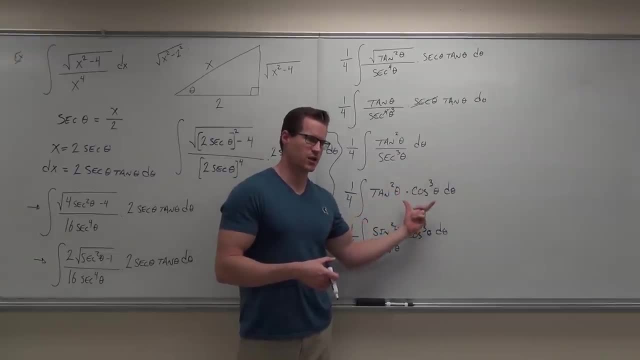 What am I going to do here? Substitution ain't going to work. Try changing it in sines and cosines. Once you do that, maybe you get lucky and get something that you can really work with Here. this is really nice. 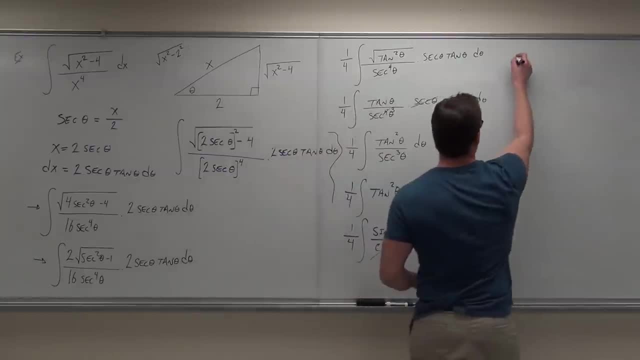 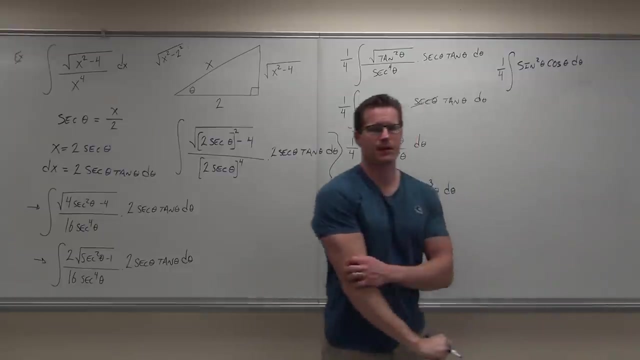 Those are gone. All but one of those is gone. We have integral. sorry, I forgot the 1 fourth. 1 fourth integral of sine squared theta, cosine, theta. Now take a look at it. What would you do if you were doing this problem? 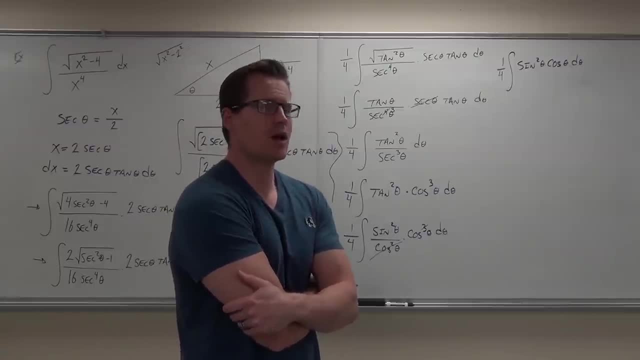 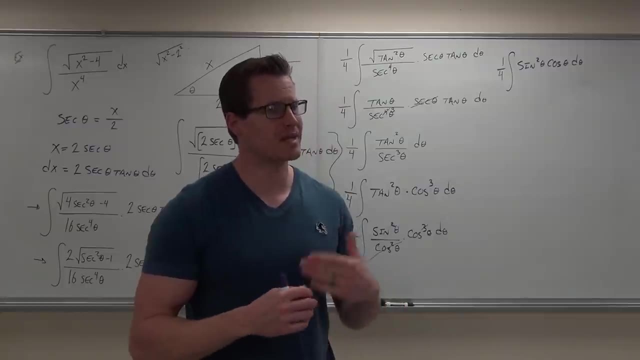 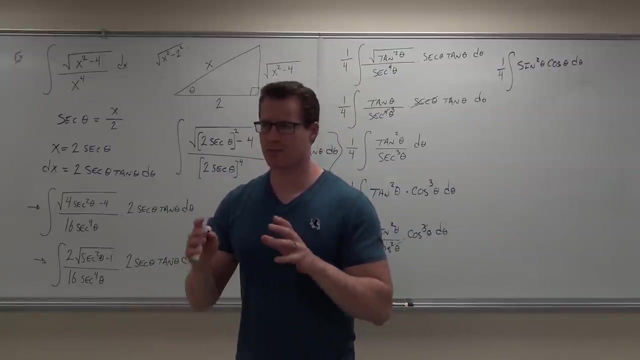 Use of substitution. I would do use of, for sure. Just remember, listen, this is a perfect example of go through the patterns that I taught you. Do not immediately jump to one technique or another. Honestly go through. The easiest thing you can do in integrals is well. firstly, it fits the table. 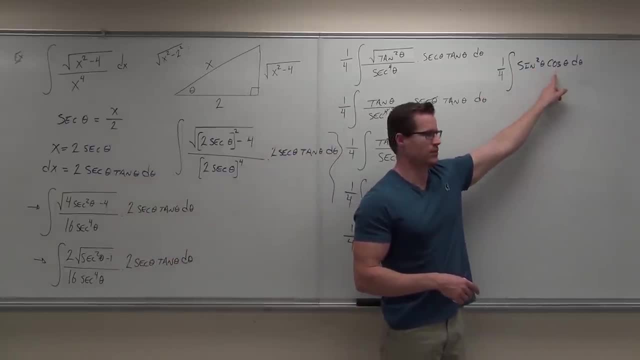 So we check it. Does this fit in integration table? Yeah, No, it doesn't. Can you do a substitution? Yes, Yeah, Then for heaven's sakes, don't start doing identities and stuff if you can do a simple. 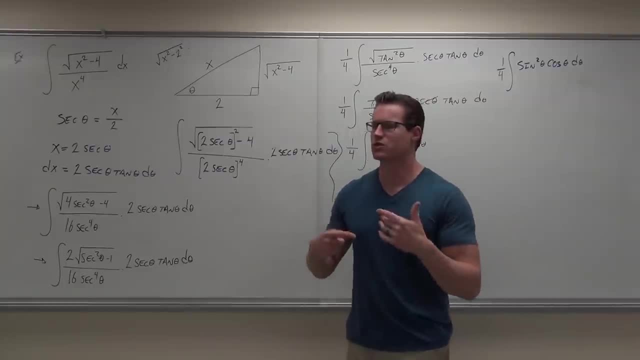 substitution. Does that make sense to you? So what I'm trying to get you to do is really think through these. Don't jump to a certain section because we're in it. Really think it through. We start here We go: hey, can we do it like it is? 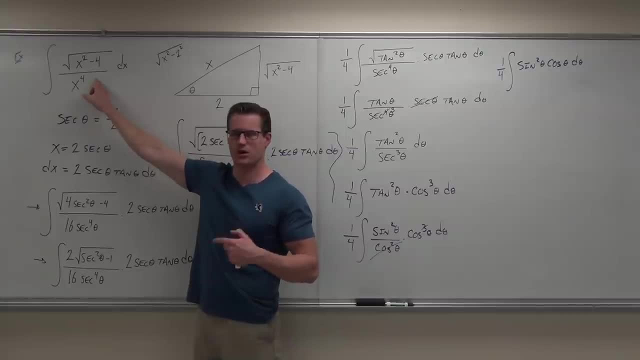 No, Can we do a substitution? No, Is it trigonometric? No Integration by parts. No Trig sub. Yeah, Do a trig sub. That's what your trigonometric functions are. After that, does it fit a substitution? 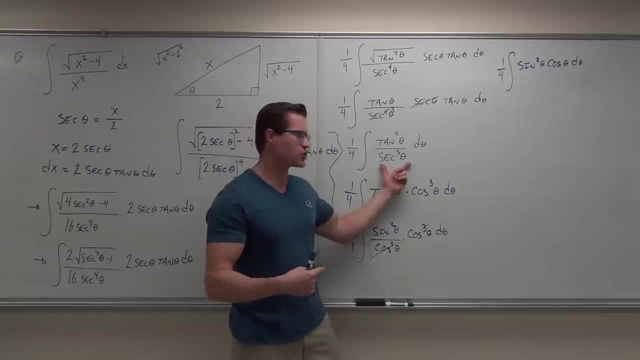 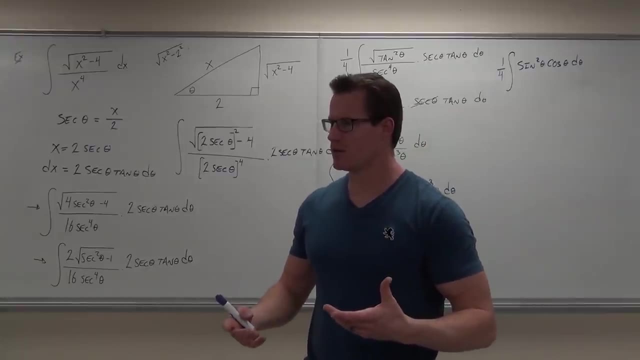 No, Does it fit any of the trig models that we have? No Change the size of the cosines. Can you do a substitution? Notice how I'm always going back to. can I do a substitution? Are you listening? We're always doing that. 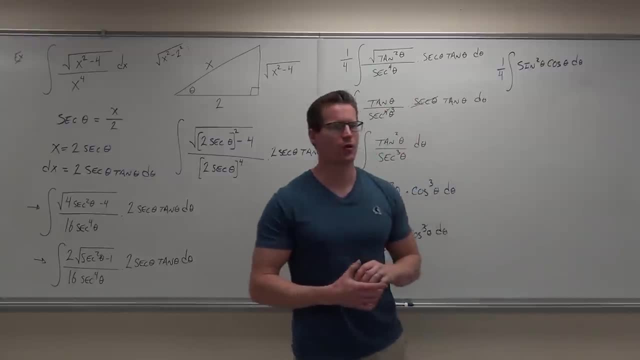 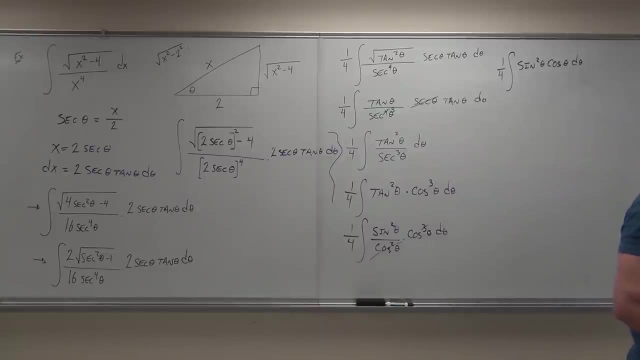 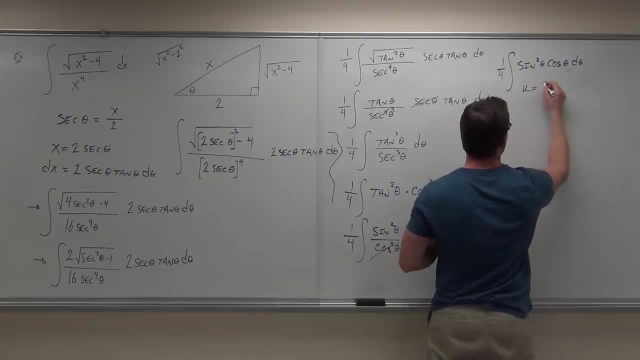 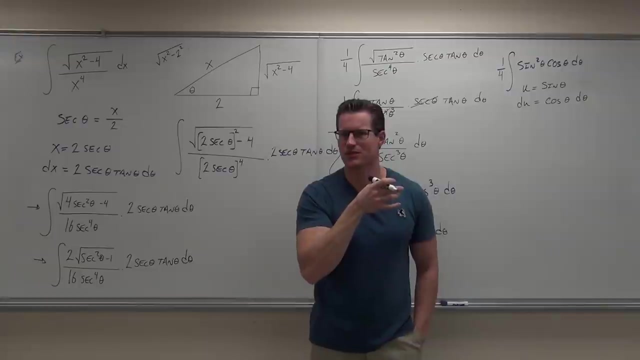 Ok, so I'll do q and d. What would I do with myprotection of xi? Huh, Aren't you glad we did a substitution? Couldn't you use an identity or something? Oh, that's silly right. If we used the identity, we'd have 1 minus cosin squared, wouldn't we? 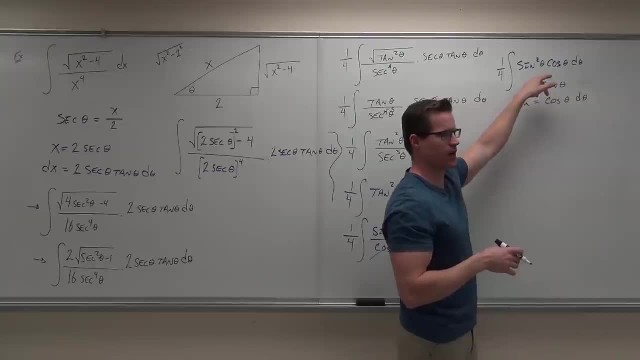 Then you distribute. So if you have cosine, don't do that. What we want to have is sine with one power of cosine off to the side If we have that already. this is the whole idea from the beginning. right, Make a substitution. 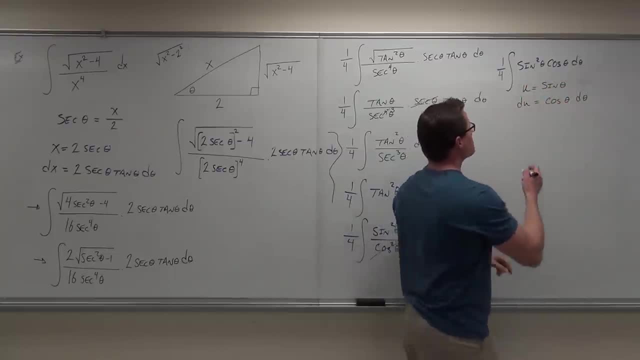 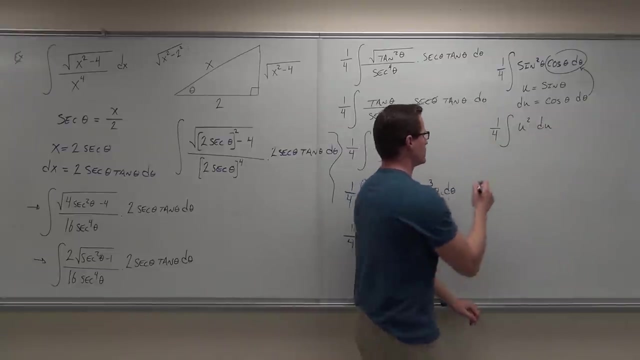 Substitute for sine cosine. theta d theta's right there. So we know this is gonna be one fourth integral of this piece is our du. So this is gonna be. what was it? U squared u. How much easier can we get? Just don't forget about the one fourth. 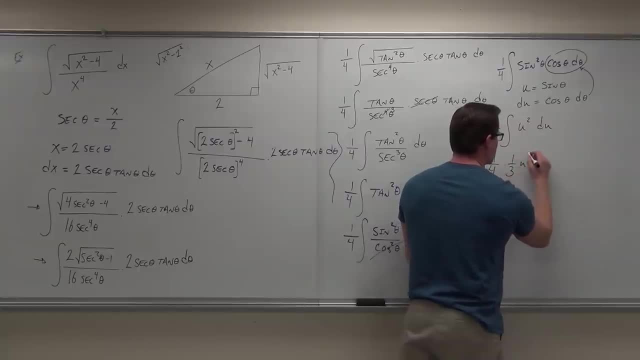 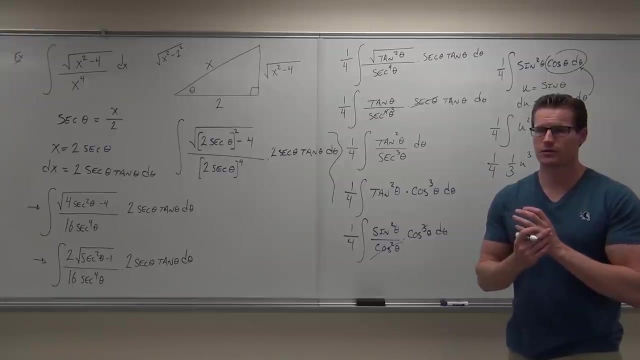 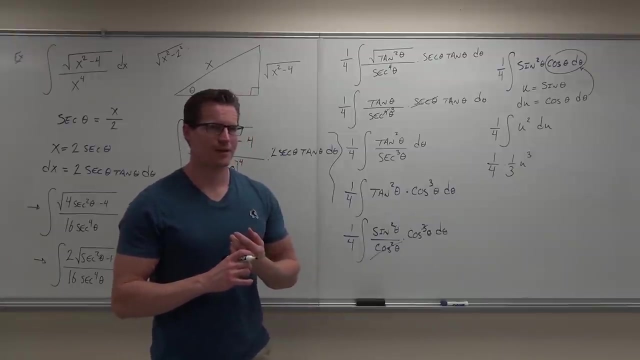 that follows all the way down. This would be one third u to the third. Still okay, so far. Okay, Now are we done? No, Almost done, almost Okay, we're gonna simplify. Sure, we're gonna get one twelfth. 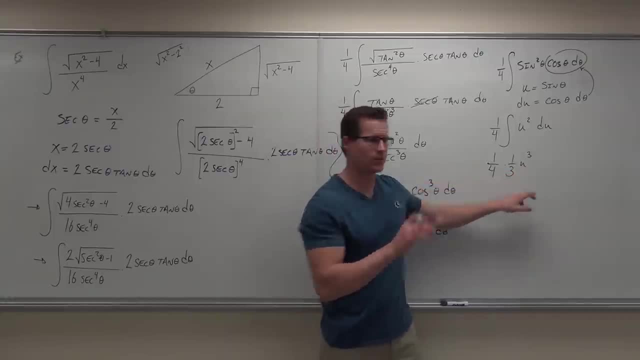 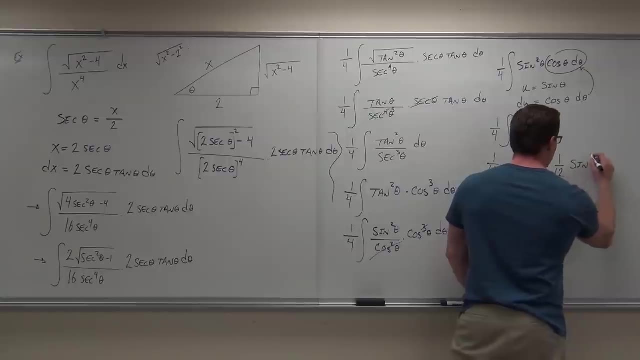 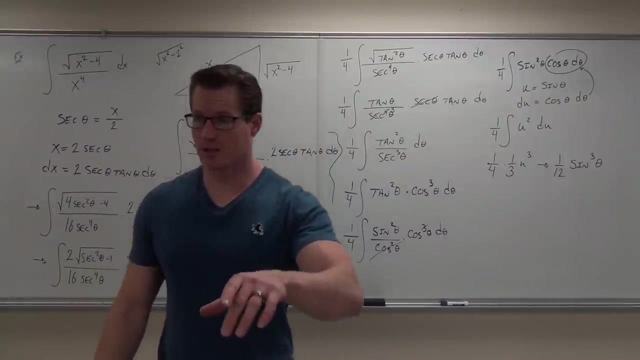 Do we keep the? u? No, What's the? u become Sine. Okay, we're gonna have a couple things to do here, So this becomes one twelfth: sine cubed theta. Very good, sine cubed theta. Now we've already substituted once. 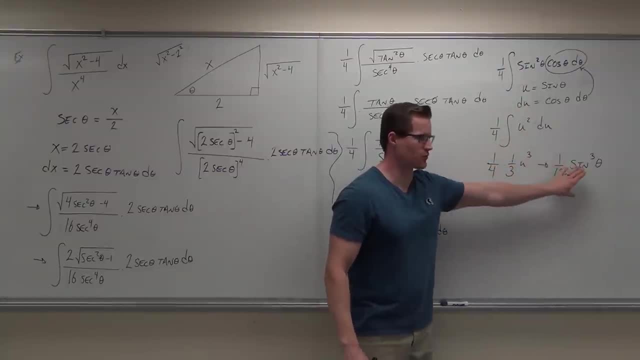 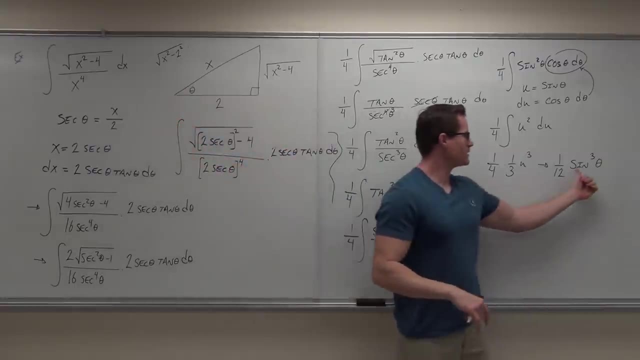 because we had one substitution here. We're done with that. We got it back in terms of theta. Look back at our integral. Back at our integral. Did we start with thetas? No Xs. So now that you have sine theta, 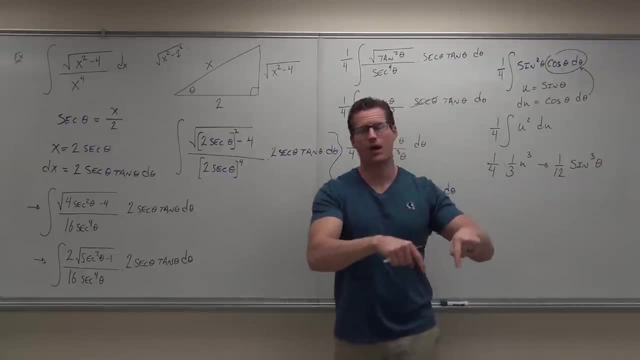 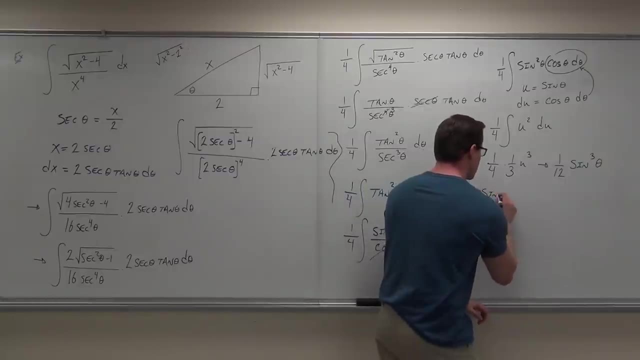 can you make that back to xs? Where are you looking right now? Triangle, Use your triangle. Everyone should be able to do this. Go ahead and do it right now. Make sine theta equal to something and then use that substitution. So I want something right here. 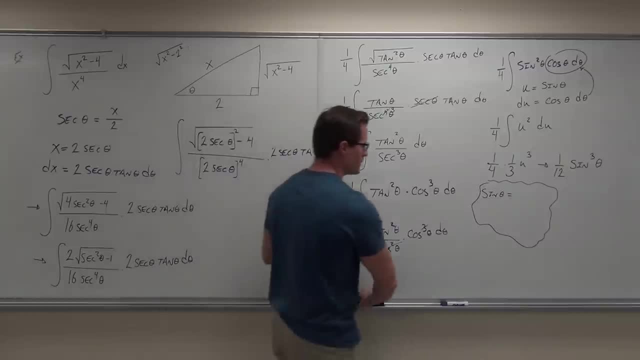 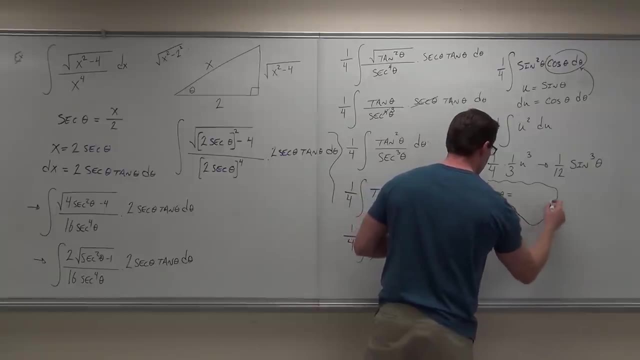 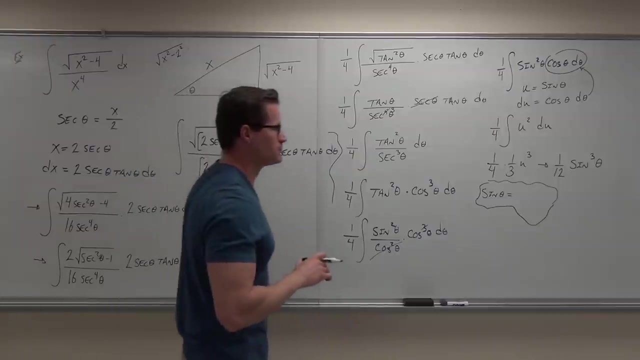 and then I want you to substitute. That's it. We don't even need that big, So it becomes sine minus sine, minus sin. What relationship is sine? what over what? Opposite or hypotenuse? Opposite or hypotenuse? 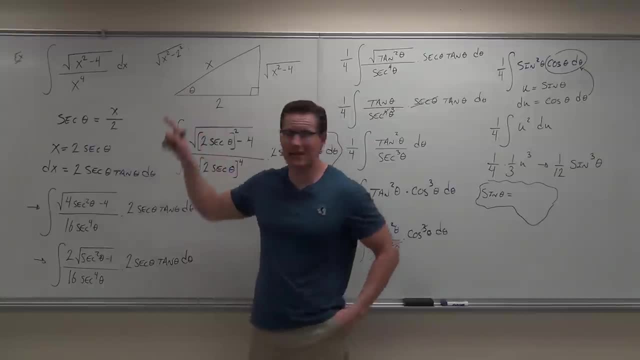 Do you have an opposite? Yes. Do you have a hypotenuse? Yeah, Notice, it's based on that theta. This is exactly what we're talking about here, so hopefully you should have the square root of x squared minus four over. 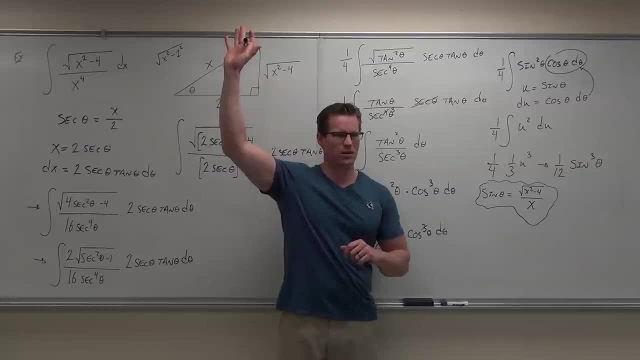 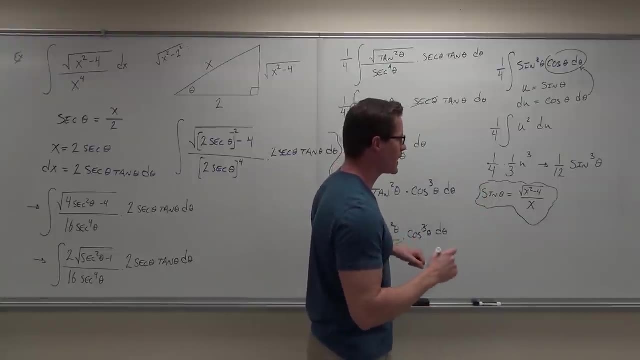 X, X. Did you all get that one? How many people did get that one? That's great. that's almost everybody. that's fantastic. So one last little step that we have. We've got a 1- 12th, we've got a sine to the third. 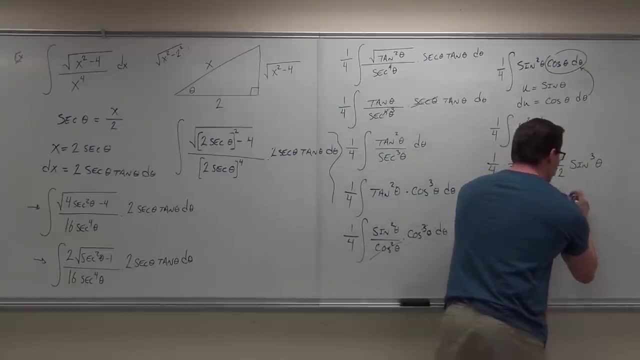 So basically, all this stuff is being raised to the third power. So we get a 1- 12th, we get a square root of x squared minus four to the third and we get an x to the third. Are you guys okay that both of these? 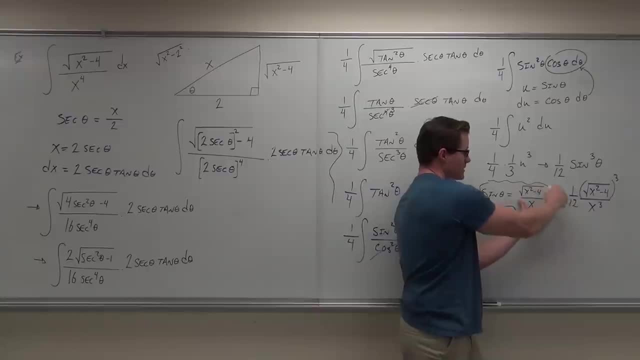 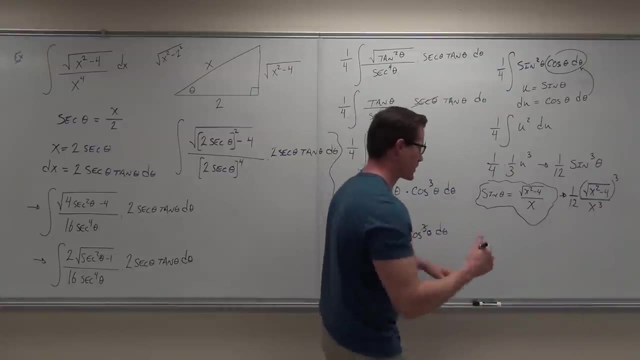 are gonna be raised to the third power. It's sine to the third, so this is sine theta to the third. both numerator and denominator gets raised to the third power. If you want to make it just a little bit nicer, it's really kind of up to you. 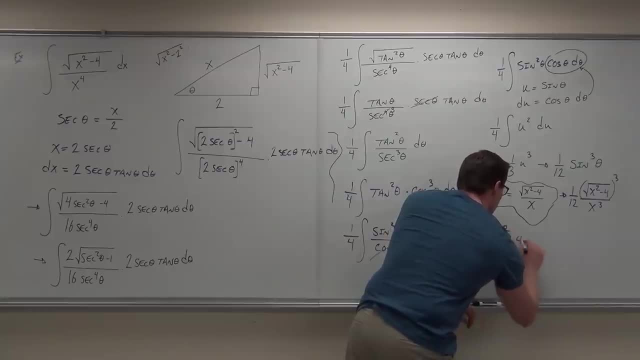 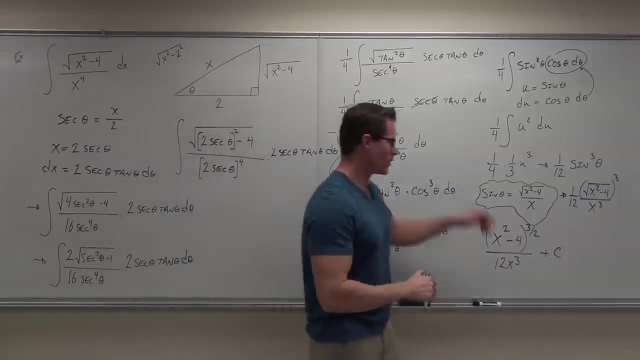 I might choose to write this as this, Because that's how we were given. Do you see that how we were? Oh, sorry, that was a previous problem, My bad, Whatever you want, You can leave it like this. you can write it like this: 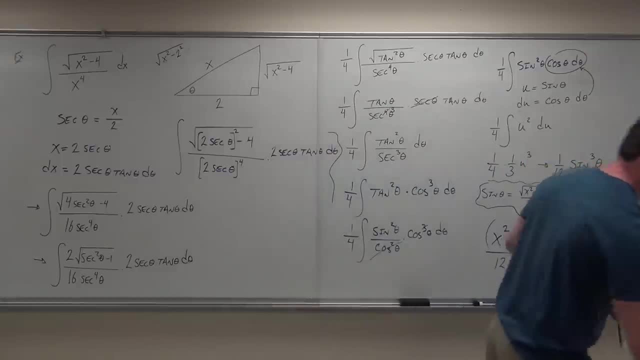 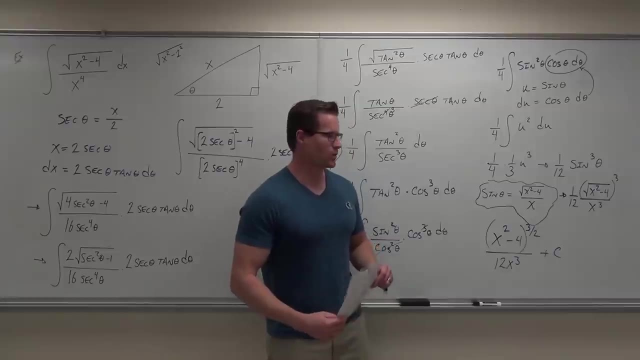 I really don't care Plus c, That's how I know I'm done. I never stop at integral until I either have the number, if it's definite, or I have plus c. I need to show of hands if that made sense to you guys. 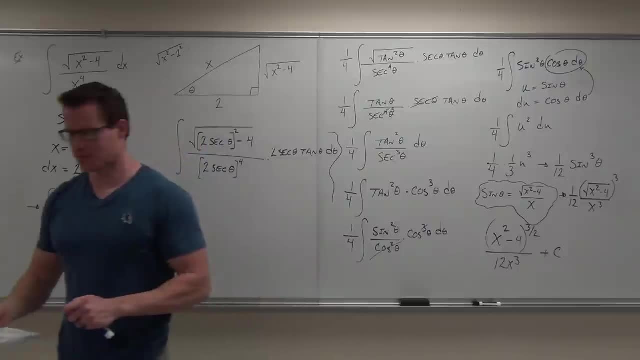 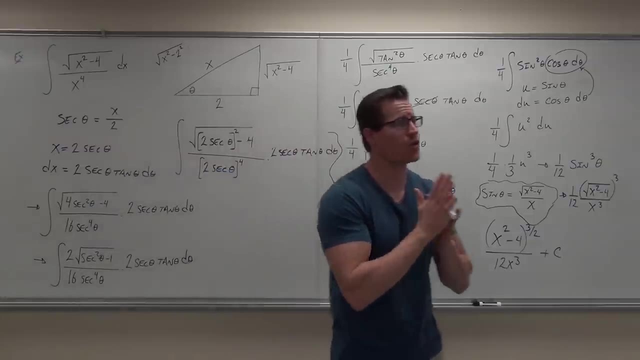 Good deal, all right, fantastic Question, Any questions? We're gonna start our last problem of the section. We're gonna get through the first little piece of it and then I'm gonna ask you to do most of it. You can do most of it on your own. 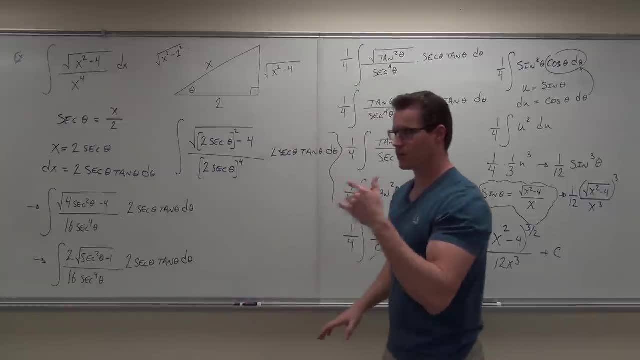 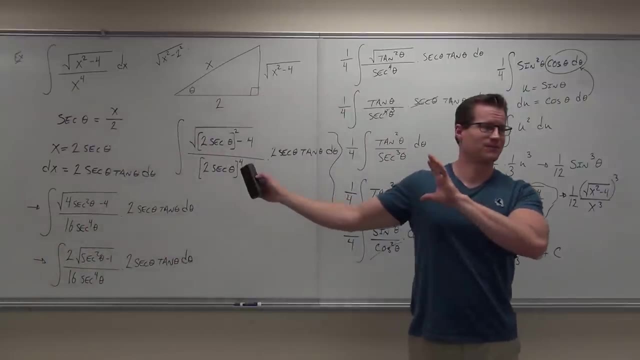 I think you can do it on your own, So we're gonna do the first part though, because the first part is a little tricky and I want to make sure you see this at least once. Last chance for any questions at all. 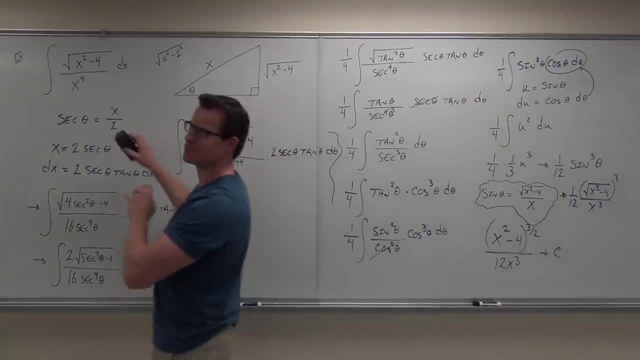 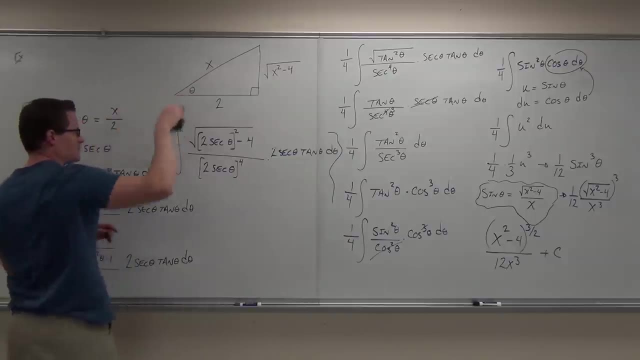 Michael, One word, two dates and the other. No, no, no, just for simplification purposes. before you erase it, that one right there under the triangle. can you turn that into like a two square and then get rid of the radical event? 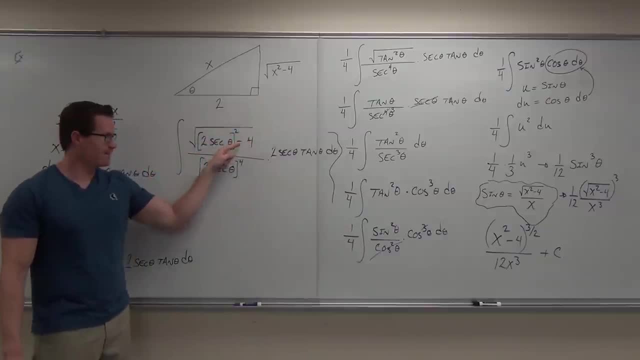 Let's write down one more Down, one more step. That step Right there to get rid of the radical. can you turn that into a two square? This one, Yeah, you can turn that into a two square, but there's no way that's gonna simplify that square root. 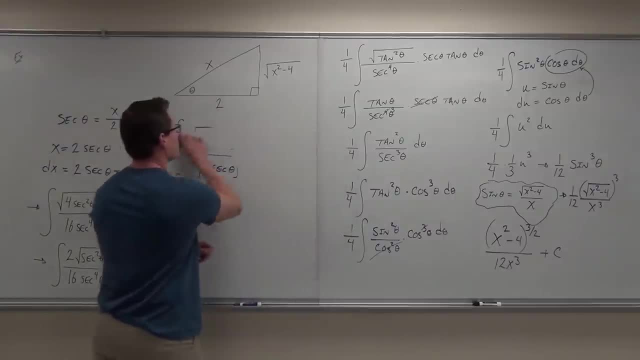 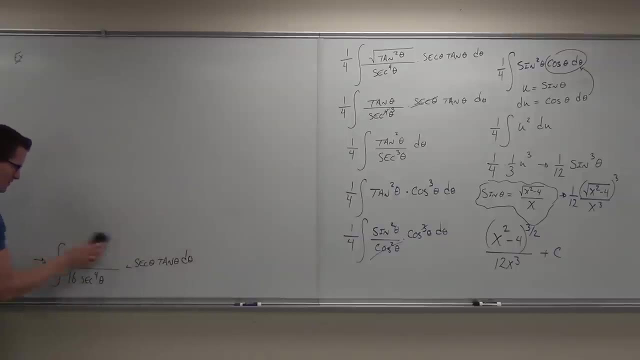 No, All right, Cool, Don't make up your own math. Never a good idea, unless you're Isaac Newton Who invented this. Are you Isaac Newton? I'm not, though. Oh good, You got some advantages now that you're a mathematician. 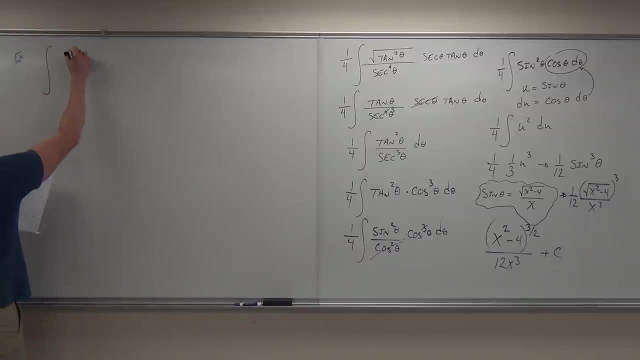 I'm not, No. I'm not, No. I'm Valentin Making my own math. That would be awesome. He's Cupid, He's Cupid. Oh yeah, Back to the work, Valentin. 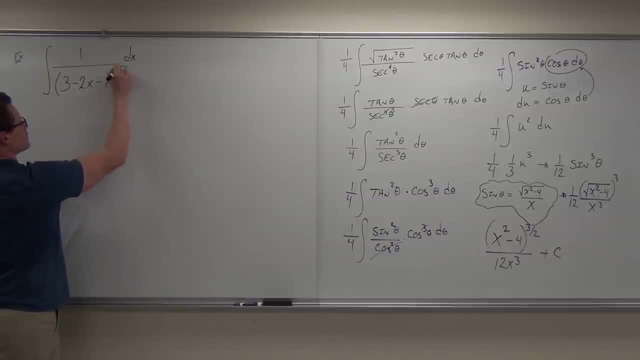 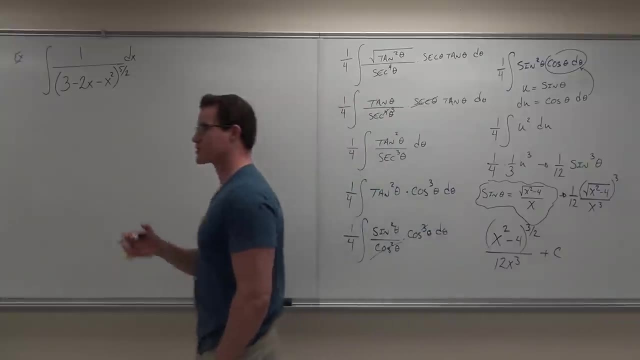 Valentin, Valentin, Ooh, ooh. OK, I think we can agree that looks nastier than some of the other things that we have done so far. So What is this? First things to do, first thing, I know it's fun, right. 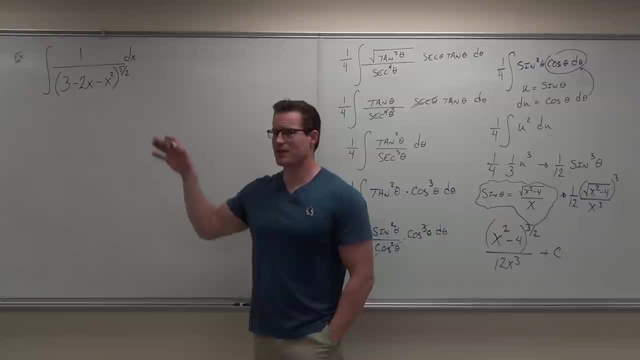 First things to do: go through your whole process. Does that fit the integration table? Heck, no, No, it's not even close. Okay, do substitution No? Do you understand that? every time I see an integral- and I've been doing this for years- that's what I do. 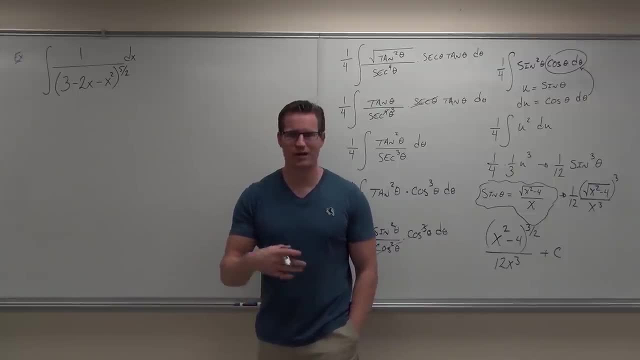 I'm not just following you down a rabbit hole. This is literally what I do, So I'm trying to tell you this is the best way to do it. I don't think I've done an integral wrong in a really long time, Really long time. 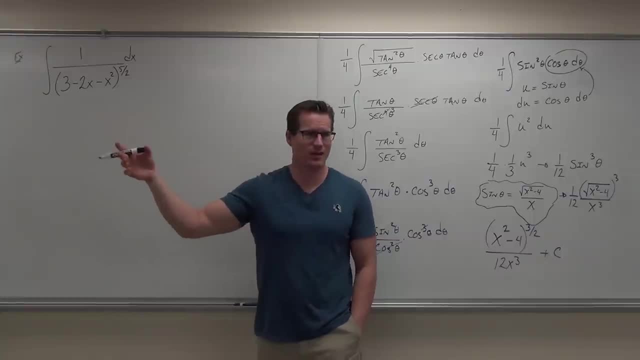 But this is what I always stick with. that pattern, I think. does it fit the table? If not, okay, go to substitution. If not, I'll write integration by parts. That's not going to work here. I don't have a product. 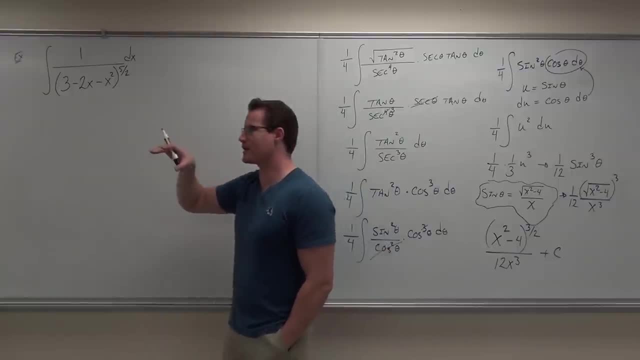 All right, if that doesn't work- or I don't have anything that will work with an L in here- If that doesn't work, does it have trig in there? Well, no, not yet Can I fit it to something that has trig in there. 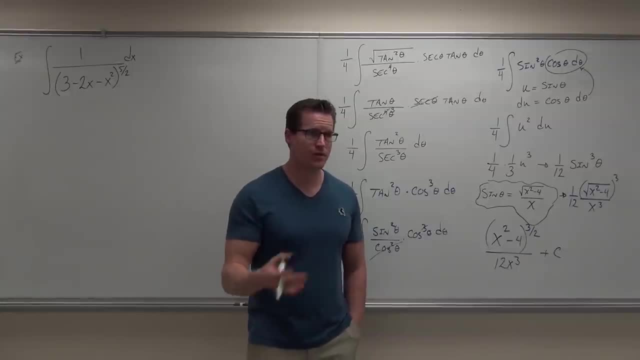 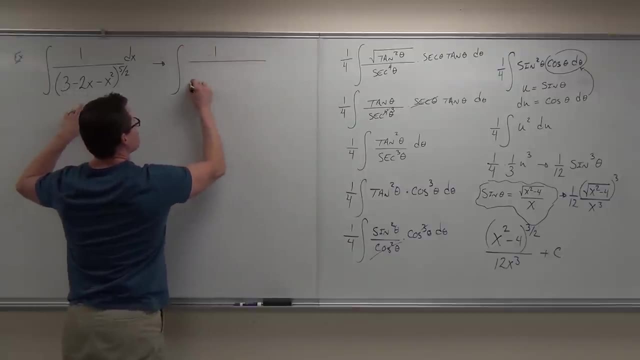 Maybe Does it have a square root. Yep, That's a good indication that I might be able to do that. So I'm going to write this, just for my own mental well-being, As a square root to the fifth power. Don't forget that fifth power. 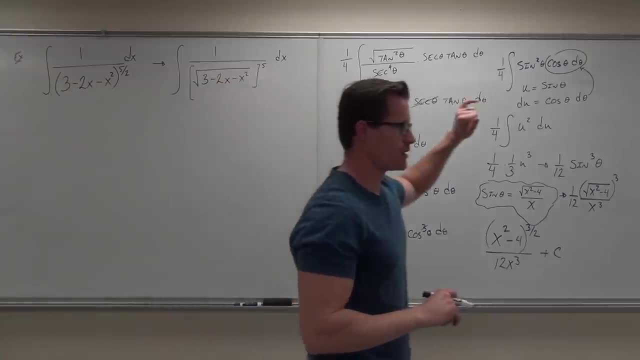 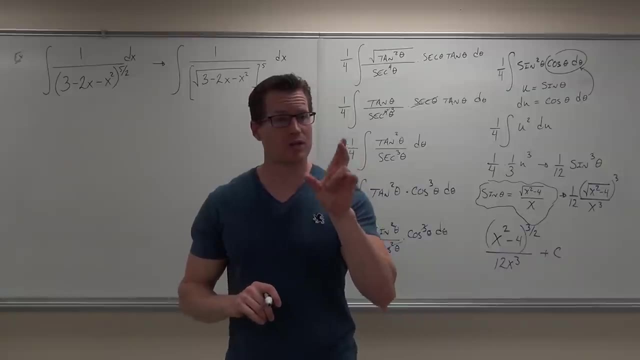 Now here's the issue. This part sucks Because that part right now does not look like a right triangle. Does that make sense to you? It's not something squared plus or minus something squared, And that's what we need for a right triangle, for Pythagorean theorem. 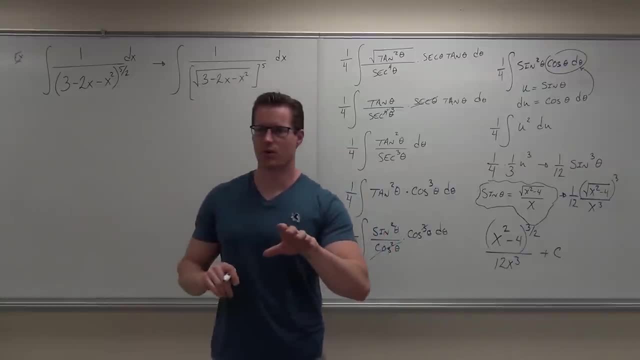 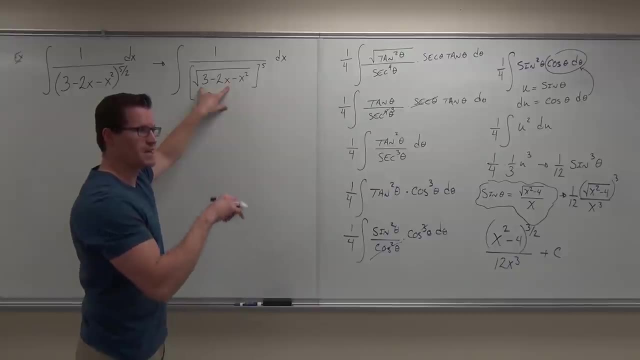 So the idea is if this- listen carefully, please. This is the whole thing. This is the whole, whether you're going to get this right or wrong. If this does not fit something squared minus something squared- you make it fit something squared minus something squared. 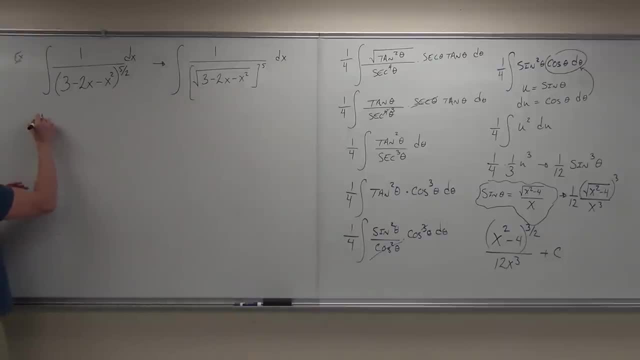 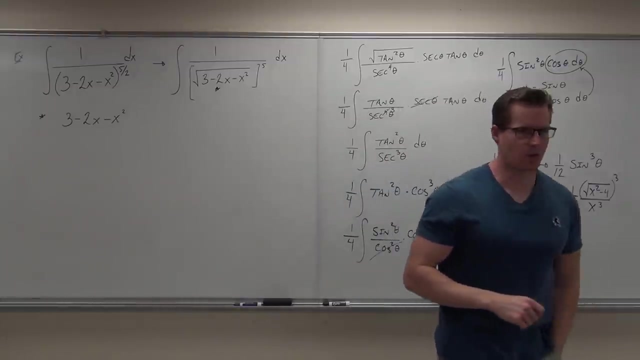 Or plus something squared. So we have- let's take this off to the side your little asterisks- Three minus 2x minus x squared. Take a look a little bit more closely at that one. You ever heard of completing the square? 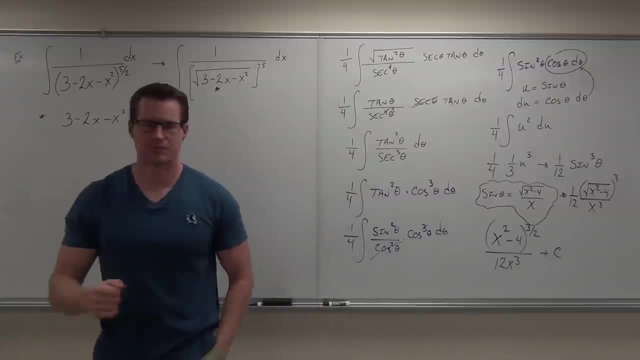 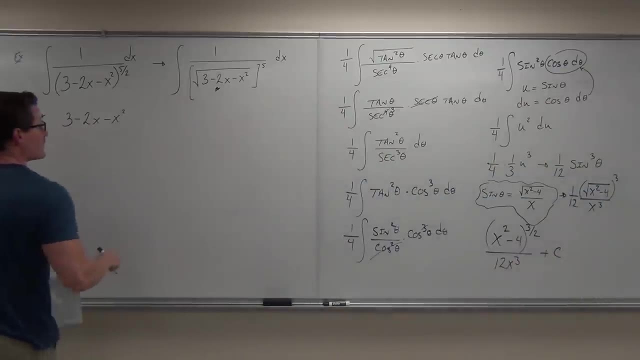 Yes, We're going to complete the square, We're going to make this thing be a perfect square. So how in the world are we going to do that? Well, the first thing you might want to do is have this thing in order. 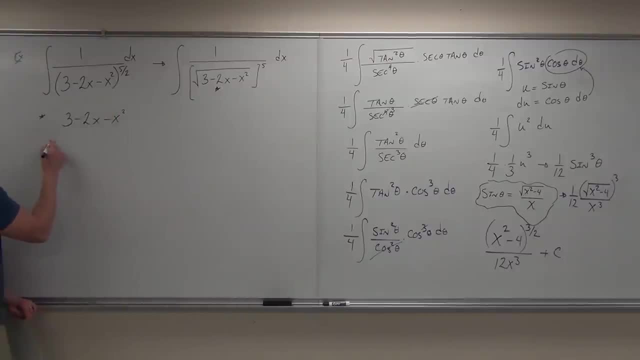 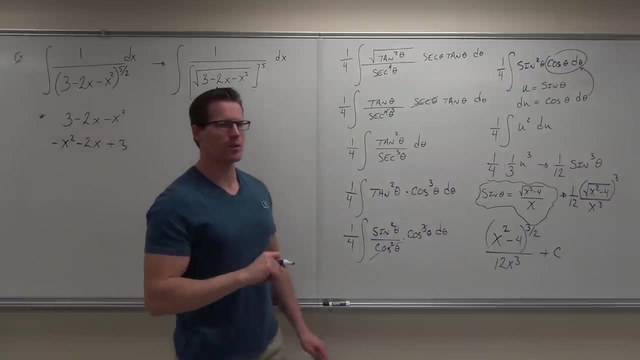 Because that's how completing the square works. So we'd probably write this as negative x squared minus 2x plus 3.. You with me on that one. By the way, these are special cases. This is not going to be true for all the ones that look like this at all. 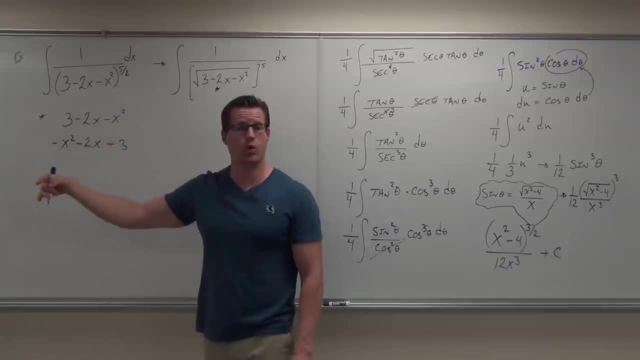 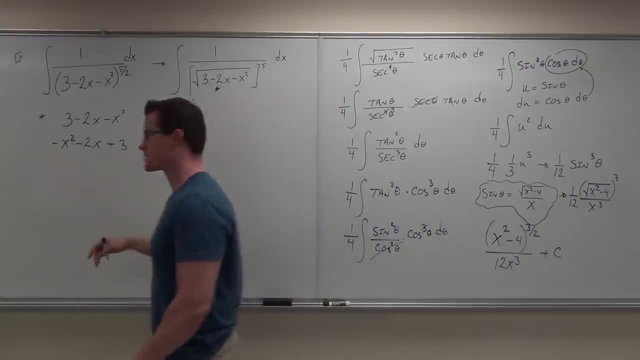 These are special cases That you can actually complete the square and it didn't work. So not all of them. you can do this universally. I'm giving you special ones here. Does that make sense to you? Okay So, but this one, we're going to see that this will. 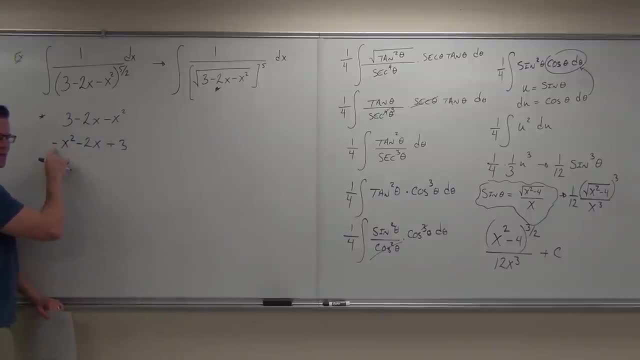 Next thing you do, you make sure that first term's positive. That's got to be the case. So what I'm going to do is I'm going to factor out this negative here. I'm going to have x squared plus 2x. 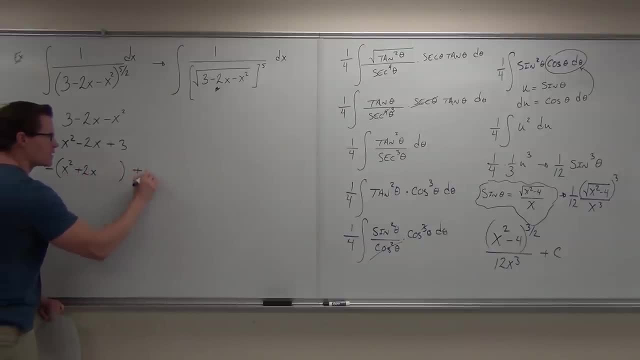 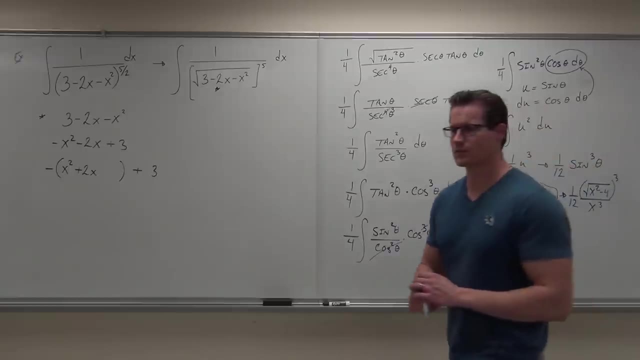 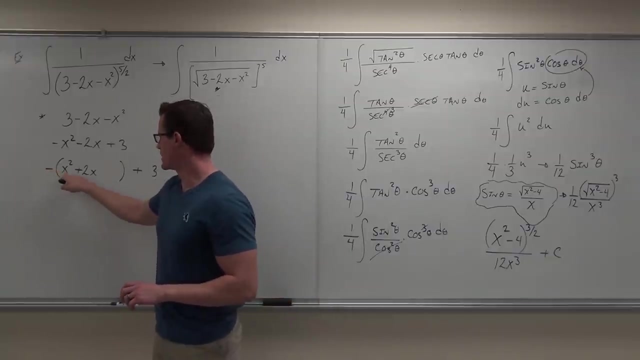 I'm going to leave some space here. I'm going to leave that plus 3.. You'll see why It's completing the square, You guys. okay with that one. So notice, this is negative x squared. This is minus 2x, but the plus 3, I'm leaving that alone. 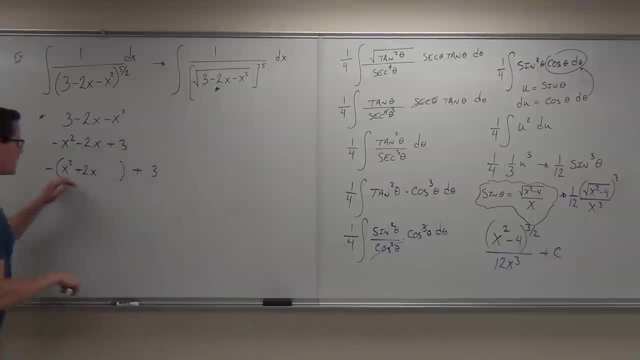 You follow. Now how do you complete the square? You have your first term, positive. You don't worry about this right now. You look just in here. We take the middle number, the middle coefficient, which is your b a plus b. sorry, 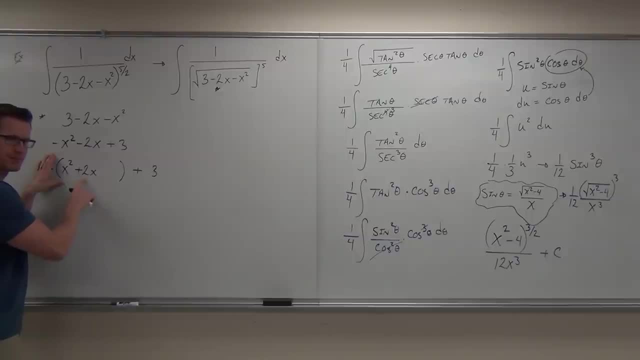 a x squared plus b x plus c. Take half of it: Square, Square, Square. Add it Now. whatever you do here, you have to also undo it, Otherwise you're changing the value of this thing. Does that make sense? 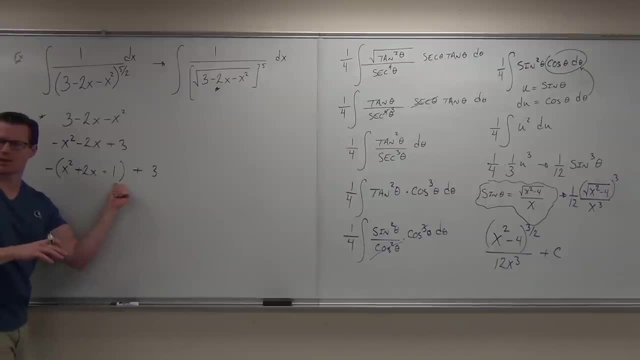 But watch real carefully. First of all, you guys all okay with where the 1 came from. That's kind of a big deal. It's completing the square, So we go, hey, take half of this number and square it, add it over here. 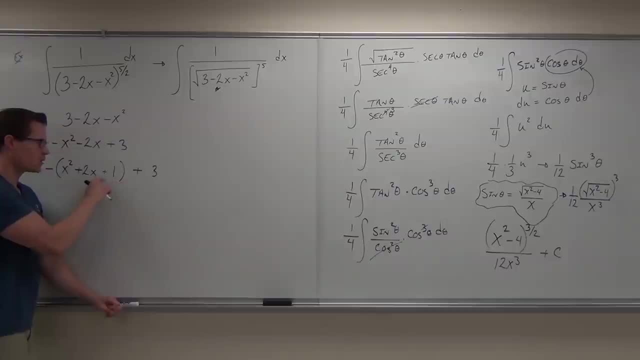 Now you have to undo what we just did. I know it says plus 1, but watch carefully. We really see how the negative's going to distribute. We really subtracted 1.. To undo that: we're going to add 1.. 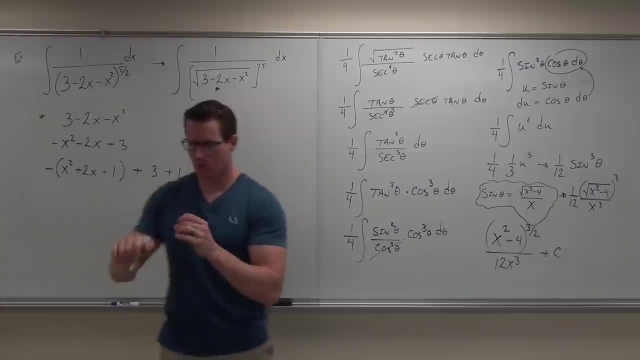 So are we adding 1 twice? No, we're not. We're adding 1 here because, really, when you distribute, you subtracted 1.. Notice how this is going to be a minus 1? Minus 1 plus 1 gives you 0.. 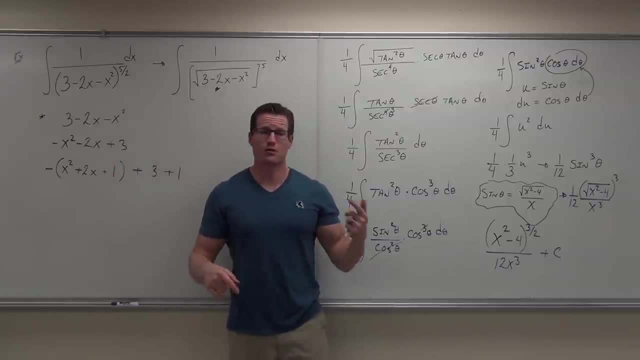 These black letters should be gone if you were to distribute this. So if you want to check your work, if you distribute this and combine like terms, do you understand that it's going to give you this back again? It's going to be the same thing? 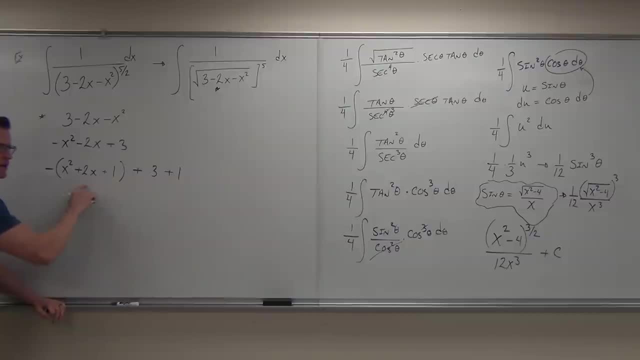 What we've just done right here is: we've completed the square, So this becomes negative x plus 1. squared, This becomes plus 4.. You guys, all right with that one, Complete the square. If you do this, you automatically have a perfect square. trinomial of factors. 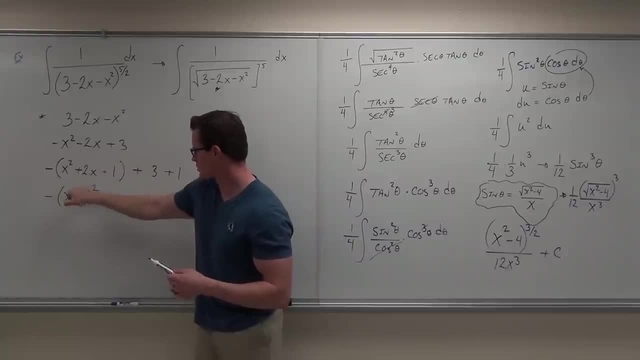 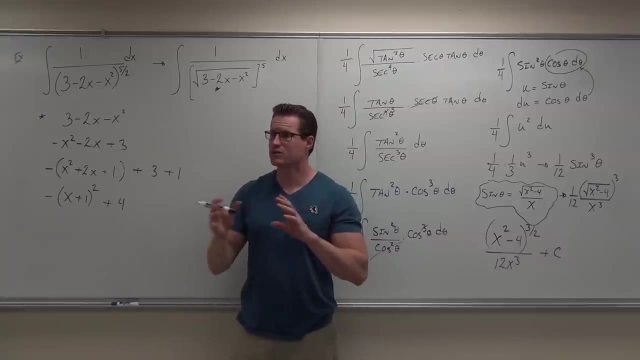 Negative. we kept that up front. This is x plus 1 squared. This is plus 4.. Show of hands. if you're okay with that one, Write it in the appropriate order. We want something squared, minus or plus, something else squared. 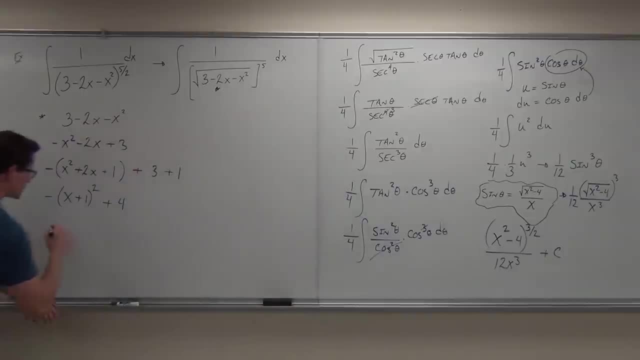 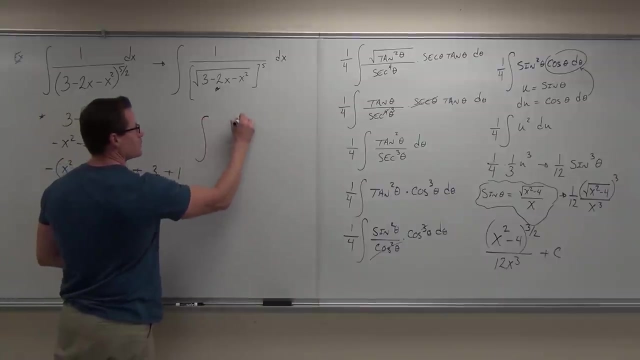 This doesn't cut it right now for that negative, So I'm going to rewrite this as 4 minus x plus 1, squared. Now, working back to our asterisks. You guys, all right with that one. We've got a 1,. we've got a square root. we've got a nasty 5th power. we've got a dx. 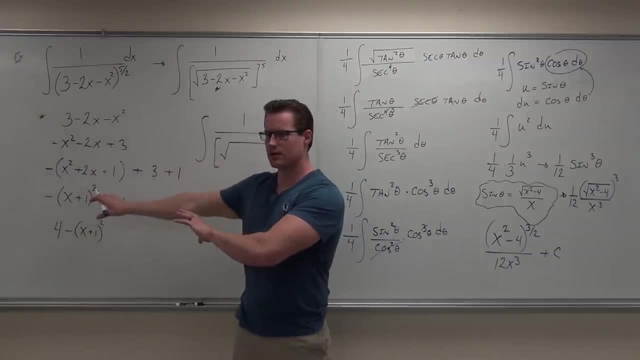 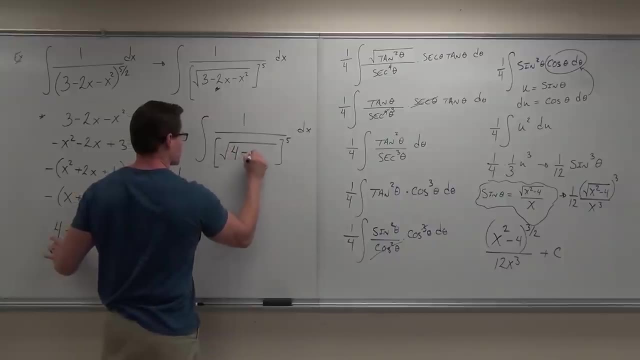 In there. watch carefully. First of all, are you guys okay with completing the square idea? No, Look at what happens to us When we plug this back in. we've got 4 minus x plus 1 squared. Do we have something squared plus or minus something else squared? 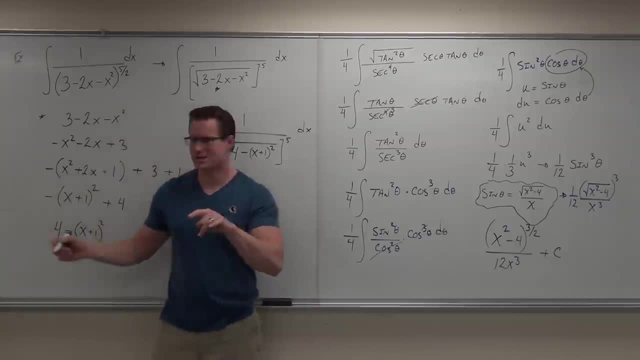 Yes, Notice why it's a special case, Because If this was like a 5, it'd be kind of difficult to do. You can still do it all right, You could, but it'd be a little bit harder. I think you can do it. 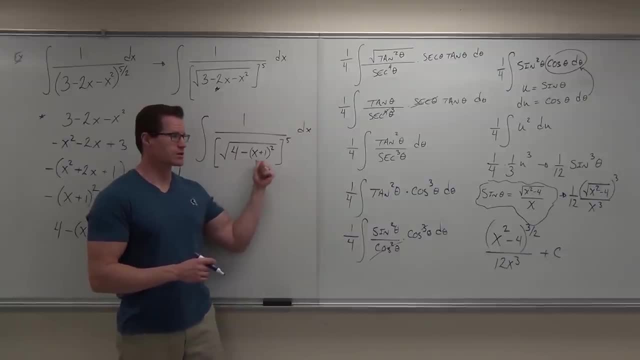 I don't remember now, I'm pretty sure, But this is nice for us. This will be really good. Here's the next idea. I'll give it to you right now, because I want you to do this on your own at home, okay. 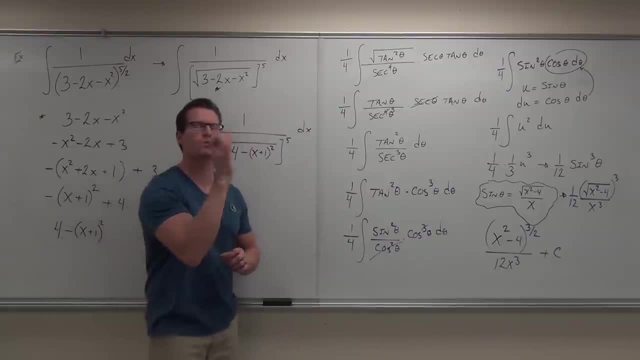 This is for you to do. You need this completed by the time you come back to class, because I'm going to rip through this thing next time in about 5 minutes. Do a substitution right now. Get rid of the x plus 1.. 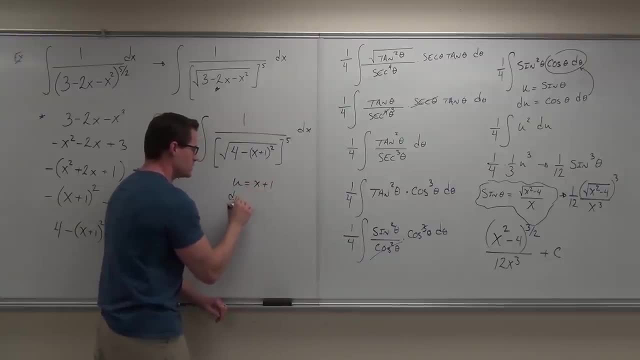 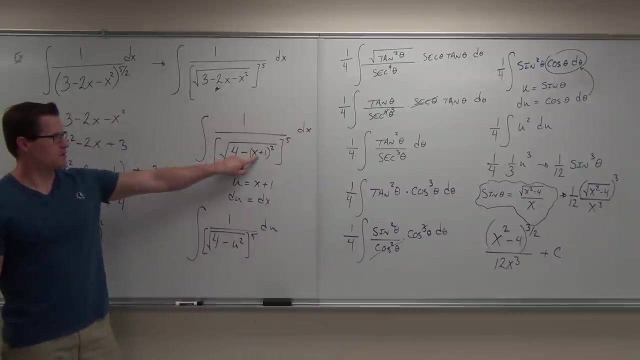 So if you did, u equals x plus 1.. Du equals dx. This just becomes a? u. So we get 1 over 4 minus u, squared under the square root to the 5th power, du? u is this. So 4 minus u squared. 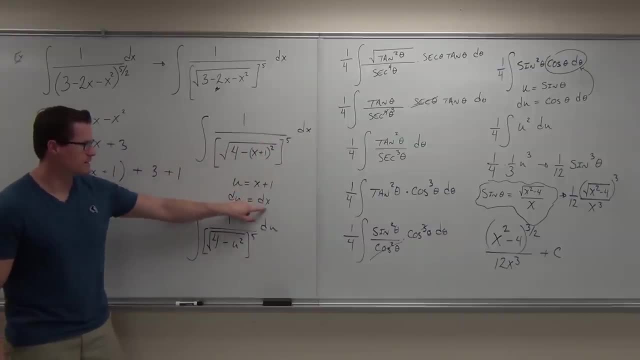 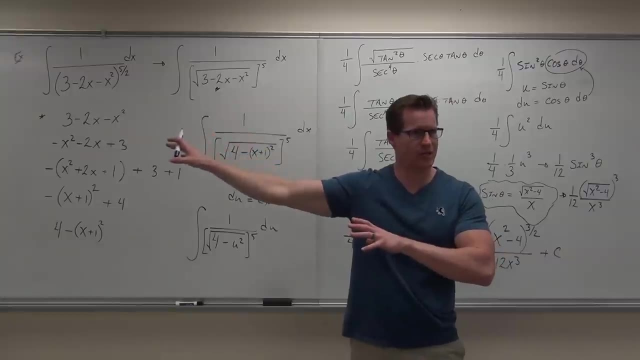 5th power. 5th power Square root, square root dx becomes du Show of hands. if you can follow that one, Could you do? could you have done that on your own? Probably not before this. Can you do it now? 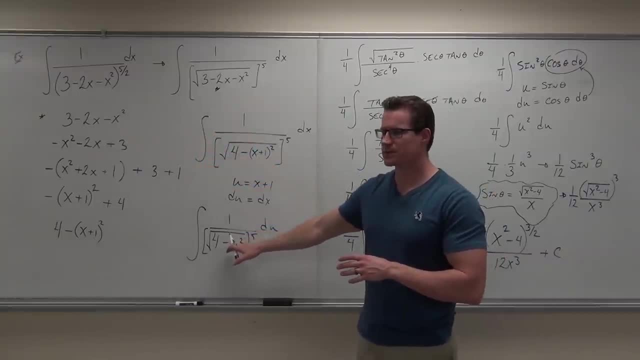 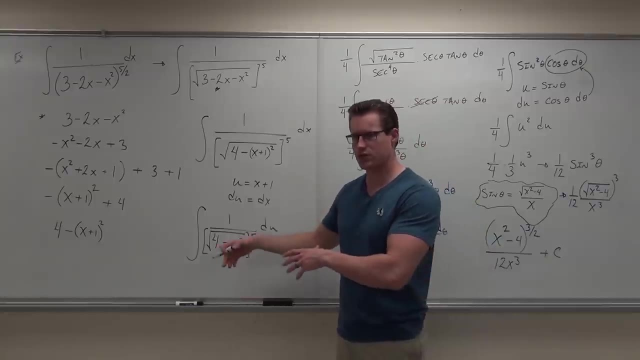 Yeah, Of course you can. Can you please finish that up for me? This is not going to be super, super difficult. I think you can all do that. Can you make a triangle with this? Yes, Okay, So of course, don't forget to substitute back in for u at the very end. 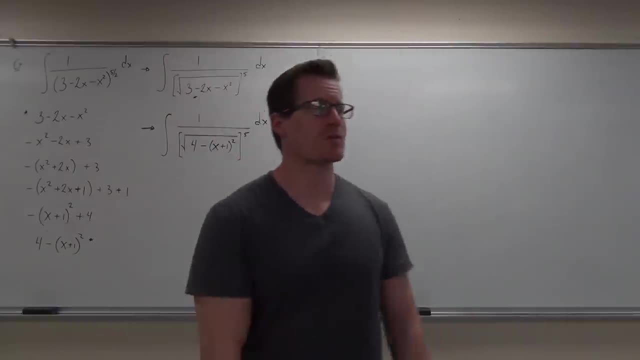 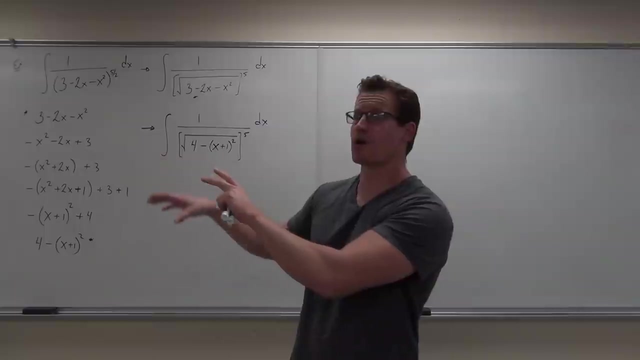 We'll work on this next time, All right? So let's finish up. our problem, As you know, what we're trying to do is we're trying to fit part of our integral into a triangle, to use a trigonometric substitution on either tangent or sine or secant, because 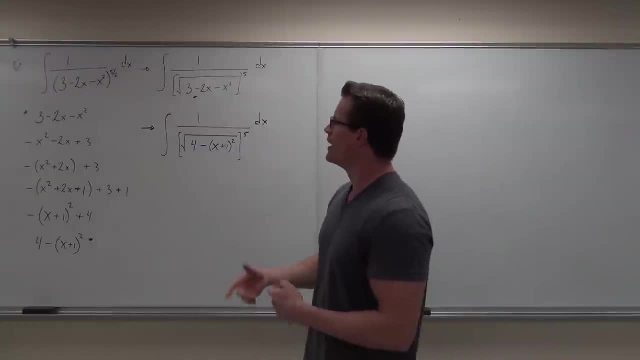 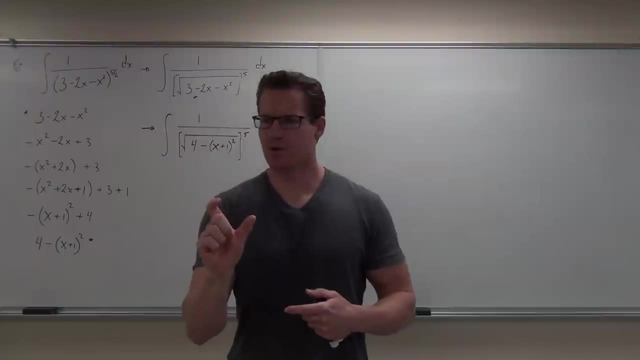 we have some nice identities with those. So we're working on our problem now and right off the bat, we understand it's got a square root, but it's not something nice. Well, something nice is a number or a variable squared plus or minus another number or variable. 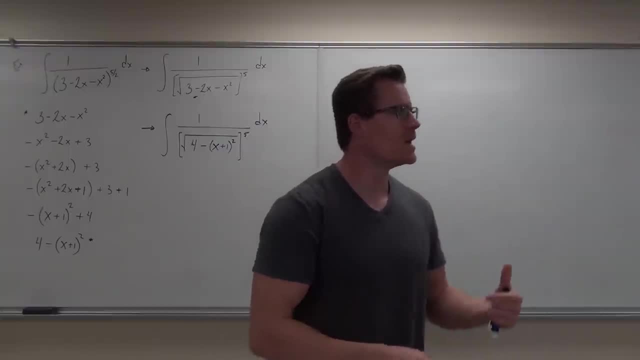 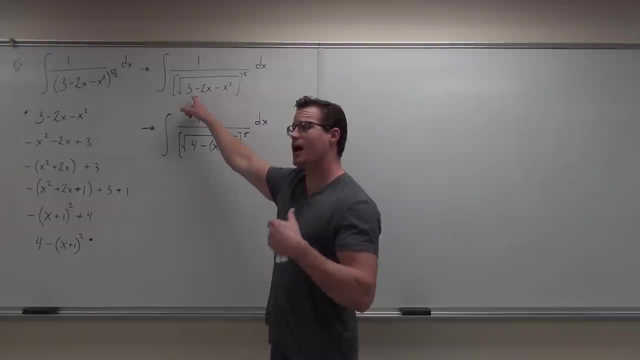 squared. We want something squared, plus or minus something squared. That's the idea. If we don't have that immediately, don't give up on it. You might still be able to work with it. So square root is the first indication that I might be using a trig sub here, but substitution. 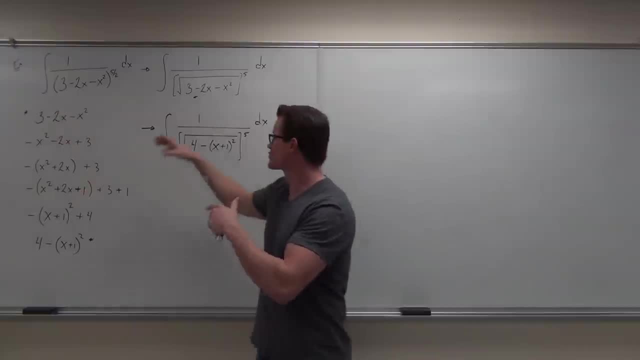 wouldn't work. of course, Nothing else will work. so we're down to just a trig sub. Square root is our solution. The square root says: yeah, you know what you might want. to give this a try with trach sub. 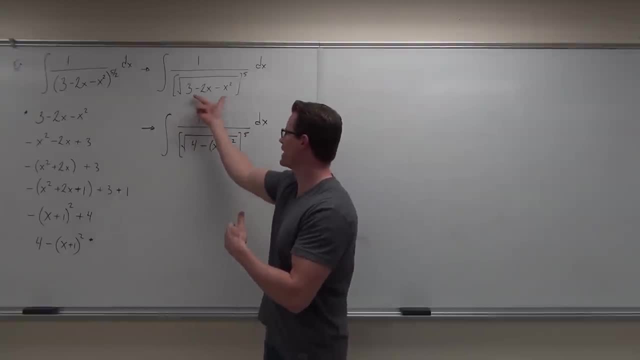 but we gotta change it a little bit. So whenever you have a case where, man, it's not obvious what this is gonna be, take it out to the side, see if completing the square is gonna work. So that's what we did here. 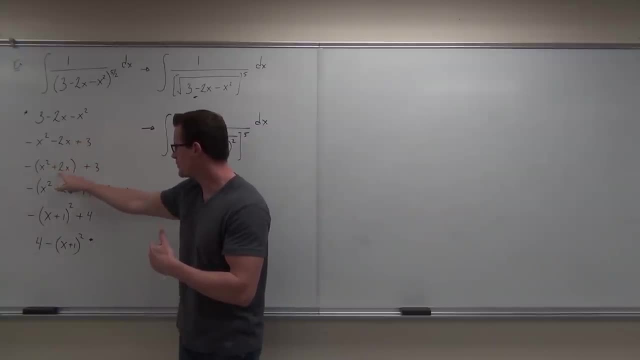 We organized it. we factored out the negative, we added half of this number squared. Notice that when we add it here it's really like subtracting it. so I undo that. So I know it's both plus one plus one. 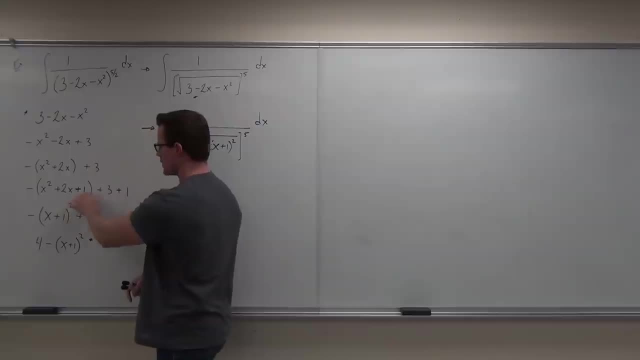 but because of that negative this is really like a minus one. so I undo it with that plus one. We organized it again. we have a quantity minus a quantity. Here we have two squared minus something else squared. This is our first little manipulation. 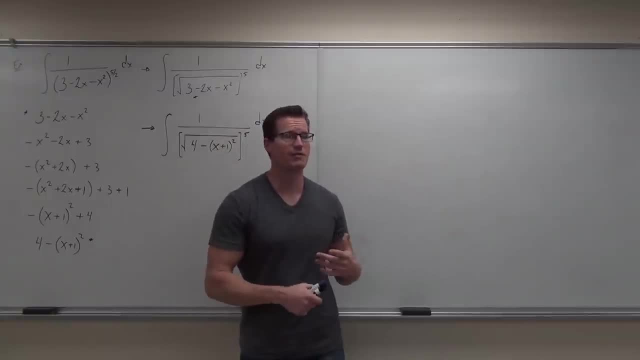 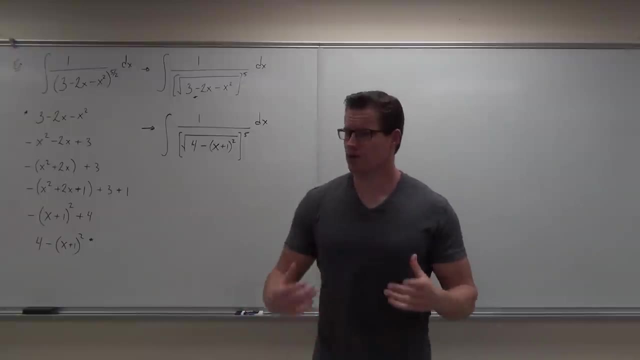 Are you guys okay with that first step? It's just completing the square. I know that many of you haven't done that in a long time, but that's what it is. Maybe review about completing the square and how to do that Now, at this point we could go straight to our triangle. 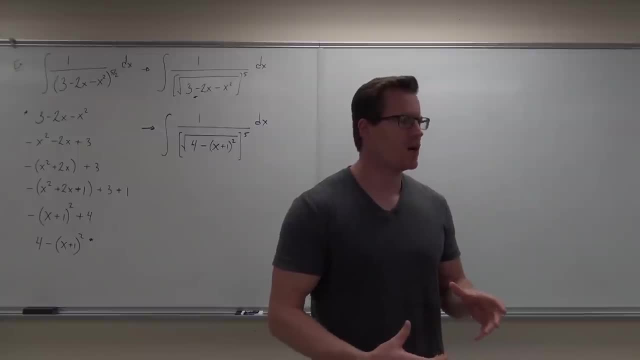 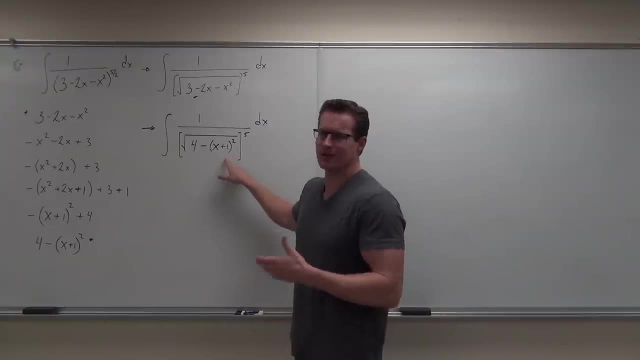 if we wanted. but to make things easy, to make it nice for me, what I'm gonna do is just a very basic substitution. I want to get rid of that x plus one You guys follow. That way I don't have to look at x plus one. 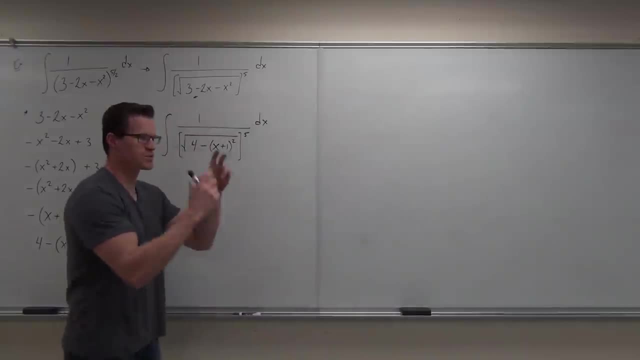 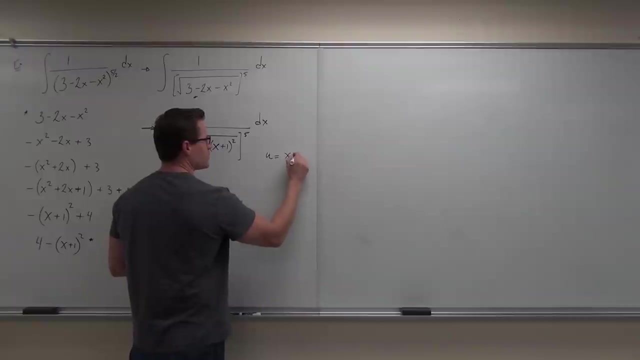 I'm gonna look at a u instead. So whenever this is the case, when you get something squared and you don't really want to deal with it right then feel free to do a substitution. So, off to the side, I'll do: u equals x plus one. 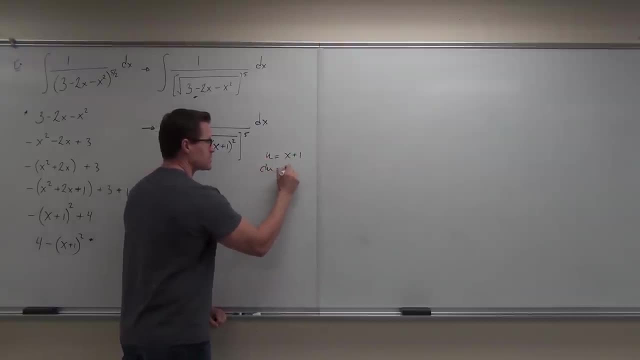 This is really easy because du is just equal to dx. I mean, it's a straight sub. it's nice If you're getting like, after your derivative here, something in terms of x. yeah, don't do that. Just the constant is what we're trying to get out of that. 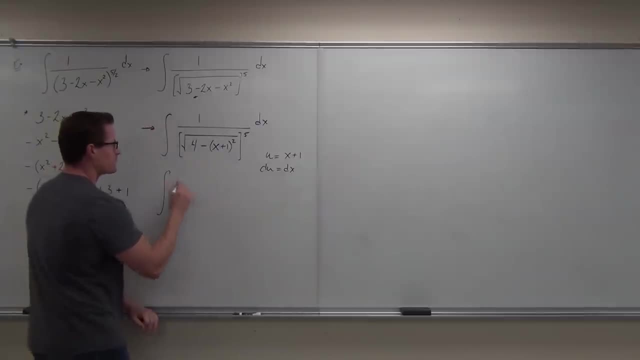 Does that make sense to you? So here we go. all right, cool, Well, we got an integral, then We got one. We still got this bracket with a square root. We got a four still, but here we're just gonna do minus u squared. 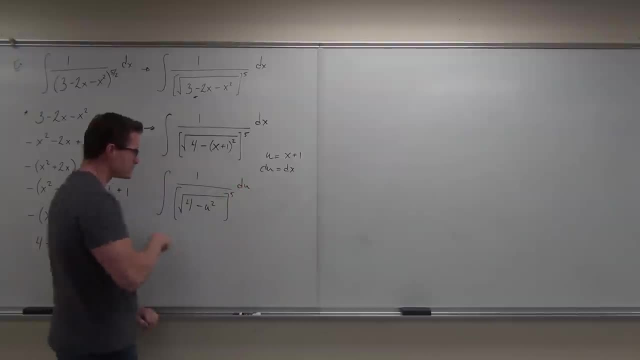 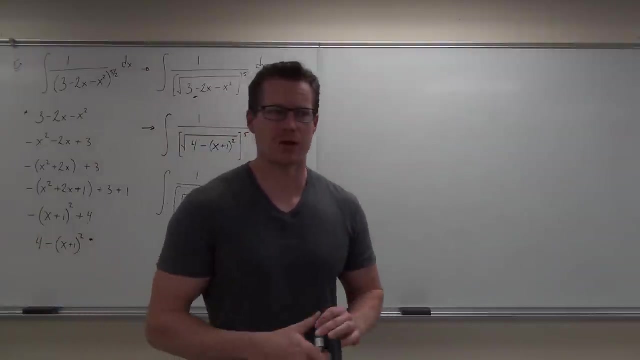 to the fifth and then du, straight substitution for dx. Now this looks a little bit more manageable. So right now, what do we do? Yeah, we're gonna do that triangle. It's a square root, It has something squared minus something squared. 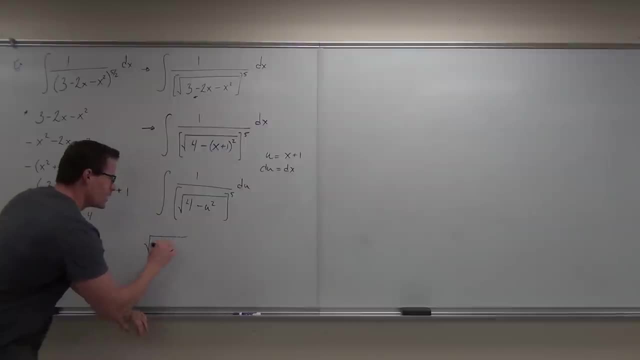 That's fantastic. So, right here, this is my square root. I'm not gonna think about it as four. I'm gonna think about it as: yeah, that gives me the length of a side or a hypotenuse or, I'm sorry, a leg or a hypotenuse. 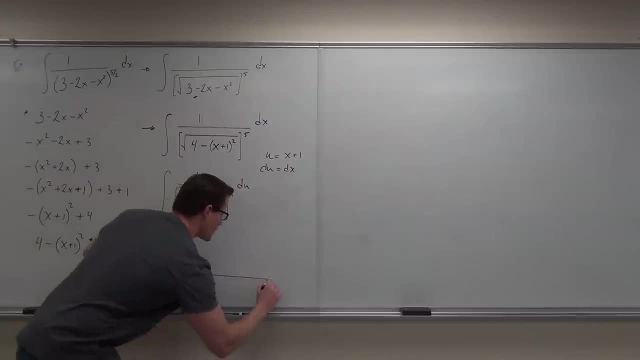 depending on what we're given and which order we're given, And I'm gonna draw my right triangle from this. What I definitely don't wanna do is leave that at four and mistakenly put four here or here or here. Then my integral's gonna be all screwed up. 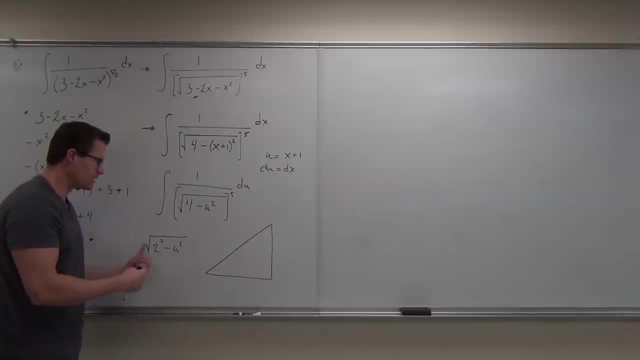 I'm not gonna get this thing right, So I really wanna make sure that we understand that this number is the length of a hypotenuse or the length of a side. a leg squared is what that is, So right. triangle always drawn in the same orientation. 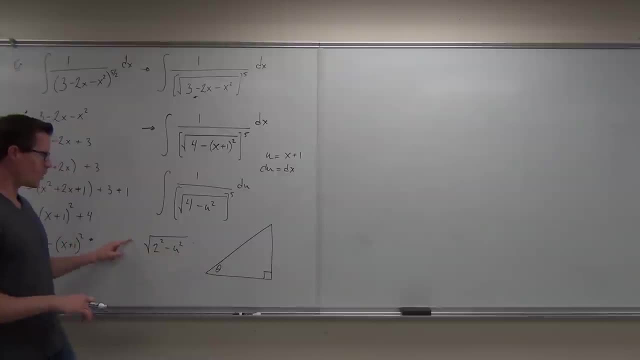 We always have this thing right, By the way. what is this thing? Is this whole thing the length of a leg or the length of a hypotenuse? The length, Yeah, how do you know? Minus that? Yeah, the minus right there. 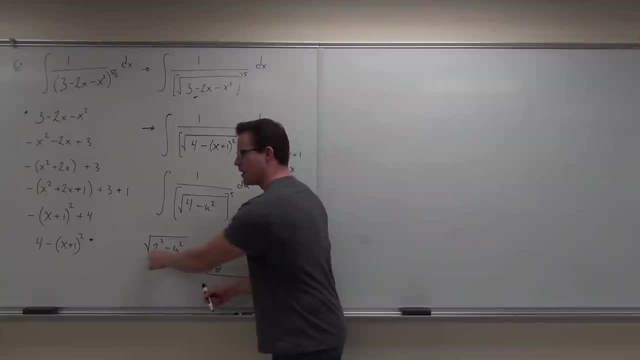 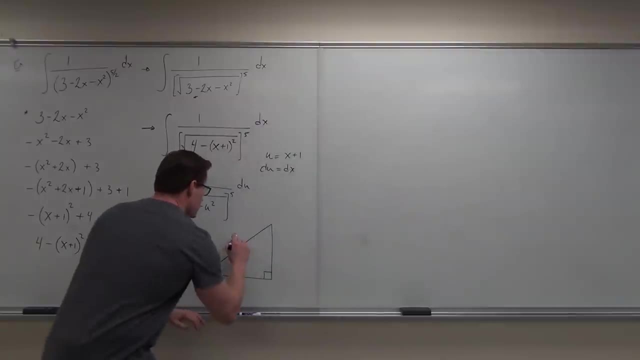 This says what this is. which one of these pieces is the hypotenuse? then The four bigger ones, the two, The two, not the four, but the two. So the two is the hypotenuse, The first one is the bigger one. 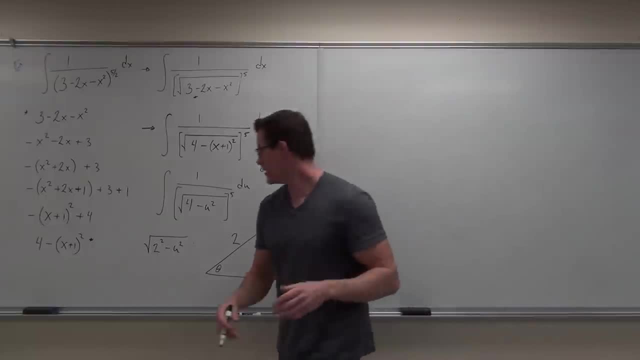 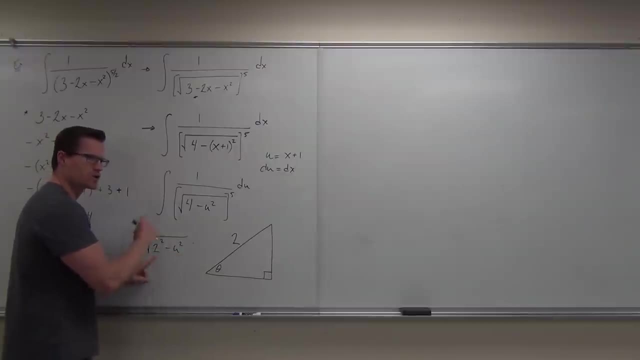 Otherwise we'd get something negative instead of the square root. We can't have that. So if the two's the hypotenuse, the only way this comes about is if I take the hypotenuse squared minus another leg squared into the square root of it. 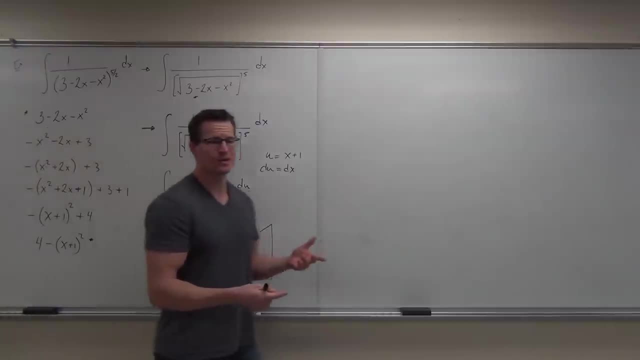 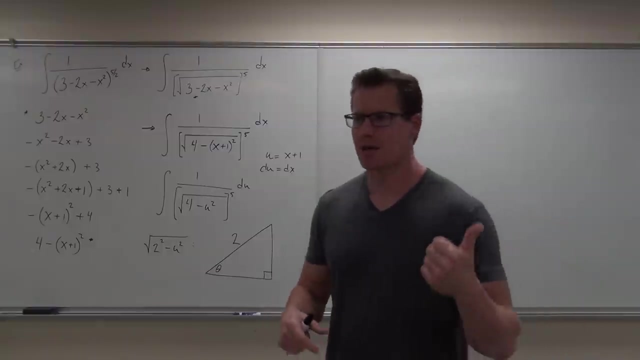 That says this piece is one of the legs. Now we just have to be really good about fitting the legs in the right place. We want a trigonometric substitution that works. It's gotta be sine or tangent or secant, So which one's gonna work for us? 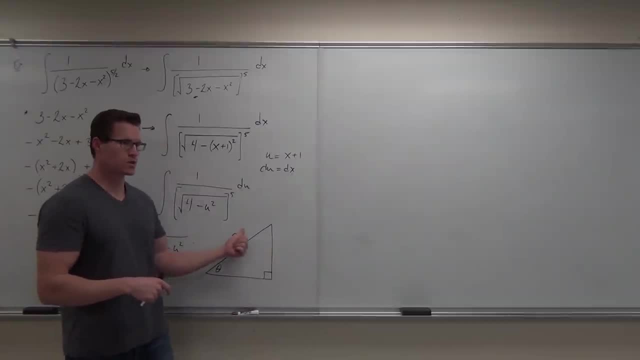 Would tangent be a good choice. No, No, heck, no, I wanna deal with the two. It's someplace right, So it's either gonna be sine or it's gonna be secant. However, I want the two to be on the denominator. 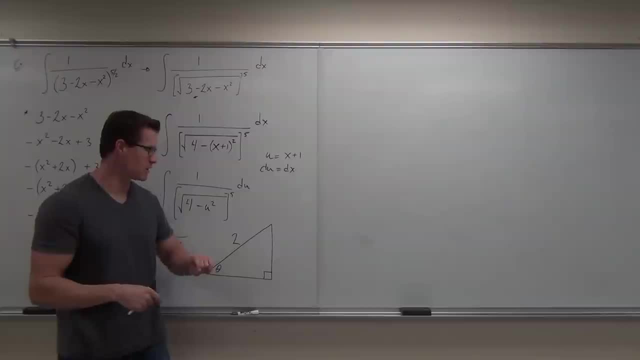 I want the constant on the denominator for whatever fraction I'm gonna create here, whatever relationship, So it's gonna be sine, which means x goes opposite or x goes adjacent, Opposite. You Make it, so this stuff works for you. 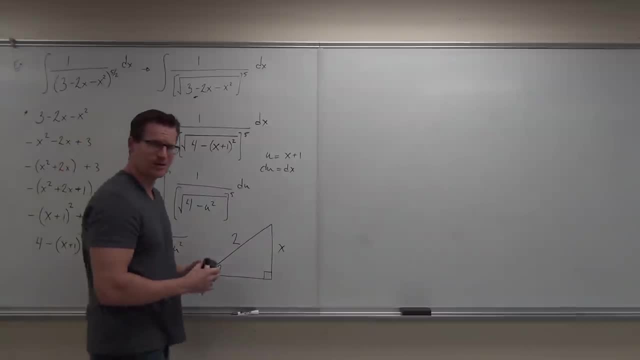 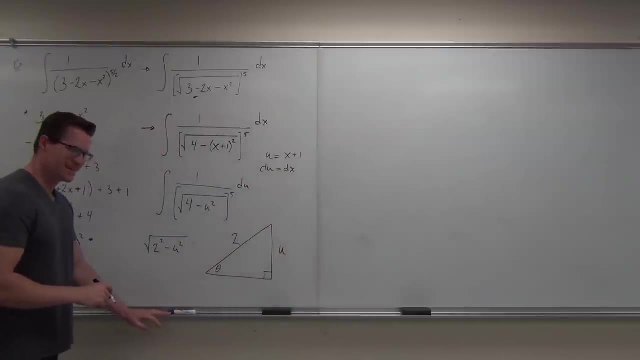 Don't make it sorry, It's you, It is me. Yes, I know It's not me, It's you Anyway, And we have the square root of four minus u squared. That's right, I did the substitution, so I have u now. 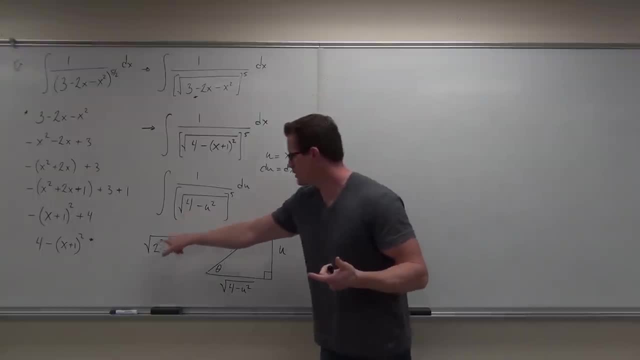 Two of you guys feel okay with that one, So we go. hey, high-plot news, No problem, it's two. This stands for a leg. Just put it in the right spot so that we get u over a constant for whatever trig sub we're gonna do right now. 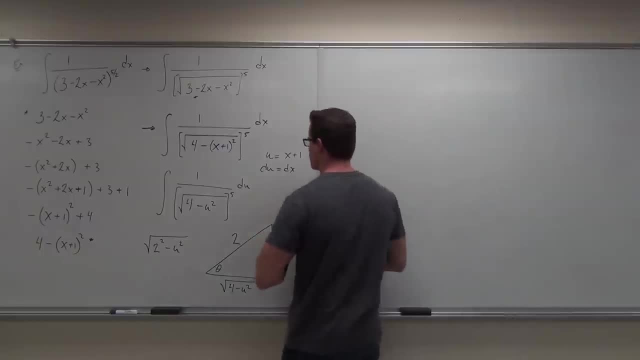 What's the appropriate one? again, Sine. Yeah, sine's gonna give us u over two, So sine Sine Theta. So sine theta equals u over two. Two sine theta, And then we're going to do what Solve for u. 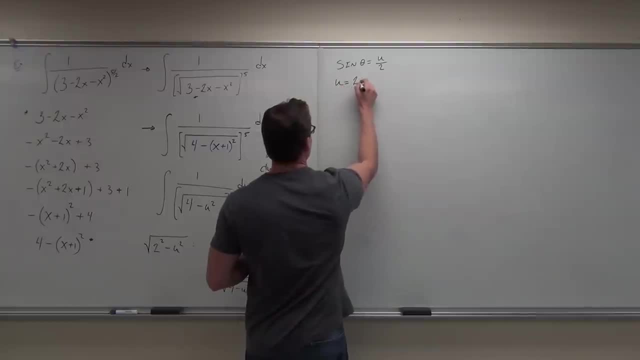 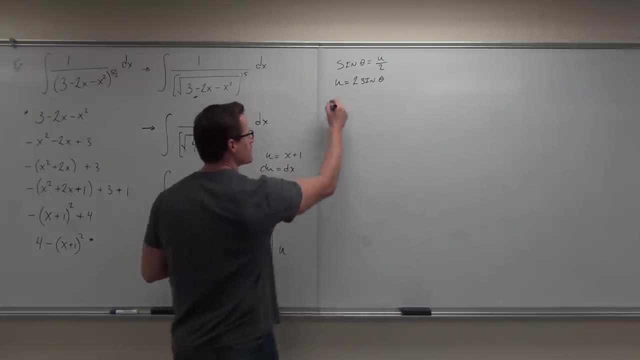 Solve for u. okay, so u equals two sine theta. And next step: what is that D? Sure, because we're gonna do a couple things here. We're gonna substitute for our u. We're also gonna substitute for our du. 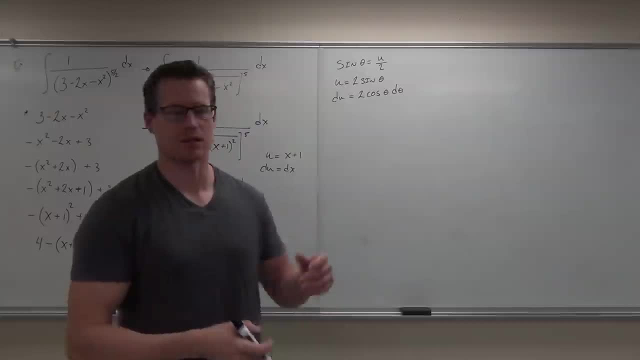 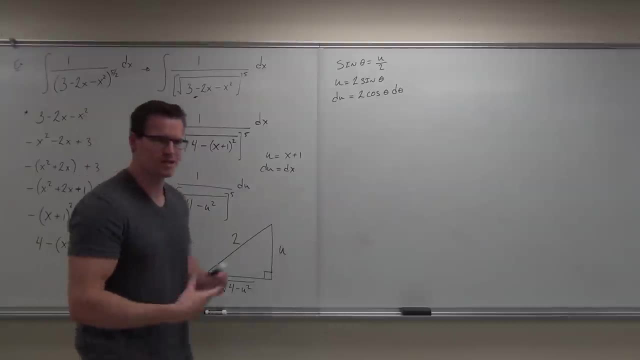 Hopefully we're all okay with the derivative of two sine theta being two cosine. There's no product rule, nothing like that. Now we get to put this back into our integral and make it a lot nicer looking. well, not nicer looking, but easier for us ultimately. 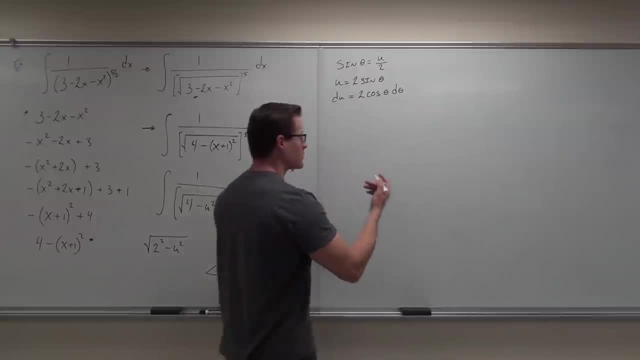 It's gonna look nasty at first. you know, oh my gosh, there's stuff everywhere, But it'll all simplify for the most part, So we got a one. What's gonna be inside of our square root right now? Can you tell me, please? 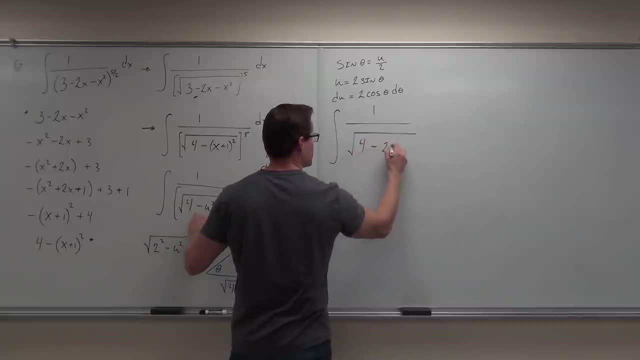 Four minus two sine theta squared, And if you do two sine theta squared, that should all be in parentheses. Yeah, yeah. And then this whole thing is raised to the fifth power, And then, finally, I do gotta remember about my du. 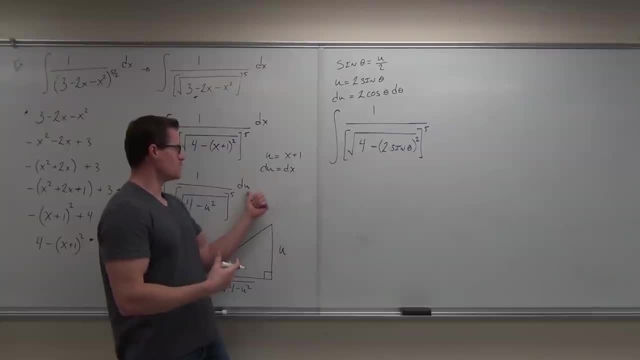 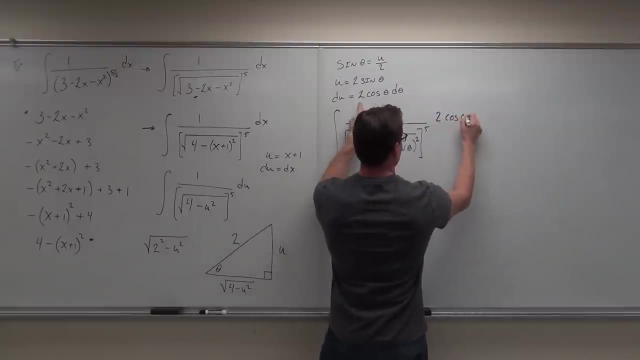 Some of you guys are forgetting some of this. I can't have you forget this. Du has to be substituted for So, instead of du, instead of du, we're gonna put two. perfect. Okay, let's make sure we got this. 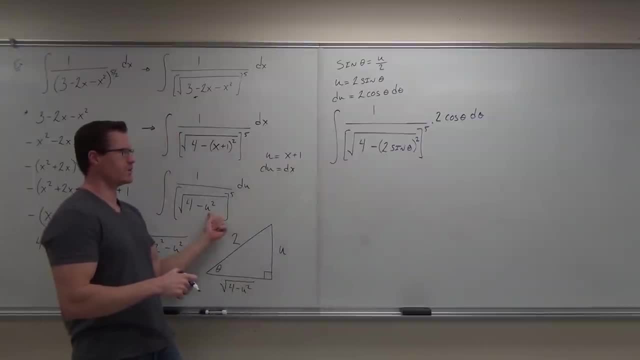 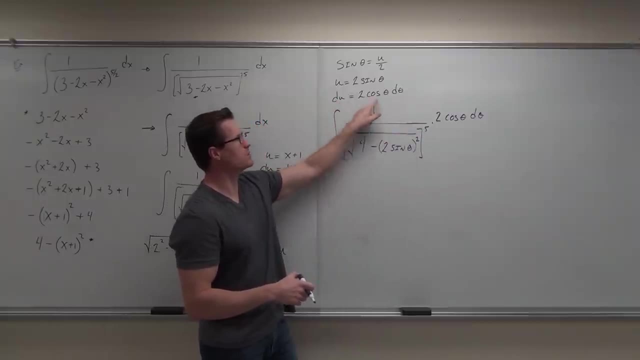 One stays, four stays minus. stays U? no, no, no, no. U is two sine theta. we got it, We have it squared. We have two to the fifth power: Du, no, no, no, not du. 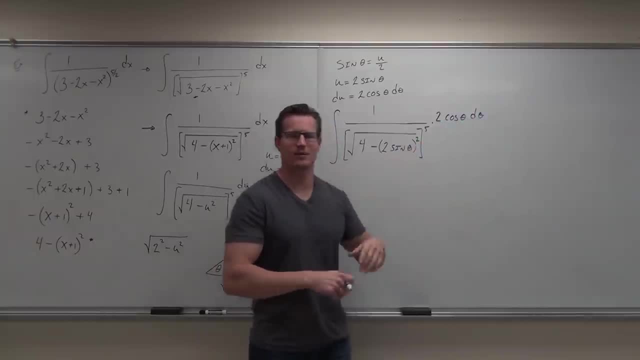 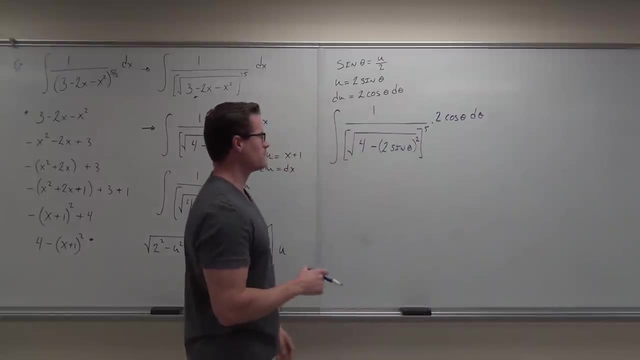 Two cosine: theta, d, theta, D theta's gotta match everything. We can't have two different variables up there. Otherwise that doesn't work for us. So far, so good. Now what do we do? Square root two: pull it out. 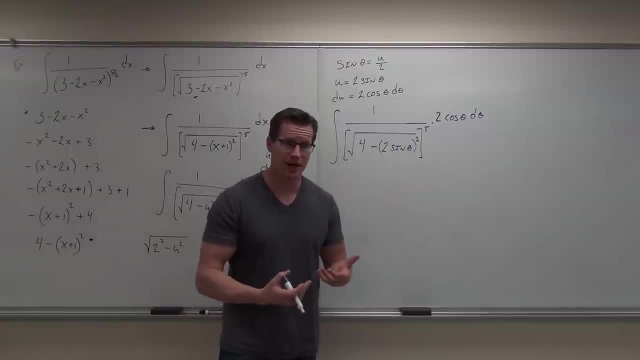 Yeah, we're gonna simplify as much as we can. We don't start any sort of substitution right now. That'd be crazy, right? I mean, how are we gonna do that? What we do wanna do is, well, simplify as much as we can. 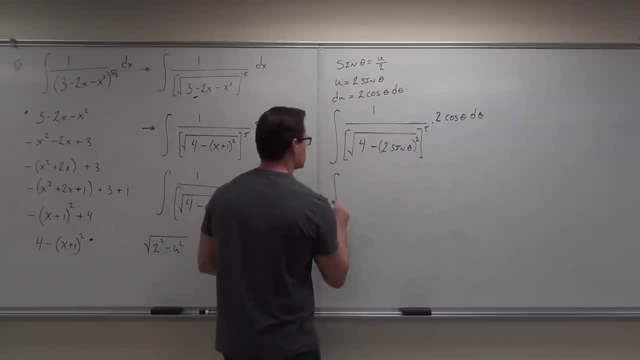 Change it into an integral that we know how to do So one over. if we do this, this is gonna happen a lot for you, where you have four minus the same number, whatever number it is, four, and then sine squared theta to the fifth power. 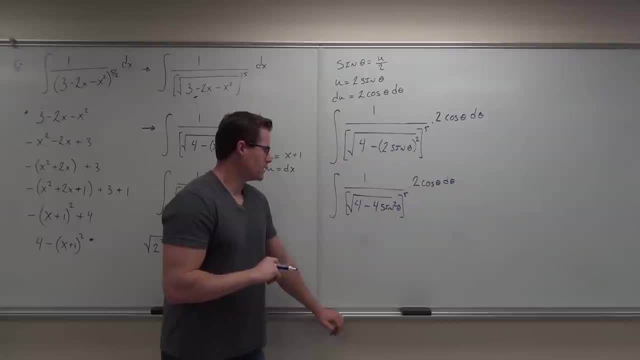 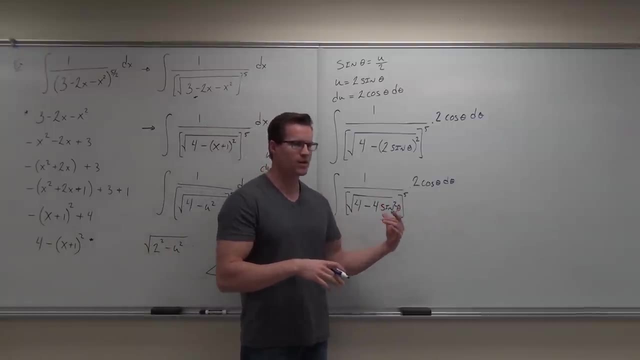 Are you still okay? Mm-hmm, Okay, awesome, What else? Back to your alphabet for us. We're gonna do the four. We gotta have this as one minus something for this, Otherwise we got four minus four sine squared theta. 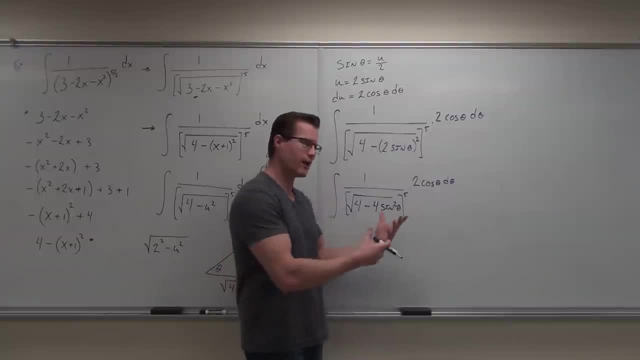 isn't an identity, One minus sine squared theta is, so we're gonna factor that If we factor out the four. just be careful with your algebra. Don't do all of this stuff in your head. Give yourself some time to really think about it. 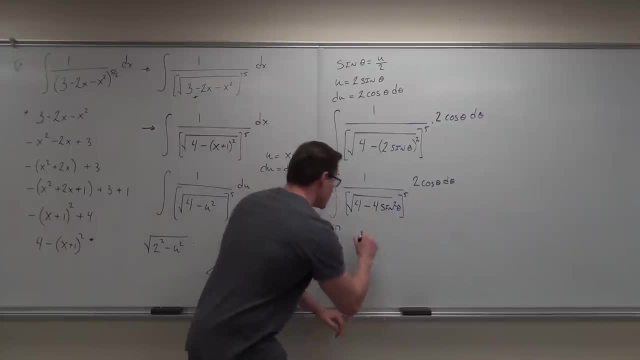 I don't want you just pulling out a two and having one half. You really need to see that. what's going on here is: well, we're pulling out the four. Yeah, the square root of four is two. So we factor out the four and take the square root of two. 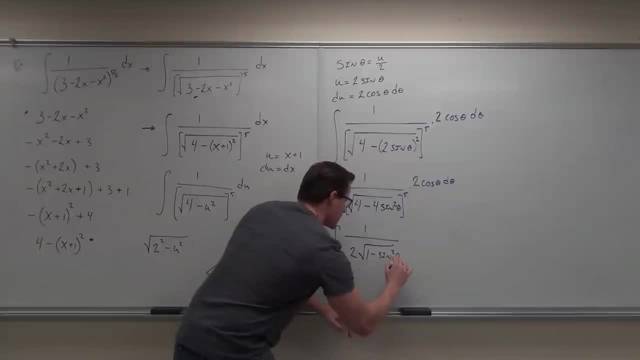 We still have a square root of one minus sine squared theta. Are we all okay with that one? Yeah, you got it. Factor the four. We can separate square roots by product. Square root of four is two. no problem, It's outside the square root. 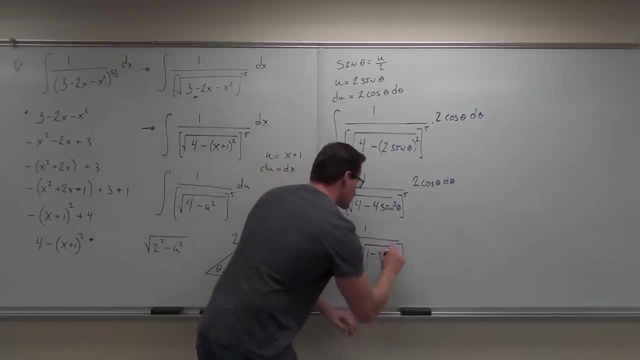 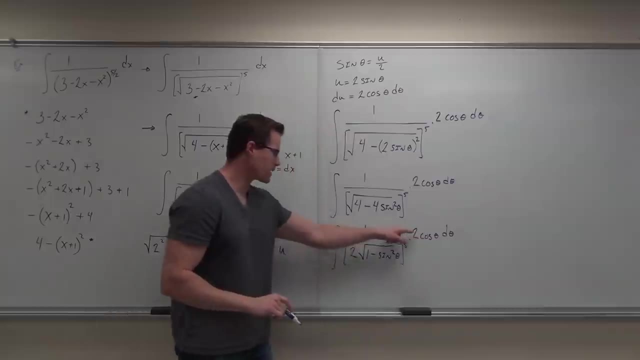 This is inside the square root, but it's still being all raised to the fifth power. So don't do something silly right now and cross out this two with this two. Order of operations says you do exponents before you start simplifying. You'll find things like that. 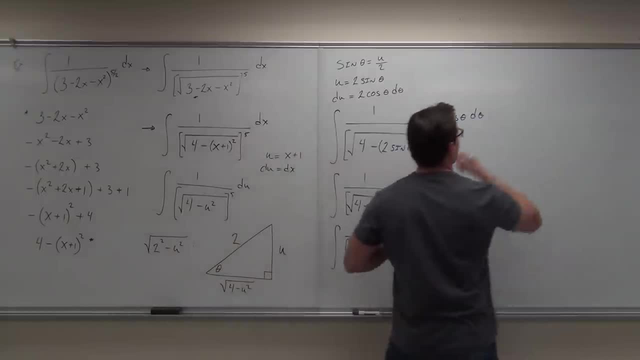 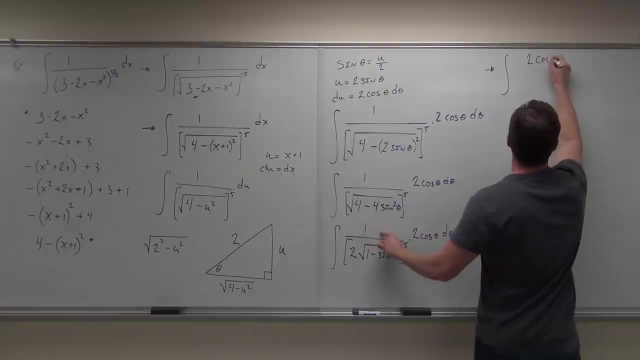 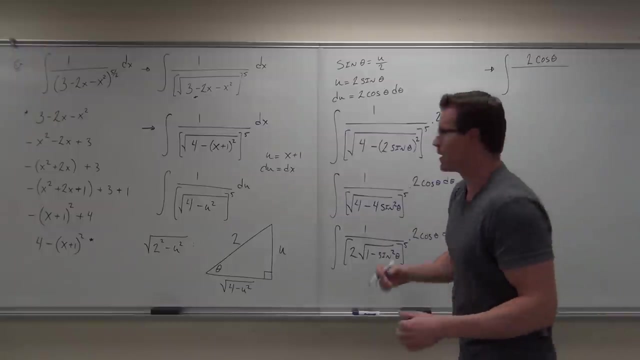 Well, what that means is: then we got an integral. We got two cosine theta. Oh, you got it all at once. We got two cosine theta. What's that? two gonna become 32.. Yeah, because it's two to the fifth power. 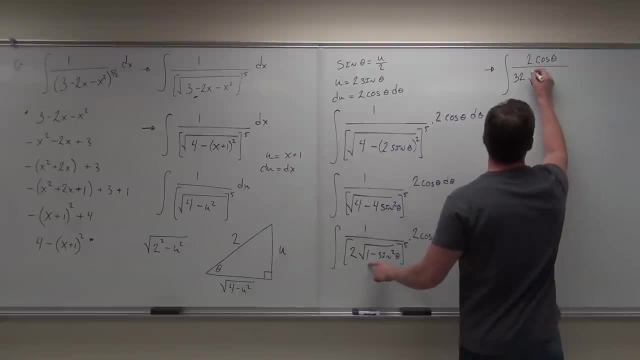 So we got 32.. And then we got one minus sine squared theta. Two to the fifth, Yeah, two to the fifth D theta. We're gonna do a couple steps right now. What's the first thing we're gonna do? 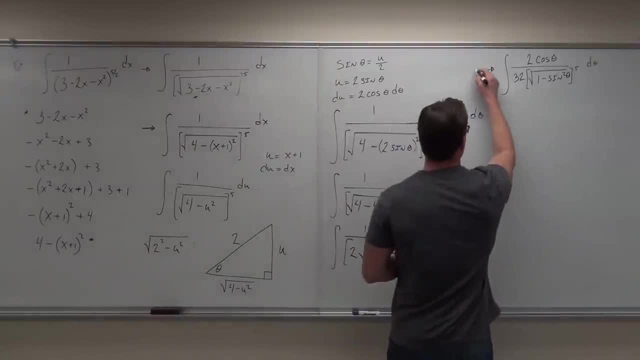 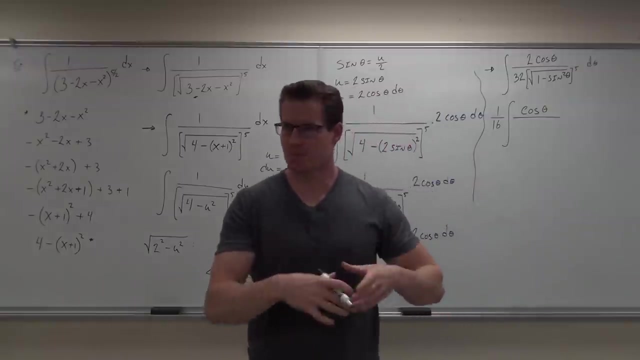 One sixteenth, Yeah, one sixteenth goes up front. So this is one sixteenth. We got it. We got a cosine theta. This is why we did that substitution for sine, because we knew it was gonna be one minus something squared. 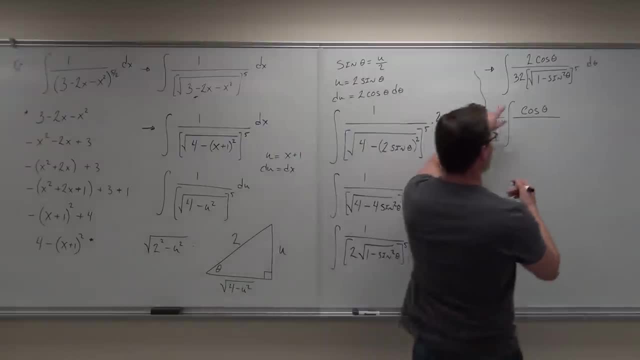 Well, that something squared's gotta be sine for this to work for us. So one minus sine squared, well, it gives us. well, it gives us the square root. Cosine squared, And that's all raised to the fifth power. 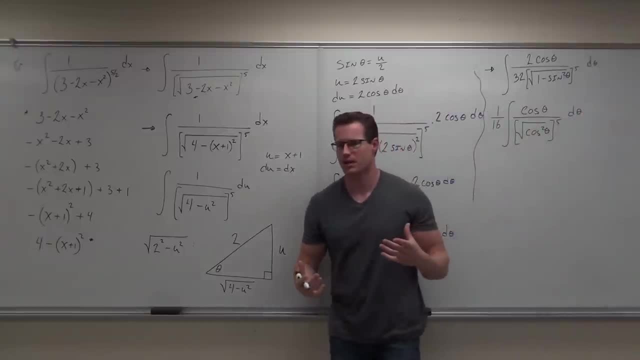 Notice how I'm writing lots of steps. I'm not trying to do everything in my head right now. I know you guys are smart, I know it, But I don't want you doing everything in your head, because what if you forget a little constant? 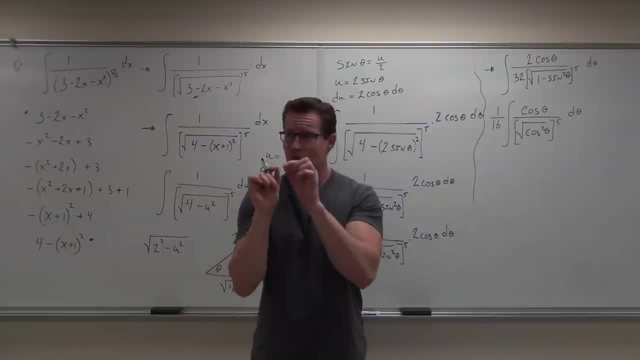 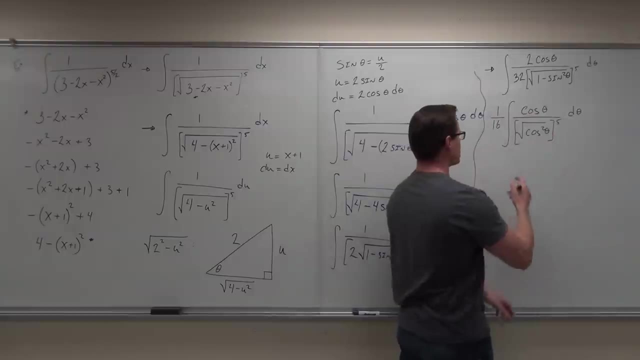 Is that gonna be a good thing? No, It's a bad thing. If you forget a little square or a fifth power, that's a bad thing. I don't want that to happen. Square root of something squared Passes Awesome. 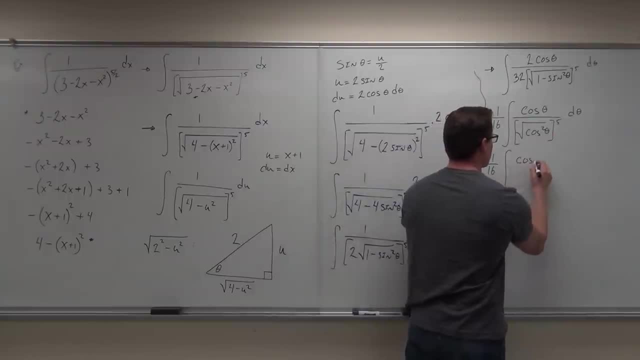 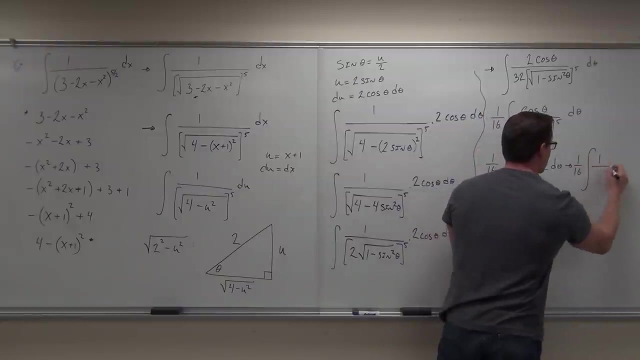 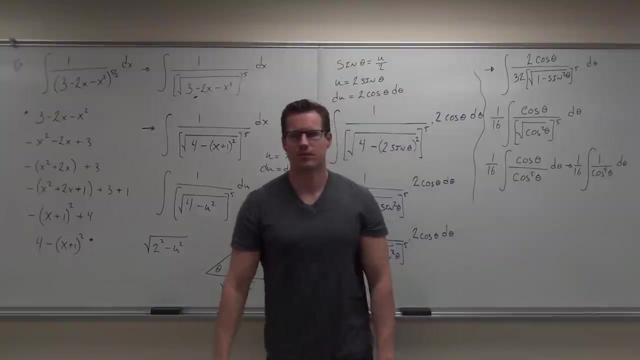 So I'm gonna have one sixteenth integral of cosine theta. Let's do this at once. okay, This gives you cosine theta. Cosine to the fifth, yeah, One sixteenth one over cosine to the fourth: theta, d theta. Now, before you start working with this integral, 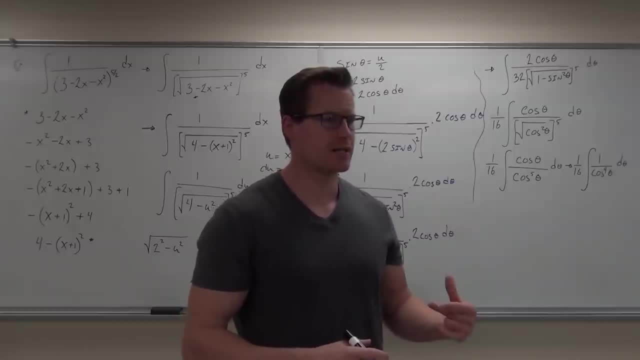 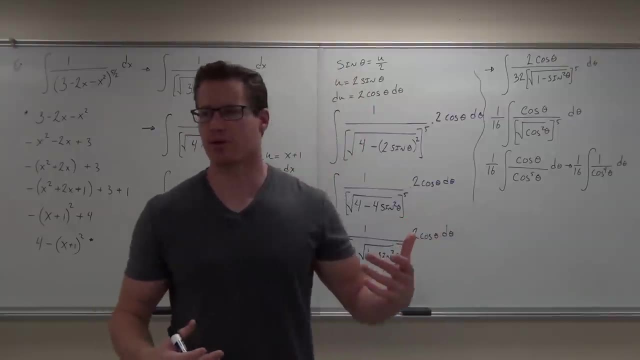 the way it is, one over cosine. to the fourth, it's probably a good idea to check if it fits one of our integration models first, which means that, well, when I'm looking at that, I'm not thinking one over cosine. 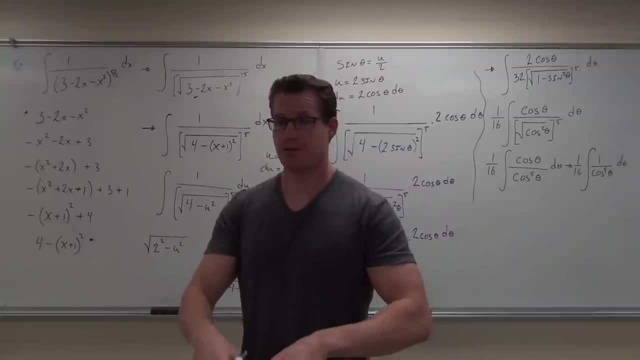 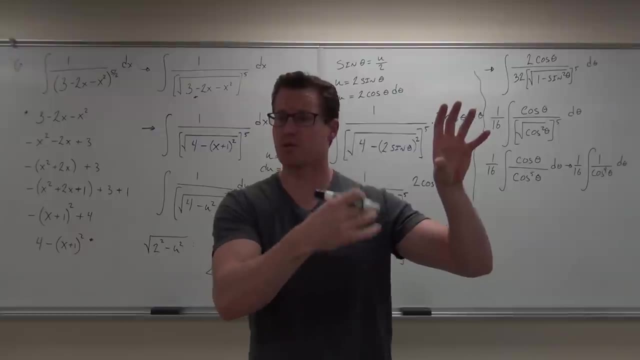 because I don't know what to do with one over something, do I? I know what to do. if this was cosine to the fourth, That'd be great. I'd split it up. That's cosine squared, squared. I'd do one half times one plus cosine two, theta squared. 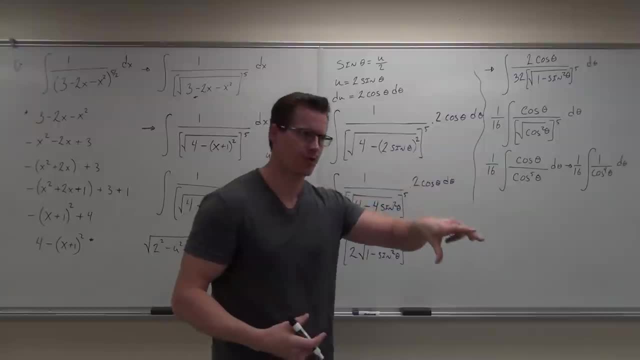 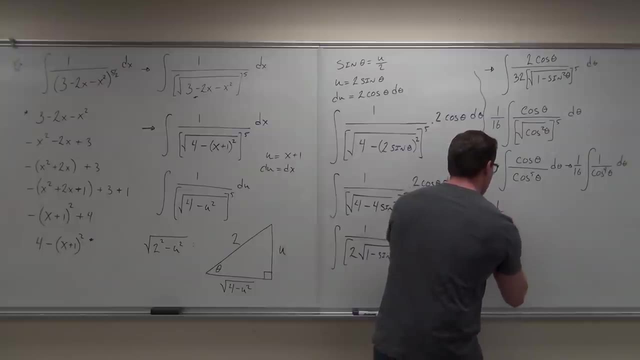 I'd distribute, I'd do that again, But it's not that, It's one over cosine to the fourth. So let's change that into a trig function. that we know how to do it. Okay, So one sixteenth integral of yeah. 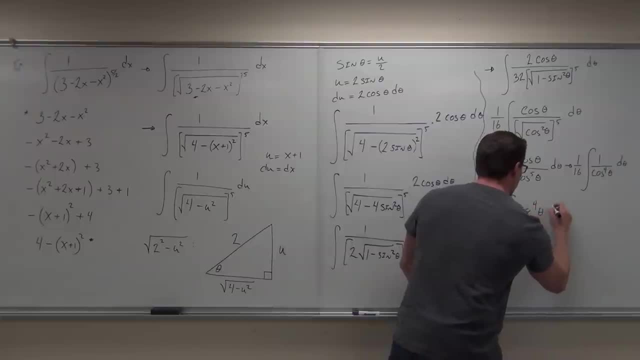 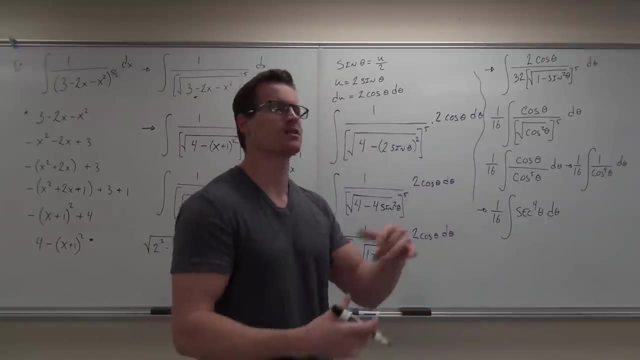 Let's talk about this as secant to the fourth, theta d theta And, fortunately for us, we know what to do when we have secant to the fourth power, when secant is even Think back to your trig, to your last section. 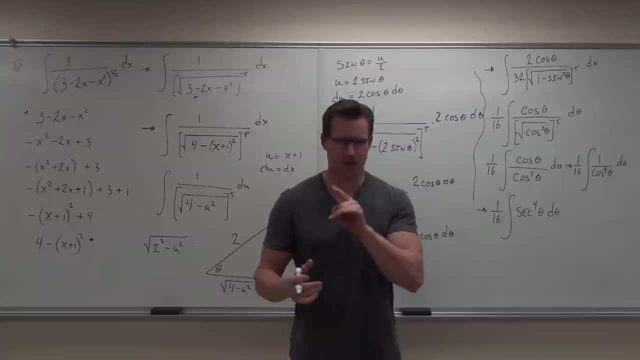 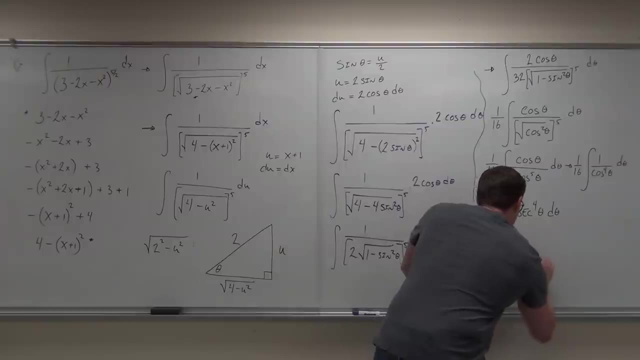 What do you do when secant is even? Bring it up to a secant squared, That's right. So we're going to take a secant squared out of there. So one sixteenth secant squared, theta times secant squared, theta d theta. 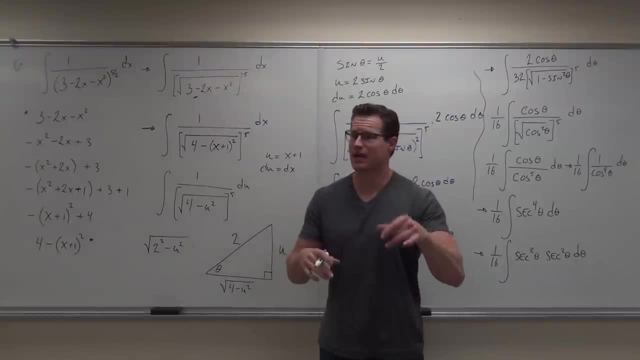 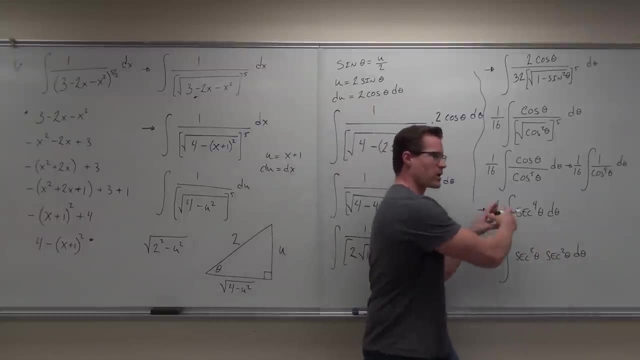 The reason why we do that is because we're trying to get a tangent. If we get a tangent by some sort of a Pythagorean identity here, then derivative of tangent is secant squared. So the reason why we break up the secant squared is: 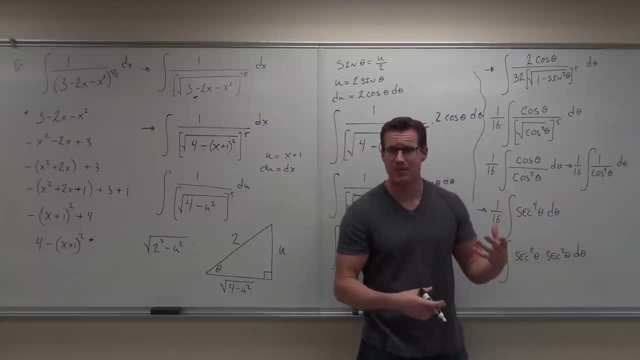 because we're looking for a tangent from the rest. That's why we did that. with even powers of secant- Because of even powers we can strip off the secant squared It's still even- We'll be able to get an identity of one plus tangent squared somewhere. 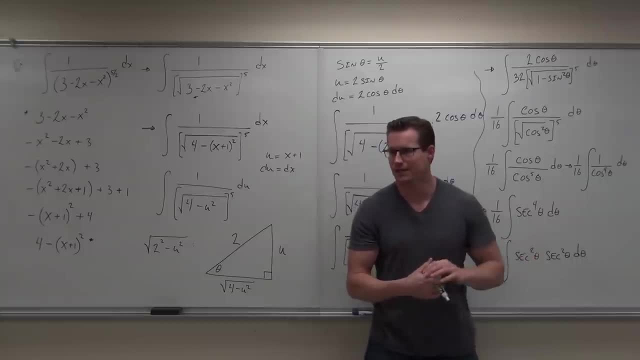 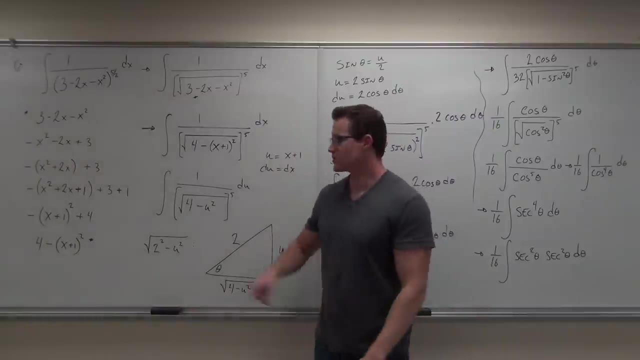 in there, if I'm right, Hopefully Identity. Now I'm going to have to erase part of this. Do you have any questions on this before we continue? So you've got all this written down right. This is basically just an algebra completing the square. 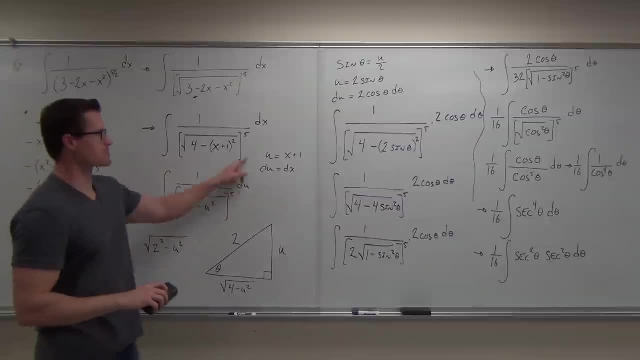 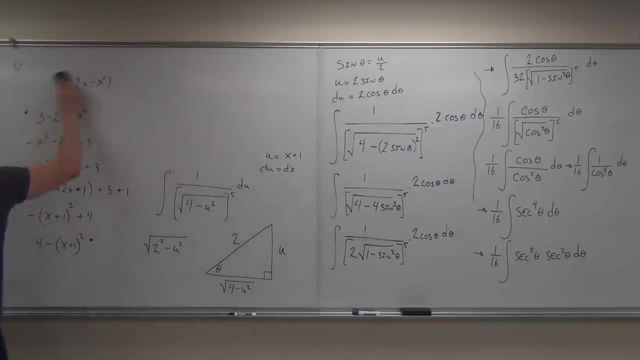 and then doing one basic substitution. One thing I do want to remember is this: OK, I'm going to leave this on the board, because this was kind of big for us at the very end, And I'm sure going to leave this on the board. 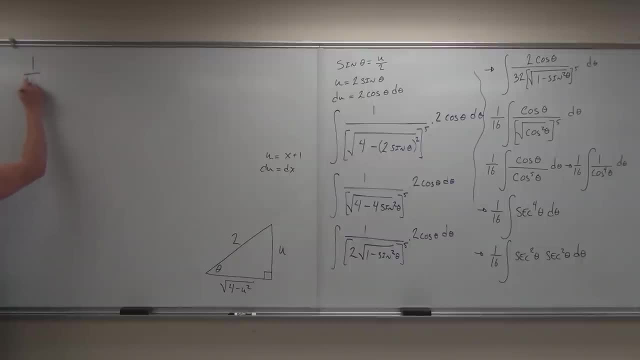 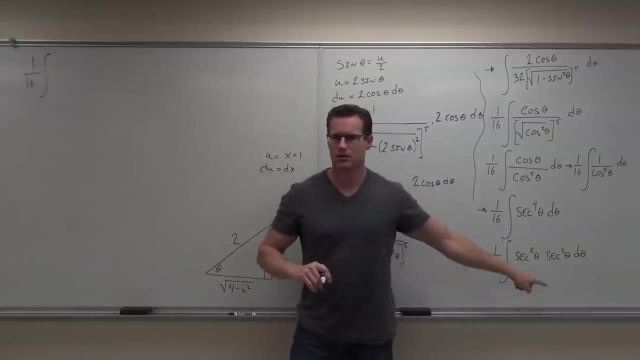 So 1, 16th, no problem. Integral looks like we're going to have. what do I change that secant squared into? What's that going to be? 1 plus tangent squared theta, whatever you want to write that as. 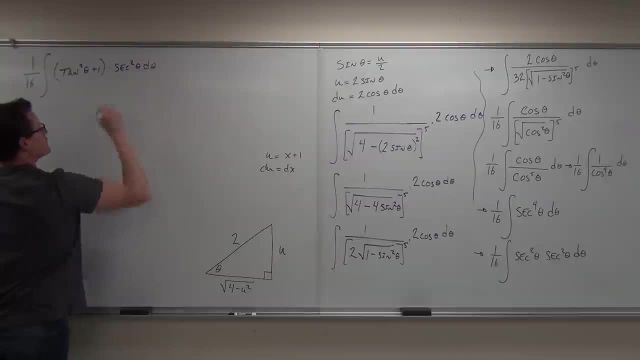 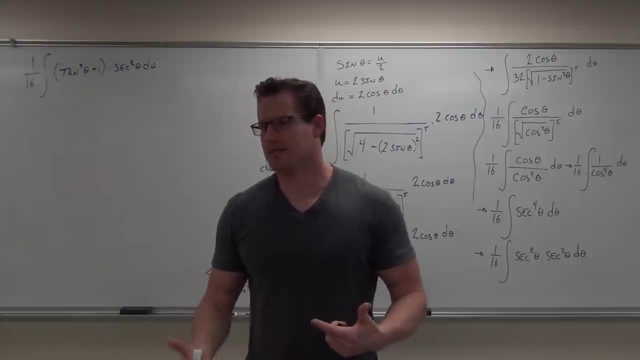 Times, the secant squared, theta d theta. Look how everything, what this does. it changes it back into some sort of a trig model that we know how to deal with. That's what our trig sub does: Changes to something we know how to do. 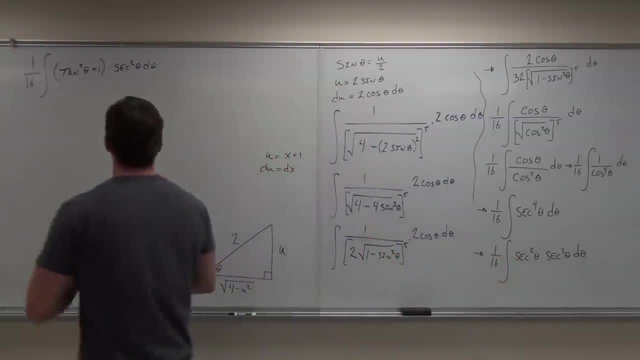 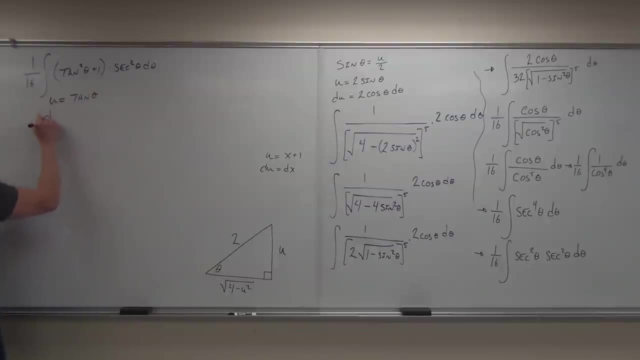 That's what substitutions always do: Change it into something we know how to do. Yeah, no, it's kind of basic. after this, We know a? u sub for tan theta. We've already dealt with this stuff. du equals secant squared theta d theta. 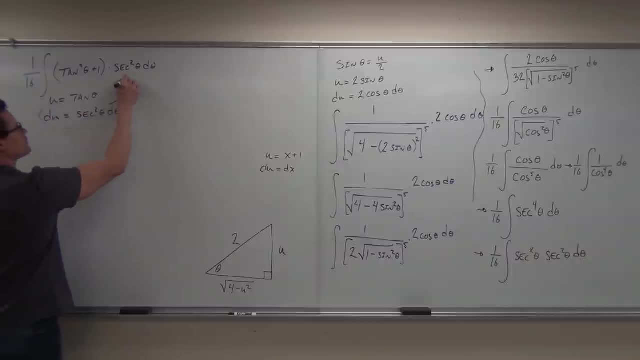 That's right here. That's exactly what we want. That's why this stuff worked, or what I forget. So we can? no, I think I was wondering if we can. Oh, you know what? yeah, We have a? u. you might want to change it. 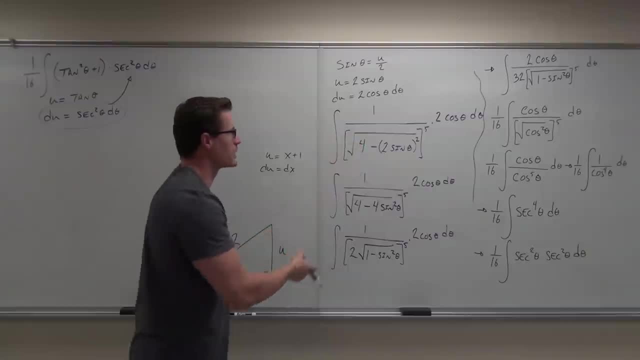 to a different variable. So I already used a u, so that's a good point. Forgot about that one. Let's make this into like a w, Just so we don't get confused, because we will be resubstituting back in for u. 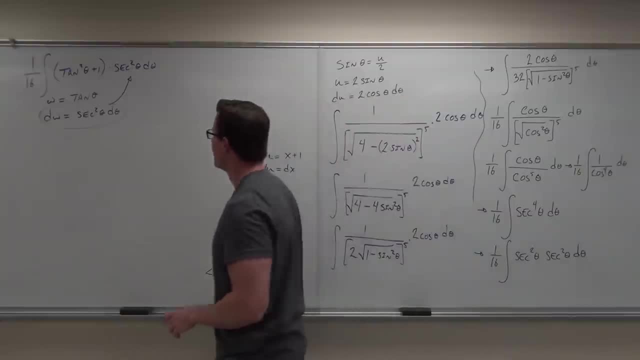 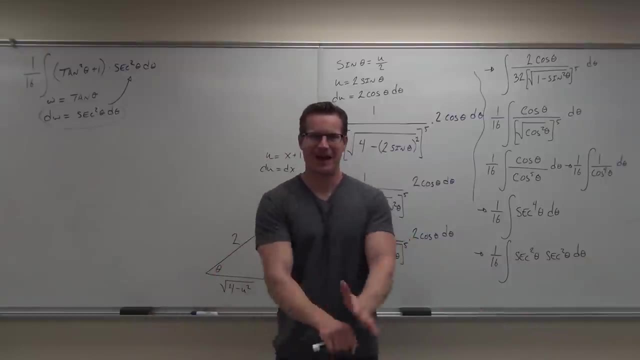 and I don't want any confusion there. So good point. thanks for catching that. I saw the look on your faces. Wait a minute. wait, Mr Lanarker, You got. yeah, I made a mistake. I mean, I was testing you. 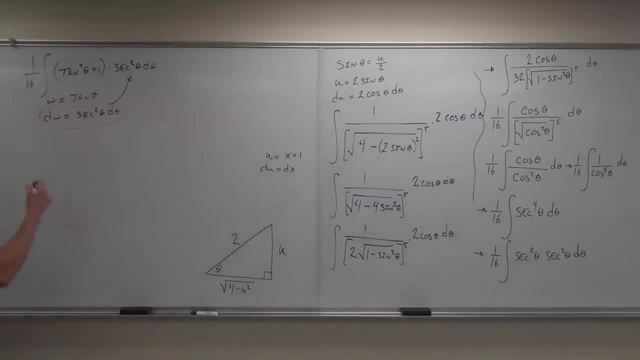 You passed. Making sure we're awake, That's right. and making sure you're awake, That's the age-old, age-old. That's the age-old excuse for mistakes from math teachers. So, integral: tell me what's inside my integral right now. 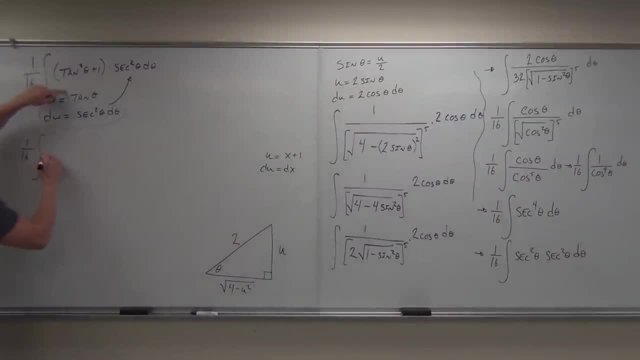 please, what is it? u squared plus one, Not u W squared, Not u W W W squared plus one. Yeah, dw Good. this whole thing is dw Whole thing. is dw Now integrate? Yeah, let's do it. 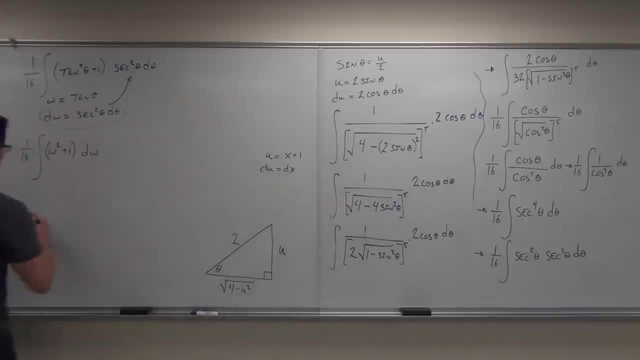 Let's integrate. Can you all do that? Yes, Push me. So when we integrate here we've got 16.. One third w. W is third over three or one third. That's the last answer. W. OK, now it looks pretty painless. 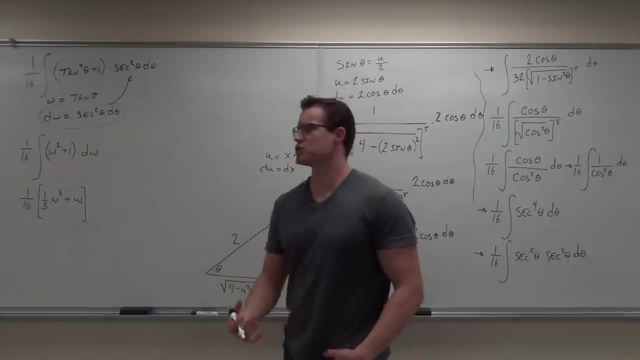 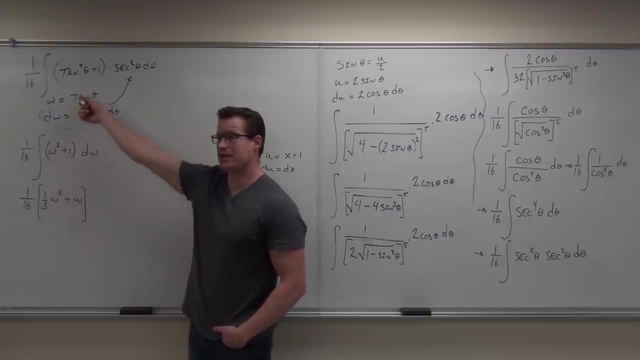 but we have some things that we're going to do. We've done two substitutions here, So first thing we're going to do: we had w's here. We started with some thetas. Originally we started with x's, So we're going to have to translate this back twice now. 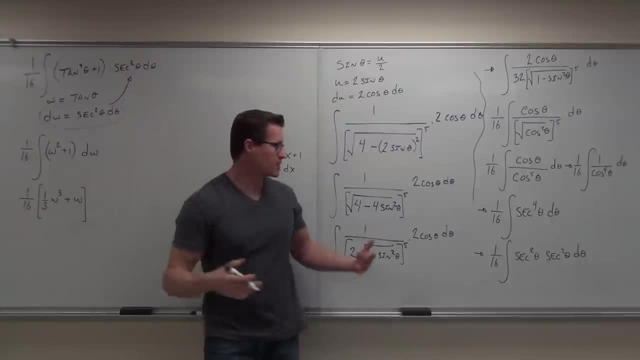 Firstly, I want to make sure you're all OK with this so far Show of hands. if you are, After this point, it's pretty easy. It's stuff you know how to do, So just do it like we've been doing. 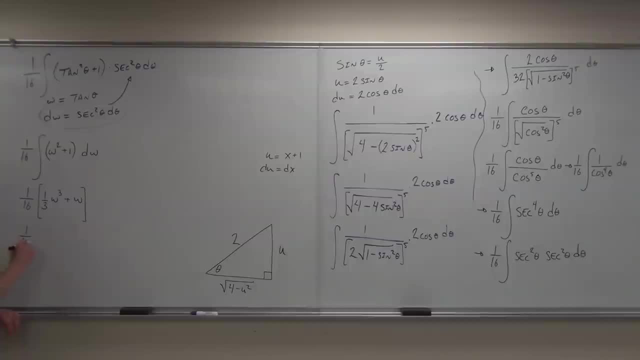 OK, so we're going to have 1 16th, We'll have one third. Well, what's that? w become Ten, Ten One there, And then cube theta. So sure, ten, cube theta, plus how much. 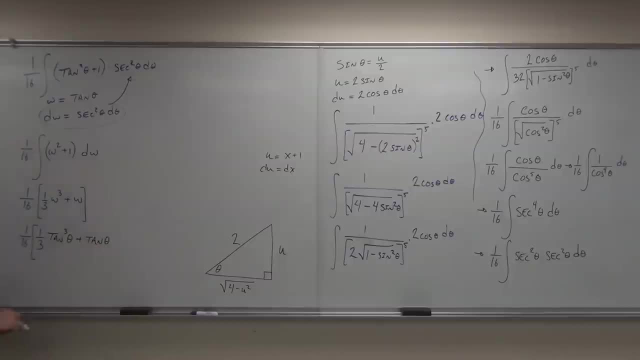 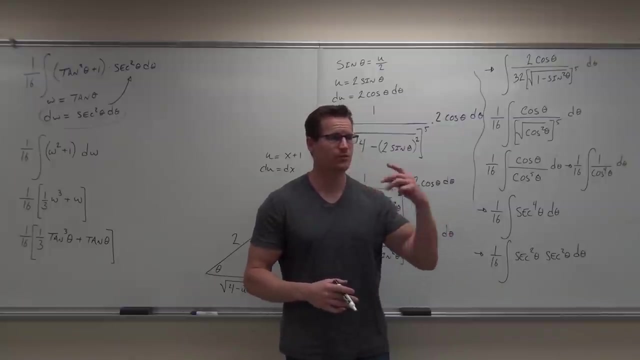 Ten cubed theta, We still OK. No, You've got to put your x's back in. OK, so we are going to put x's back in. but it's kind of weird. We've done three substitutions. We substituted first with a u. 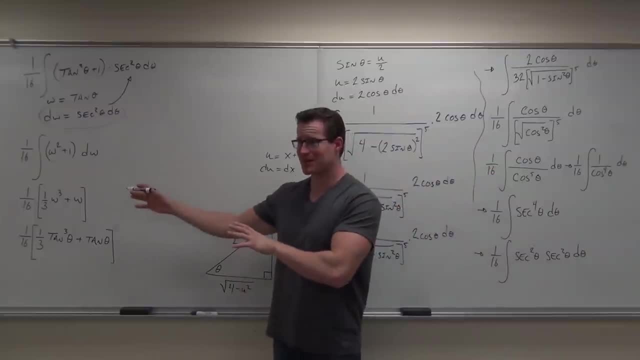 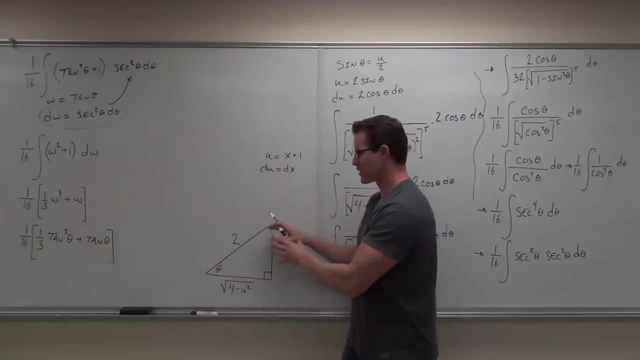 Then we made u's into thetas, Then we made thetas into w's. So now, Not theta, We've got our w's. we've got them back into thetas. We're going to use this to translate our thetas back into u's. 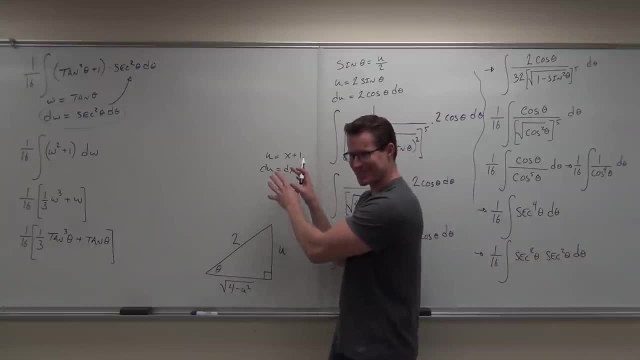 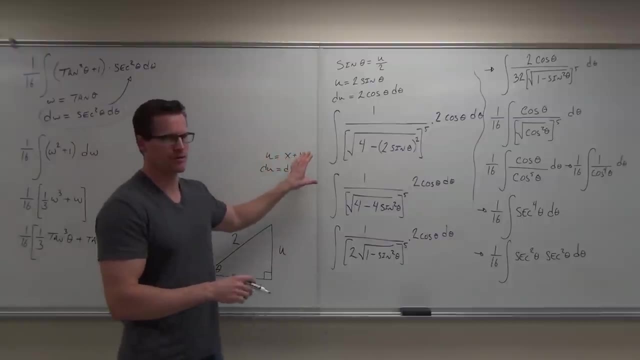 Then we'll use this to translate our u's back into x's. Does that make sense to you? All right, so as long as you have your breadcrumbs to come back with, you'll be fine. Just don't forget this stuff. We don't want to get too involved in this. 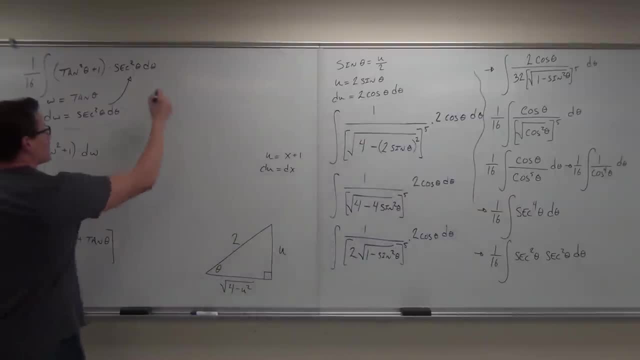 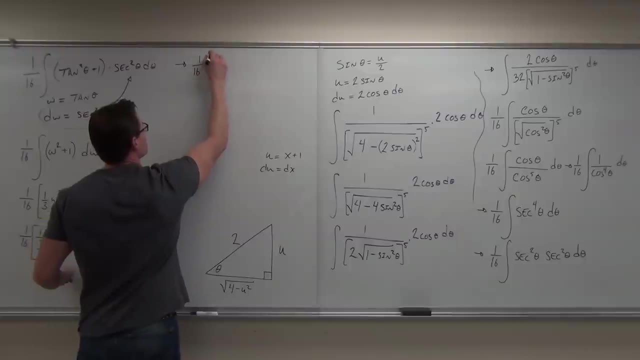 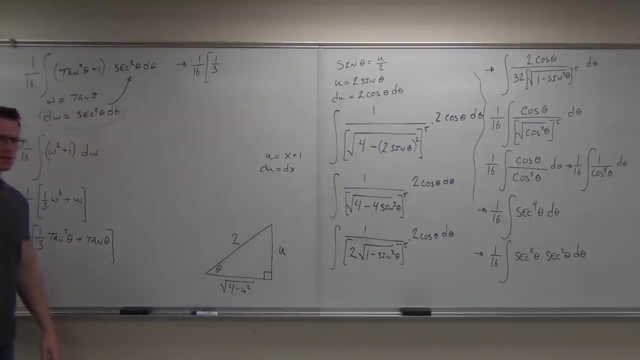 to forget what we actually started with. So we went here, we got 1- 16th. going back up, top 1 16th, We got 1 3rd. Oh, let's think about tangent. Can you figure out what tangent theta is? 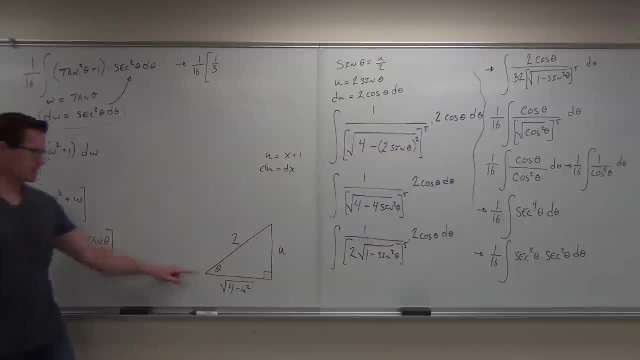 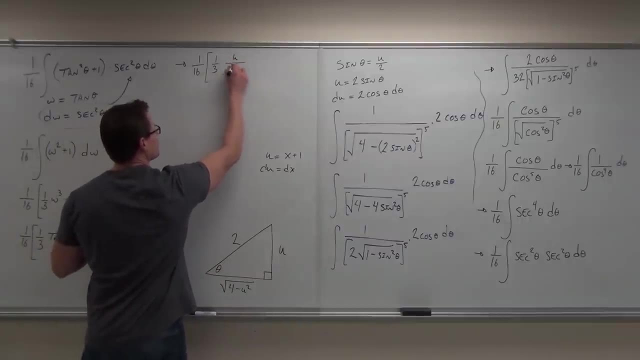 And so we're going to leave our triangle here. This is theta, So tan theta: is u over square root of 4 minus u squared Over 1 3rd cubed, Cubed, Cubed, The whole thing Plus. 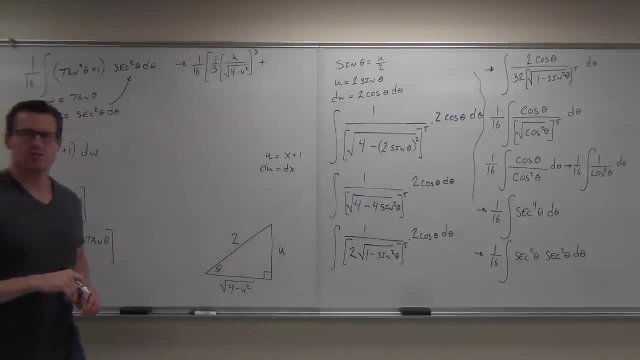 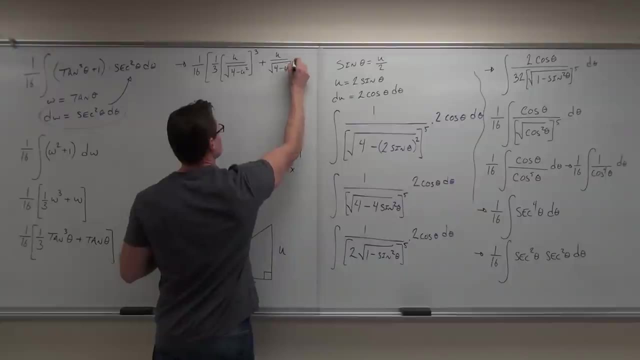 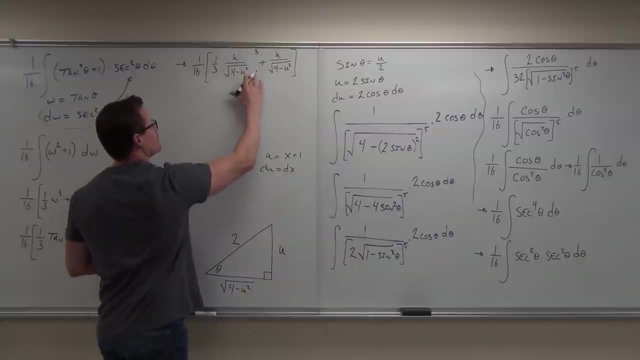 Can you do tan theta? Same thing, but not. I'm going to change that to a parentheses, just so it looks a little bit better. By the way, Is it the 1- 3rd that's also getting cubed, or not? 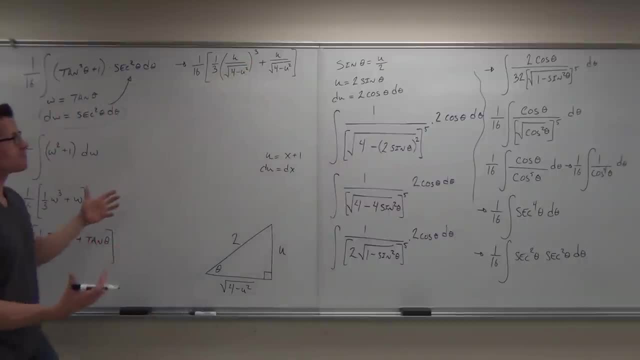 No, OK, that wasn't inside there, It's just the tangent. So tangent of theta. Hey, look at that Tangent of theta. is u over this guy? square root of 4 minus u squared. No problem, We got it to the third power. 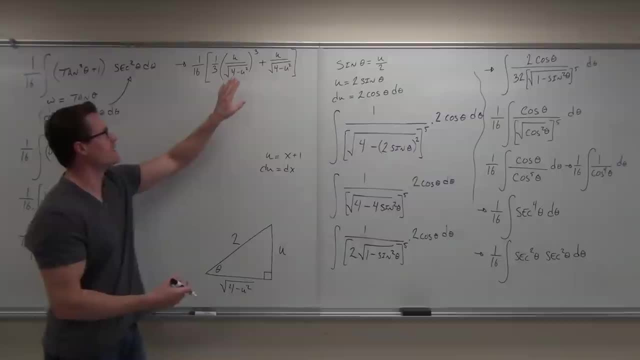 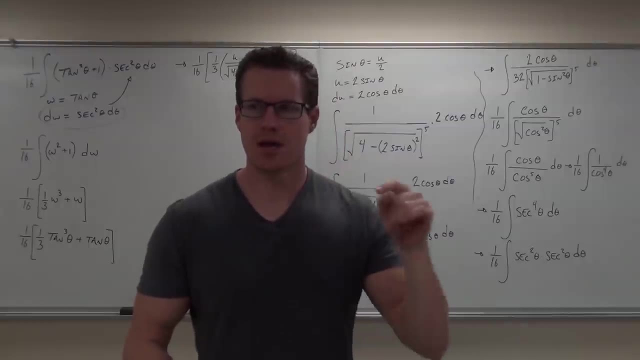 Plus another tangent, Same idea: Opposite over adjacent. It's right, there, Are we done? No, Nope. One more thing to do Now, at this point. if you are going to choose to simplify this, this is where you would do it. 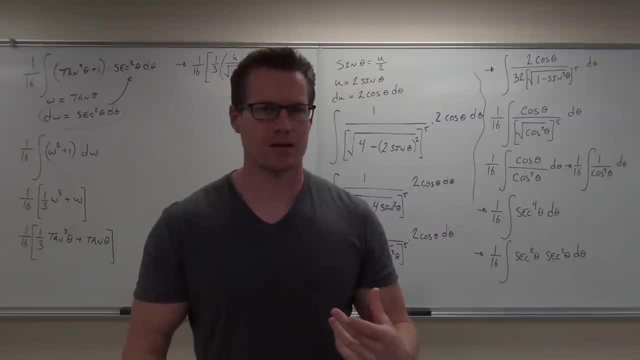 OK, you try to make one fraction out of this right now. instead of plugging in, x is 0.1.. You plug in the x's first. all right, So we get all the way down to as simple as we can with u's. 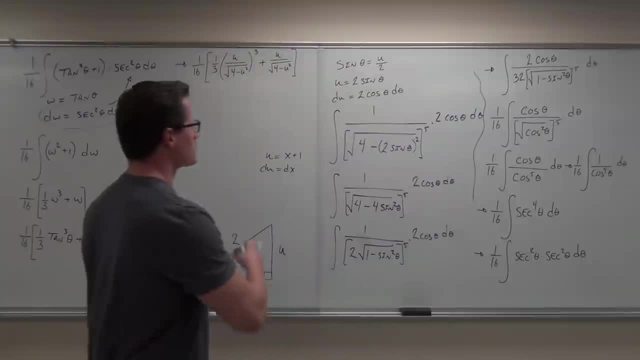 Then we plug in the x's. Does that make sense to you? So if you choose to do that, so this may or may not look like what it is in the back of your book. It might look different. They might find a common denominator here. 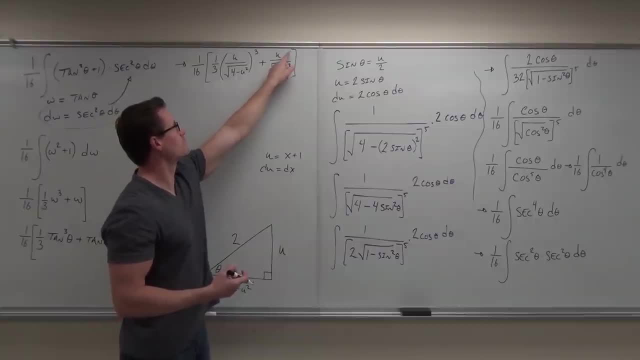 It wouldn't be super hard to do. You'd multiply this by 3 and another 4 minus u squared factor, And you can find a common denominator, get one fraction out of it And then you plug in your x's. You follow. 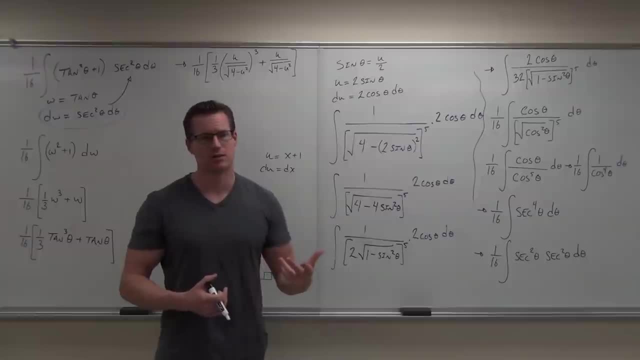 OK, So that's the idea. Now, for the sake of time, I'm not going to do that I usually do on this problem to show you how insane it gets with your algebra. But I'm not going to. That's going to be on u. 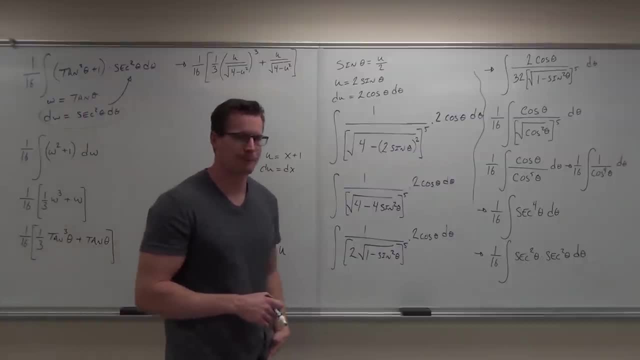 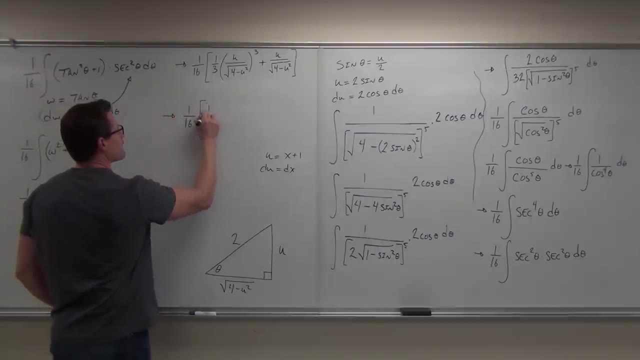 What I'm going to do is do one more thing. What am I going to do? Use one of the x's. Are we still keeping the 16 outside? You can distribute, You can keep it outside. I'm going to keep it outside just for the sake of seeing. 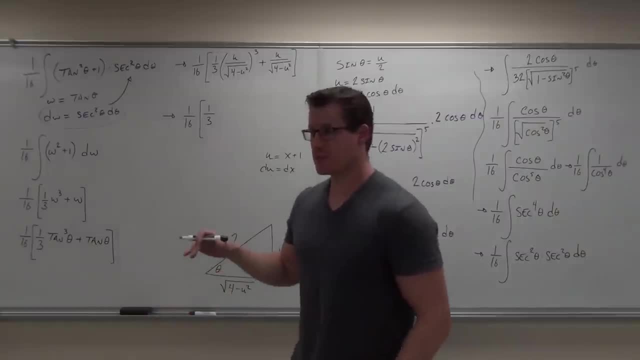 where everything's coming from. OK Again, If you were to simplify this, you would do it here before doing what I'm doing right now, Because otherwise you'd have a lot of different terms of x plus 1. You're changing every u into two terms. 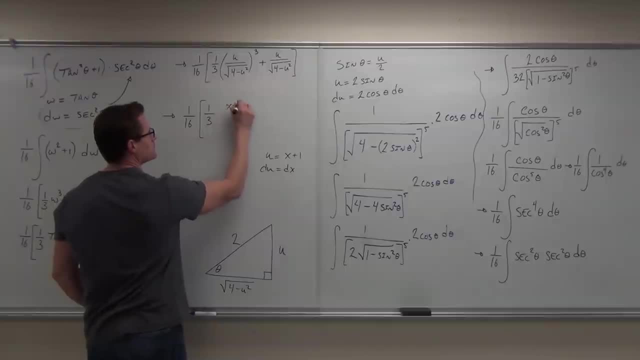 That gets kind of crazy. So we'd have an x plus 1.. We'd have 4 minus x plus 1 squared, And then that's under square root And this whole thing is raised to the third power. Then we'd have another x plus 1.. 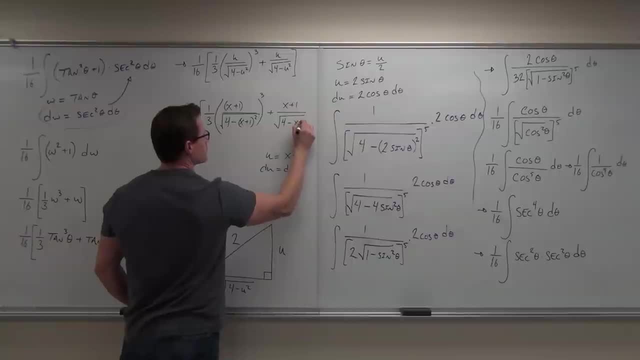 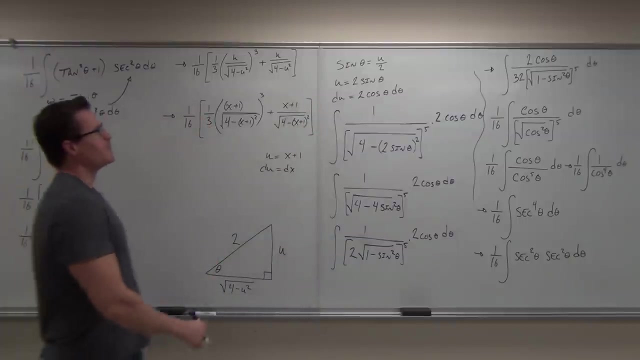 We'd have 4 minus x plus 1 squared. That's too small And that's what we would deal with. Plus c, Plus c, Plus. we know I'm not, Did you get it? Yeah, Yeah, Follow it. 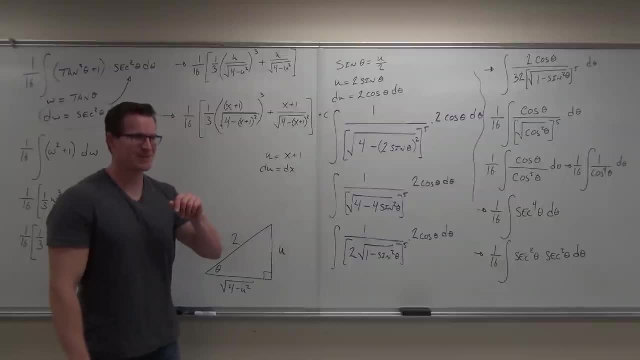 Do you want to simplify this one and see what you get? No, sir, You sure We can do it if you really want to. No, Do you know how to Yes, No, No For some of you, sadly, that's true. 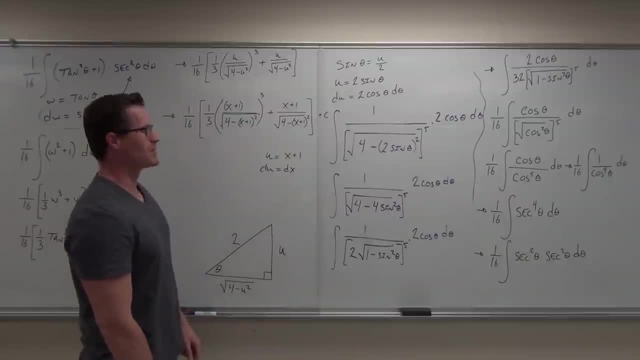 Oh, Oh. it kind of makes me want to right now: Go for it, Go for it, Yeah, No, Of course you say no, No way I know, And then I just completely say I'm going to anyway. 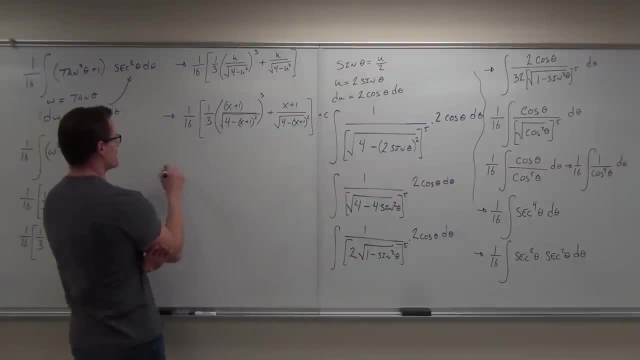 Forget you guys. Ha ha ha. Oh, let's see. If I were to do this, Here's how I would do it. I would think of this as u cubed over 3 square root of 4 minus u squared to the third. 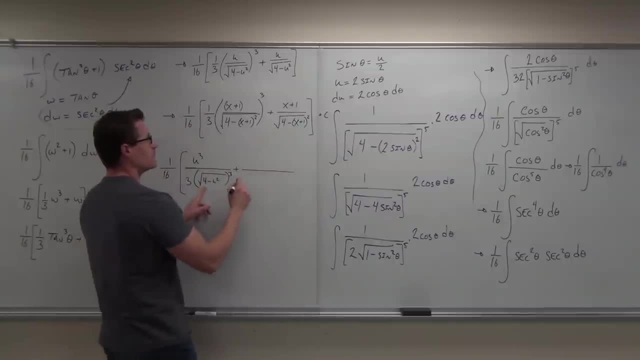 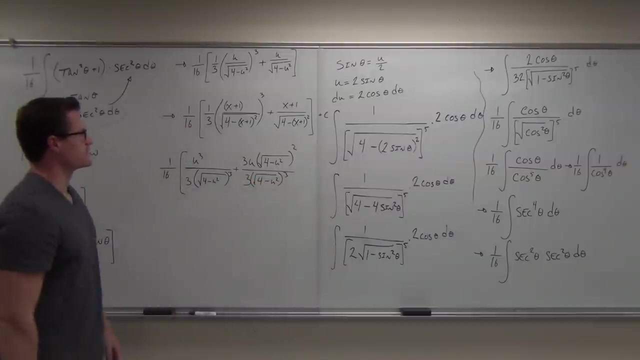 I would multiply this by 3 and 4 minus u- squared- squared on both the numerator and denominator. OK, That would change it to a third. If you simplify it, you can see that I'm right. This would cross out all but one of those. 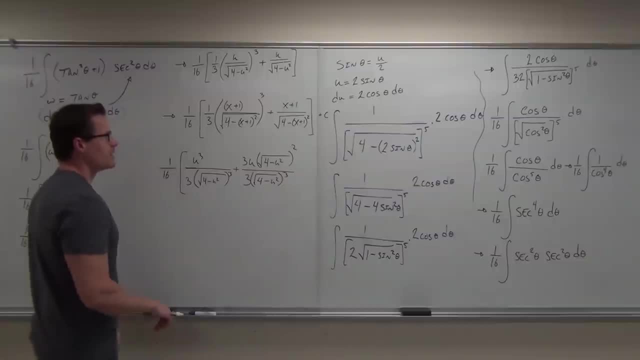 This would cross out. You'd have just the u. So this is the same. After that you do a little bit of simplification. We'd get 1, 16th, We'd get u to the third, You'd get 3,. bunch of junk. 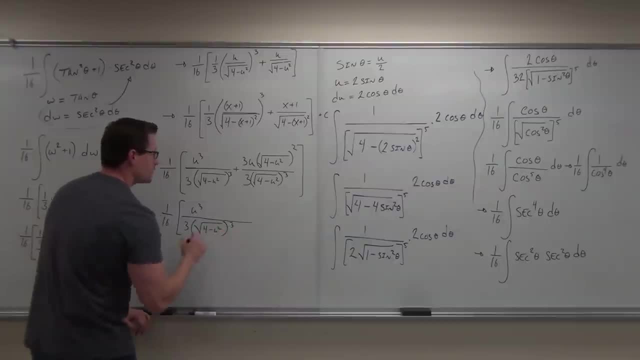 You'd get 2 to the third. This right here, square and square root are gone. We get plus 3u times 4 minus u squared. Are you still with me? You catch me if I've made a mistake. Sometimes this happens. 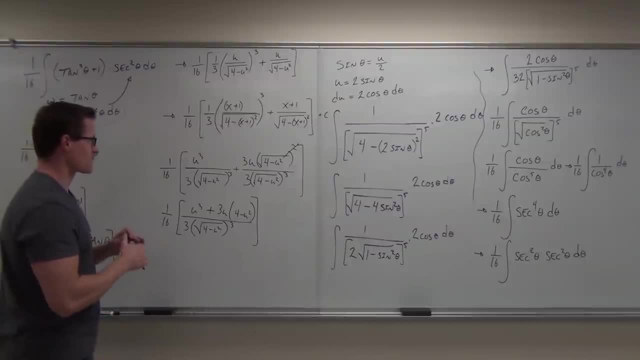 It happened to me once earlier today. After that, a 1- 16th, We'd have 3 times 4 minus u, squared to the third. We'd get 3 times 4 minus u, squared to the third. You catch me if I've made a mistake. 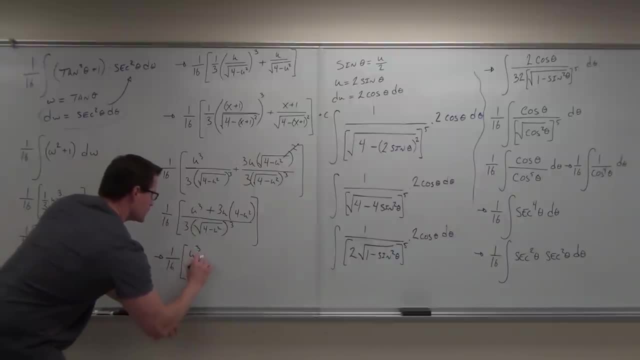 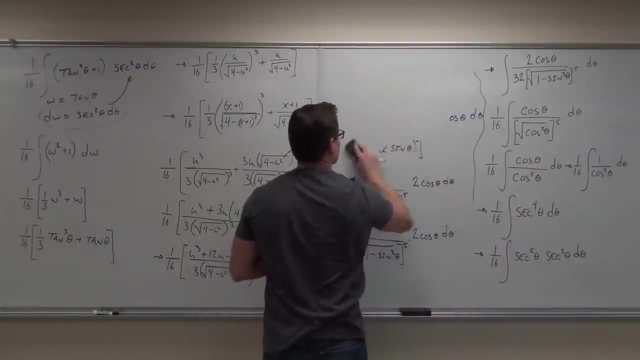 Sometimes this happens We'd have a u cubed plus 12u minus 3u to the third, over 3 square root of 4 minus u squared to the third. After that, combine your like terms if you can. I got a 1 16th. 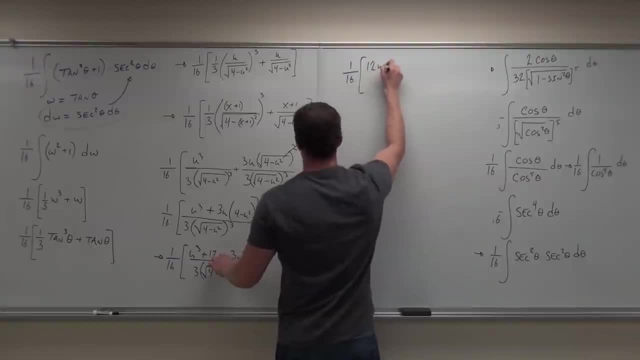 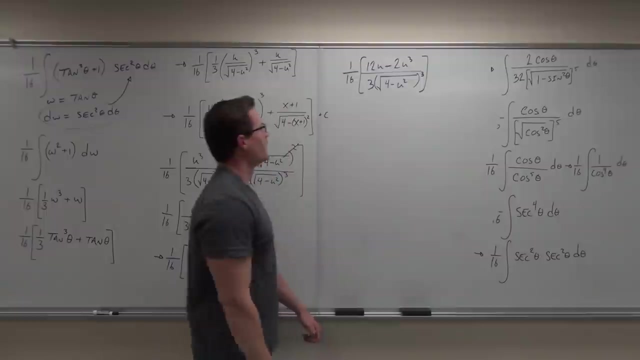 Doesn't really matter how you do this, but I'm going to have a 2- 16th, 12u minus 2u to the third over same stuff. That's as simple as we can make it right there, Not as simple. 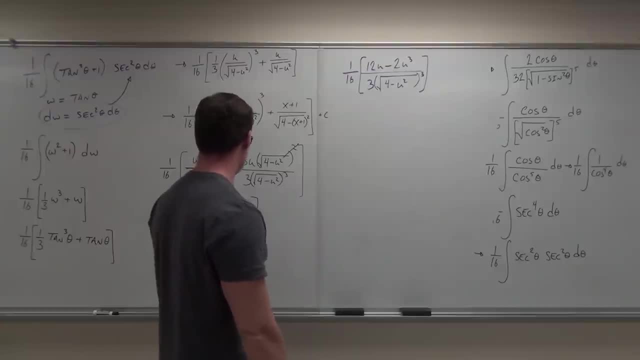 We could factor out a 2 if we really wanted to. That might be a good idea. So factor out a 2.. Then what we would get is 1- 8th. That's a good idea. When I come back next week. I could get 1 8th. That's a good idea. So when I come back next week, I could get 1 8th. I could get 1 8th. I could get 1 8th. 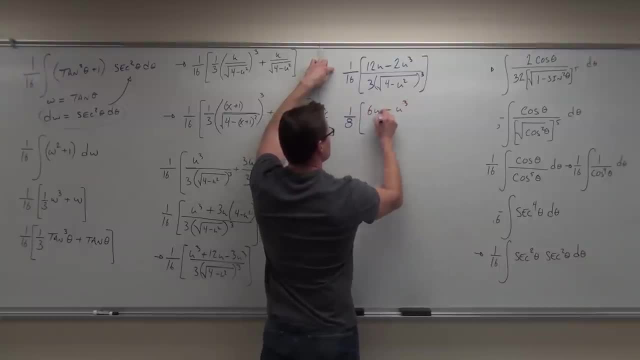 If I did, If I did 6u minus 2u to the 3rd, Say what? What did I say? You said 2u to the 3rd. Well, obviously it's u to the 3rd. 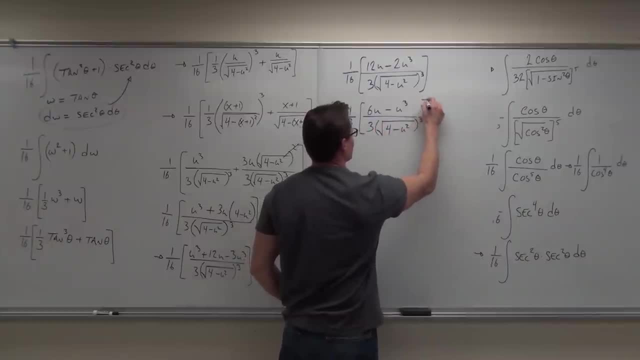 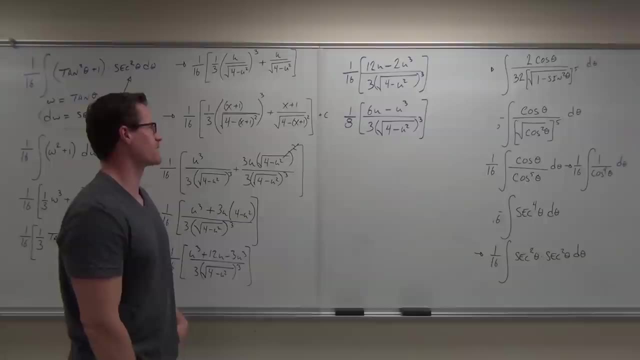 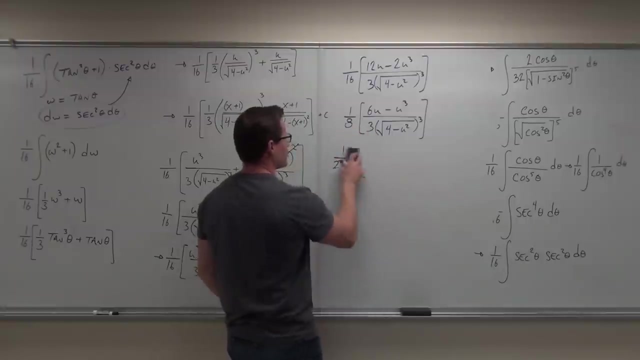 You told us to catch your mistakes. You did. yeah, Okay, that's as simple as we can make it. Well, not really. we can factor out the 3 too, One over 24.. Let's just do that here. okay, We'll get rid of this 3, we'll make that. 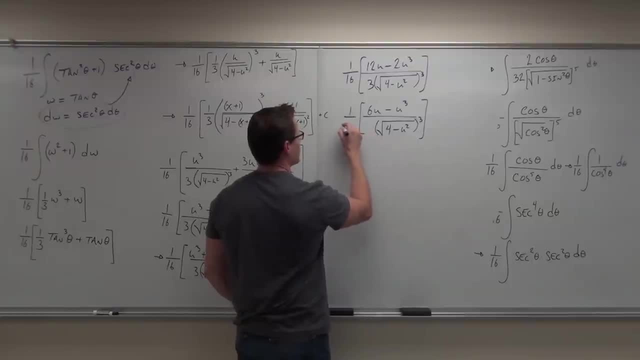 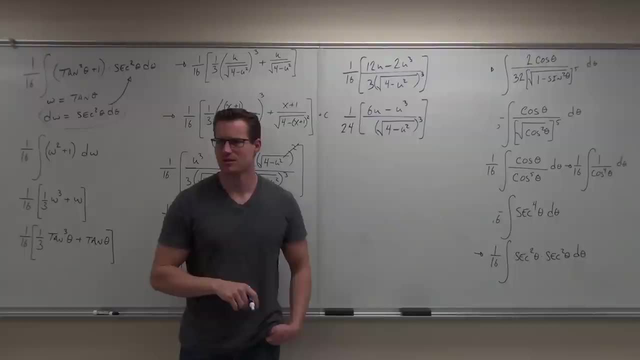 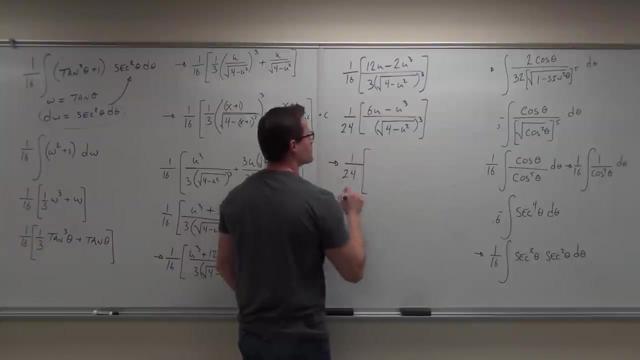 a 24.. Are we still okay? so far? Is all my algebra right? I certainly hope it is Not, yet I'm going to do the x's. Bless you, Thank you, Bless you, Thank you At this point, when you've had it simplified here's. 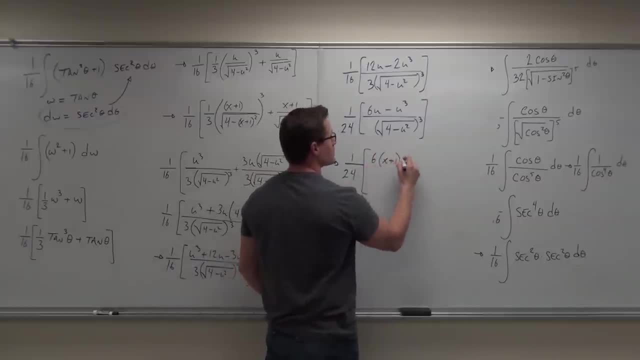 when you plug in x plus 1, so 6. x plus 1 because u is x plus 1.. Minus x plus 1 to the 3rd power, All over 4 minus x plus 1. squared Square root. 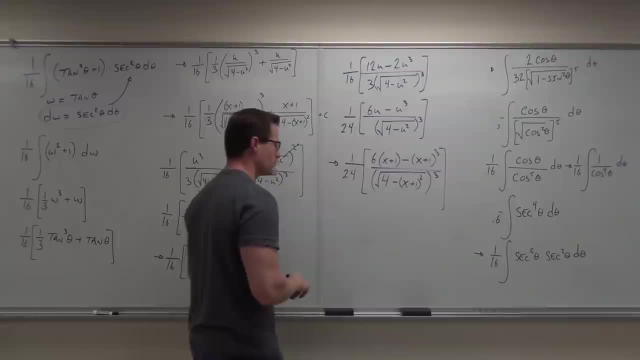 to the 3rd. We can't. No, we can't. We still have the square root. I'm going to leave this as 3 halves power. I am going to simplify this one Because I want to show you that what you're going to get back is exactly what we started with. 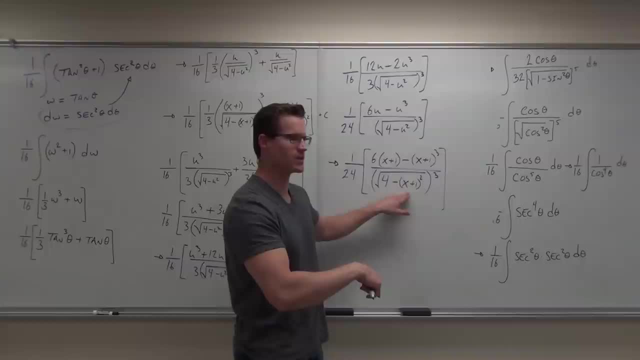 3 minus 2x plus x squared Or minus x squared, It's going to be the same. So if I do this, this will be 1 24th. We got it. We got a 6x plus 6 minus. 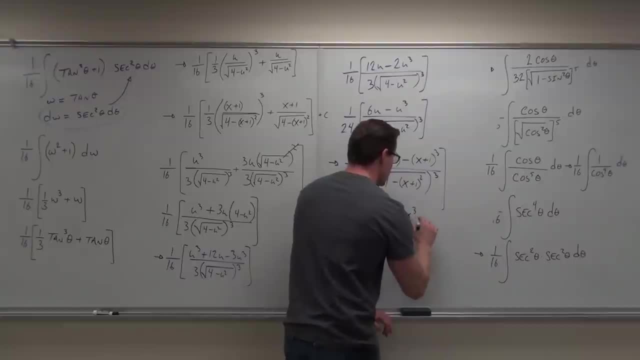 if you're going to distribute that, it's 3x squared plus 3x plus 1.. But that's inside parenthesis. Here we got square root of 4 minus x squared plus 2x plus 1.. In parenthesis, This should be the 3rd. 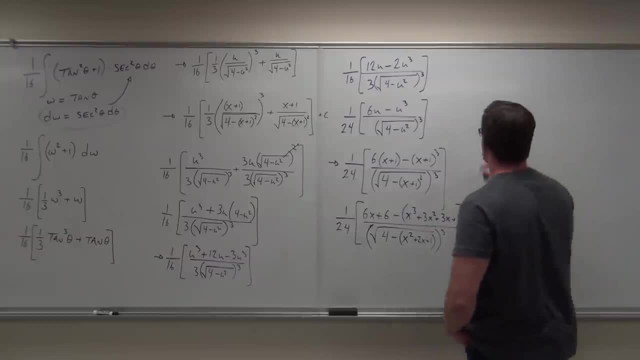 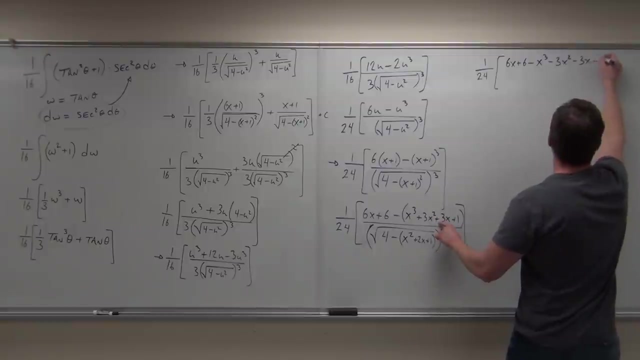 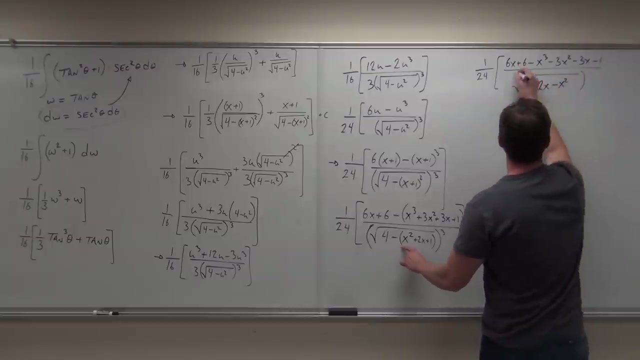 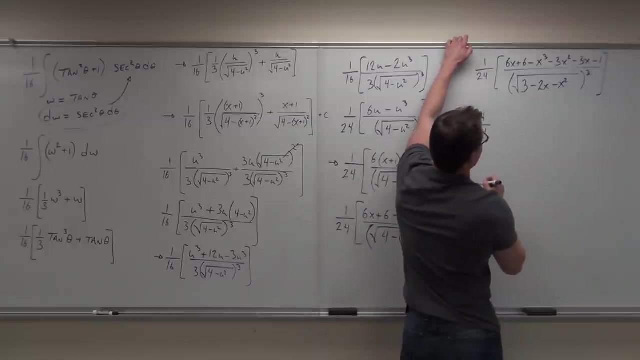 Moving on, Distribute your negative and then we'll combine some like terms: Almost done. So let's see, here We've got a 5., We've got plus 3x, We've got a minus 3x squared And a minus x cubed. 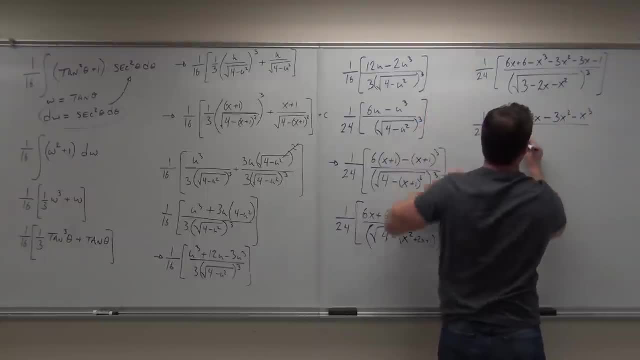 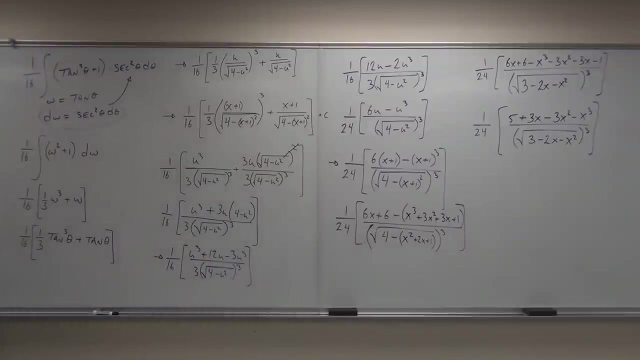 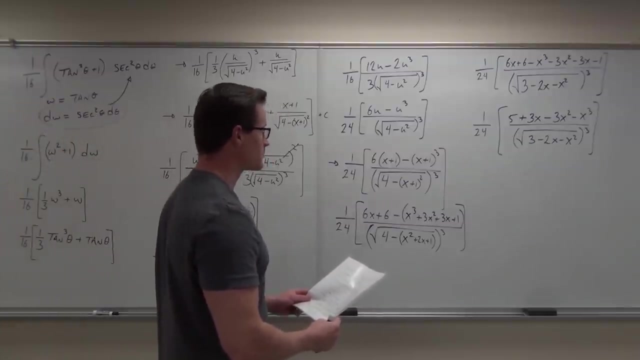 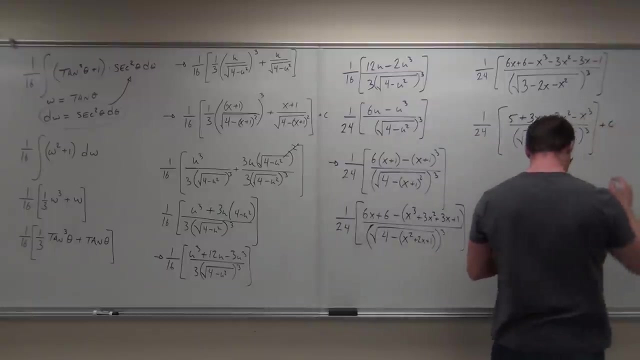 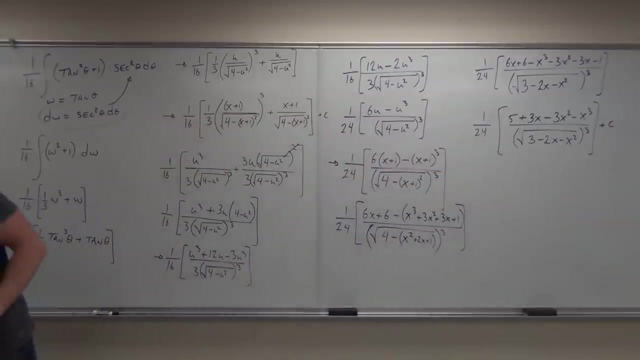 Can you double check my combined like terms for me please? Yes, no, Now it's a plus 3.. I think good, So it's about a test. So I want this. No, Alright, I just want you to see what potential you can get out of this thing. 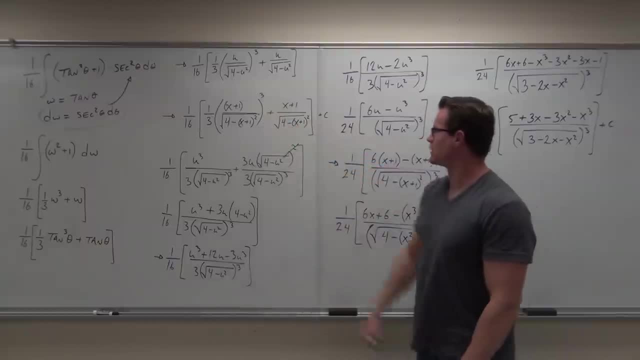 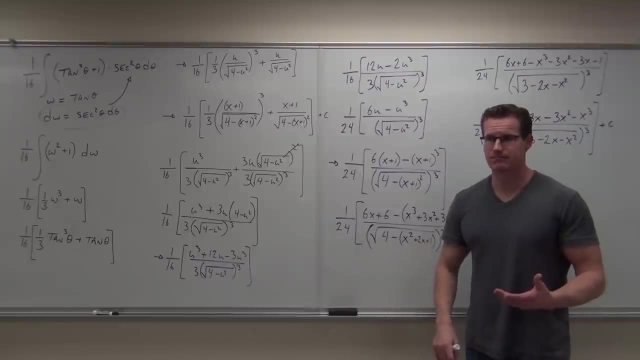 We stopped right here. You need to see that this and this are equivalent by algebra. They're the same thing. So can your answer look a little different? It would be the same. This is simplified. You can actually factor out an x plus 1 here. 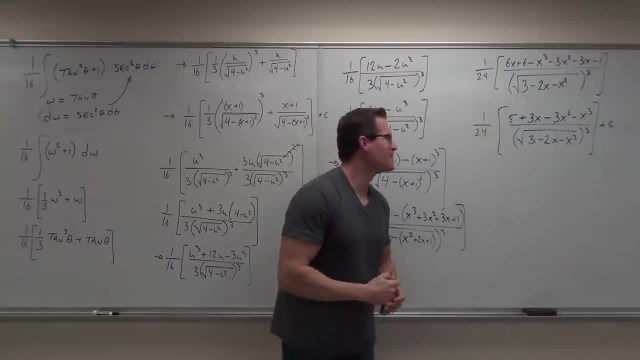 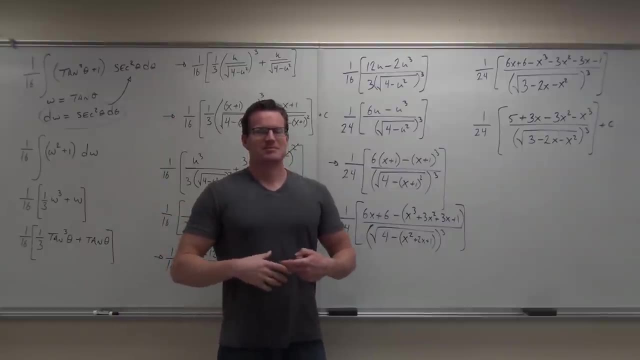 So if you factored that out, then it would be simplified. But that's the idea. Alright, Take a deep breath. We're done with trig sub For like 10 minutes. Well, here's the point. You now have a whole bunch. 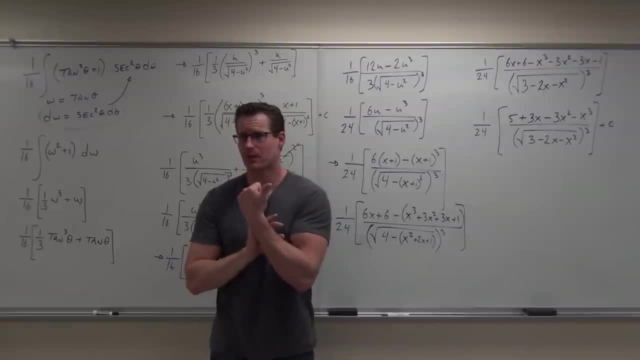 of integration techniques, right. We know substitution. We know integration by parts. We know how to do trigonometric integrals. We know now how to do a trig sub. All those play of. Oh, we know integrals of inverse trig functions, right. 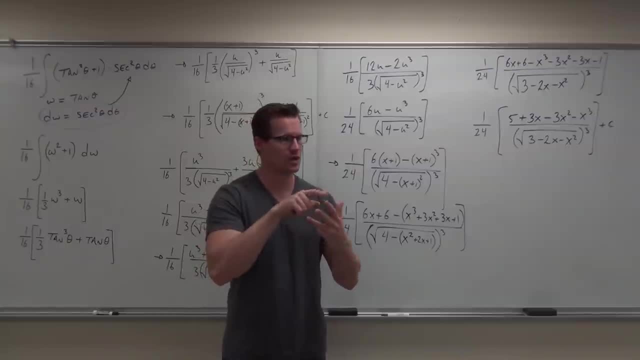 And hyperbolics and all that stuff. All those things play a part in the following sections. All of them, We're going to use all of them. That's why we did integration techniques, so that when I give you an integral, you can do it.